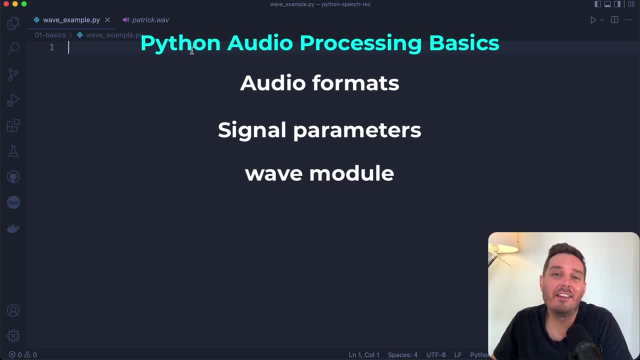 Then I show you how to use the WAV module to load and save a WAV file. Then I show you how you can plot a WAV signal. Then I also show you how to do a microphone recording in Python. also show you how to load other file formats like mp3 files. So let's get started. So first of all, 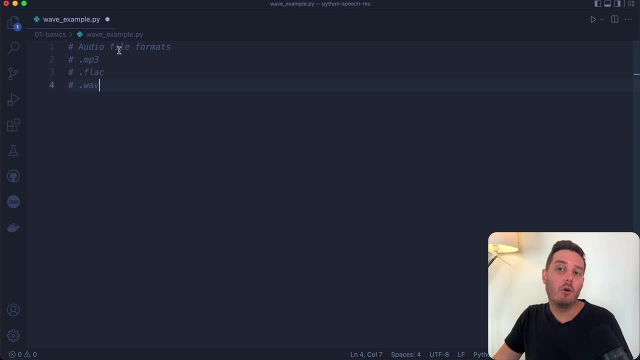 before we write some code, let's talk briefly about different audio file formats, So here I've listed three of the most popular ones: mp3, FLAC and WAV. mp3 is probably the most popular one that you may know, And this is a lossy compression format, So this means it compresses the data. 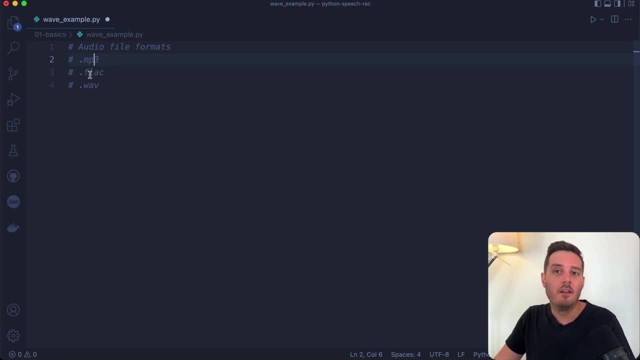 And during this process we can lose information. On the other hand, FLAC is a loss less compression format, So it also compresses the data, but it allows to perfectly reconstruct the original data. And WAV is a uncompressed format, So this means it stores the data in an uncompressed way, So the 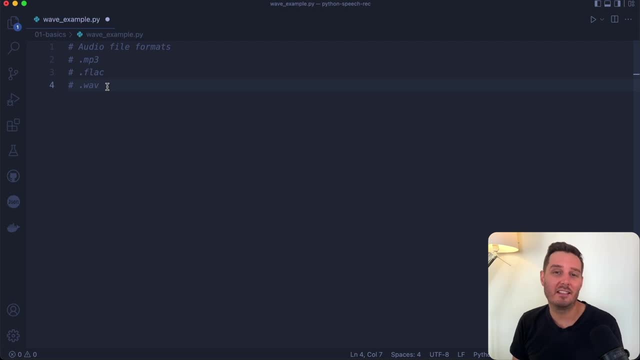 audio quality here is the best, but also the file size is the largest And WAV is the standard for CD audio quality. So we focus on this in the first part, because it's actually very easy to work with this in Python because we have a built in WAV module, So we don't have to install this. And now let's. 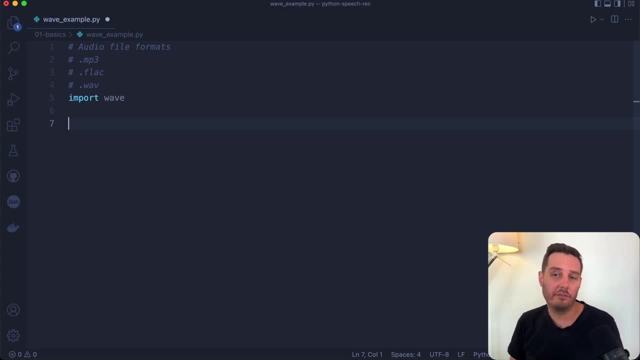 have a look at how we can work with a WAV audio file. By the way, WAV stands for waveform audio format, And before we start loading some data, let's talk about a few parameters that we have to understand. So, before we load our first WAV file, let's understand a few parameters. So we have the 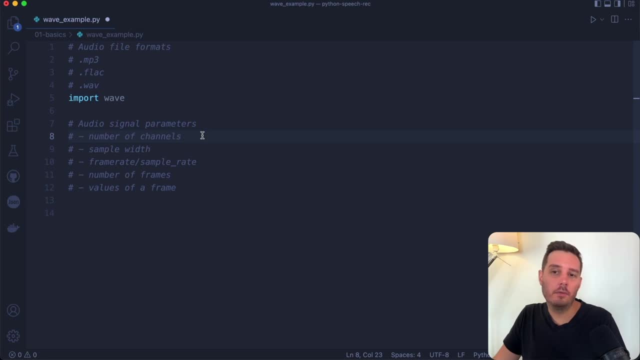 number of channels. this is usually one or two, So one is also known as mono and two is stereo. So this is the number of the independent audio channels. for example, two or stereo has two independent channels And this means it gives you the impression that the audio is coming from two. 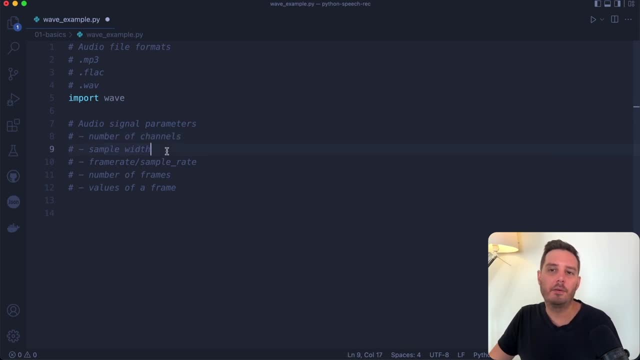 different directions. Then we have the sample width. This is the number of bytes for each sample, So this will get more clear later when we have a look at an example. And then we have the frame rate, which is also known as the sample rate or sample. 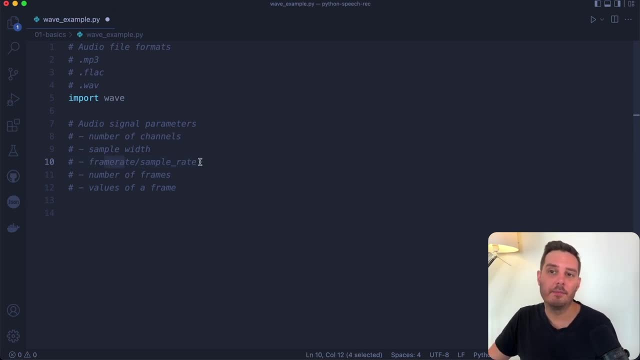 frequency, And this is a very important parameter. So this means the number of samples for each second And, for example, you may have seen this number a lot. So this means 44,100 hertz or 44.1 kilohertz. This is usually the standard sampling rate for CD quality. 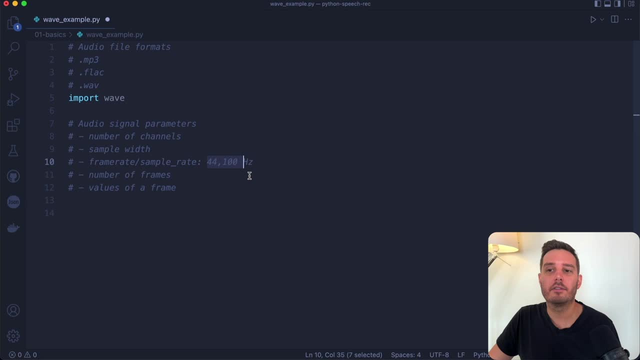 So this means we get 44,100 sample values in each second, And then we have the number of frames. So yeah, this is the total number of frames we get, And then we have the values in each frame. And when we load this, this will be in a binary format, But we can convert this to integer values. 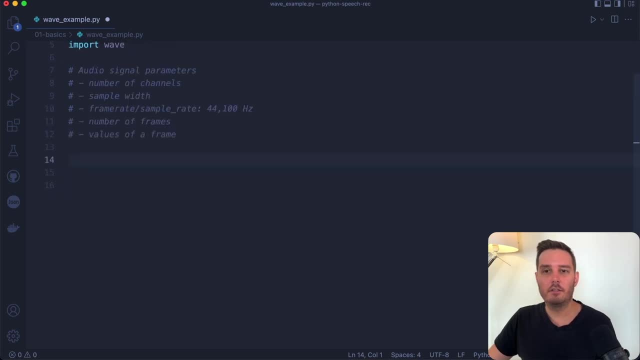 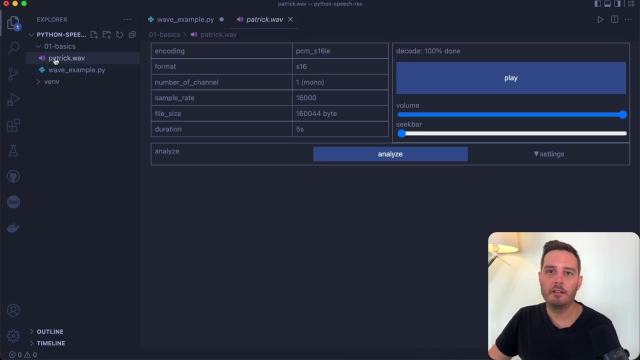 later. So now let's have a look at how to load a file. So with the WAV for WAV module. So here I prepared a simple WAV file, So this is five seconds long, So let's actually listen to this. Hi, my name is Patrick and I'm a developer advocate at assembly AI. 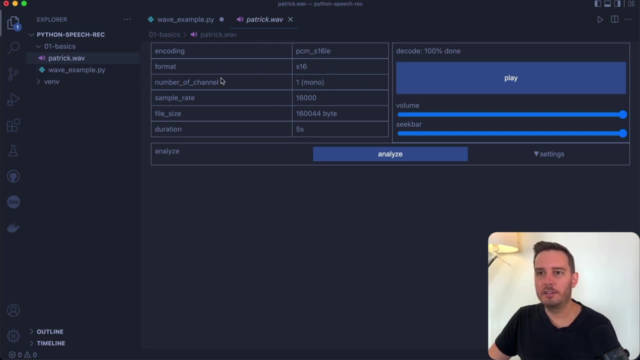 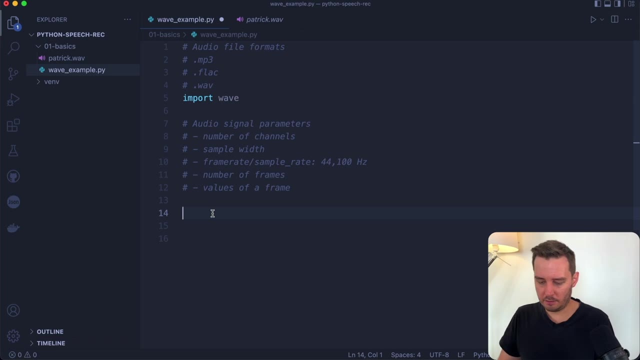 And yeah, here we also see a few parameters already. So now let's go back to the code and now let's load this file. So for this we create an object and we simply say wave dot open. then we have to give it the name. So this is called Patrick dot wave. And to read this: 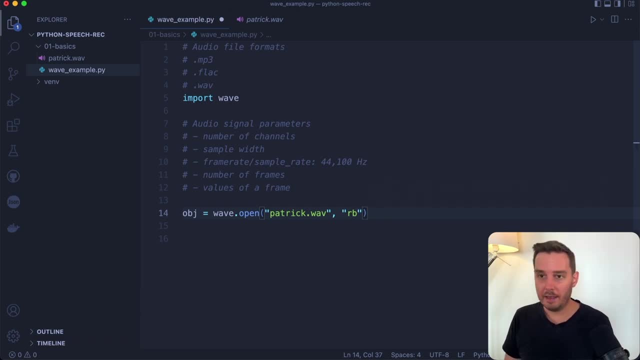 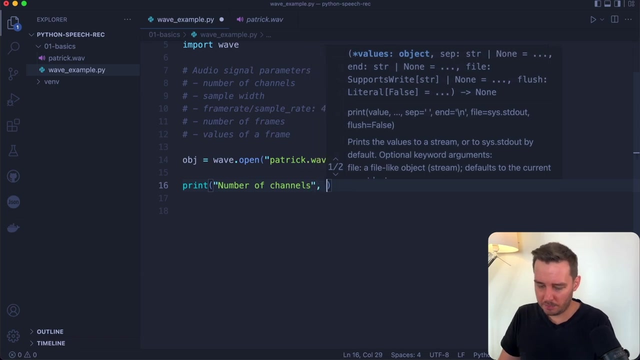 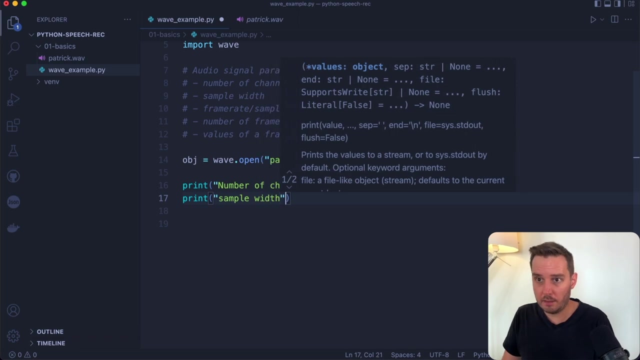 we say we read this in read binary And now we can extract all these different parameters. For example, let's print the, let's say the number of channels, And we get this by saying object dot get n channels. then we also want to print the sample width, So print the sample width. 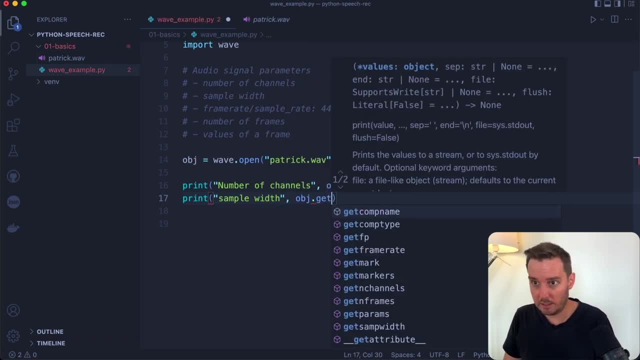 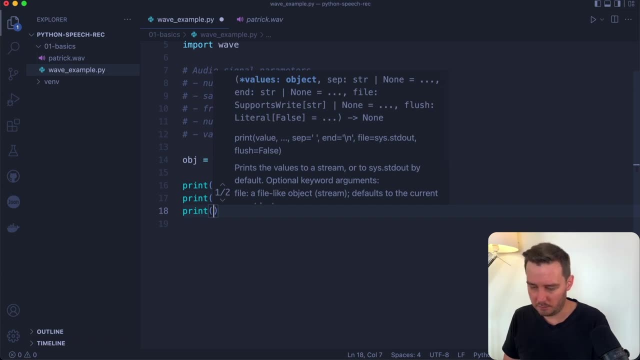 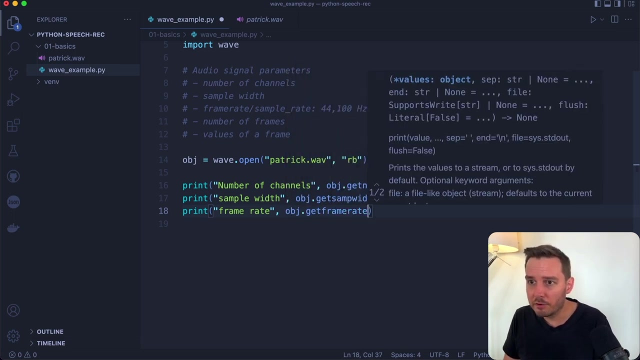 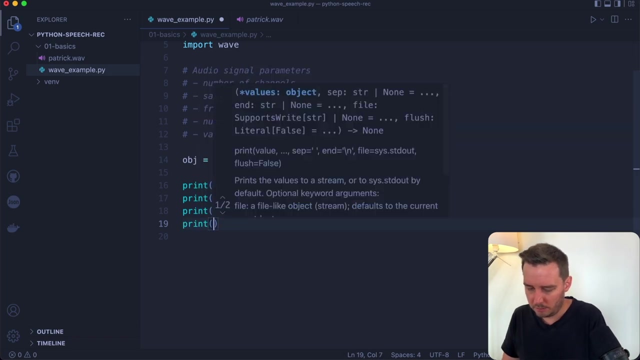 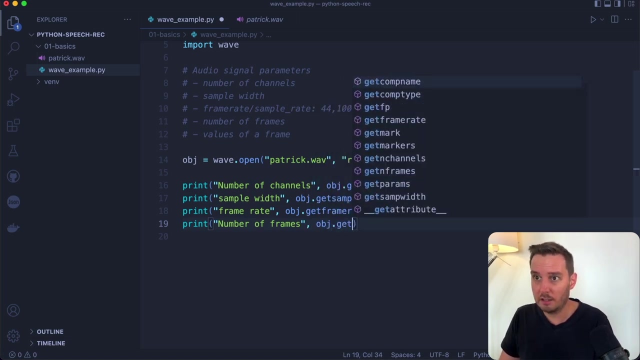 and we get this by saying: object dot get Sam with. then let's print the frame rate. So print frame. and we get this by saying: object dot get frame rate. then what do we also want? we also want the number of frames. So we print the number of frames and then we say objects dot get. 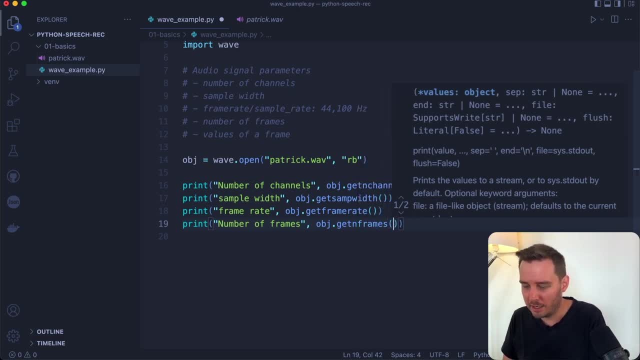 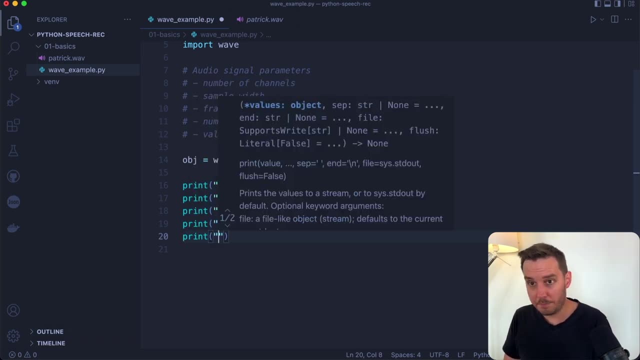 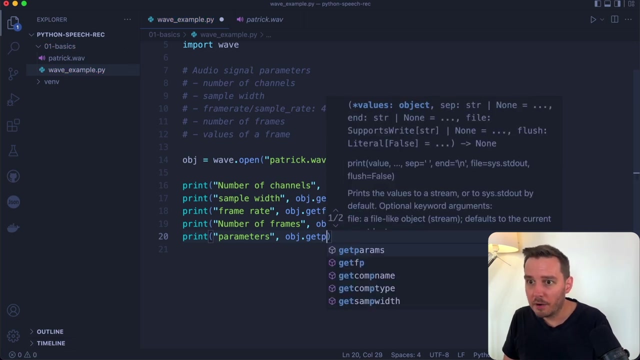 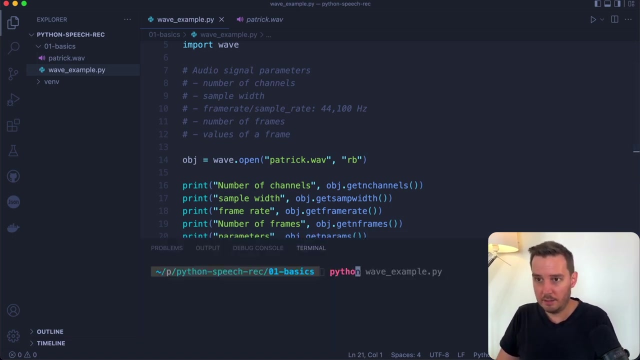 n, not dot n, channels and frames. And lastly, let's also print the all the parameters, So we can get all the parameters at once by saying object dot get par params. And now let's print this. So if we run this, so I say Python wave example: dot pi. 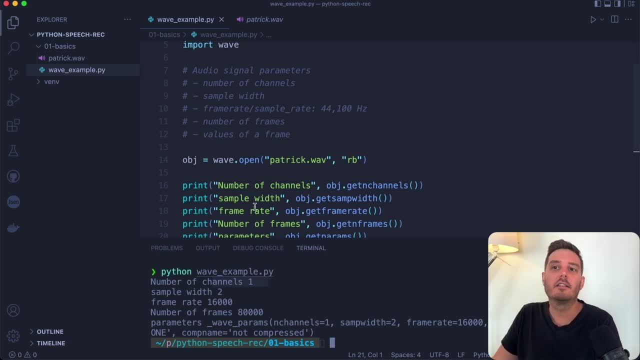 then we see we have only one channel, So this is a mono format. we have a sample width of two, So we have two bytes for each sample. then we have a frame rate of 16,000, and a number of frames of 80,000.. And here we also have all the parameters as a 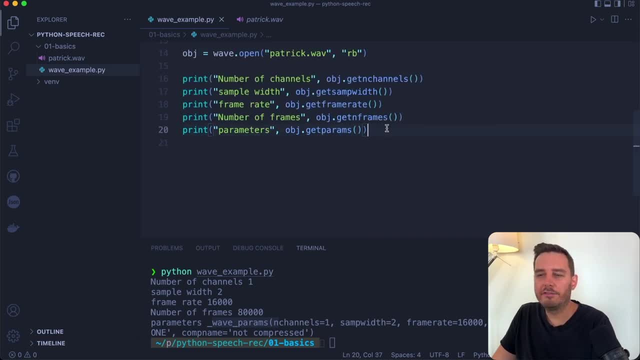 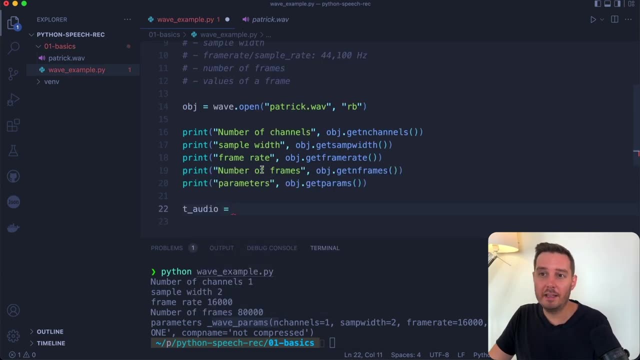 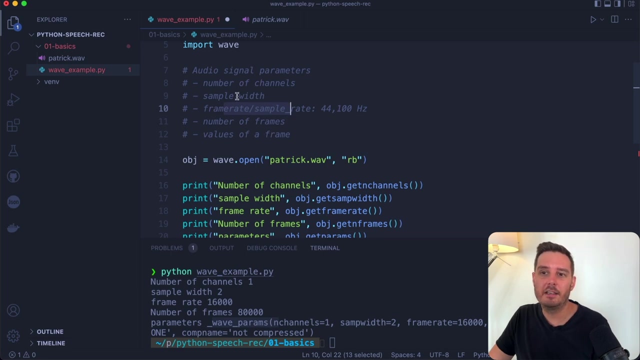 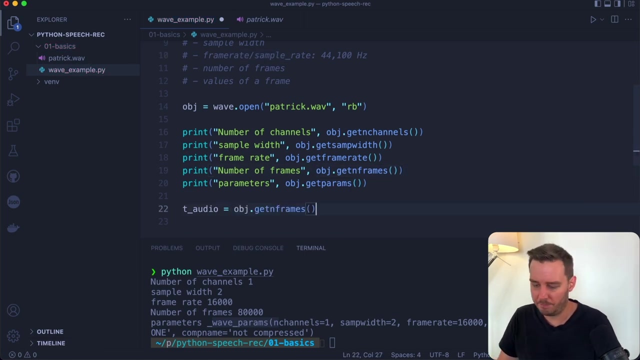 wave params object. So, for example, now we can calculate the time of the audio And we, as I said, the frame rate is the number of samples per second. So if we get the whole number of frames, so the number of frames or number of samples divided by the frame rate. 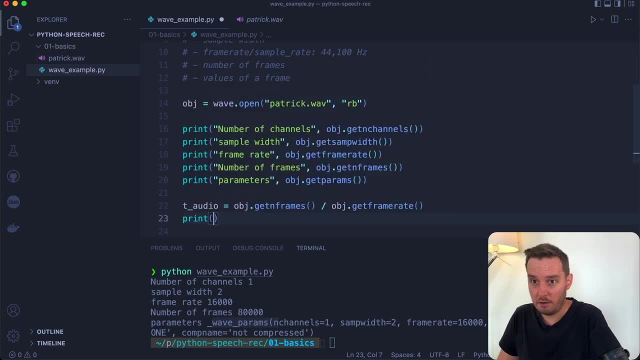 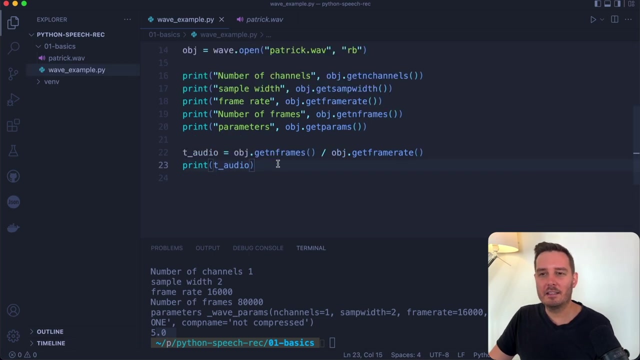 then we get the time in seconds. So now, if we print T audio and run this, then we get 5.0.. So five seconds. So this is the same that we see here. So this works. And now let's get the actual. 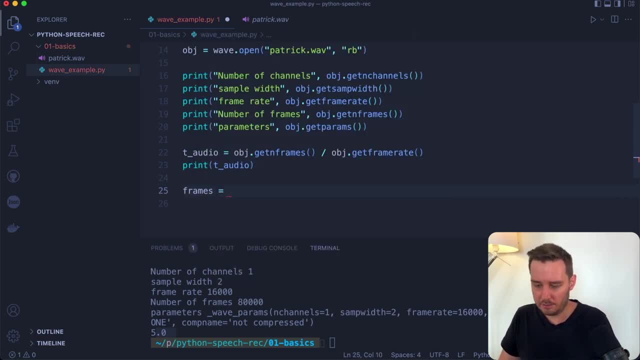 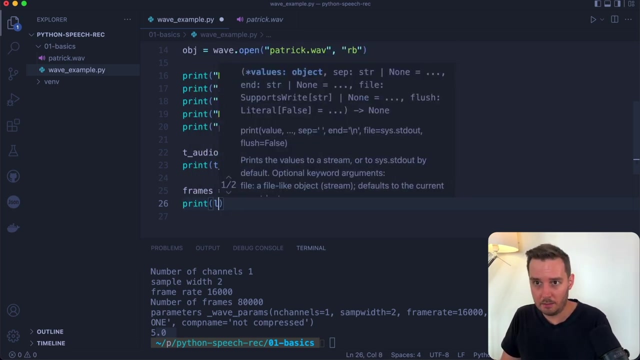 frames. So the frames equals object dot get frames. gets known sorry object dot read frames, and then we can give it the number of frames, Or we can- I think we can- pass in minus one. So this will read all frames And let's, for example, so let's print the type of this to see what this is. 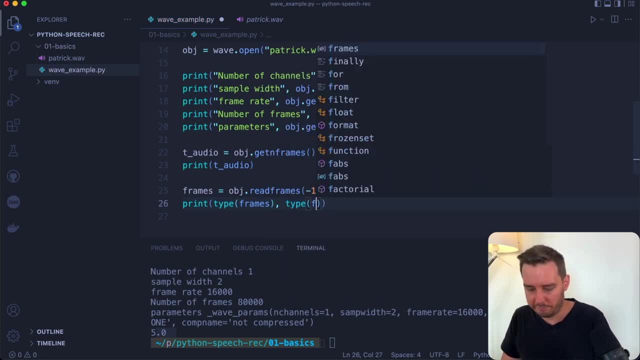 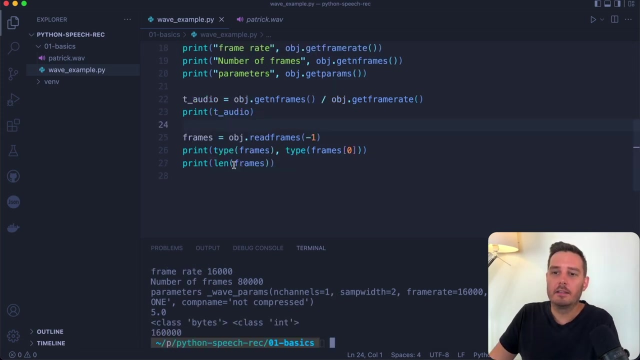 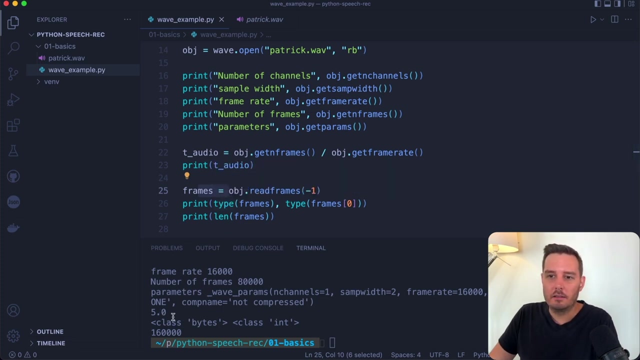 And then also print the type of frames- zero- And then let's print the length of frames. So now let's run this And then we see this is a bytes object, And so here we see class bytes, And when we extract the first byte then we get the number of frames And then we can also print the type of 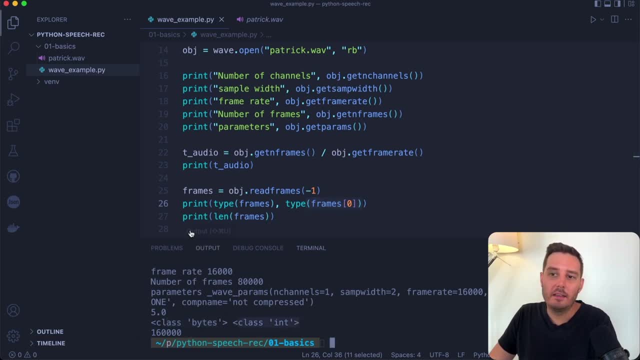 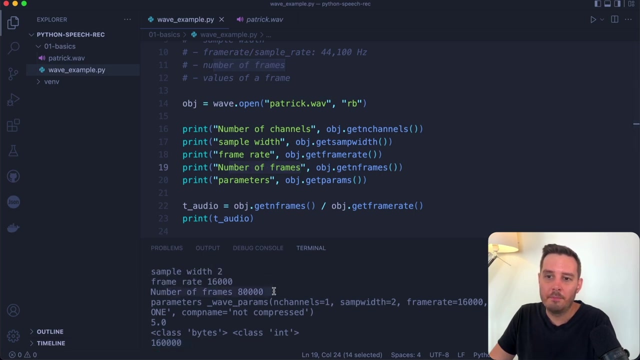 frames. And then we see this is a integer And now the length of the frames object is 160,000.. So this is not the same as the number of frames. So if we have a look here the number of frames is 80,000.. But if we extract the length here then this is twice as much. 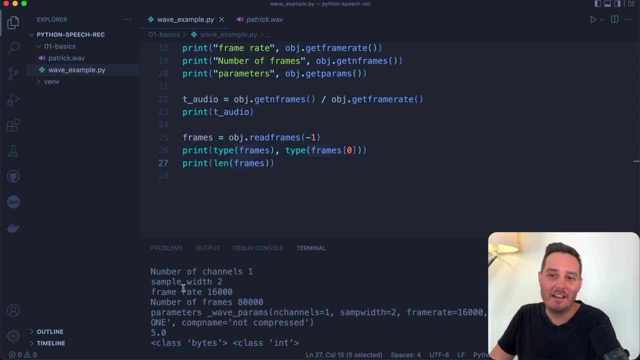 And if you listen carefully- in the beginning here I mentioned the sound- the number of frames is 80,000.. But if we look at the sample width, this means we have two bytes per sample. So now if we actually calculate this divided by two, then again we get our 80,000. 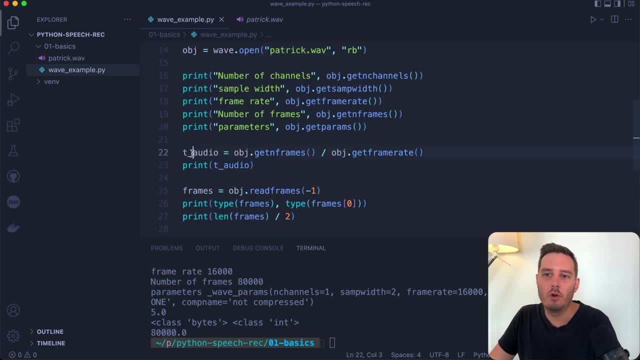 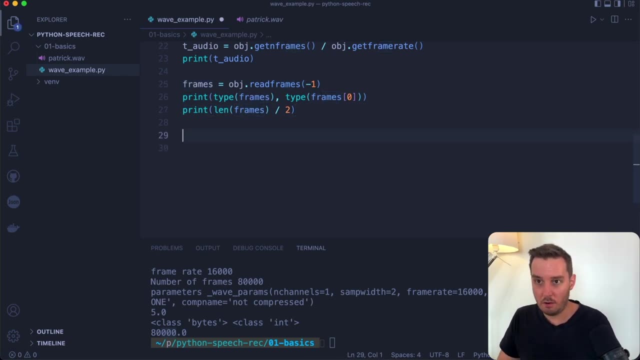 number of frames. And yeah, this is how easily we can read a wave file And then we can work with this and work with the frames, And now to load or to save the data. So our second step is to open. let's call this object. 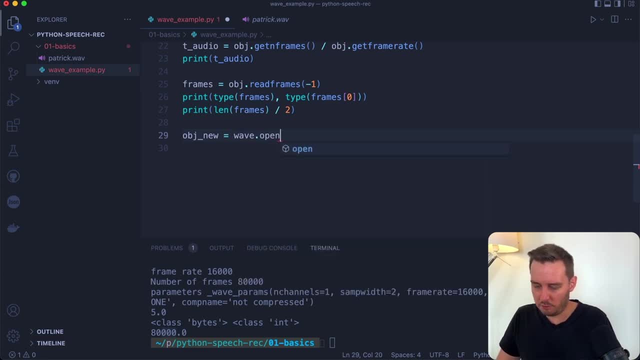 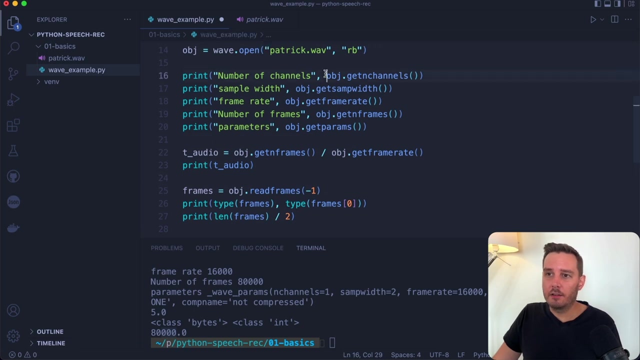 new equals and then we say wave, dot open. then we can give it a new name, let's say Patrick underscore, new dot wave. And now we open this in right binary mode And now we can basically call all those functions as setters and not as. 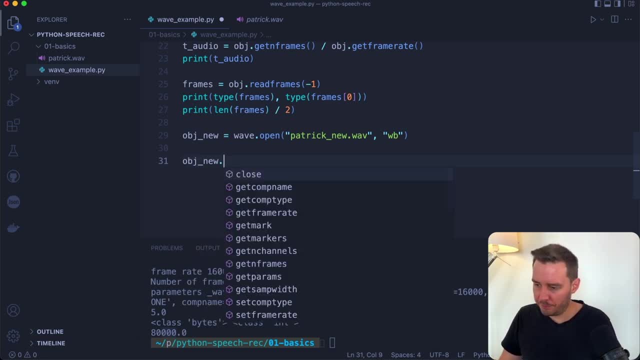 getters. So we say: object: new dot set. not getter, not getter, let's sayccent, I'm just going Scripture. number of channels. So this is only one channel. then we say: object: new dot set sample width. this should be to object: new dot set frame rate. this is 16,000 as a float. So these are all the. 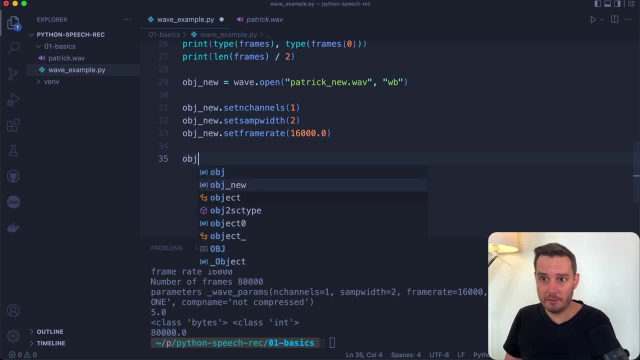 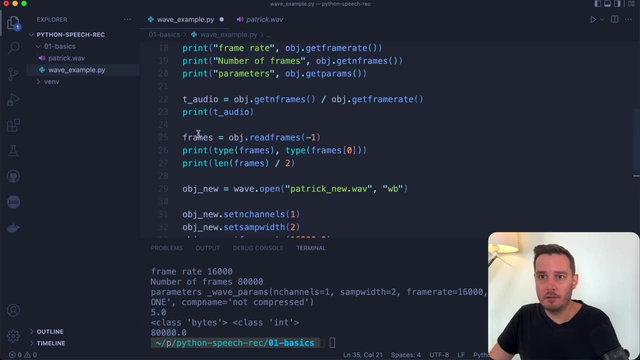 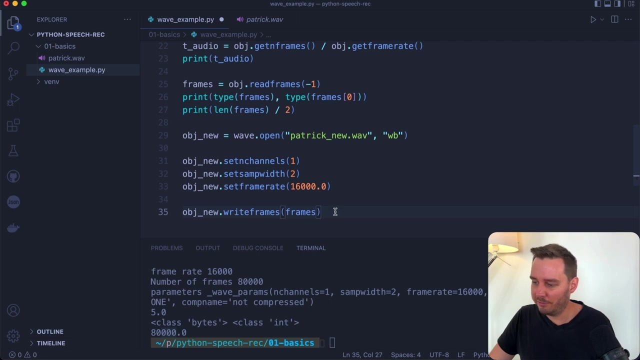 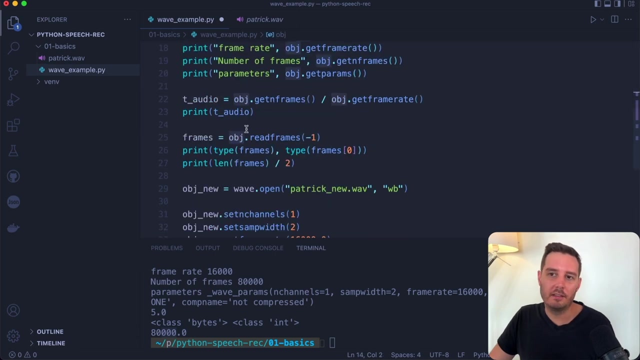 parameters we should set And then we can write the frames by saying: object: new dot right frames and then the frames. So here we have the original frame. So now, basically, we duplicate the file, So we write the frames and what I forgot. So when we are done with opening this and reading all the 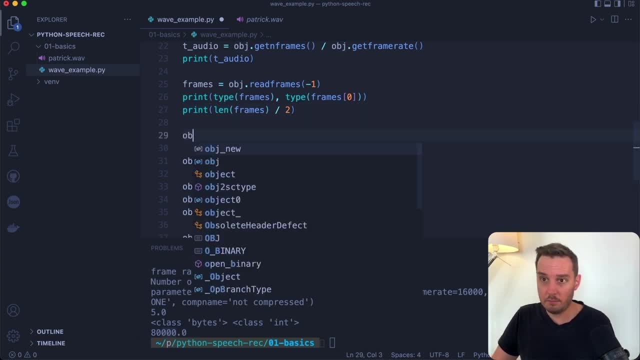 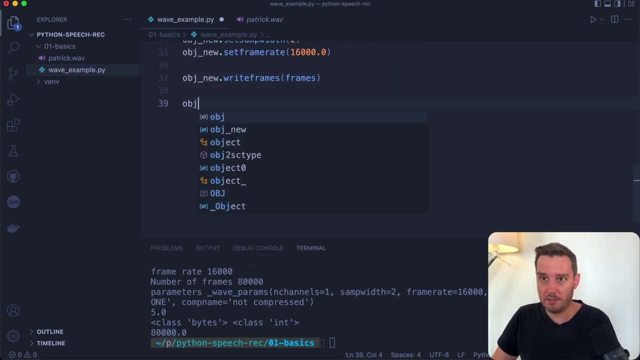 information we want. we all should also should call the object new dot set frame rate And then call object dot close, And then the same here. So here we say object new dot close And this will close the file objects. And yeah, so now if we save this and run this, then now here we see, we 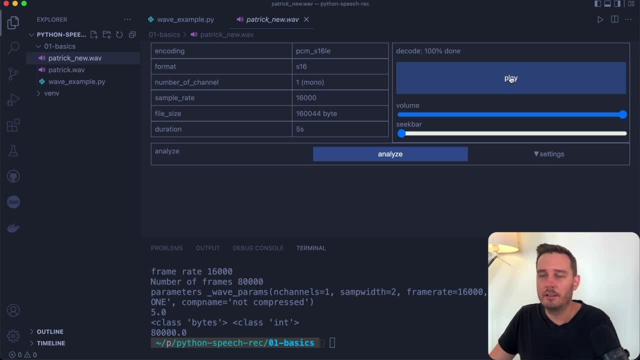 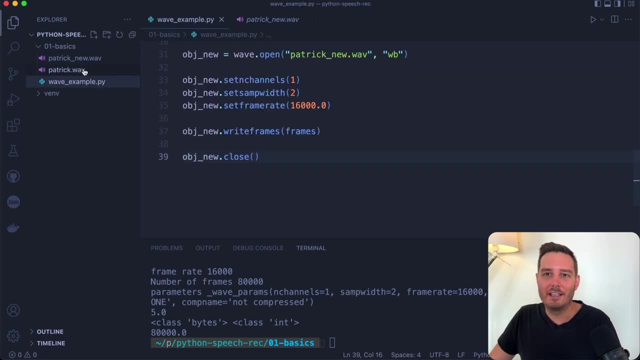 have the duplicated file And if we run this- hi, my name is Patrick and I'm a developer advocate at assembly AI- then we see this works And it has the same data in it. So yeah, this is how to work with a wave file and with the wave. 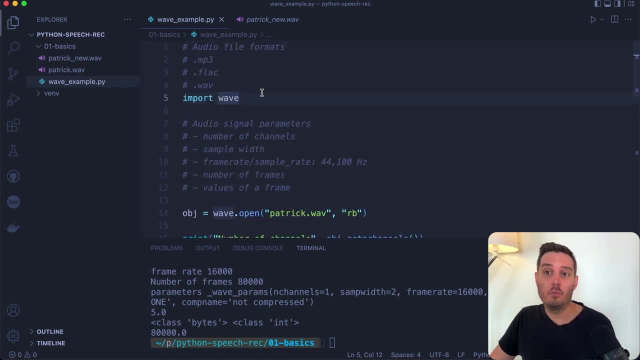 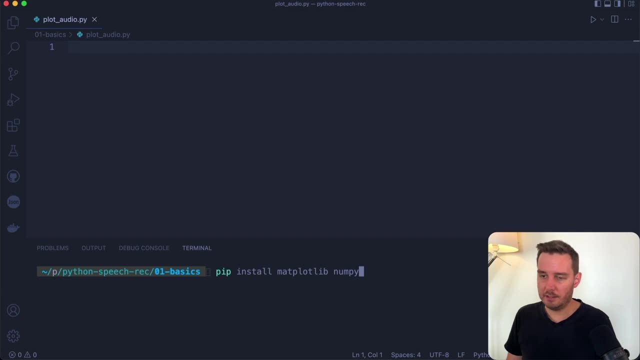 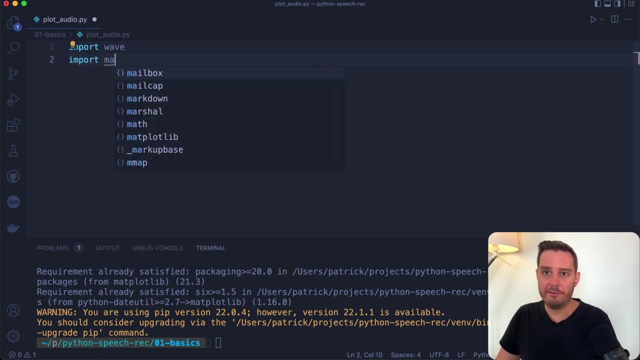 module. So now let's see how we can plot a wave file object. Now, plotting a wave signal is actually not too difficult, So for this we just need to install matplotlib and numpy. Then we import all the modules we need. So again, we need wave, then we need matplotlib, dot, pi, plot, s, p, l t. 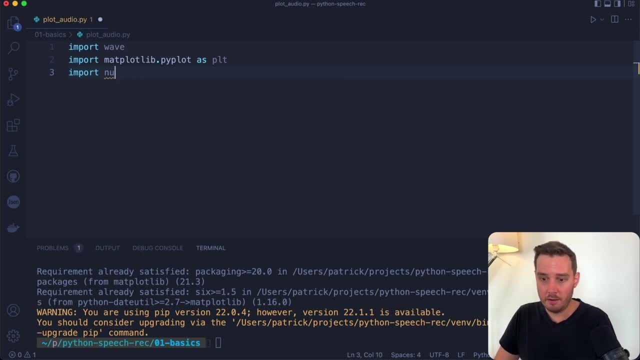 then we import numpy, num pi, s and P. then again I want to read the wave file, So I say wave dot open, And this was Patrick dot wave in read binary mode. then I want to read all the parameters that I need, So I want to read the sample frequency And this is object. 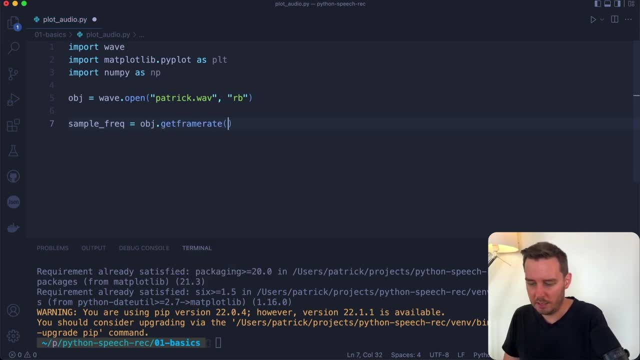 dot get frame rate. then I need the number of samples, So this is object dot get n frames. And then I also need the actual signal. So I call this signal: dot wave equals object dot read frames minus one, So all the frames, and then I can say object dot close. 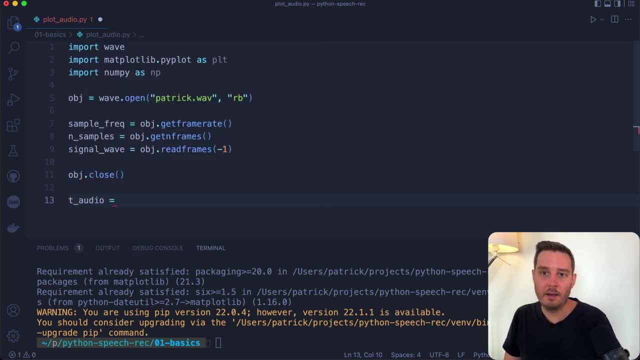 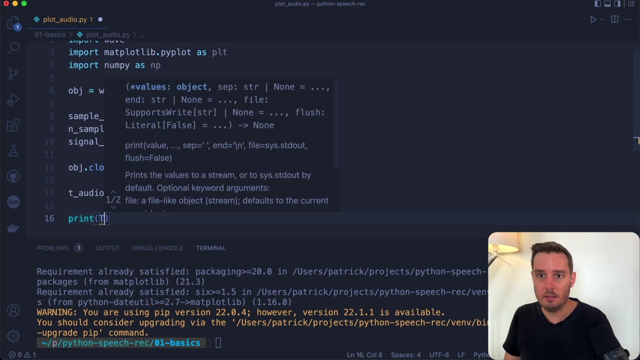 And then, for example, we can calculate the number on the length of the signal in seconds. So I call this T audio And, if you remember this from the first code, so this is the number of samples divided by the sample frequency. And now let's print the T audio and save this and run this. 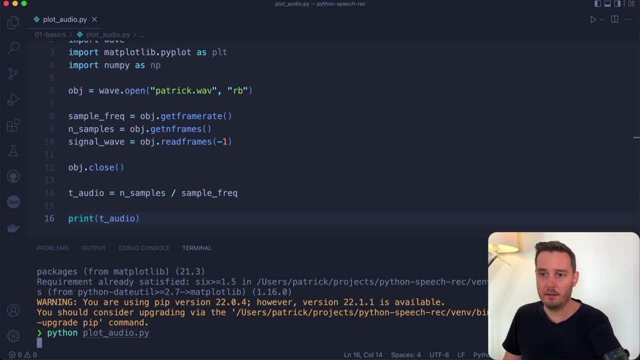 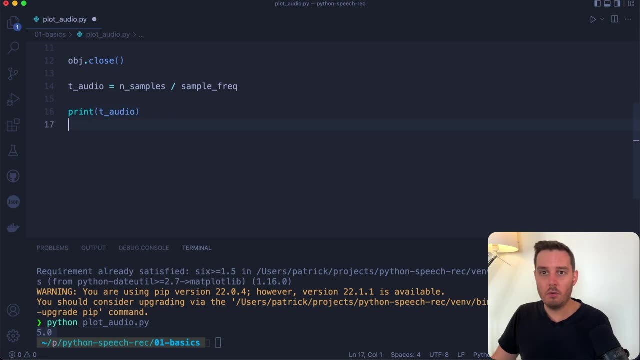 Just as a test. So now we can run Python plot audio and we get 5.0.. So this works so far. So now I want to create the plot. So this is a bytes object, so we can create a numpy array out of this very easily. So I call this signal array equals, and then we can. 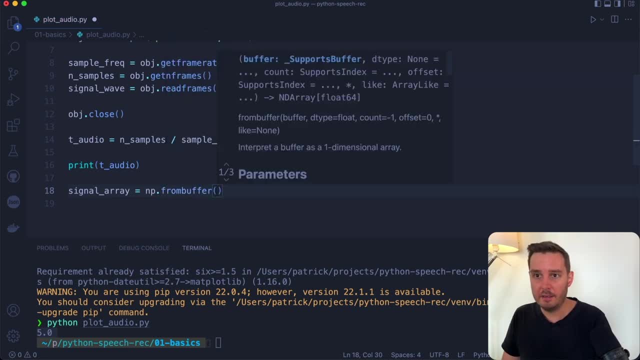 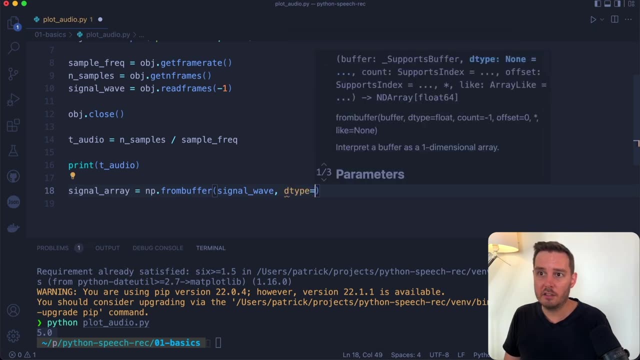 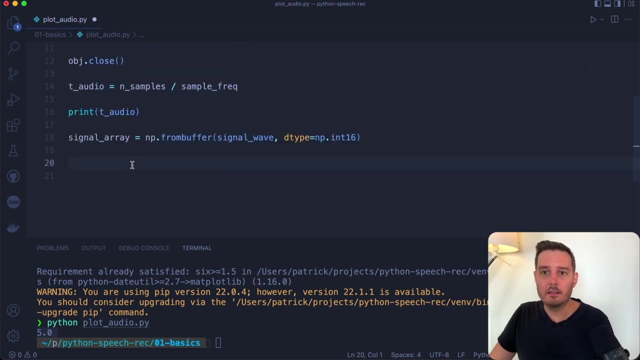 can use numpy from buffer And here we put in the signal, signal wave, And we can also specify a data type. So here I want to be to have this int 16.. And now we need an object for the x axis or the, so the times access. So we say times equals and here we use the numpy linspace function. 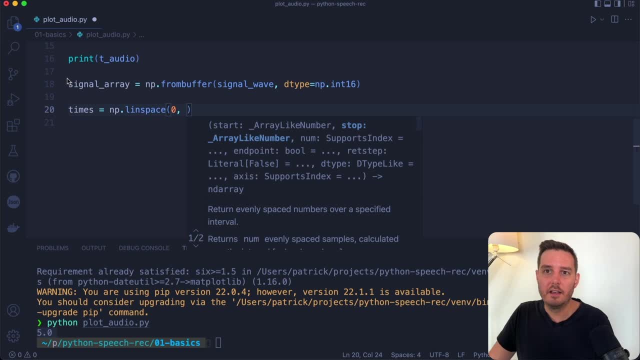 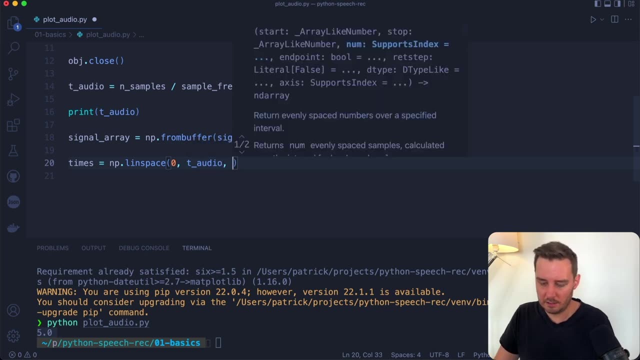 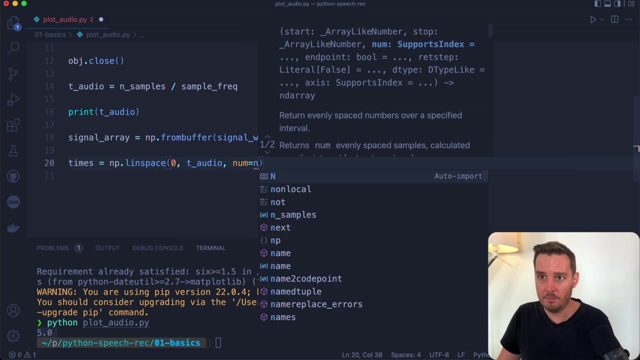 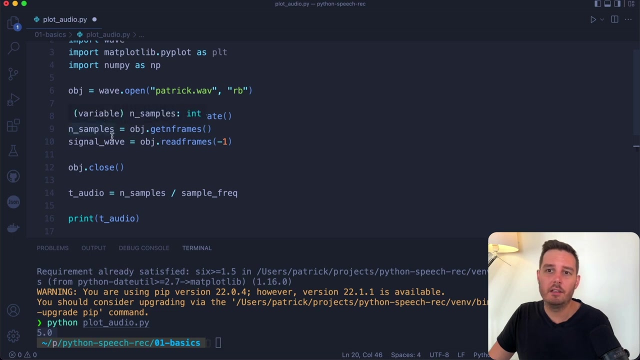 this gets zero as the start and the end is the length of the signal. So this is t audio, or five seconds, And then we can also give this a number parameter, and the number is the number of samples. So, if you remember, so the signal wave. so here we basically get a sample. 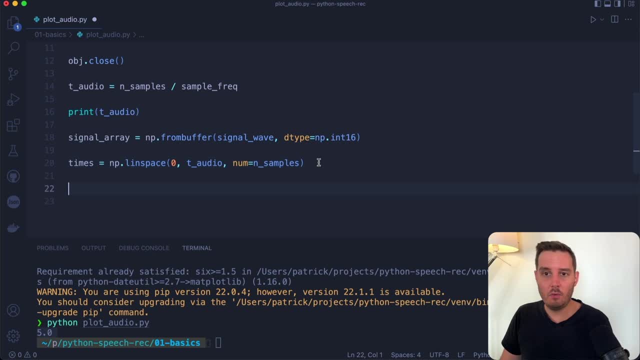 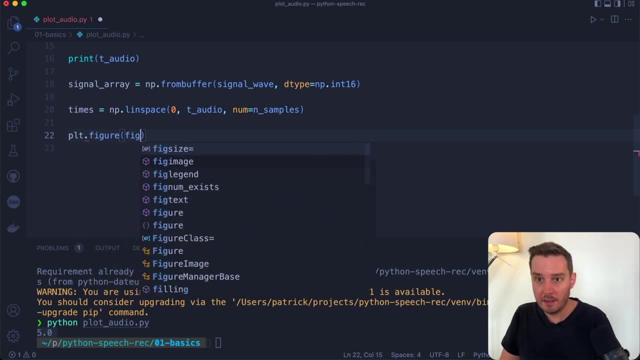 for each point in time. And now we want to plot this. So we create a figure, so we say PLT dot figure and we give this a fixed size of 15 by five. then we say PLT dot plot and we want to plot. 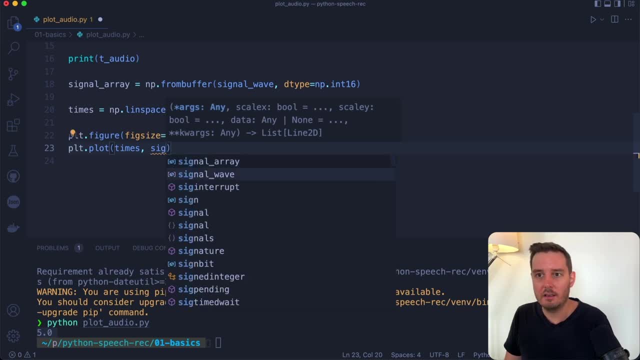 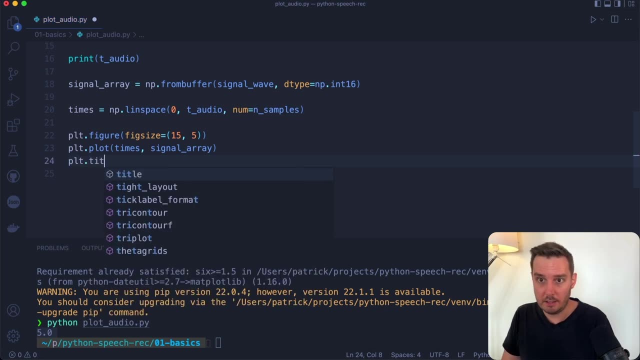 the times against the signal array. then we simply give it a title- PLT dot title, And let's call this audio signal. then I also want to say PLT dot y label, And the y label is the sick null wave And the PLT x label is the time time in seconds. And then we say PLT x limb, And we limit this to. 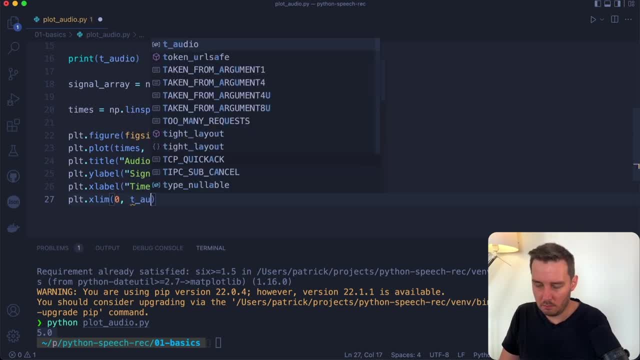 be between zero and T audios for five seconds And then we say PLT, dot, show. And this is all we need and know if we want to do this, we can do this. So let's go ahead and do this. So let's go ahead. 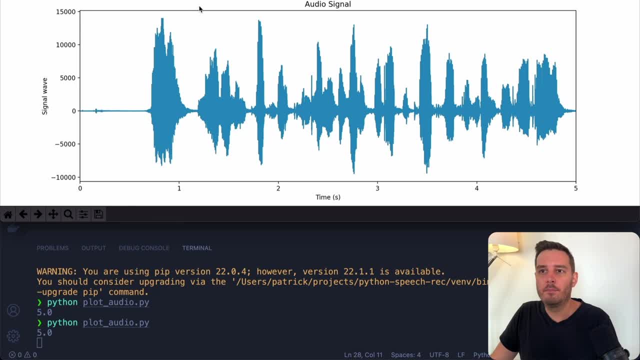 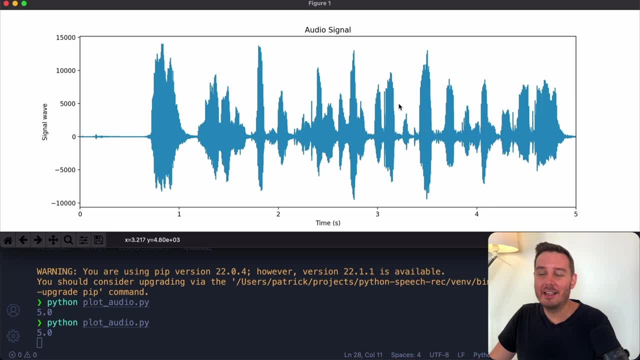 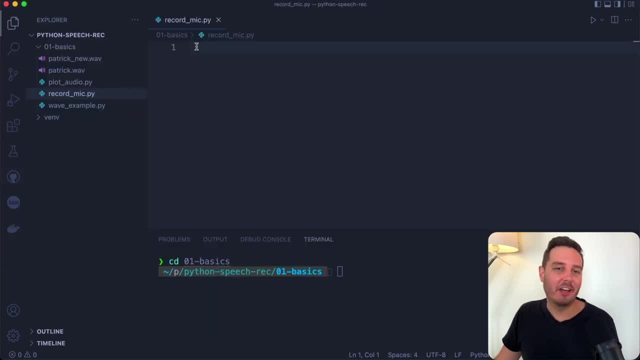 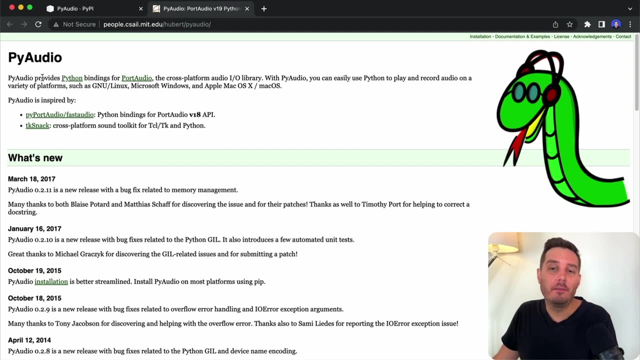 here we have it. So here we have our audio signal plotted as a wave plot, And this is how easily we can do it with Matt Township and the wave model. Now let's learn how we can record with our microphone and capture the microphone input in Python. So for this we use pie audio, a popular 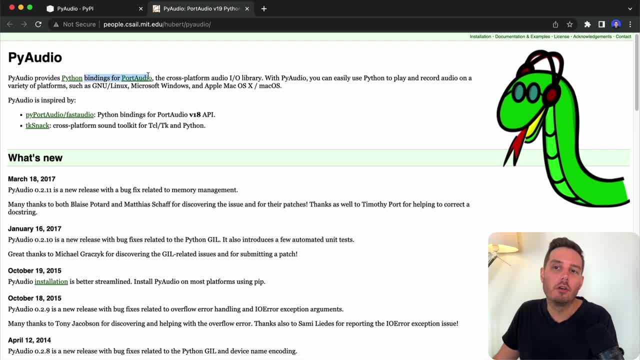 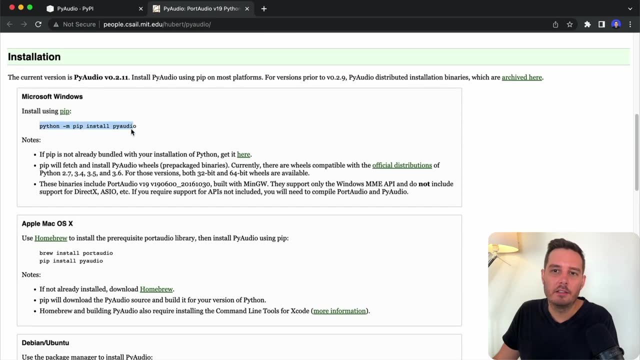 Python library, And this provides bindings for Port audio, the cross platform audio IO library, So with this we can easily play and record audio. And this works on Linux, Windows and Mac, And for each platform there's a slightly different installation command that they recommend. So, for example, on Windows, 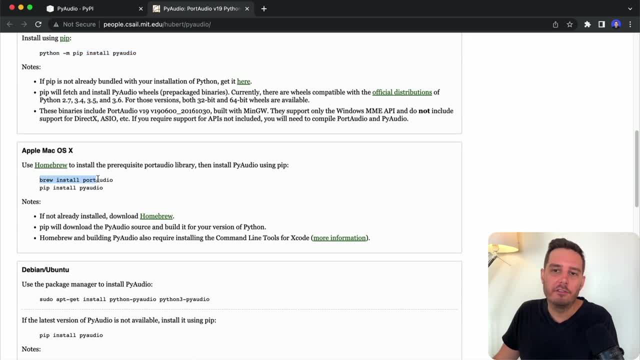 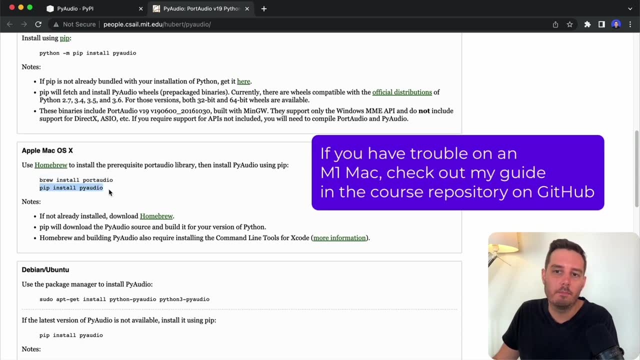 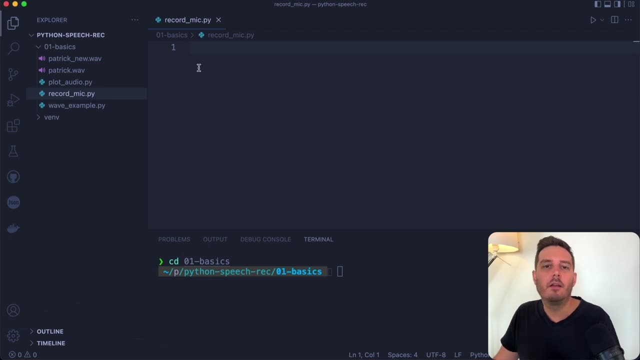 you should use this command On Mac. you also have to install port audio first. So if you use homebrew, then you can easily say brew, install port audio and then pip, install PI audio, And on Linux you can use this command. So I already did this. So here I'm on a Mac, So I 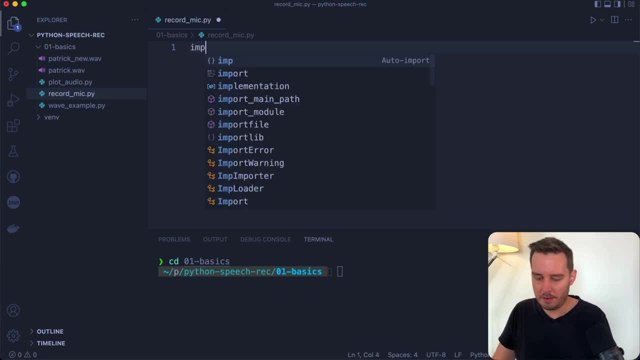 use brew, install port audio and then pip- install PI audio And now I can import this. So I say: import PI audio And I also want to import wave to save the recording later. then I want to set up a few parameters. So I say frames per buffer And here I say 3200.. So you can play around with. 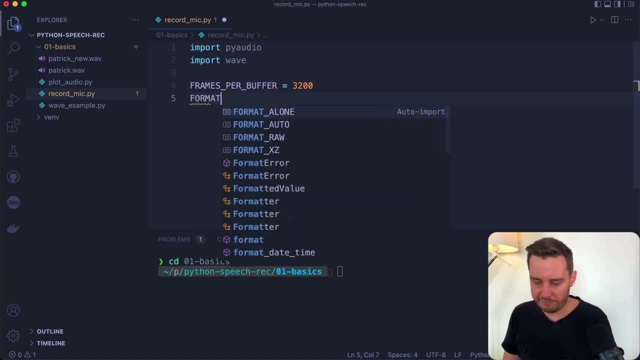 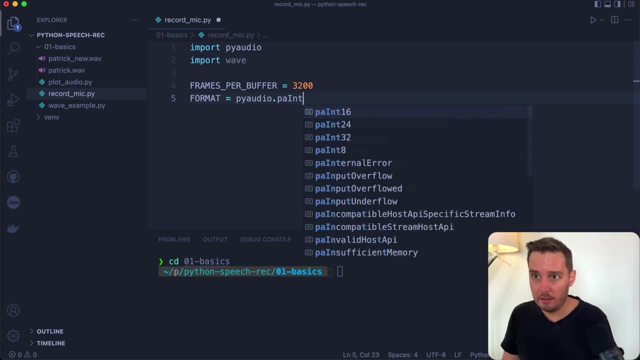 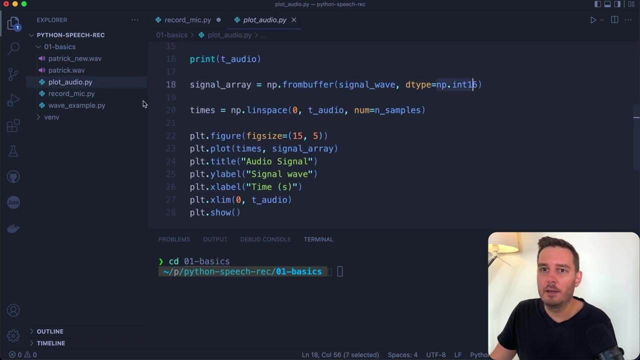 this a little bit. then I specify the format. So the format equals PI audio, P in 16.. So this is basically the same that we used here. So here we use NumPy in 16. And then here we have the PR in 16.. Then I also specify the number of channels. So here I say: 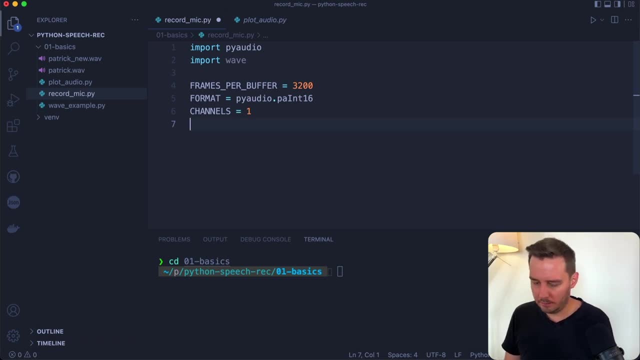 one, so simply a mono format. And then also the frame rate, So the rate: here again I say 16,000.. So again you can use a different rate and play around with this. then we create our PI audio object. So we say P equals PI audio, dot PI audio. then we create a stream object, So we say: 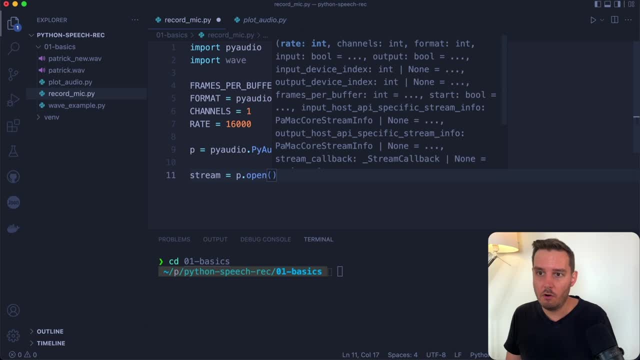 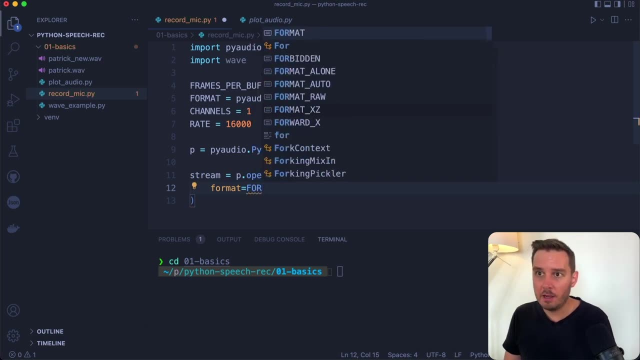 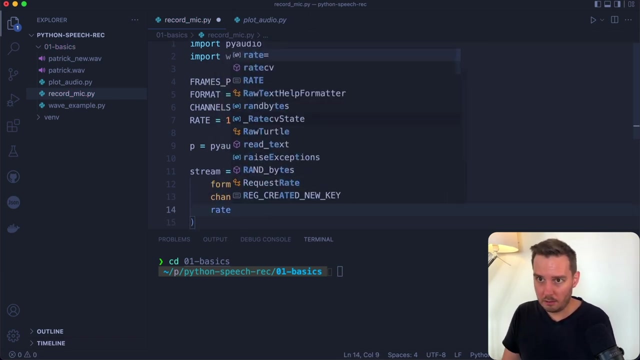 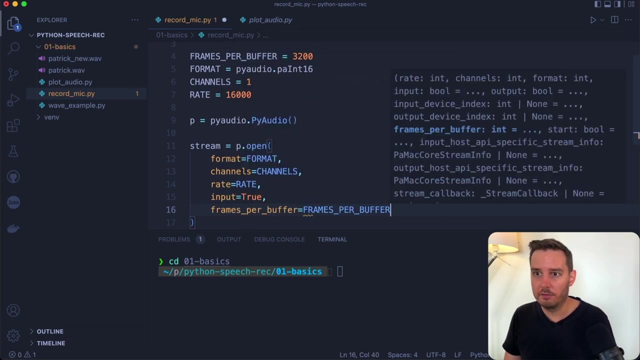 stream equals P dot open. And now we put in all the parameters, So we say format equals format. I need the channels, So channels equals channels. the rate equals the rate. we also want to capture the input, So input equals true. And lastly, we say frames per buffer equals frames per buffer. 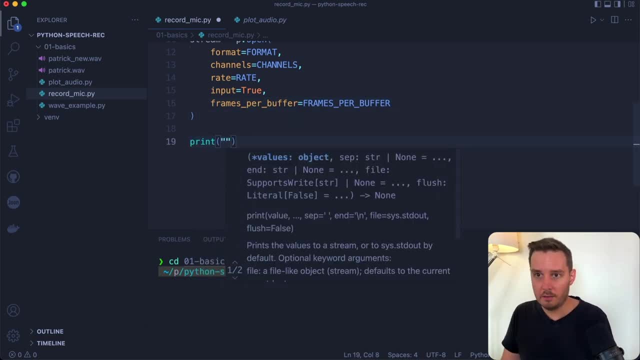 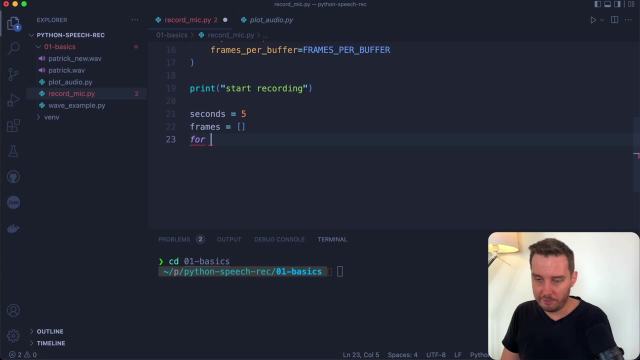 then we have our stream object, So now we can print, start reg cording, And now we want to record for a number of seconds, So here I say five seconds, And then we store the frames and we store this in a list object, And now we can iterate over and say: for I in range. 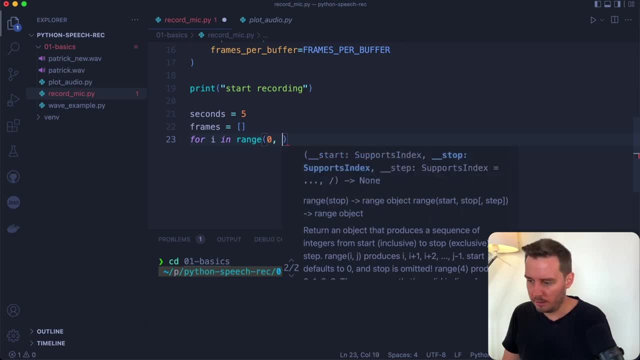 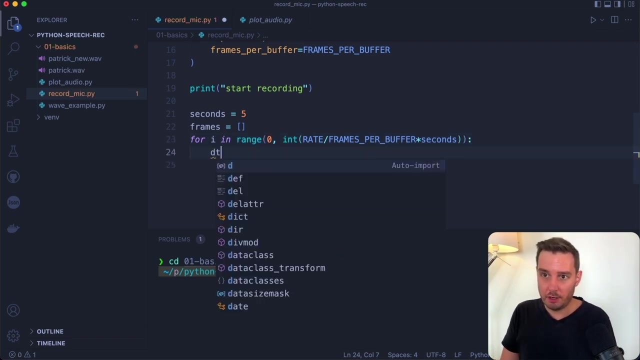 and we start at zero and go until and now. we say: rate divided by frames, per buffer times the seconds, And then we convert this to a integer, not a float, And with this we basically record for five seconds, And then we read each chunk, So we say: data equals. and then here we say: 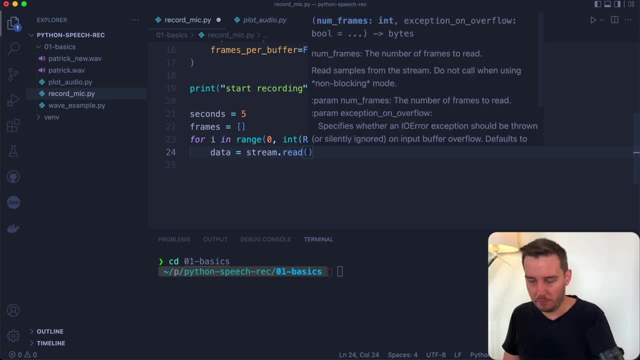 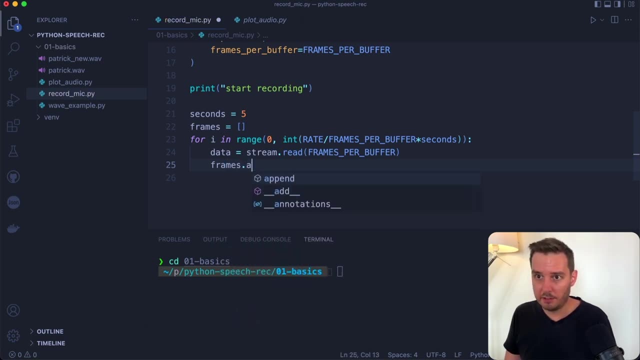 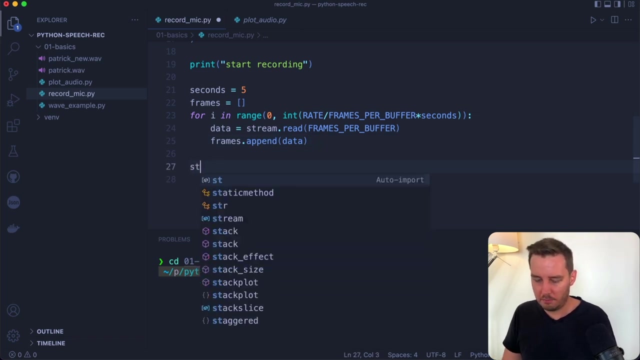 stream, dot read, and then we read the frames per buffer And then we say: frames, dots append the data. So basically frames per buffer. So this means we read this many frames in at once, so with one iteration, and now we have it. So now we can close everything again, So we can say: 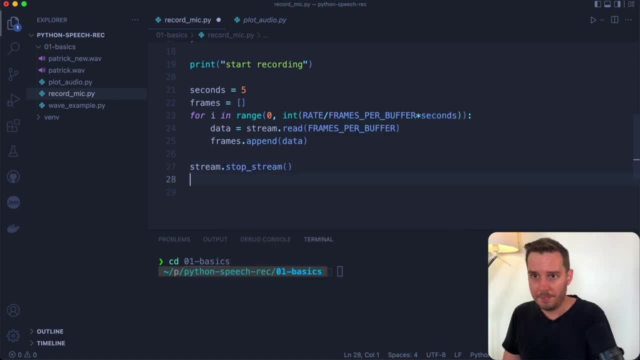 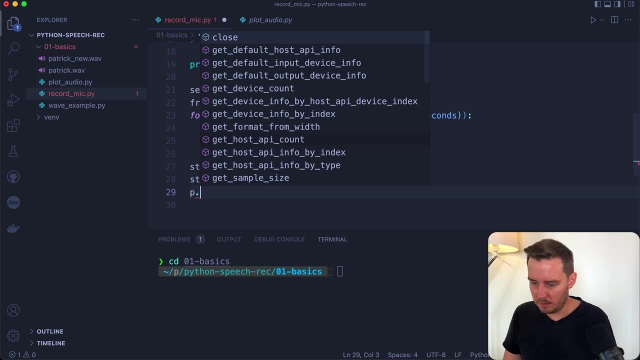 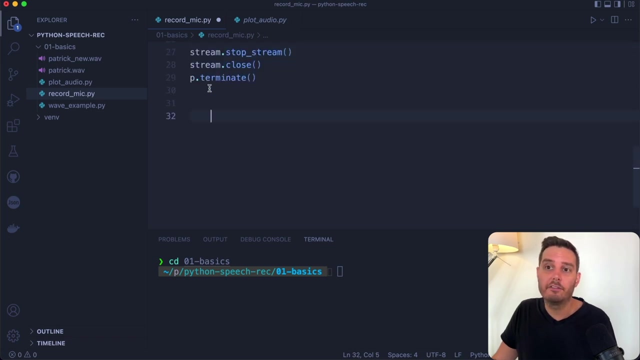 stream dot stop, stream. then we can also say stream dot close, And we can say p dot terminate. So now we have everything correctly Shut down And now we can, for example, save the frames object again in a WAV file. So for this: 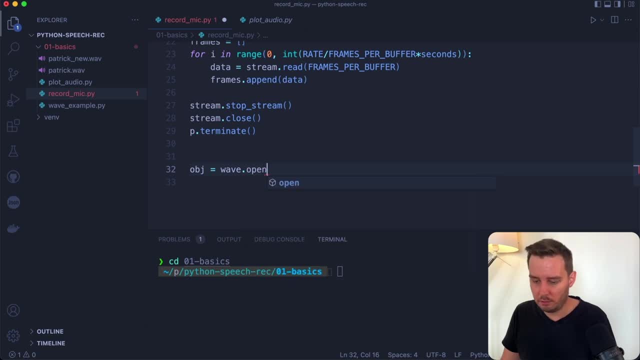 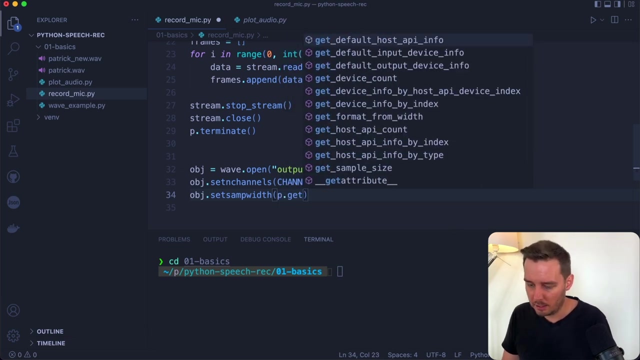 I say object equals wave, dot open And let's call this output dot wave And in right binary mode. then we set all the parameters. So I set object, set number of channels. this is the channels parameter of object. dot set sample with this is the. this we get from p dot get sample size of our format. 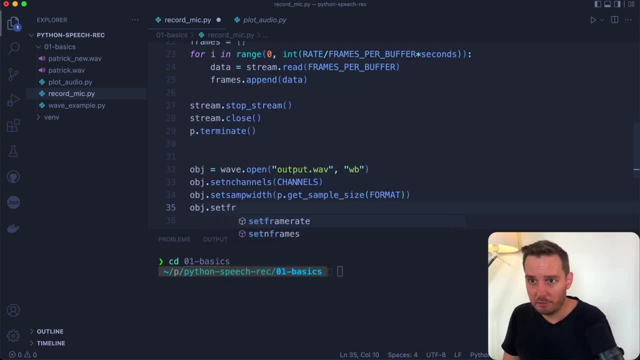 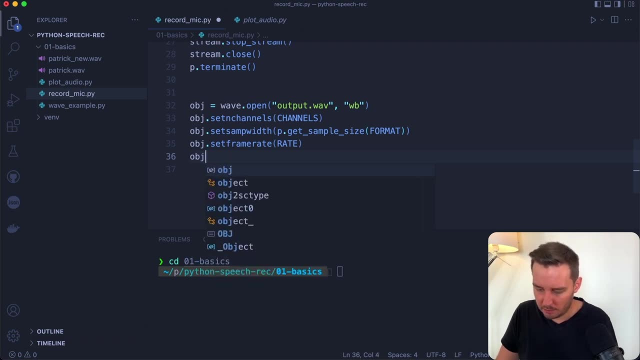 then object dot set frame rate. this is the rate And then we can write all the frames. So we say object dot write frames And we need object dot write, and then we can write everything to object dot write frames And we need object dot write frames And we need object dot write frames. And the other logic and the last thing of this pressure we don't have. we need to do for so much window column and there's a contact film thing. And I have something else right here: If we set the click and sometimes from the drive phase we'll put up a table inside of the code. 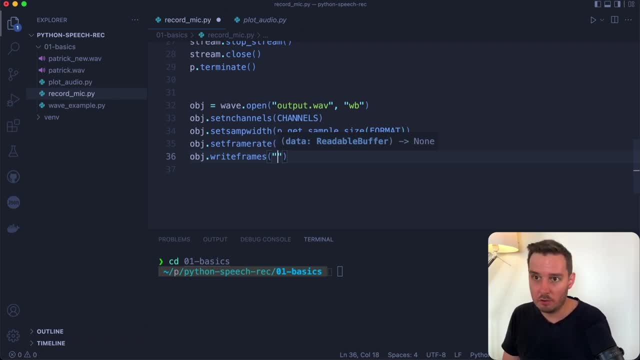 it goes into each of the other object fields And then we can actually report the project fields And And we need to write this in binary, So we can create a binary string like this, So a string and then dot, join, And here we put in our frames list. So this will combine all the elements in our 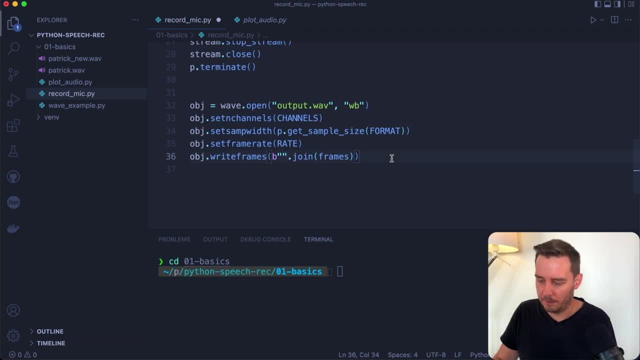 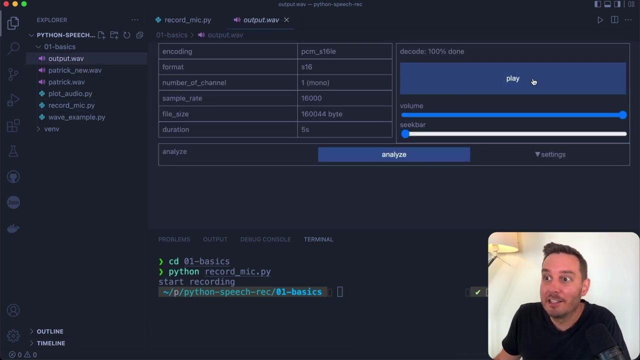 frames list into a binary string And then we say object, dot, close, And this is everything we need to do. So now we can run Python record Mike and test this. Hi, I'm Patrick, this is a test 123.. And now it's done. So here we have our new file, So let's play this and see if this works. 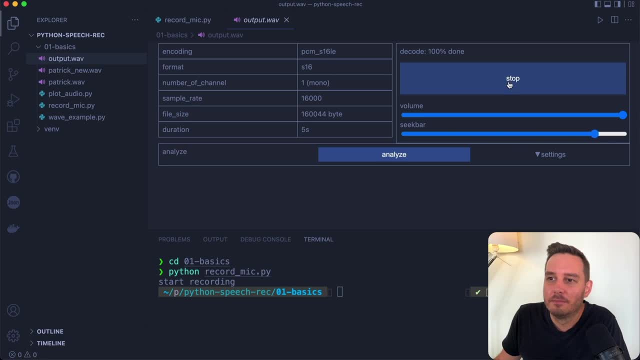 Hi, I'm Patrick. this is a test 123. And it worked Awesome. And now, as last step, I also want to show you how to load mp3 files, and not only webpages, but also other files. So let's take a look at how to load mp3 files, and not only webpages. 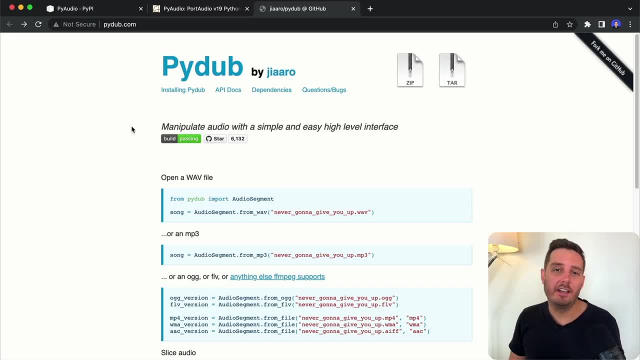 but also other files. So let's take a look at how to load mp3 files, and not only webpages, but also other wave files. So let's do this. So to load mp3 files, we need an additional third party library. 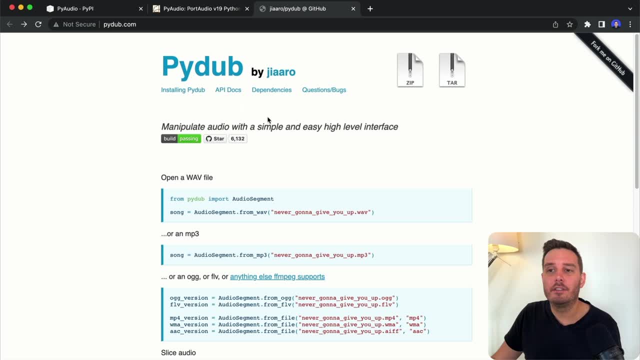 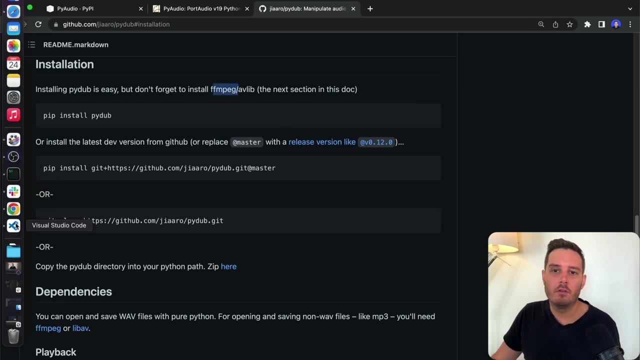 And I recommend to use pydub. So this is a very simple to use library. it provides some simple and easy high level interface to load and also to manipulate audio. So in order to install this, we also need to install ffmpeg. So on the Mac I use homebrew So I had to say brew, install ffmpeg And 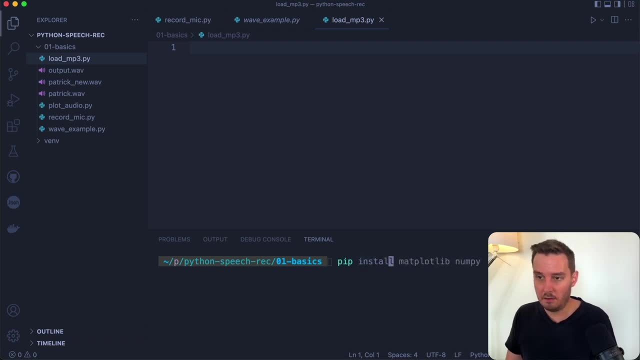 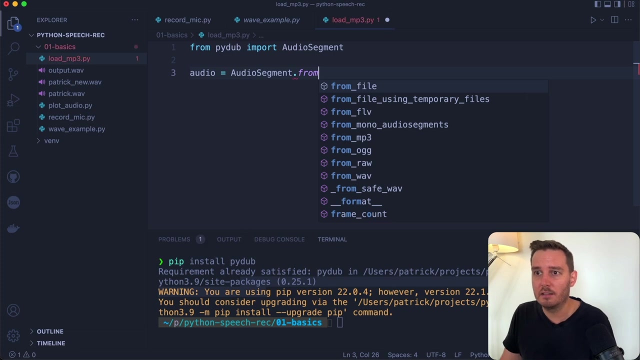 after this you can simply say: pip install, and then pydub, And now this should install it. So here it's already satisfied. And now we can for example say: from pydub we want to import the audio segment. And then we can say: audio equals audio segment. And then here we can say: 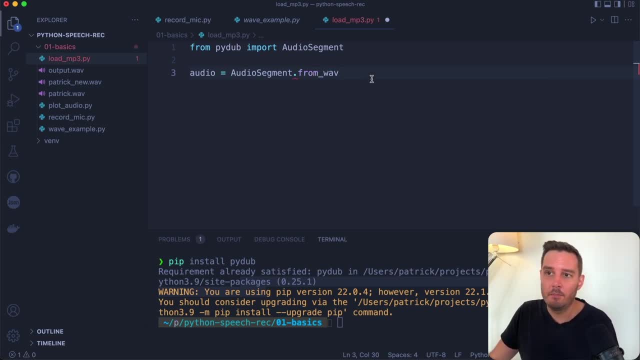 from mp3,. if we have an mp3, in my case right now I only have a from wave- And then here I let's load the Patrick dot wave, And then we can, for example, also very easily manipulate this by saying audio plus six, audio plus six. so this will. 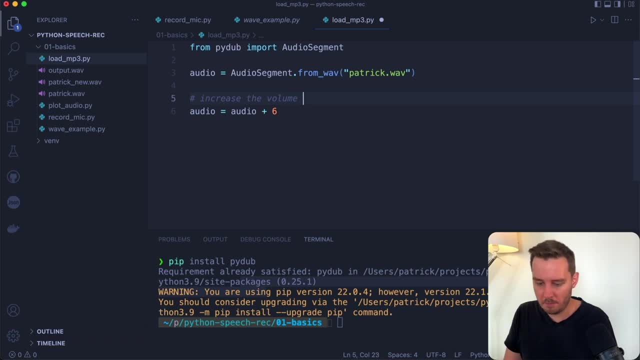 increase the volume by six. the b Roth 60. 3D. 더加把精蓄的, which will increase the volume by sixdb, 6db, 3D. we can also, for example, repeat the clip. So we say audio equals audio times two. then we can use: 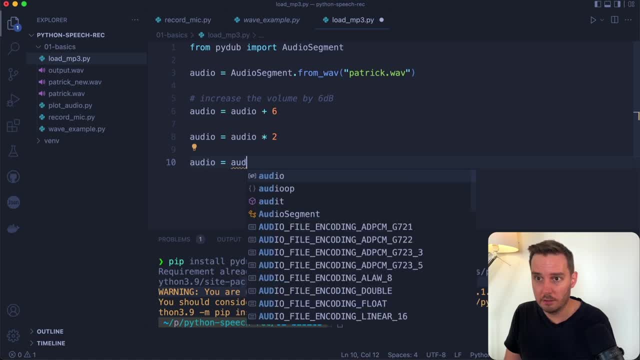 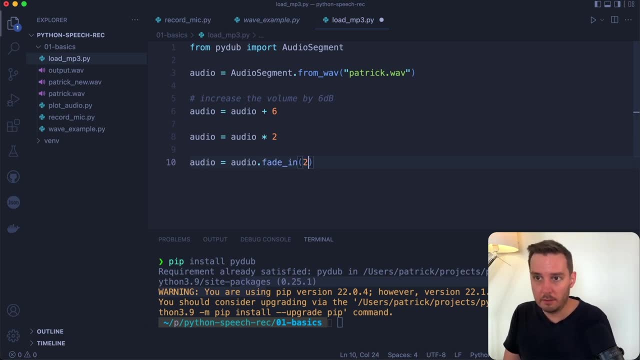 a fade in, for example, audio equals audio dot. fade underscore in with with 2000 milliseconds, so two seconds fade in the same works with fade out. So yeah, this is how we can manipulate and then we can say audio dot export. And then I want to export this in. let's call this mesh up dot mp3. 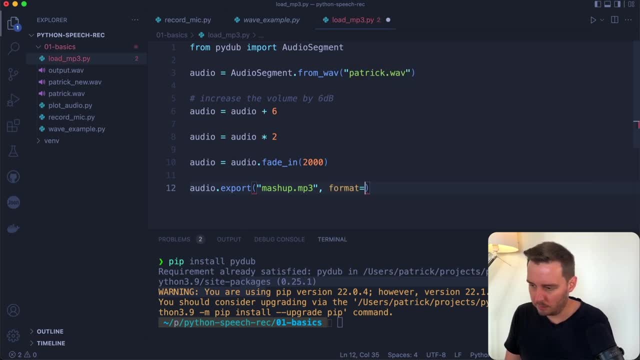 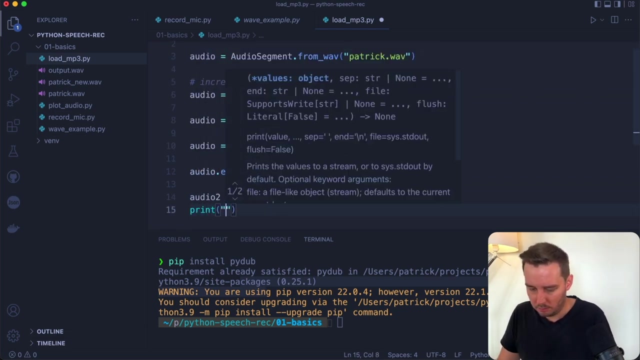 And then I have to say format equals as a string mp3. And now, for example, I could load this by saying audio to equals audio dot from mp3.. and then here I use mesh up dot, mp3, and then print done so that we see it arrives at this. 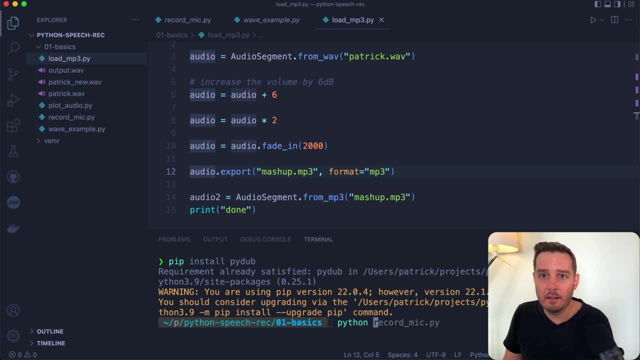 part. And now let's say Python, and then the load mp3 file And, yeah, this works. So now, here we have our mp3 file And we could also load it like this. So, yeah, that's how you can use the. 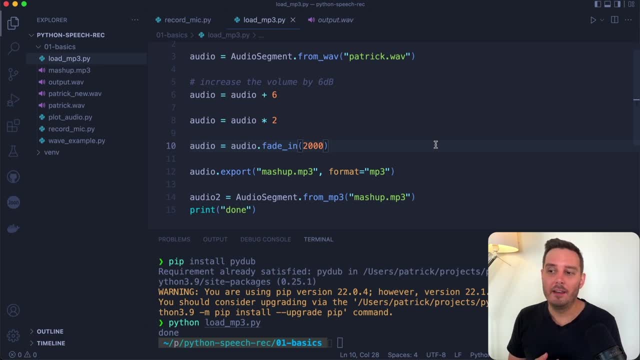 pydub module to load other file formats as well, And that's all I wanted to show you in this first part. I hope you learned a little bit about audio processing and Python and enjoyed this. And now let's move on and let's learn how to do speech recognition in Python. 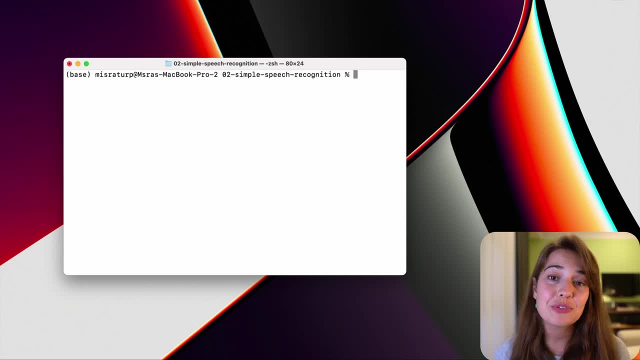 Hey and welcome. In this project we are going to learn how to do speech recognition in Python. It's going to be very simple. What we're going to do is to take the audio file that we recorded in the previous project and turn it into a text file. Let me show you how. 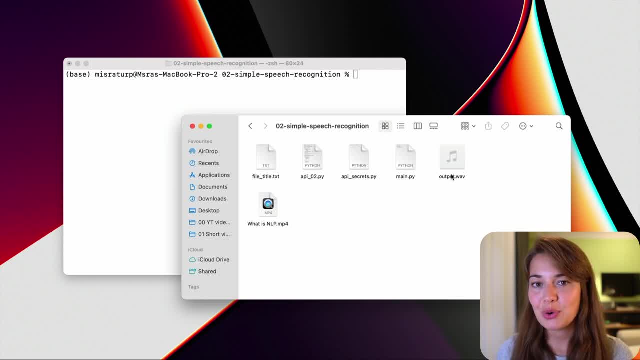 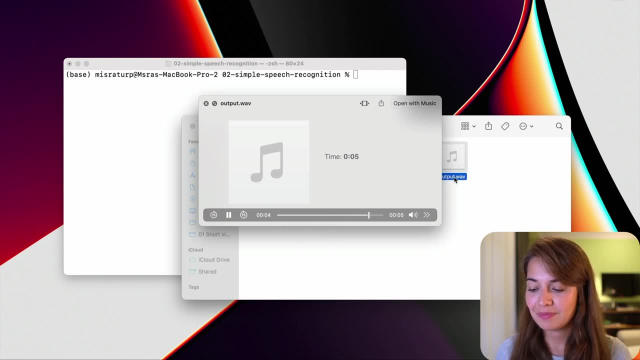 to do that. So first of all, we're going to take the audio file that we recorded in the previous project works. So here is the audio file that we recorded in the previous project. Hi, I'm Patrick. This is a test 123.. And if we run our script, 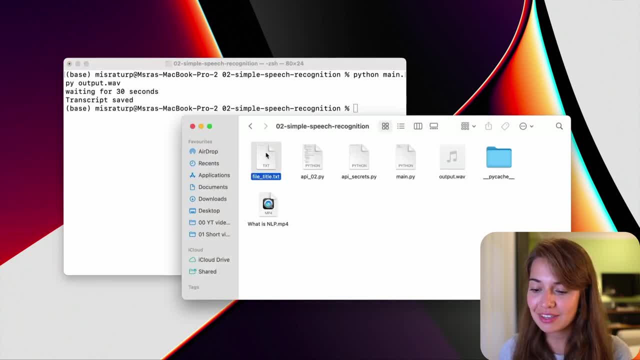 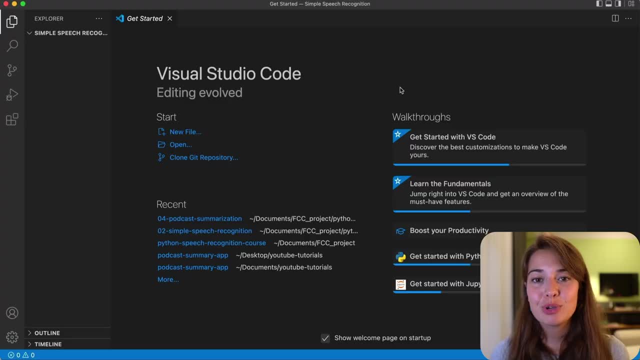 we get the text transcription of this audio file, So like this here: Hi, I'm Patrick. This is a test 123. So let's learn how to implement this in Python. So for this project, we are mainly going to need two things. 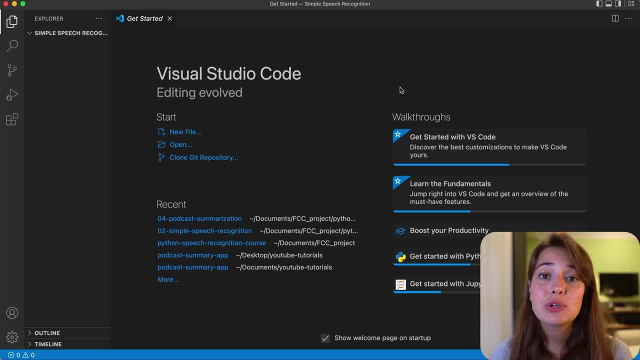 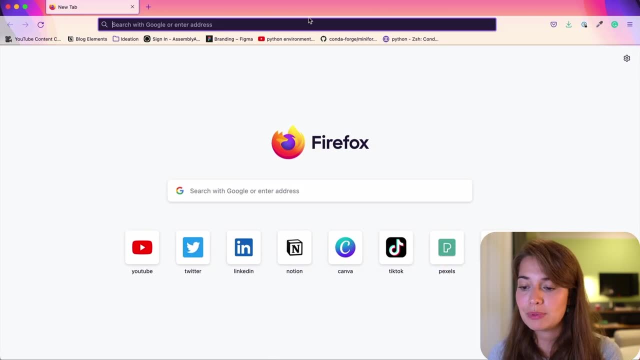 Assembly AI's API to do the speech recognition and the request library from Python to talk to Assembly AI's API. So let's first go ahead and get a API token from Assembly AI. It's very simple. You just need to go to assemblyaicom and create a free account. Once you have an account, 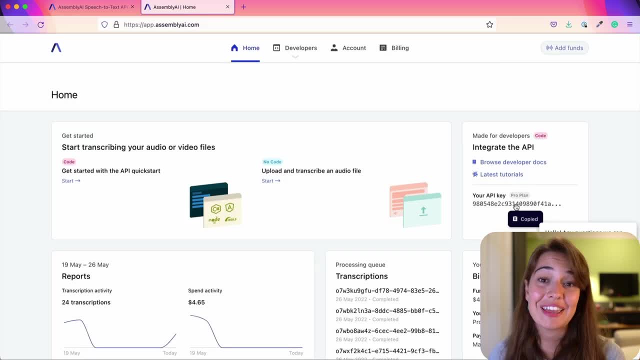 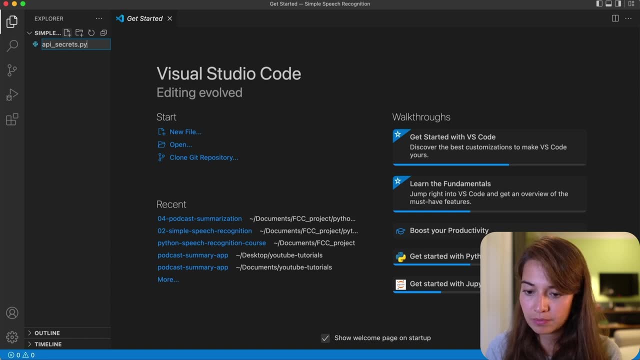 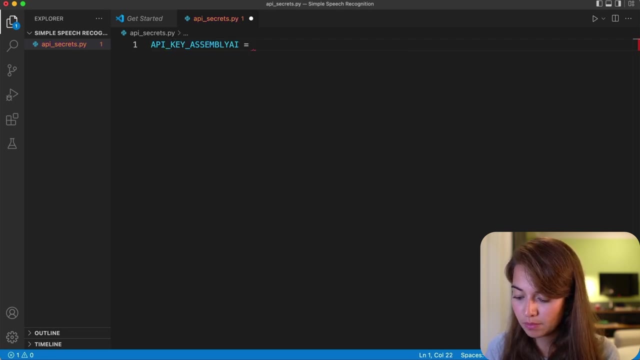 you can sign in and just copy your API key just by clicking here And right away. I'm going to create a configure file and put my API key Once I've done that. now I have a way of authenticating who I am with assembly AI's API. 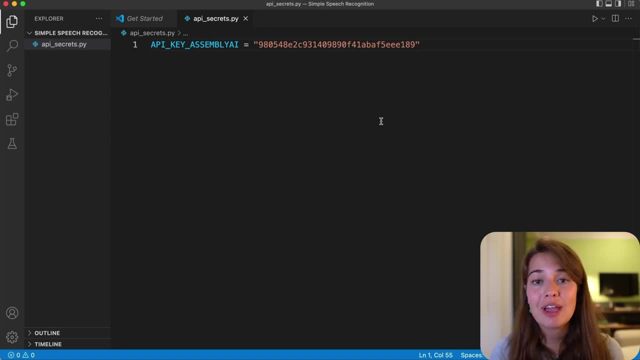 And now we can start setting up how to upload transcribe and get the transcription from assembly as API. The next thing that I want to do is to have a main file that is going to have all my code. What I need to do in there is to import the requests library so that I can talk to the 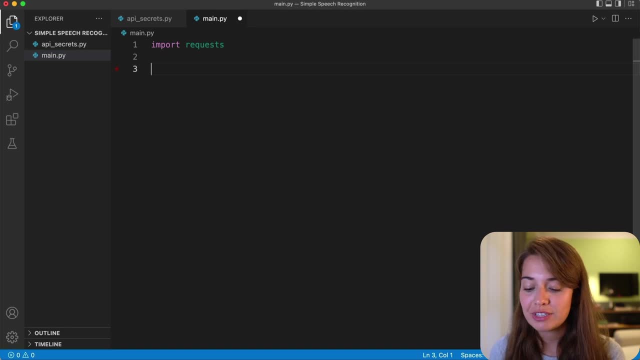 assembly API. So this project is going to be a little bit more complicated. So I'm going to have four steps. The first one is to upload the file that we have locally to assembly AI. Second one is to start the transcription. Third one is keep pulling assembly as API to see when the 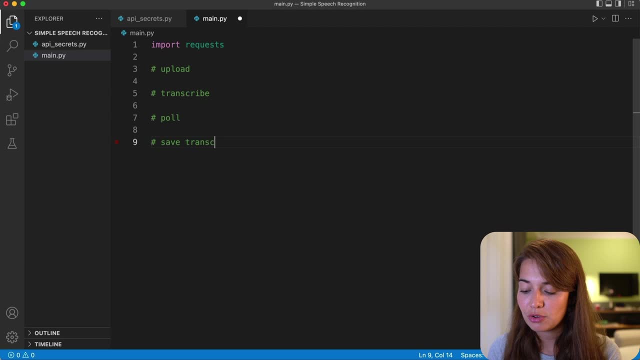 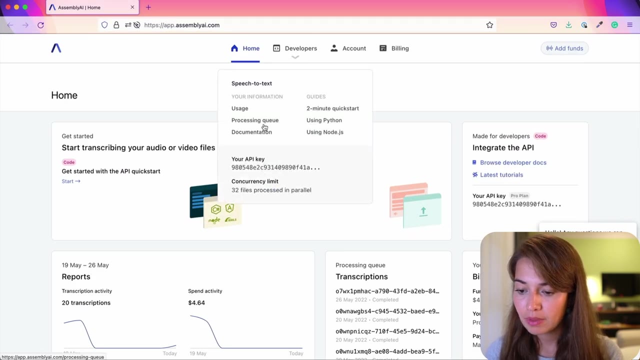 transcription is done And, lastly, we're going to save this transcript. So uploading is actually quite simple. If we go to the documentation of assembly AI, We will see here uploading local fire files for transcription. So I can just copy and paste this. 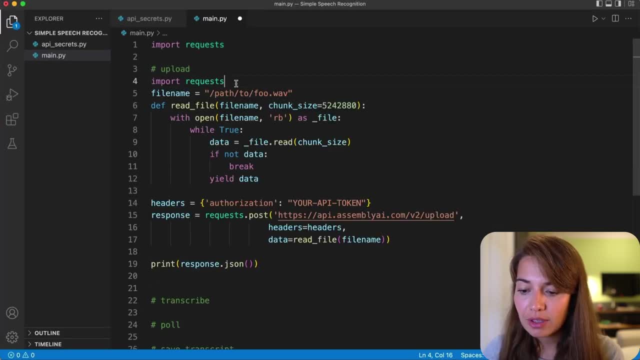 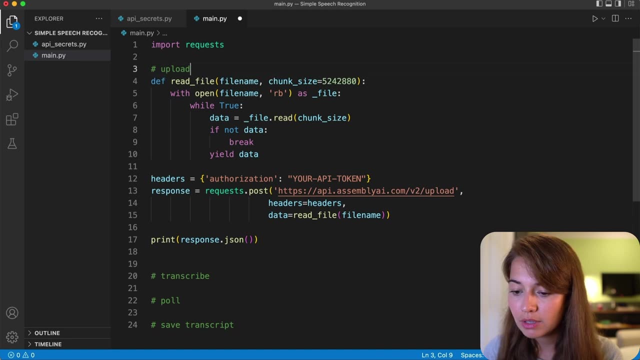 And change the code as we need it. So basically, yeah, okay, we are importing the request library already the file name we're going to get from the terminal, So I will set that later. Just a couple of things that we need to pay attention here. Basically, there is a way to read: 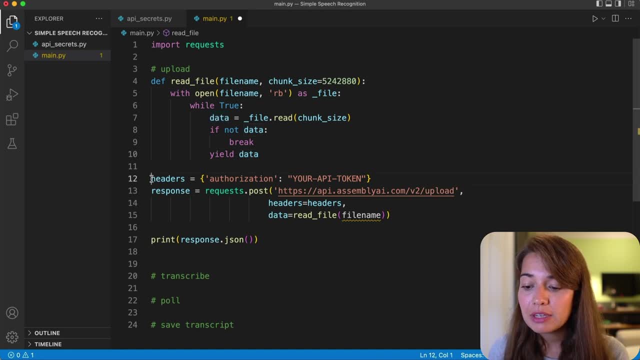 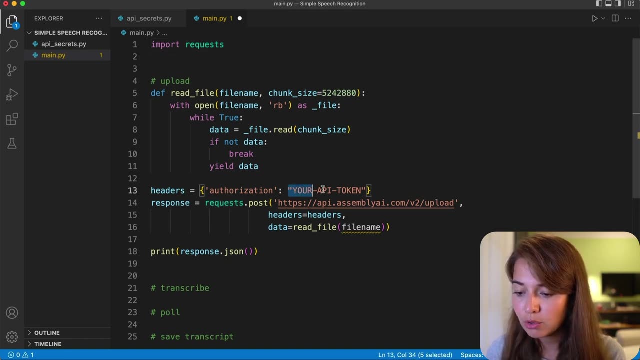 the audio file from our file system, And then we need to set up headers. The headers are used for authentication, So we can actually already set this, because this is not going to be your API token. we have set it to be API key, assembly, AI right And we need to import it here. of course, 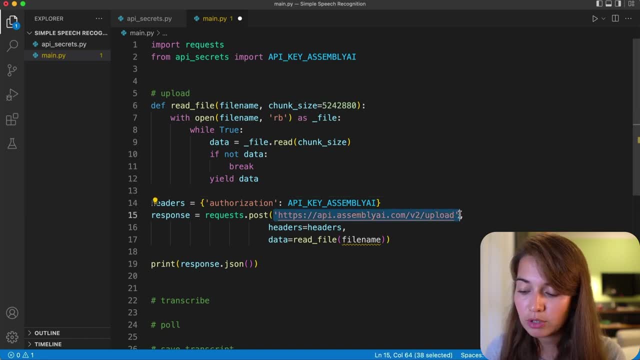 Alright, that's done. So we also have a upload endpoint for assembly, And this one is API. that assembly, ai, comm v2 upload. But you know, this might be something that we need also later, So I'm just going to put this to a separate value variable. 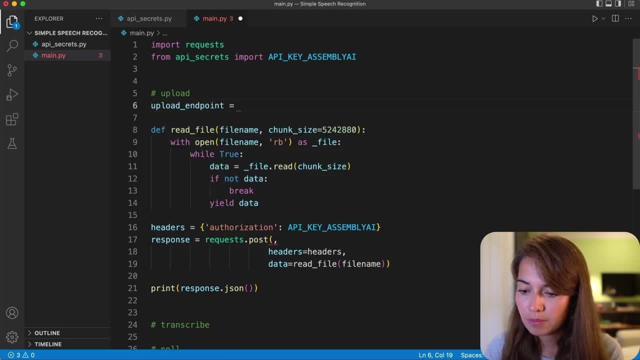 and then just call this one here. so when we're doing, uh, when you're, when we are uploading a file to assembly ai, we are doing a post request in this post request. you need to. you need to send this post request to the upload endpoint. you need to include your api key included in the headers. 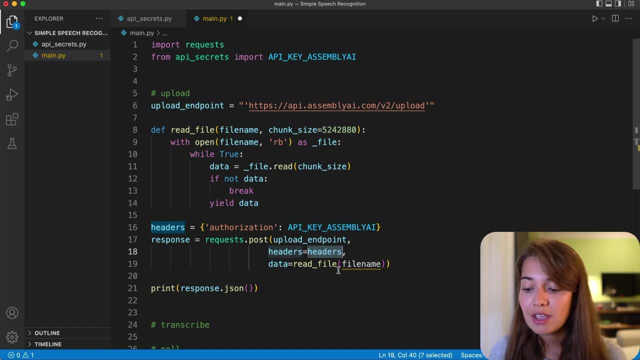 and, of course, you need the data. so the file that you read- and we are reading the data through the read file function- in chunks, because assembly ai requires it to be in chunks and in chunk sizes of five megabytes, basically this is a number of bytes that are in there. while we're at it, we can already. 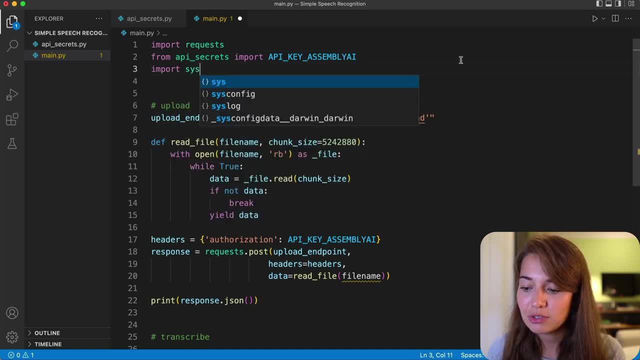 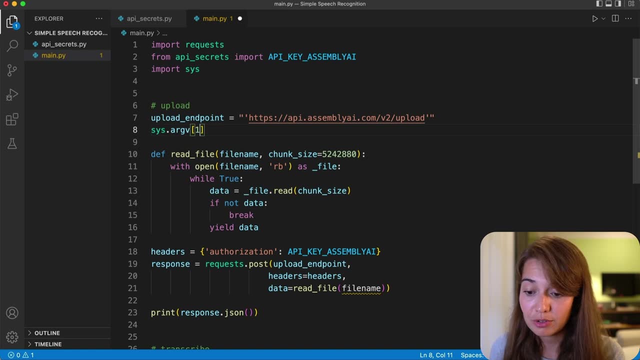 get the file name from the terminal too right, so for that i just need to import system and inside system. the second or the first, not the zeroth variable, or the argument is going to be the file name, and here let's click on it up a little bit. All right, now we should be able to just run a command on the terminal. 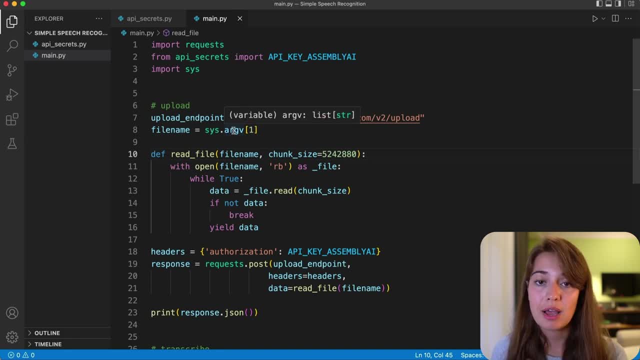 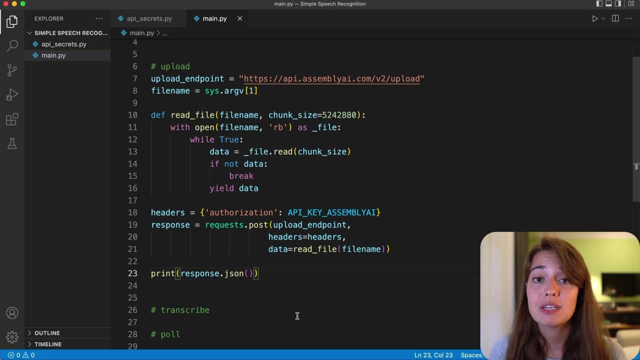 include the name of the file that we want to upload and it will be uploaded to Assembly AI And we will also. let's print the response that we get from Assembly AI to see what kind of response we get. Again, this is the file that we are working with. 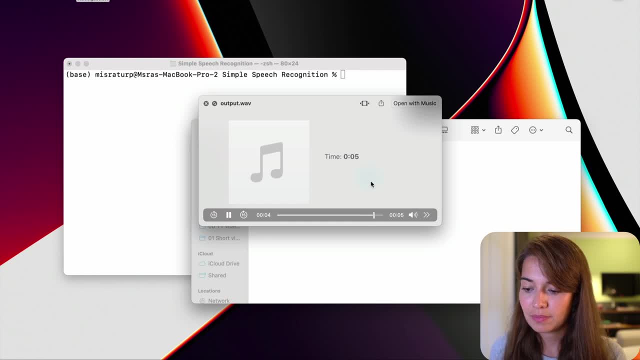 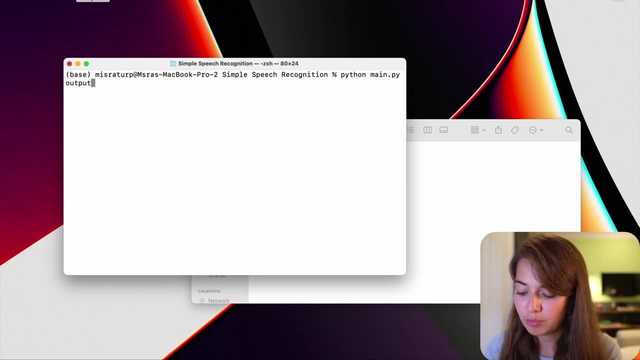 Hi, I'm Patrick. this is a test 123. And what we need to do right now is to run Python main dot pi and the name of the file, in this case output dot love. Alright, so we uploaded our file to assembly AI successfully And the response what we get is the: 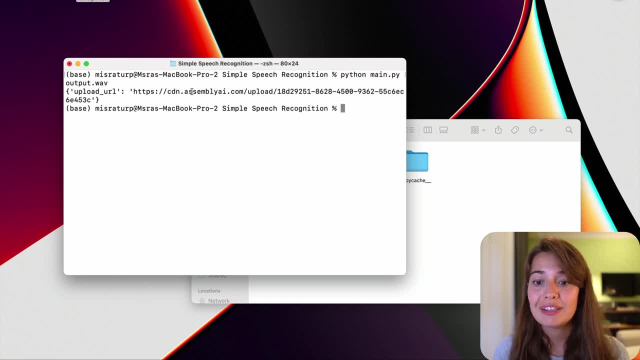 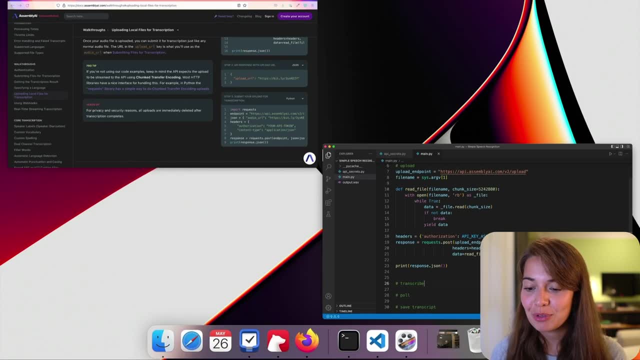 upload URL, So where your data, where your audio file lives right now, And using this we can start the transcription. So for the transcription, let's again cheat by getting the code from the docs. Here is the data, the code that we need starting. 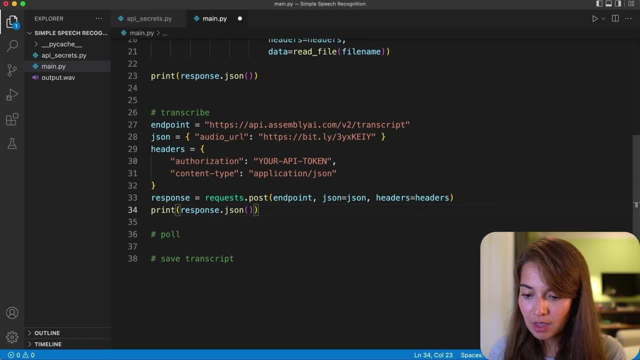 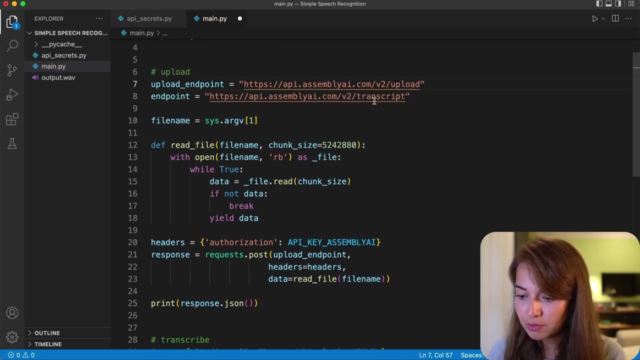 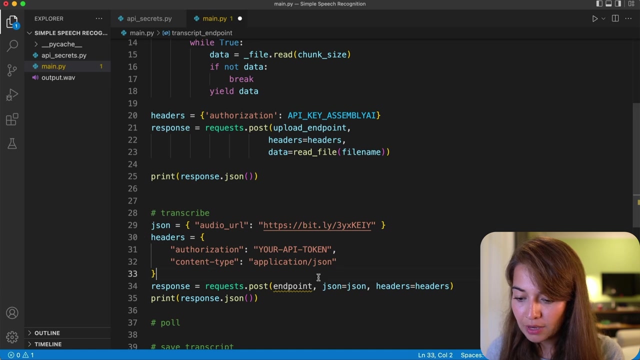 from here. So this is a transcription endpoint. you can see that it ends differently than the upload endpoint. This one ends with upload. this one ends with transcript. I will call this the transcript endpoint. Heathers, we already have a header. we don't really need this anymore. 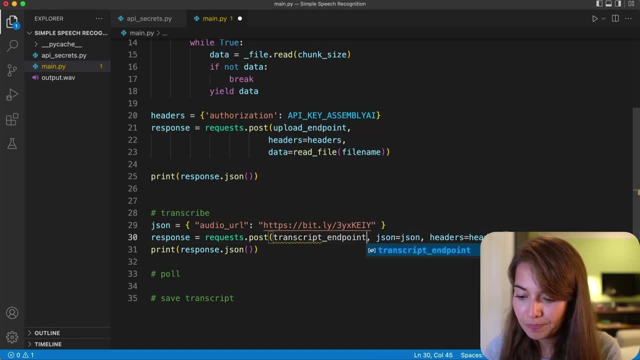 The endpoint is transcript. endpoint JSON is the data that we are sending to or the data that we want assembly AI to transcribe, So we are going to need to give it the audio URL. we already have the auto URL right, So we got the response, but we did not extract it from the 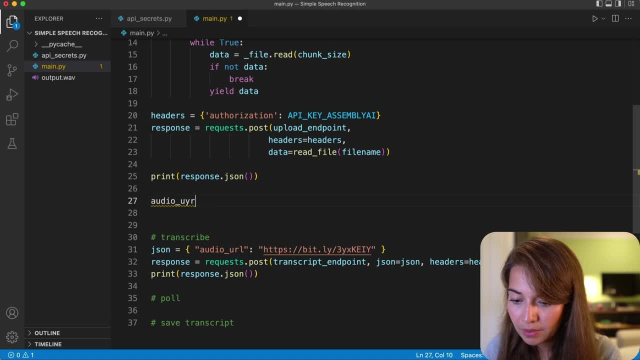 response. So let's do that. audio URL is response to Jason And it was called upload URL. So we're going to give us audio URL to here, because it was just an example. Okay, and this way we will have started a transcription, And let's do this and see what the result is. 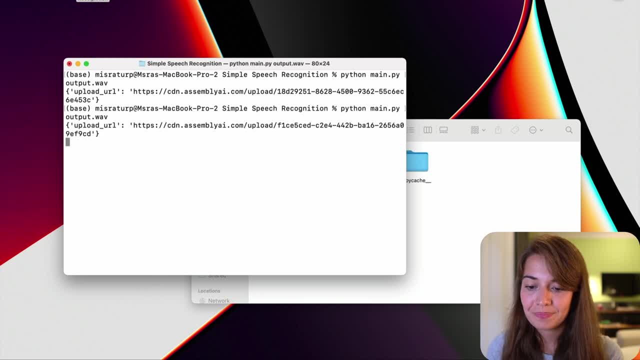 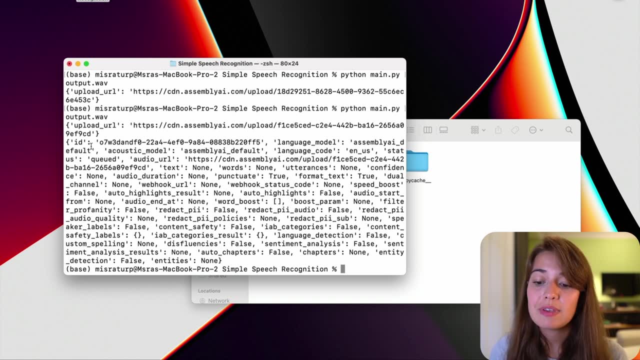 I will run this again same thing. All right, so we got a much longer response In this response. what we have? we have a bunch of information about the transcription that we've just started, So you do not get the transcript itself immediately Because, depending on the length of your audio, it might take a minute or 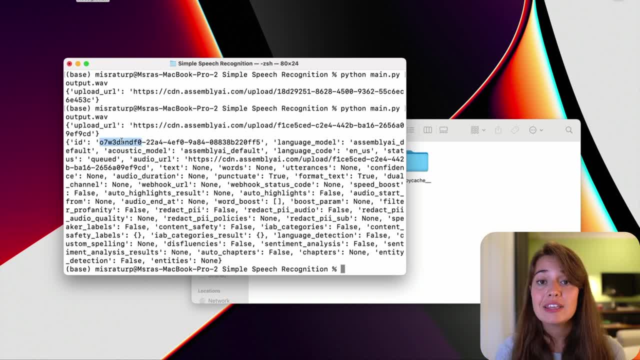 two right. So what we get instead is the ID of this transcription job. So by using this ID, from now on we can ask assembly AI. hey, here is the ID of my job, this transcription job that I submitted to you. 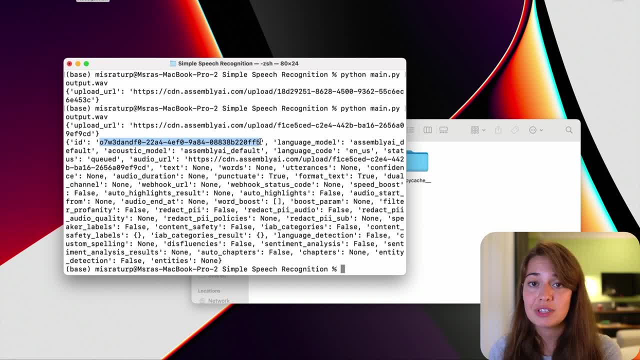 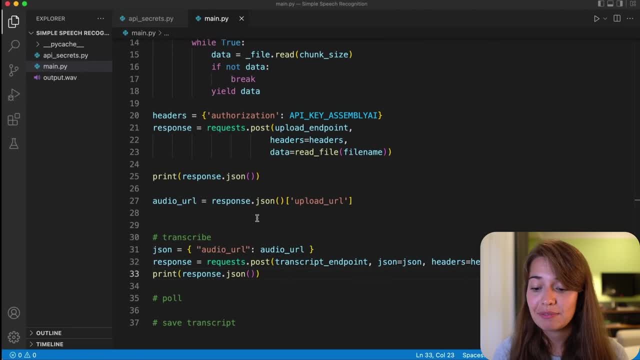 is it ready or not? And if it's not ready, it will tell you it's not ready yet, it's still processing. If it's ready, it will tell you: hey, it's completed And here is your transcript. So that's why the next thing that we want to build is the polling. we're going to keep. we're. 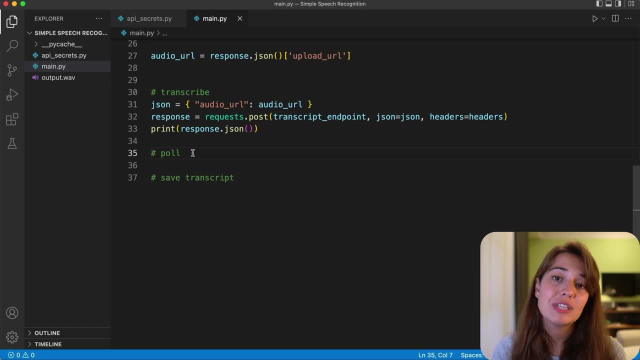 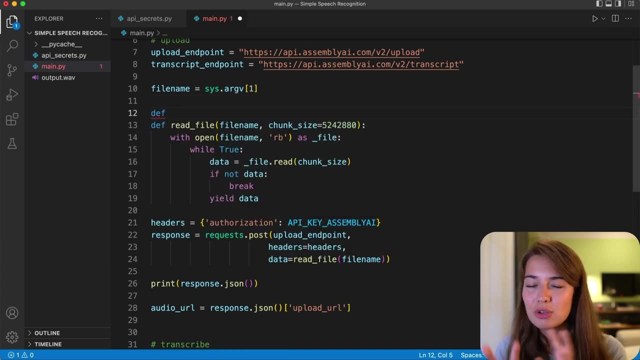 going to write the code that will keep polling assembly AI to tell us if the transcription is ready or not. But before we go further, let me first clean up this code a little bit, so that everything is nicely packed and functions. we can use them pre, use them again if we need to. So 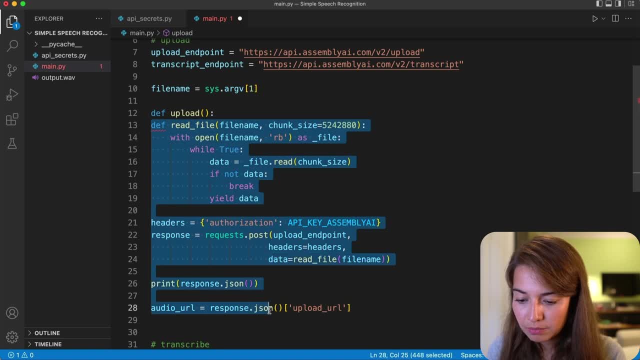 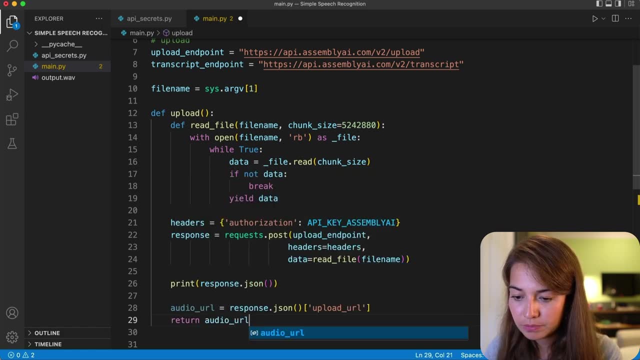 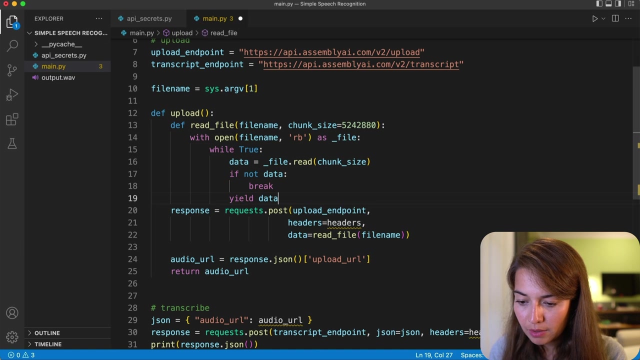 this one is the upload function. Yes, and what it needs to return is the audio URL. We do not need to print the response anymore. we've already seen what it looks like And we need to put the header separately because we want both upload and transcribe and basically everything else to be. 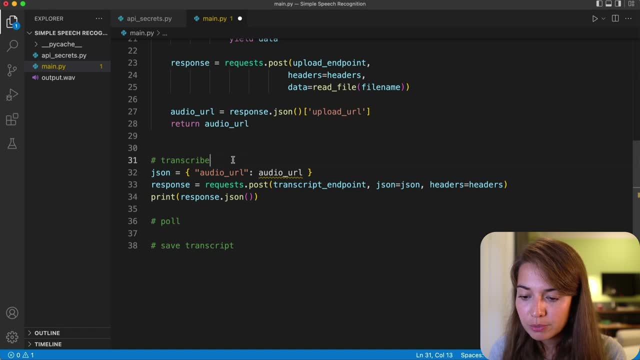 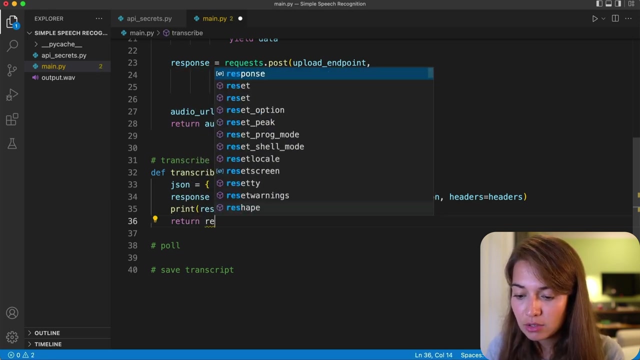 able to reach this variable code. headers For transcription again, I will create a function called transcribe, And what I need to return from the transcription function is the ID. So I will just say job ID And that would be response, dot, JSON And ID. Again, we don't need this anymore. I'll just call it job ID And then. 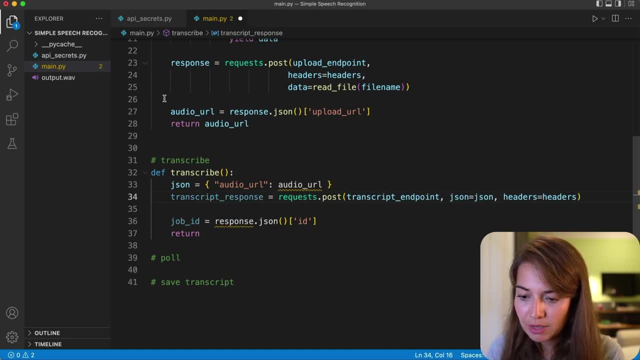 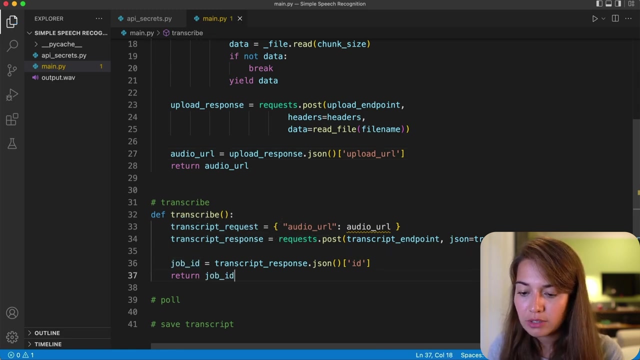 call this transcript response to make it clear this will be upload response. Let's call this transcript request. So everything is nice and clean. This is this and this goes here, And for upload response, we use it here And we need to return job ID. Alright, so now we have them, nicely. 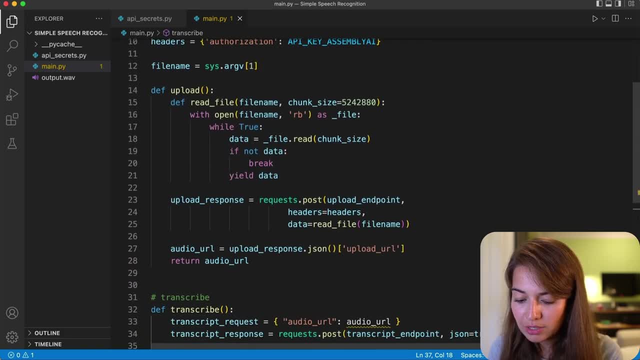 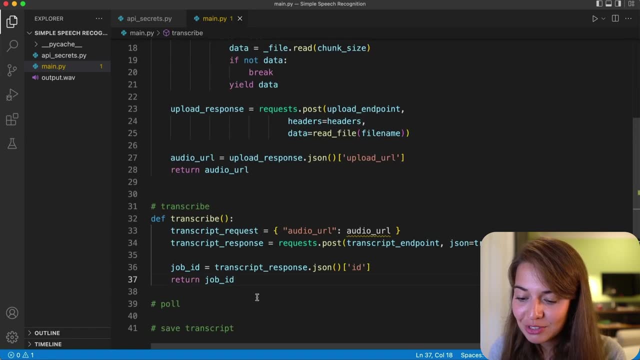 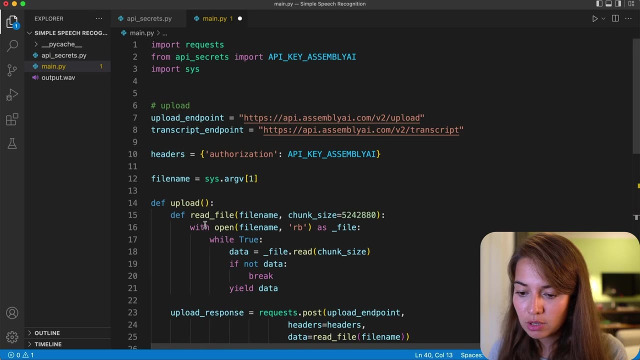 wrapped up in different functions and everything else looks good. Let's run this again to see that it works. Now, of course I'm not calling the function, So let me call the functions and then run it: Upload and transcribe. But of course I also need to pass the file name to the upload function. So 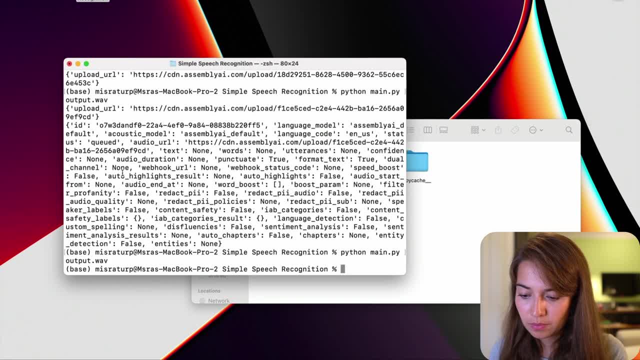 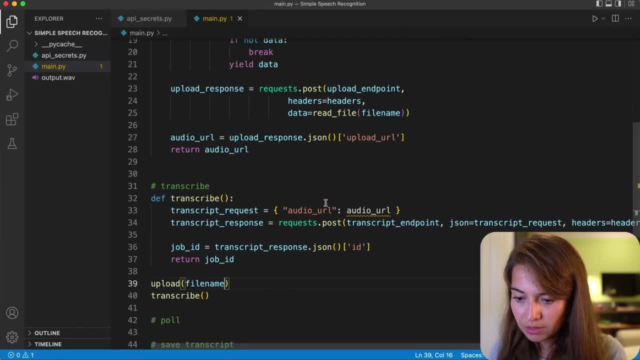 let's do that too. audio URL is not defined, Then I also need to pass audio URL. audio URL to transcribe- Good thing we tried. So this will be returned from the upload function and then we will pass it to the transcribe function And as a 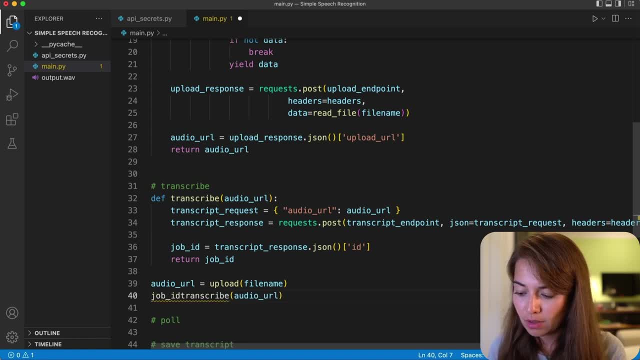 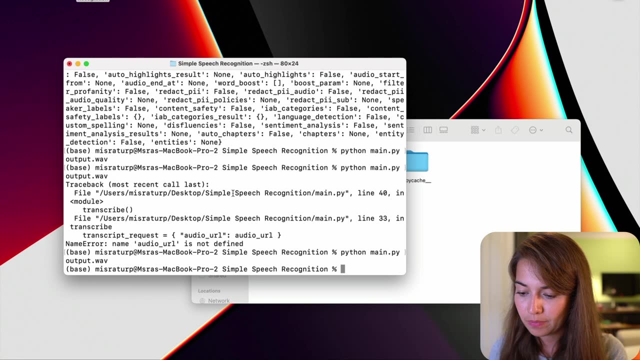 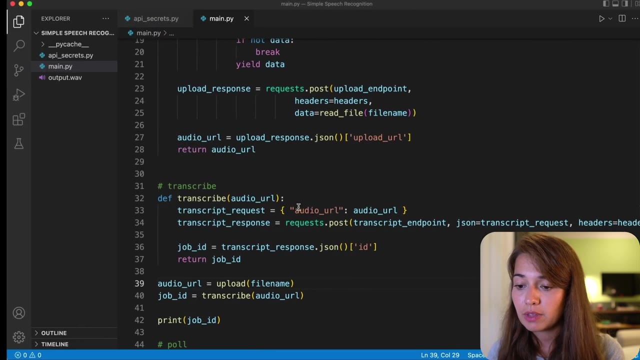 result: we will get job ID, And then I can print job ID to see that it worked. Let's see, Yes, I do get a job ID, So, okay, things are working. The next thing that we want to do is to set up the full 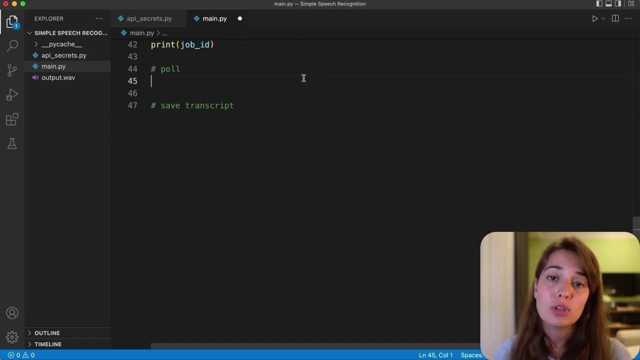 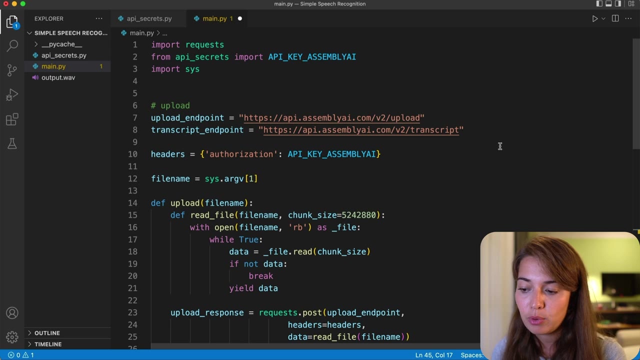 polling function. So the first thing we need to do for that is to create a polling endpoint. polling endpoint. So, as you know, we had the transcript endpoint and the upload endpoint here. That's how we communicate with assembly as API, with polling endpoint it's going to be specific to the 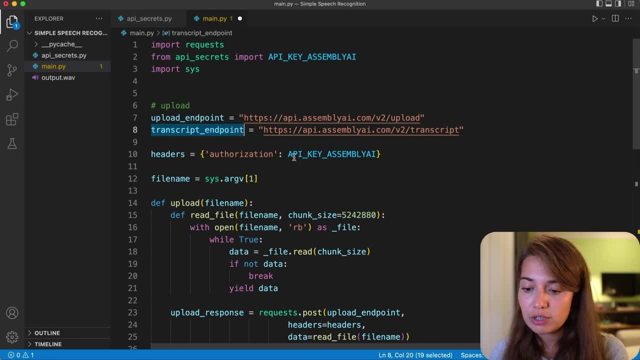 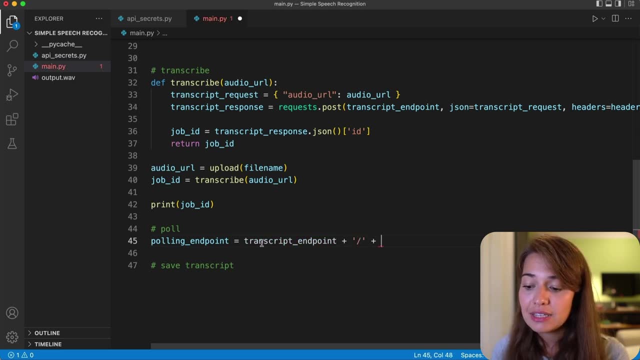 transcription job that you just submitted. So to create that, all you need to do is to combine transcript endpoint With a slash in between and add the job ID. but the job ID is a bit weak, So I'll just going to call this transcript ID. So by doing that, now you have a URL that you can ask to assembly AI, with which. 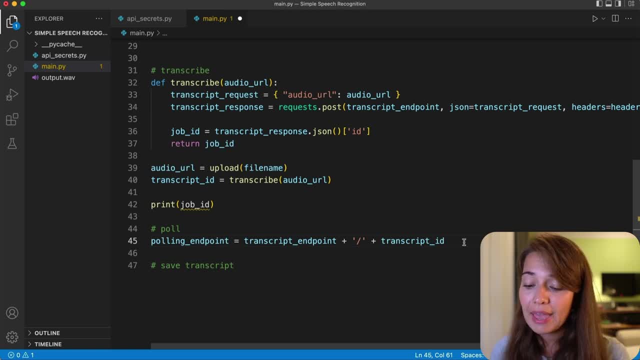 you can ask assembly AI if your job is done already or not. And again, we're going to send a request to assembly AI. this time is going to be a get request. Well, I'll just copy this so that it's easy: Instead of post is going to be a get request. we're going to use the polling endpoint instead of. 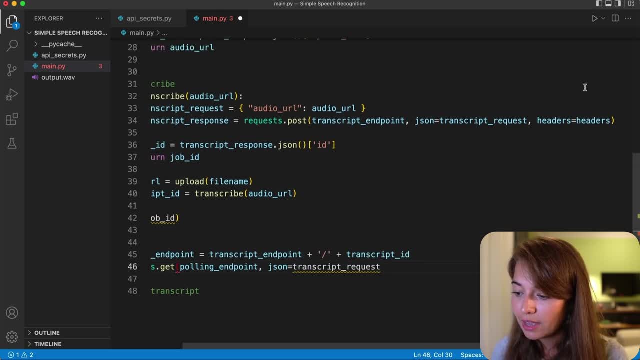 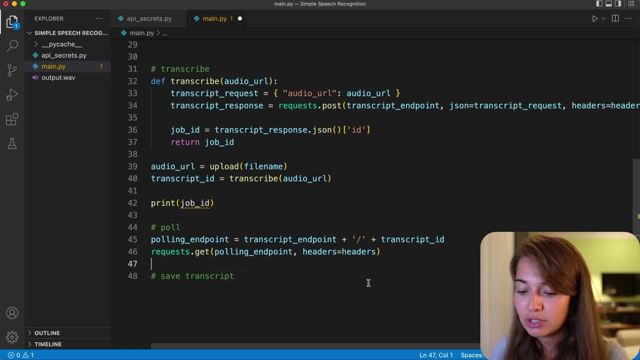 the transcript endpoint And we just need the headers for this. we do not, because we are not sending any information to assembly AI. we're just asking for information. If you're familiar with requests, normally this might be very simple for you, But all you need to know about this is that when you're sending data to an API, you use the. 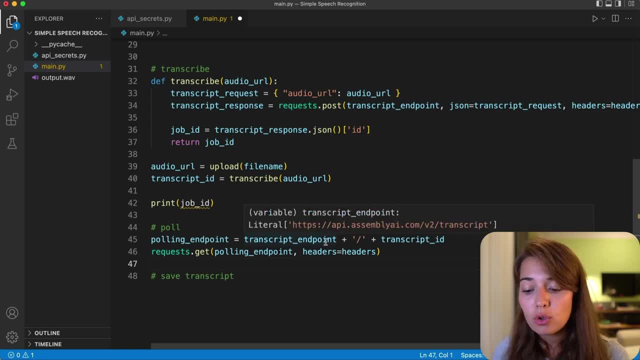 post request type And if you're only getting some information, as the name suggests, you use the get request type. The results that resulting, or the response that we get, is going to be called polling response. Let's see, it's not job ID, I called transcript ID so that it works. then we get the polling response. 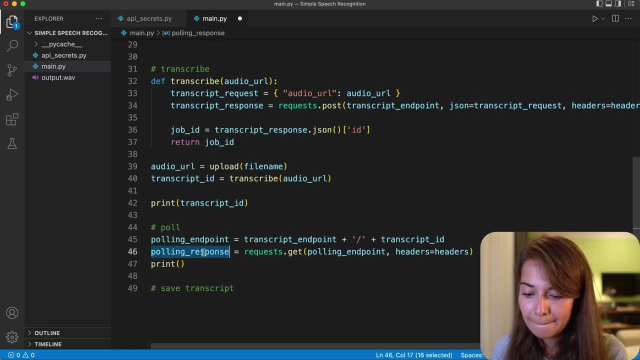 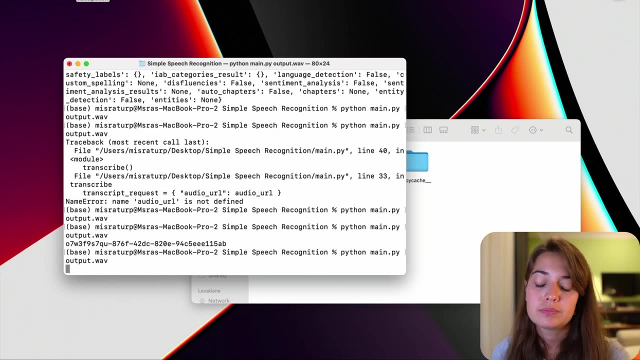 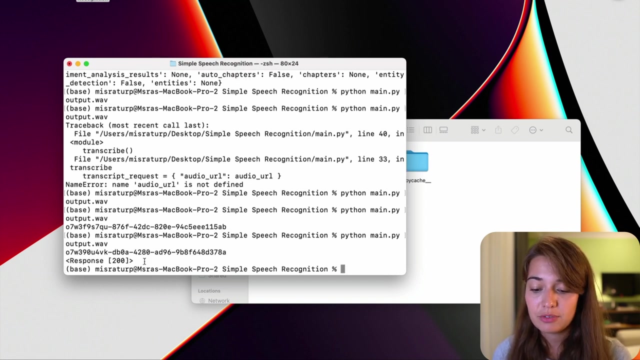 And I can also show you what the polling response looks like. Looks good, Okay, let's run this. All right. so if we got response 200, that means things are going well, But actually what I need is a JSON response. 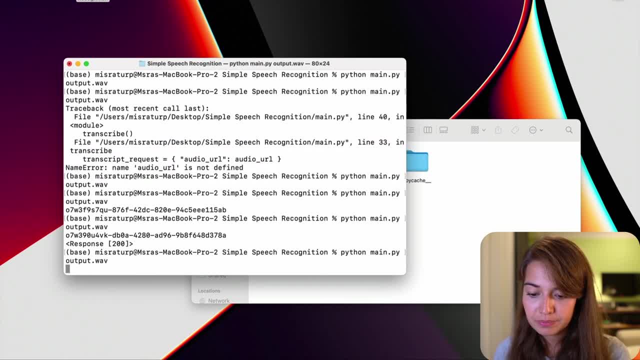 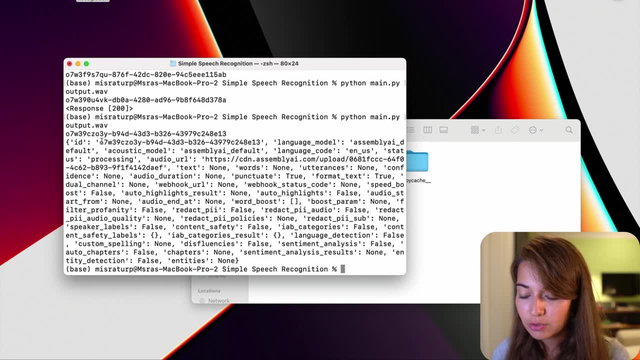 So let's see that again. Yes, this is more like it. So again, we get the ID of the response language model that is being used and some other bunch of information, But what we need here is the status. So let's see where that is. 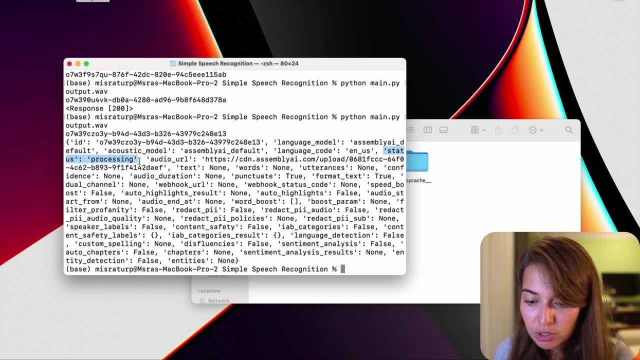 Oh yeah, there it is, So we have status processing. This means that the transcription is still being is still being prepared, So we need to wait a little bit more And we need to ask assembly AI again soon to see if the transcription is. 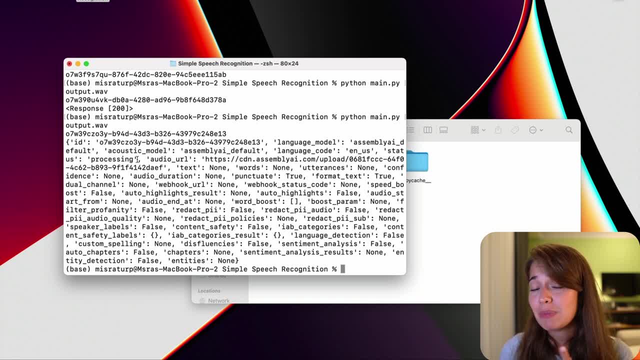 done or not. What we normally do is to wait 30 seconds, or maybe 60 seconds, depending on the length of your transcription, with length of your audio file, And then, when it's done, it will give us status completed. So let's write the. 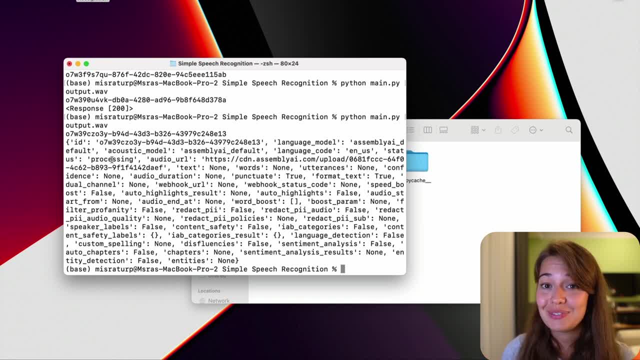 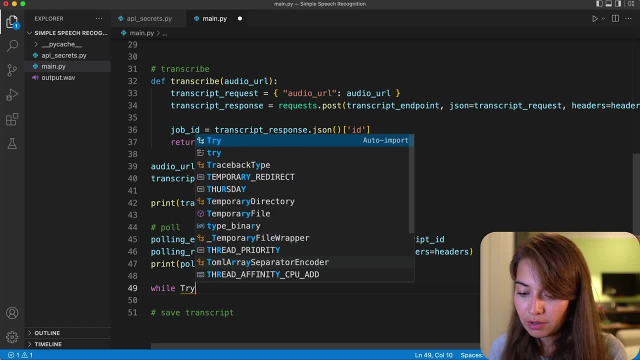 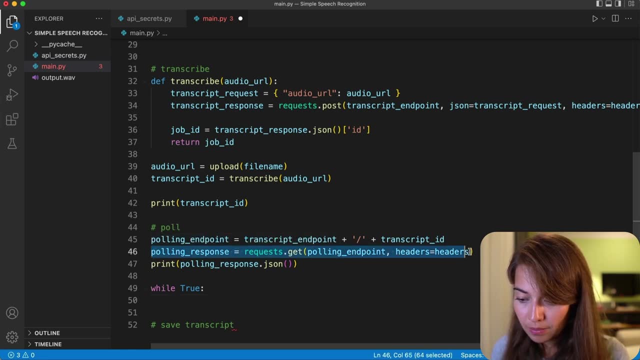 bit where we ask assembly AI Repetitively if the transcription is done or not. So for that we can just create a very simple while loop. while true, we do the polling And if polling response that JSON status equals to complete it. 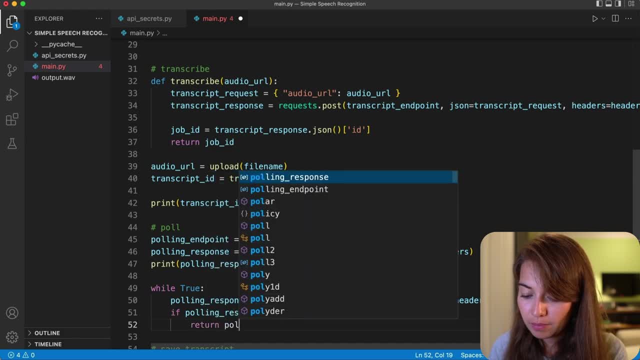 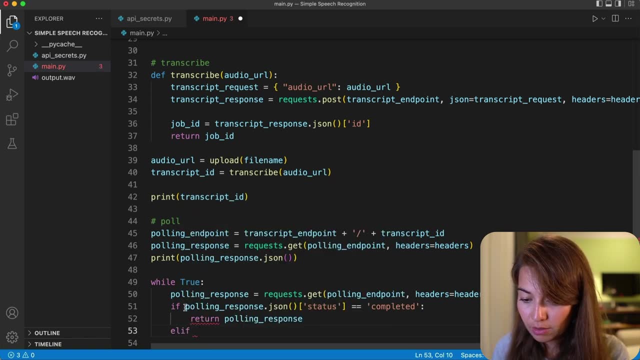 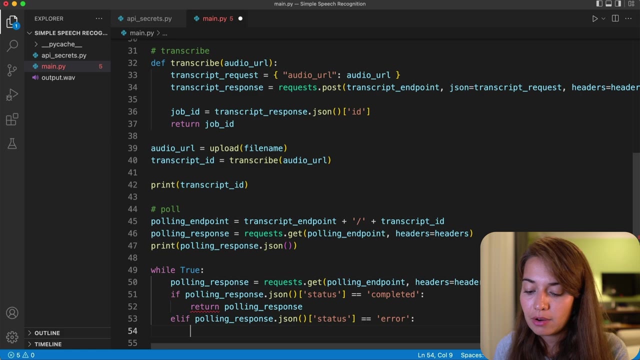 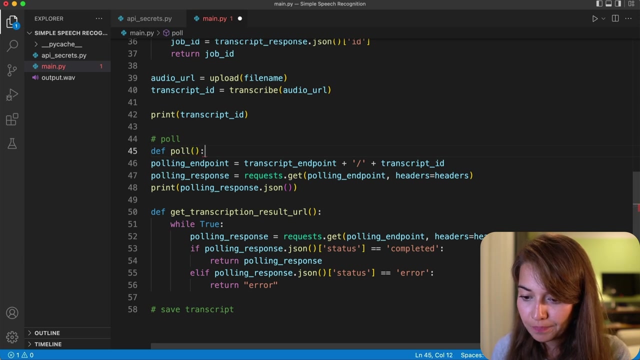 We return the polling response. But if polling response status is error- because it is possible that it might error out- then we will return error. I'll just wrap this into a function I can call this: gets transcription Results URL. And while we're at it, we might as well So wrap the polling into a function. Do we need to pass anything to it? 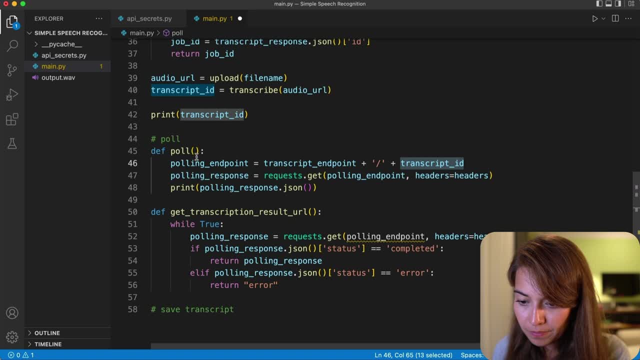 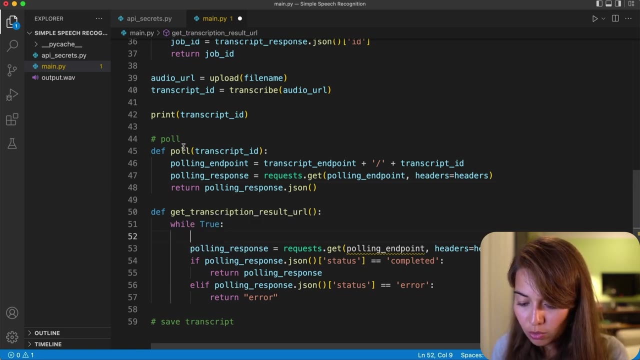 Yes, the transcript ID. you need to pass a transcript ID to it And instead of printing the response, we will just return the response. So instead of doing the request here, we would need to do is to call this function with the transcript ID. We can pass a transcript ID here, or might as well. I will just call. 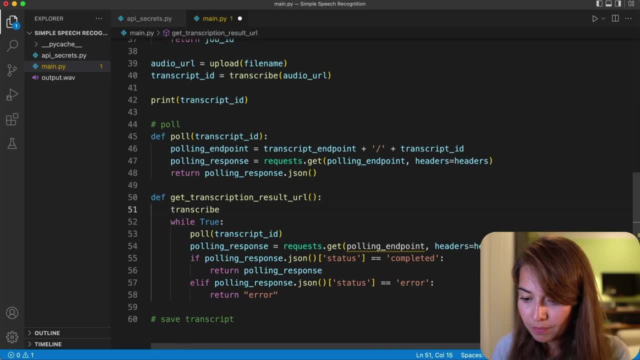 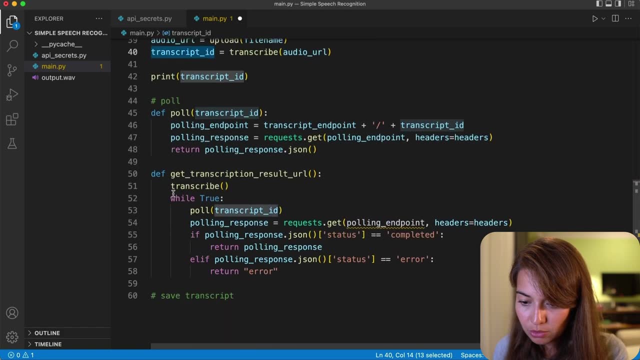 the transcription or transcribe function in here And the resulting thing would be the transcript ID from the transcription function And then I'm going to pass this transcript ID to the polling function. that is going to return to me the polling response. I will call this polling response data And inside this data, so this is not needed anymore. 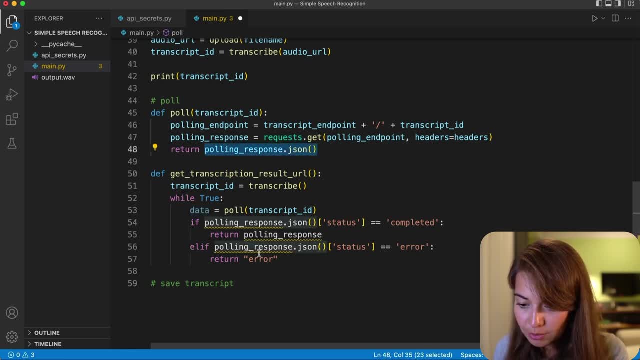 Yeah, this, this, So the polling response that, Jason, is what is being passed. I call that the data, So I changed this to data here And also data here. Yeah, then I'll just pass the data. If it's error, I can still pass the data just to see the response and what kind of what kind of error that we got. 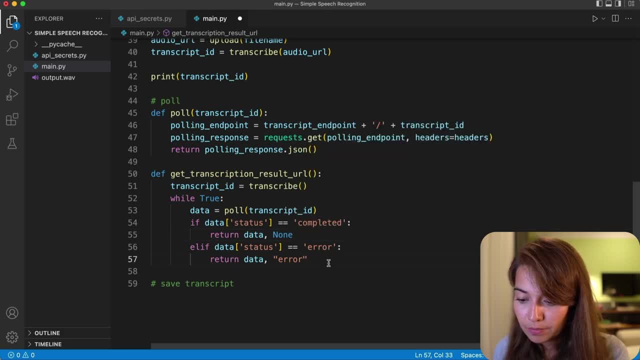 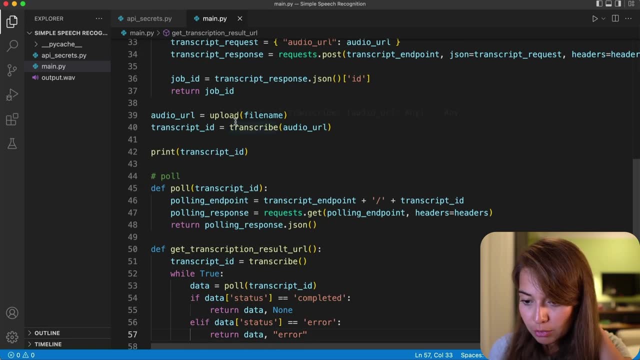 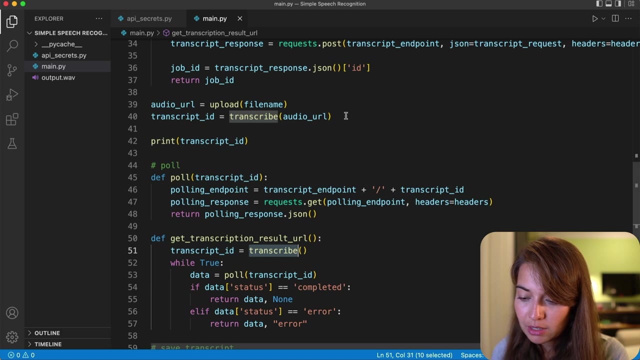 And here I'm going to just say none. All right, let's, let's do a little cleanup. So we have a nice upload function, a transcript function. What we did before was we were calling the upload function, getting the audio URL and then passing it to transcribe. but I'm running transcribe here, So I do not need this anymore. I still need to pass the audio URL to transcribe, So then I would need to pass it to here. So instead of this, 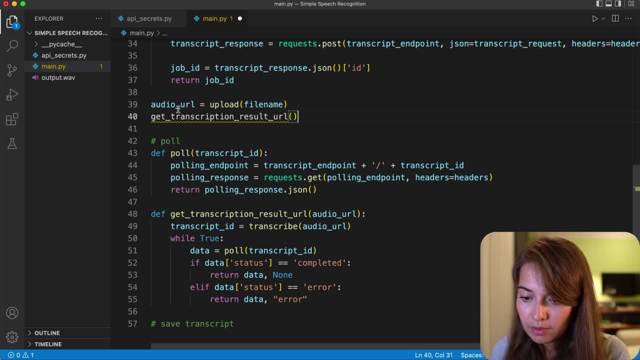 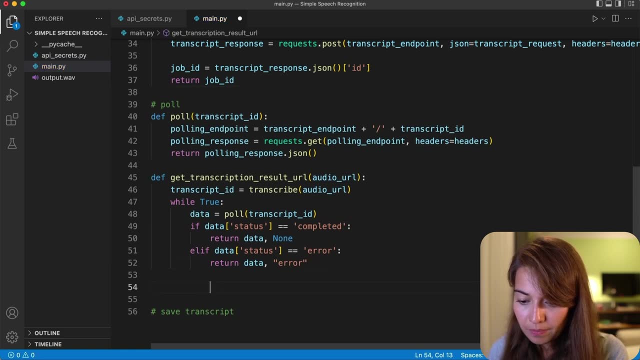 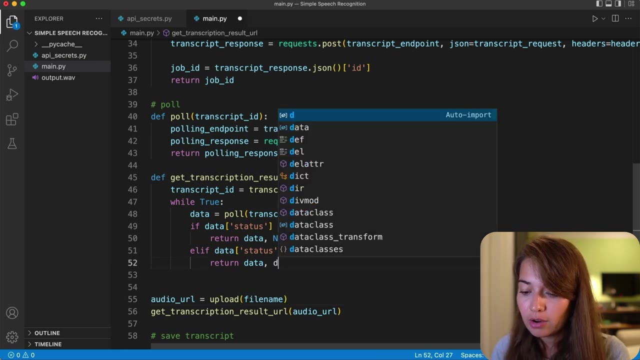 I just need to call this, This function with the audio URL. Yeah, let's put these here, Actually, to make it a bit more understandable, maybe instead of passing the string error, I can just pass whatever error that was that happened in my. 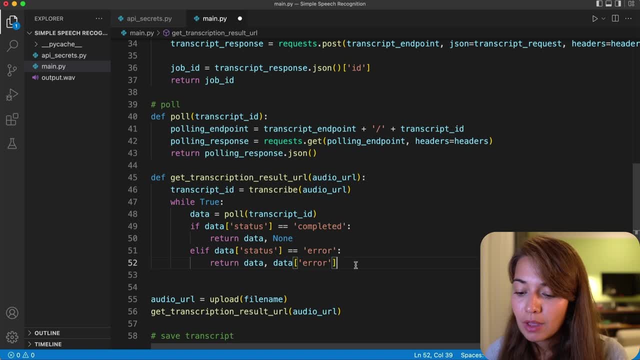 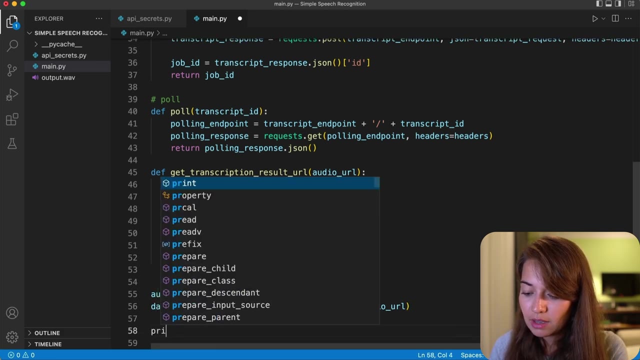 transcription, then you know, we'll be able to see what went wrong. Alright, so what we get as a result from get transcription, result ID is the data And, if there is any, the error. so then let's, why not run this and see what the data is going to look like? 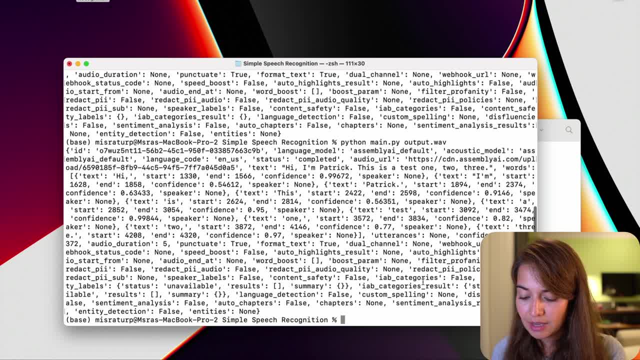 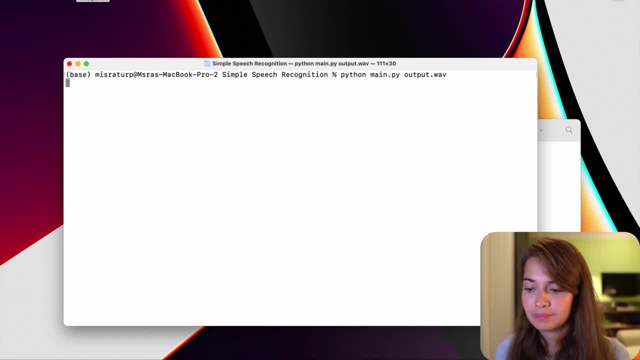 Alright, so we get something really, really big. Let's see, maybe I'll just clear this and run it again, just so that you know we can see it more clearly. Alright, so we get the ID again, the language model that is being used, et cetera. Now we want the results. Yes, it is under text. 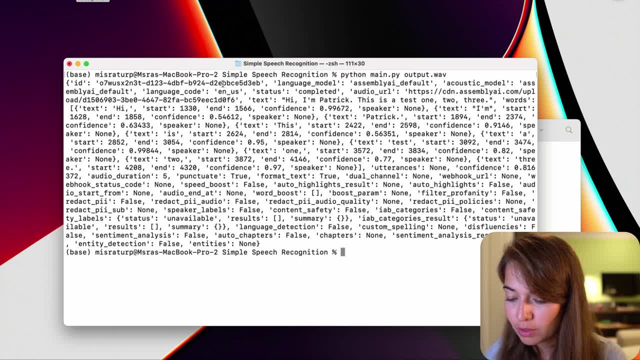 Alright, so we get the ID again, the language model that is being used, et cetera. Now we want the results. Yes, it is under text. Hi, I'm Patrick. This is a test. one, two, three. 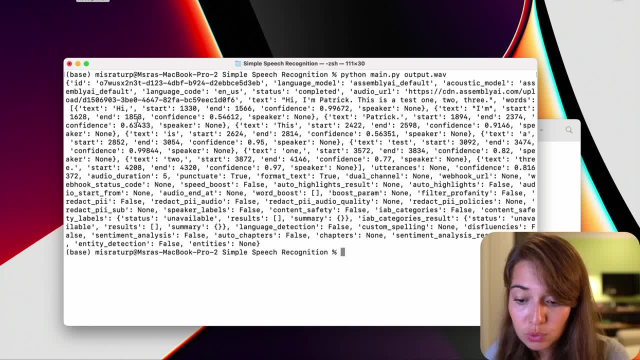 And we also get the breakdown of words, When each word started and then each word ended in milliseconds. confidence of this classification and much more information. What we want to do, though, even though we have all this information, we want to write this transcript. 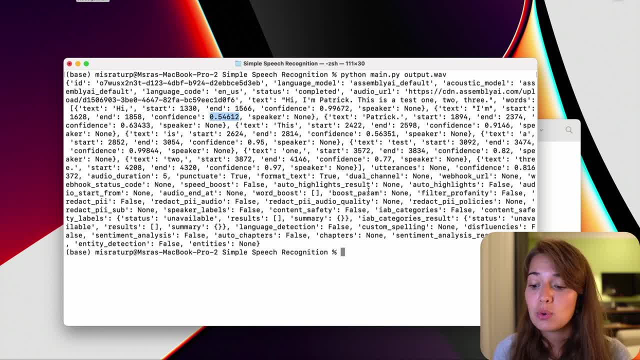 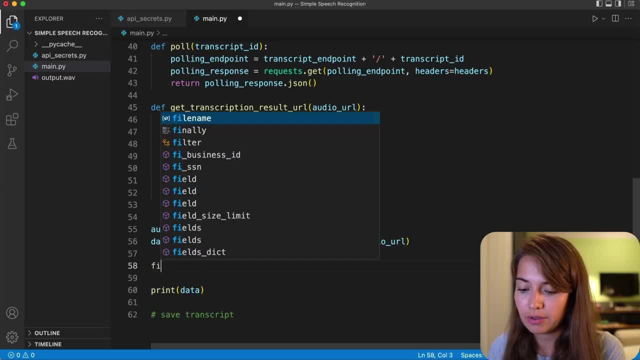 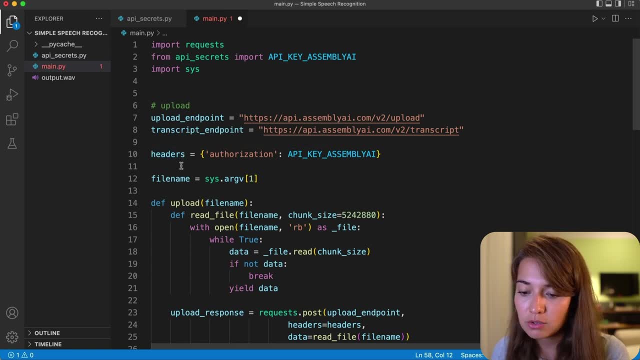 by assembly AI into a text file. So in this next step, that's what we're going to do. All right, let's come up with a file name for this file. We can call it- actually, we can just call it the same thing as the file name plus txt, So the file name. okay, we were using the argument. 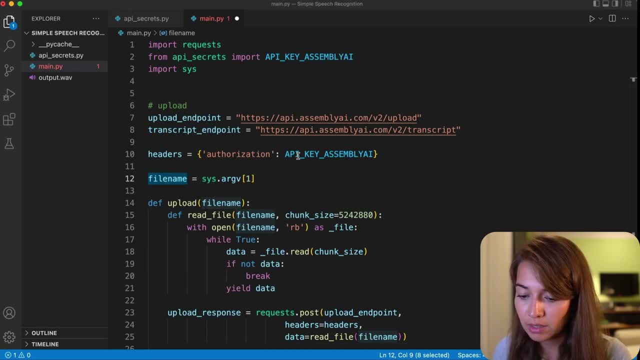 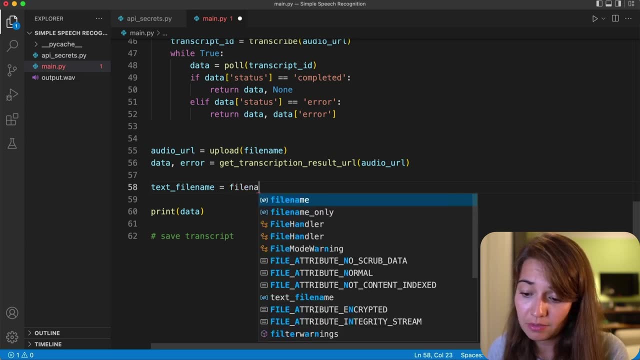 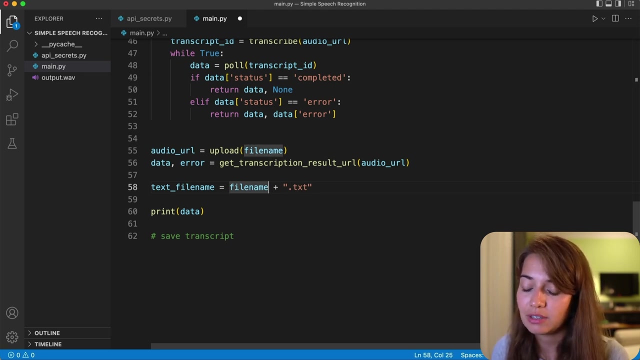 or variable file name too. So maybe let's find something else. We'll just call this text file name, And it will be the file name plus dot txt. We can also just, you know, remove the dots valve or dot mp4, or whatever, But let's not deal with that for now. So once I have this, 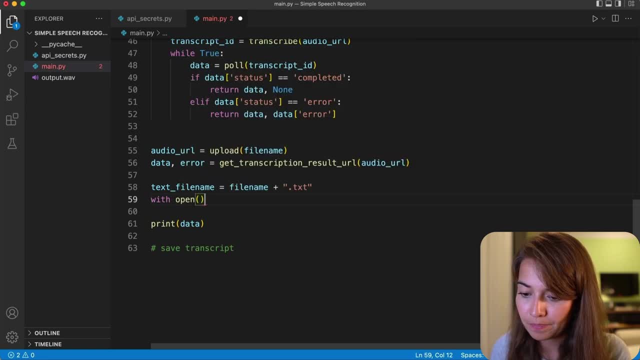 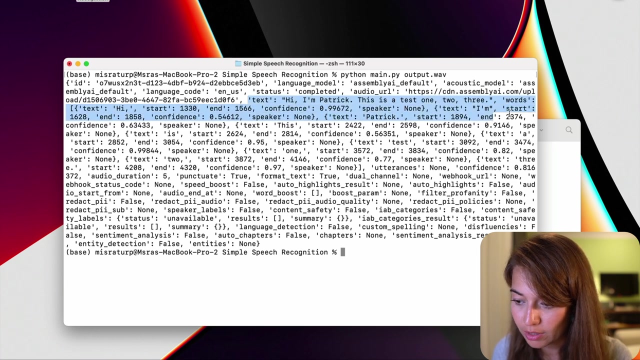 I will just open it. I will open it and write it And inside I will write data text, because that's where we have the text information of the transcript. If you remember, here this was a response we got and text includes the: 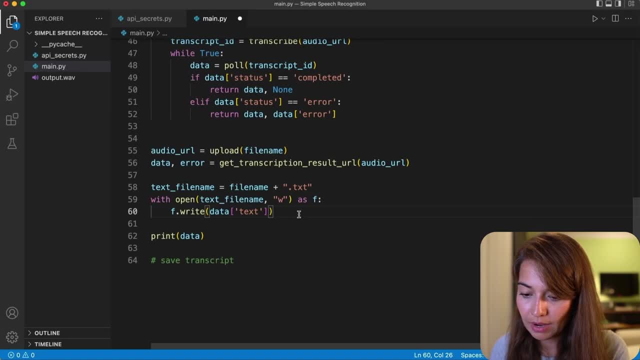 transcription And I can just prompt the user saying that transcription is saved. Transcription saved, We're happy. Of course, there is a possibility that our transcription erred out, So you want to cover that too. If you remember, we returned data and error. What we can do is you can say if data is returned. 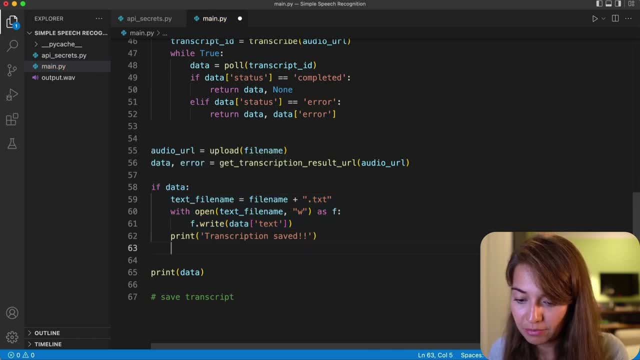 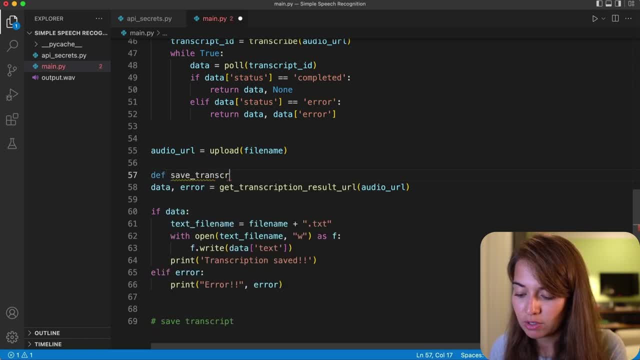 roll up in a function. we can call this: save transcript Data and error will be returned from Get transcript URL. It needs the audio URL, So I will just need to pass the audio URL here, And with that we're actually more or less ready. So let's run. 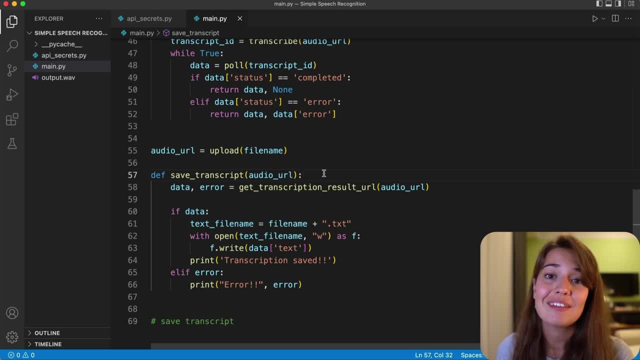 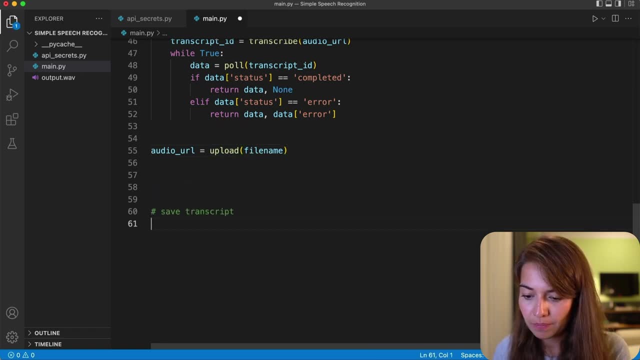 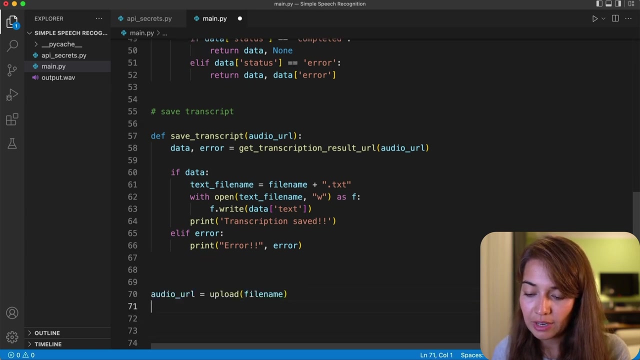 this and see if we get what we need: the transcript saved in a file For that. after the after calling the upload function, I can move this one here and calling the upload function here called upload function, And then I call the save transcript function. 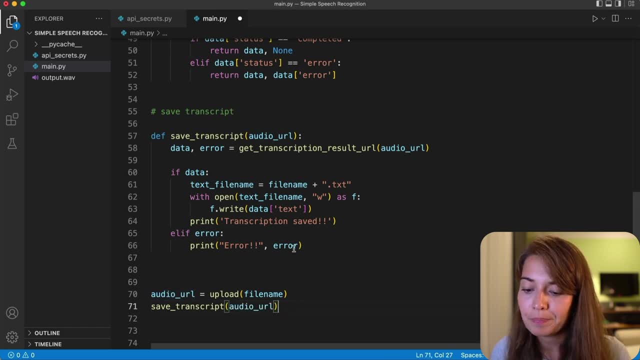 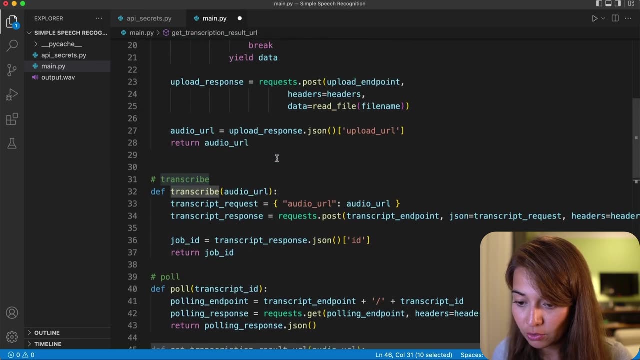 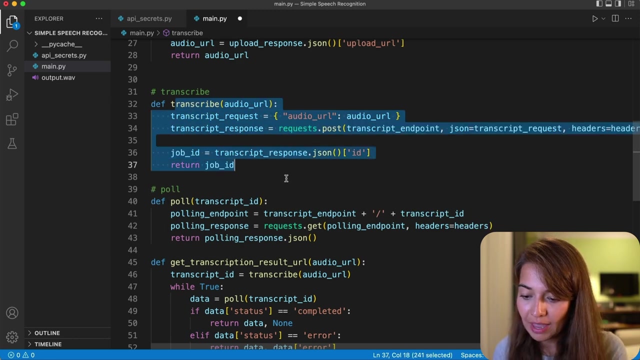 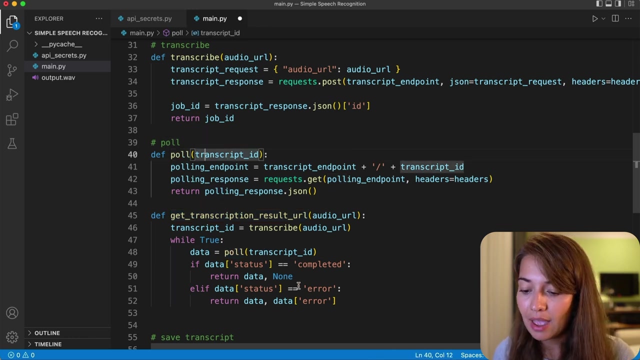 And let's quickly follow that up. I call the save transcript function equals get transcription result URL. get transcription result URL calls transcribe. transcribe is here. It starts a transcription process and then get transcription result URL also calls polling, So it keeps pulling assembly AI And when it's done it returns something and then we 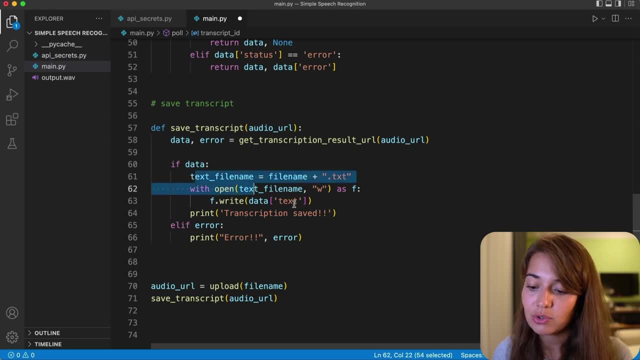 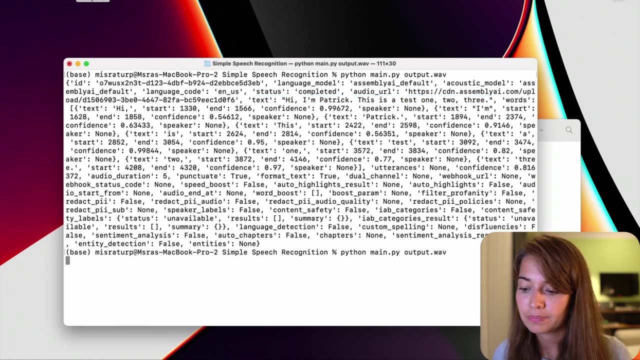 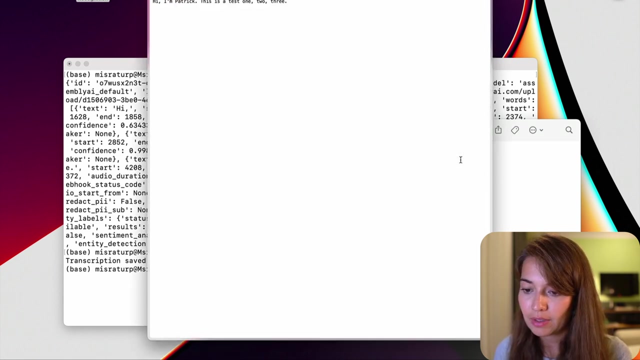 deal with it in the save transcript function and we either save a transcript or, if there's an error, we display the error. So let's run this and see if we get any errors. Transcription saved. All right, let's see Output valve dot txt. If I open it up, Looks: 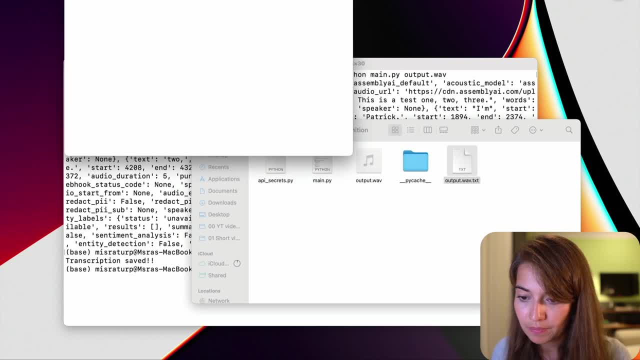 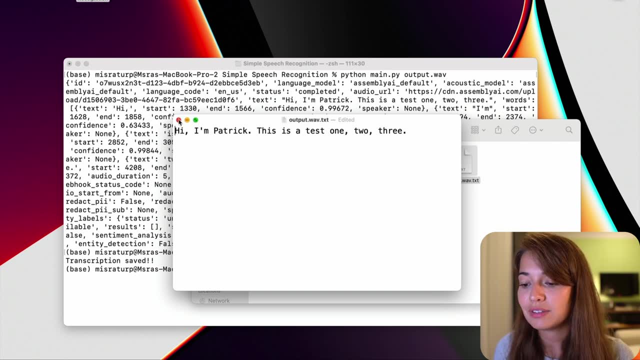 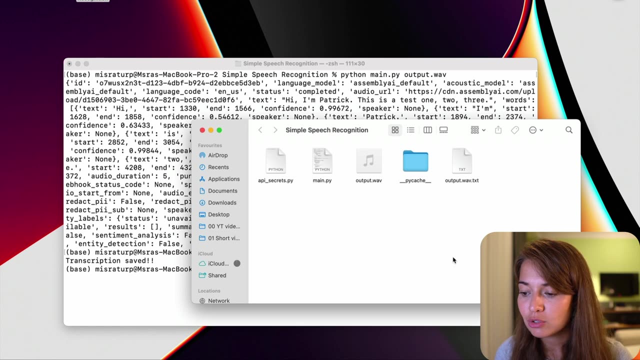 quite small. Maybe I can if I open it like this. Yes, Hi, I'm Patrick. This is a test. 123 is the result that we're getting, So that's awesome. We actually achieved what we wanted to do, So in this next couple of minutes, I actually want to clean up the code once. 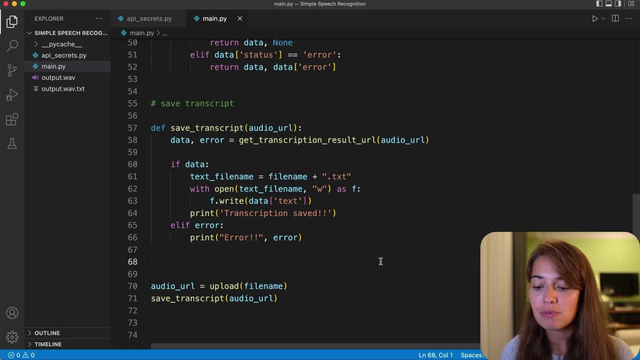 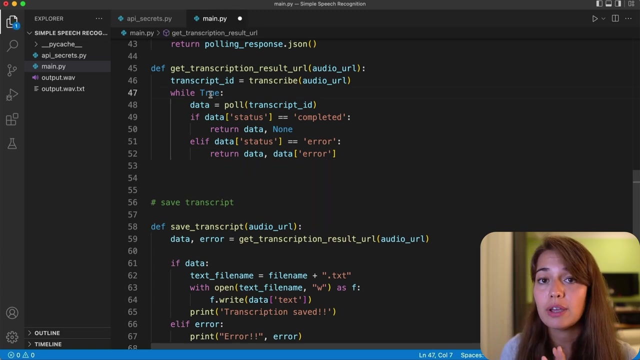 again, Because you're going to build a couple more projects And we want to have a Python file that has some reusable code, so we don't have to reinvent the wheel all the time. So let me first go here. Actually, when we're doing the polling, if we just have a while, true, 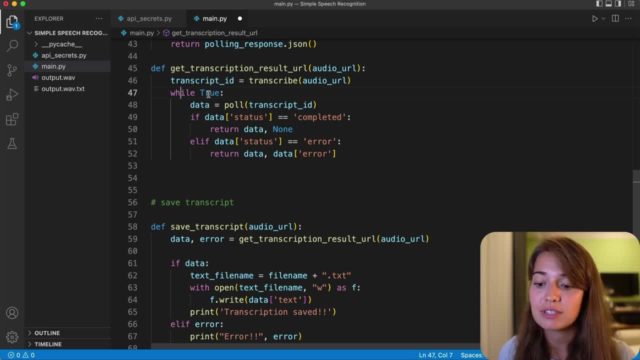 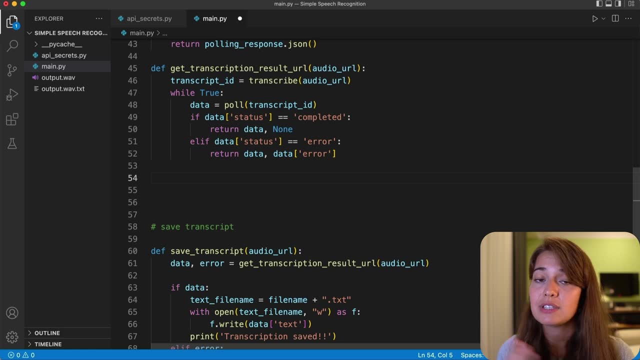 loop. it's going to keep asking assembly AI for results, And you know that that might be unnecessary, So what we can do is to include some waiting times in between So we can ask if it's not completed yet. Transcription saved, All right, so we're going to go ahead and do that. We're going. 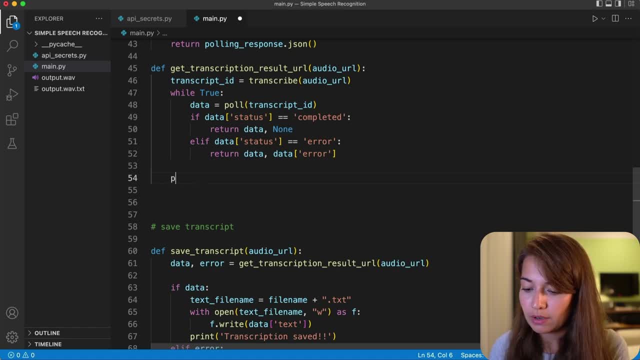 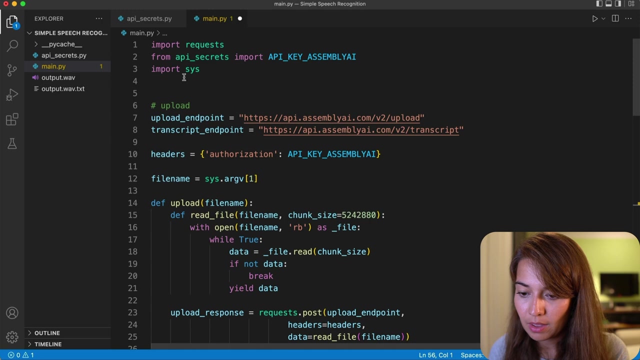 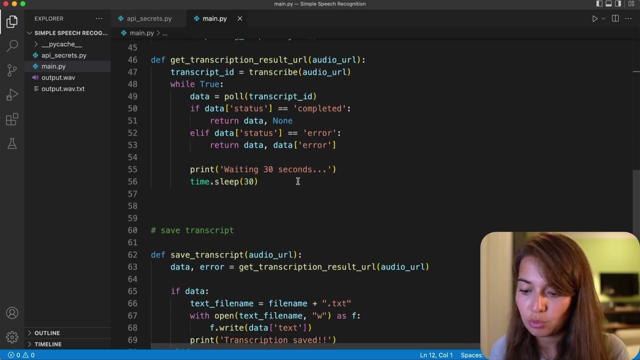 to wait- let's say 30 seconds- to ask again, So we can inform the user waiting 30 seconds. What I need is a time module, So let's call this 30. And I will just import time here, And this way it should be waiting 30 seconds in between asking. assembly AI. if the transcript 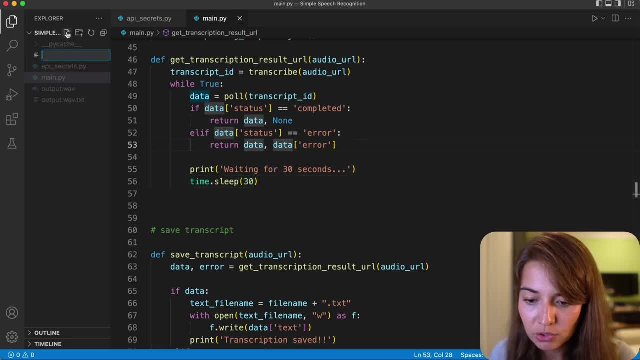 is ready or not, And okay, so this is going to be a 30 second wait. So I'm going to say that this is finished And that's how you're going to. So this is going to be a 30 second, And okay, let's create that extra file that we have API communication. I'll call it. Yes. 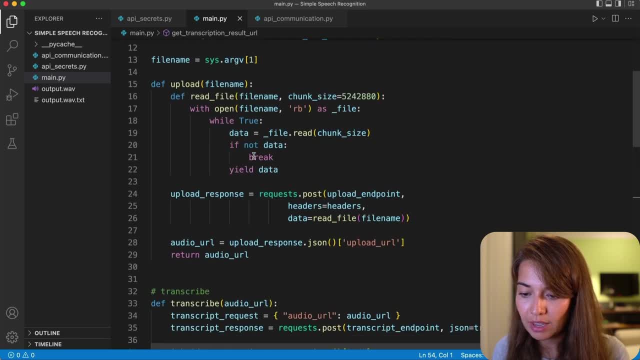 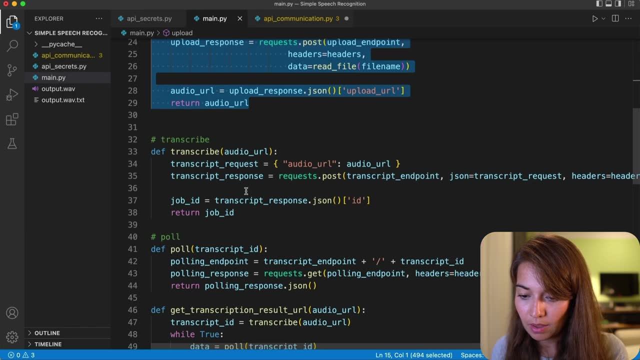 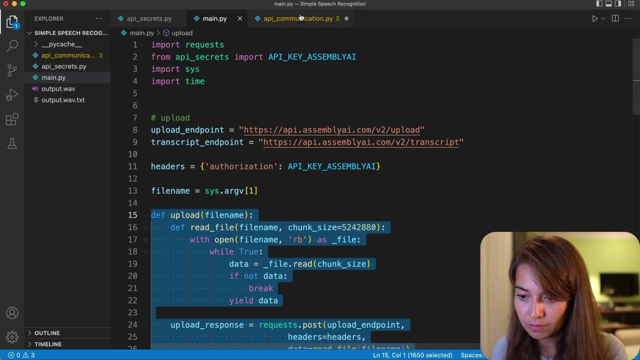 so I will move all of the functions that communicate with the API there. So I need to move the upload function, I need to move transcribe. pull all of these actually. So just remove that. yeah, Let's see, did we miss anything? 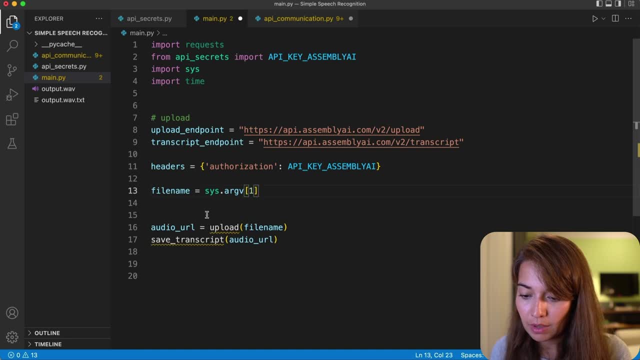 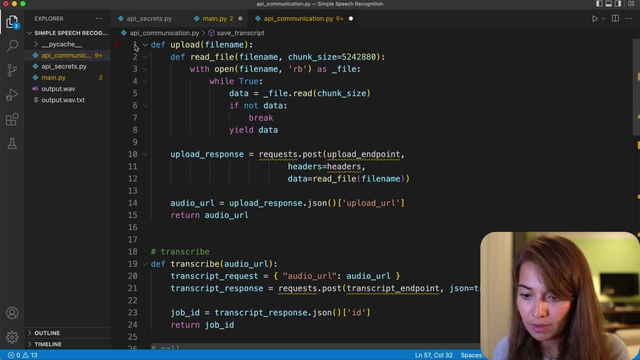 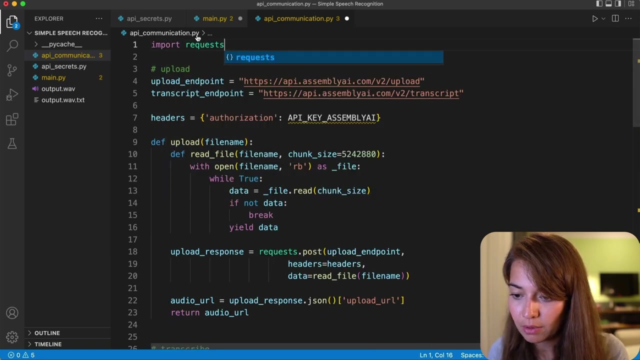 No, I'll just remove these from here. File name can stay here. of course, headers and the upload and transcript endpoints need to live here because they are needed by the functions In here. we have to import the requests library So we don't need it anymore here. 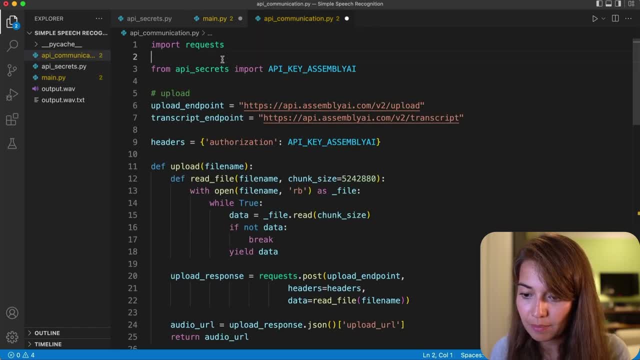 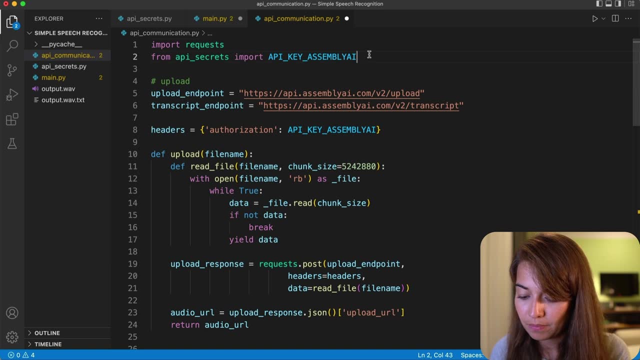 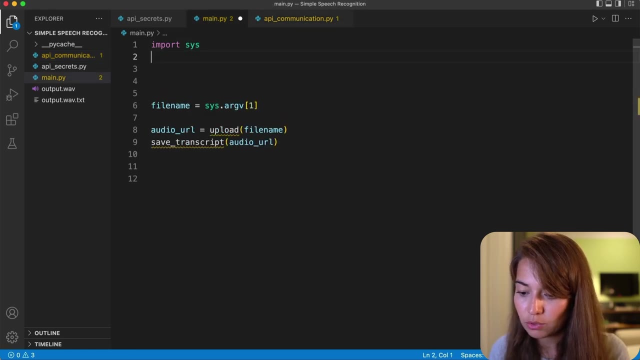 We need to import the Assembly AI API key System needs to stay here, time needs to go there. And we also need to import from API communication import. we'll just say all, And that way we can use these function in our main Python script. 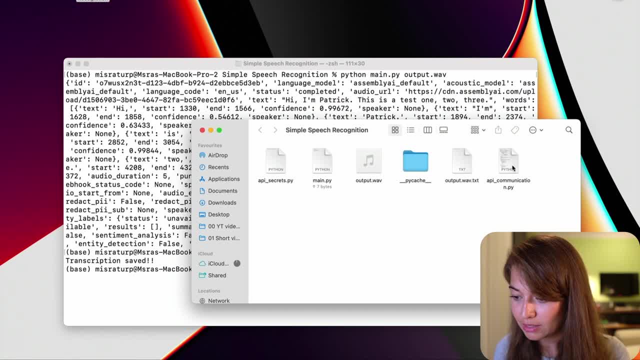 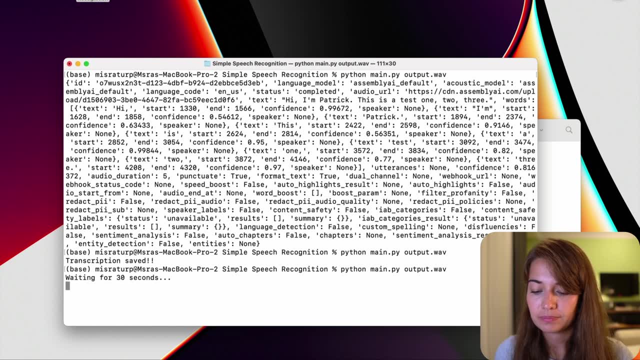 I will run this again to make sure that it is still working. So I will delete the text file that was created. I will keep the output Nice. So we also get the prompt that the program is waiting 30 seconds before asking again. 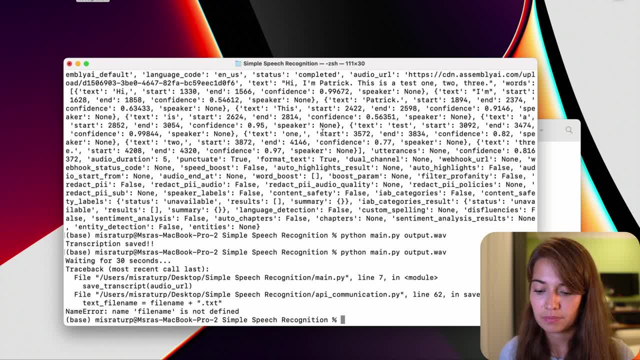 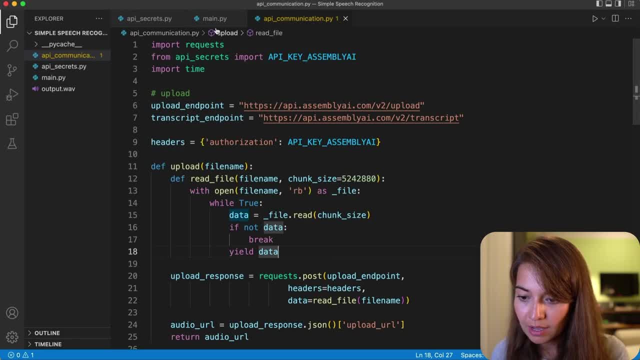 Oh yeah, we passed the file name, but of course it might not exist there, So let's go and fix that. The file name is here. We only pass it to the upload function, And the upload function is here now. 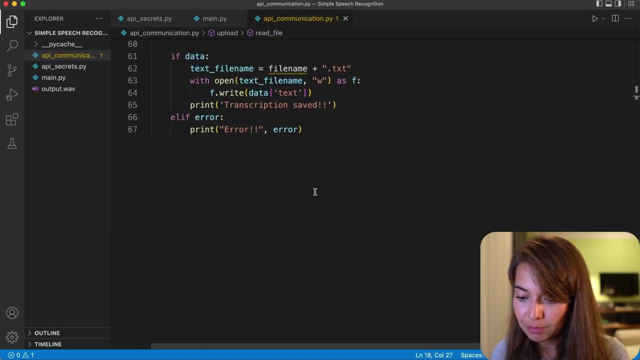 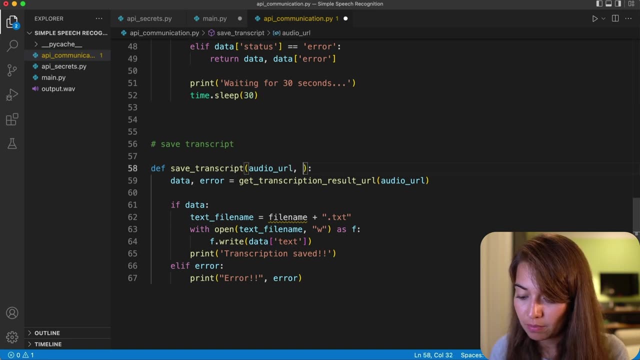 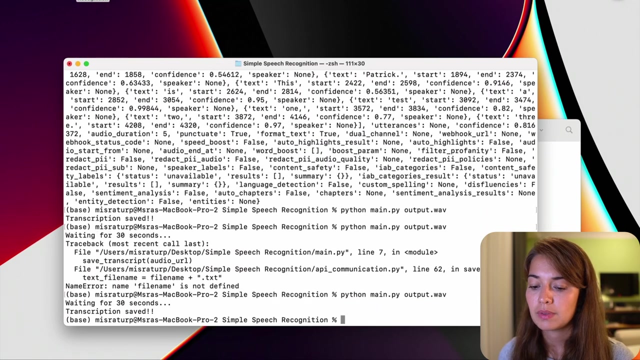 And, And. in the save transcript we do not pass it, but we are actually using it. So what we can do is to just also pass the file name here, And that should be fine. It should fix the problem. Transcription saved. 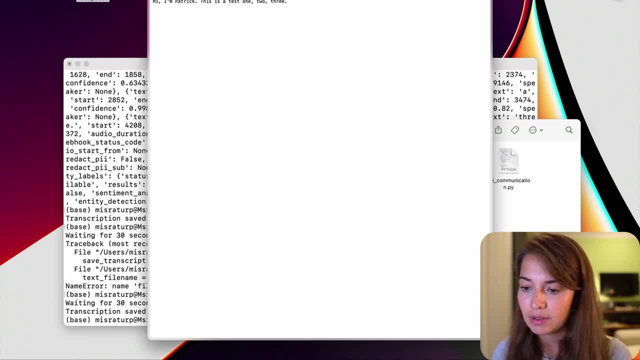 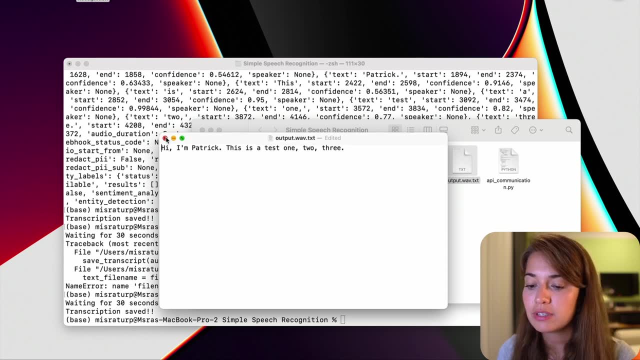 All right, Let's see Output. Hi Like this. Hi, I'm Patrick. This is a test 123. So this is a very short test. This is a very short audio file And we've actually been using it over and over again. 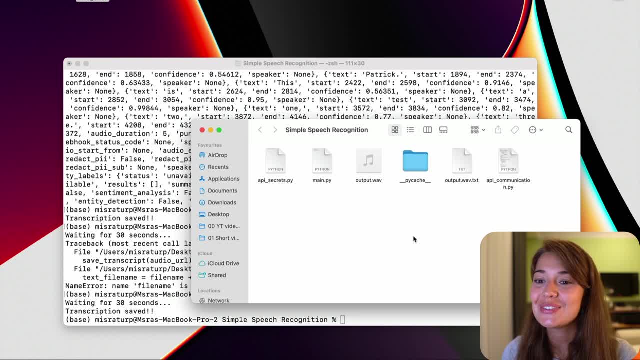 So I want to also show that this code is working to you using another audio file. This is the audio of one of the latest short videos that I made for our YouTube channel. I was just talking about what natural language processing is, So this time maybe if I add underscores, it will be easier to call. 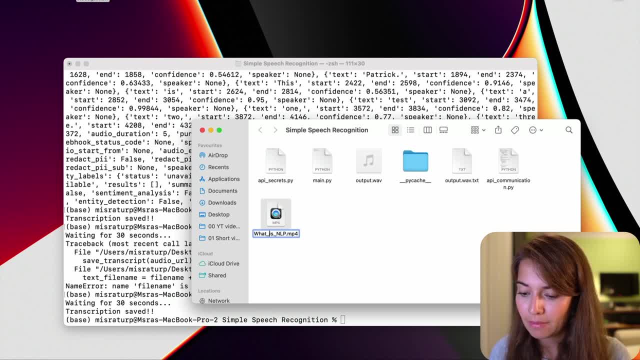 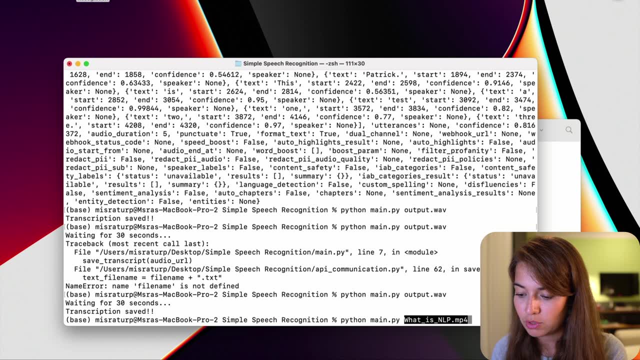 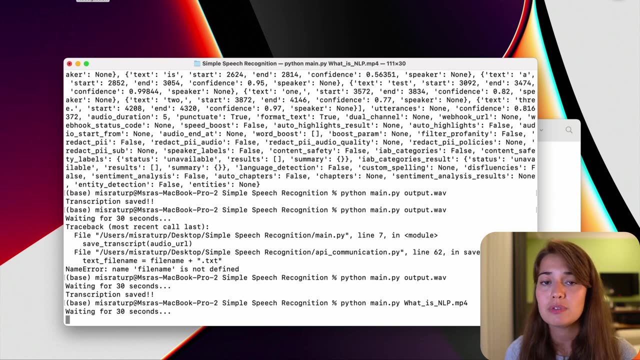 Okay, Okay, Okay, Okay. Yes, I'll just copy its name And when I'm calling the script, I will use its name. This will probably take a little bit longer, because the audio file we've been using is only a couple of seconds and this one is one minute. 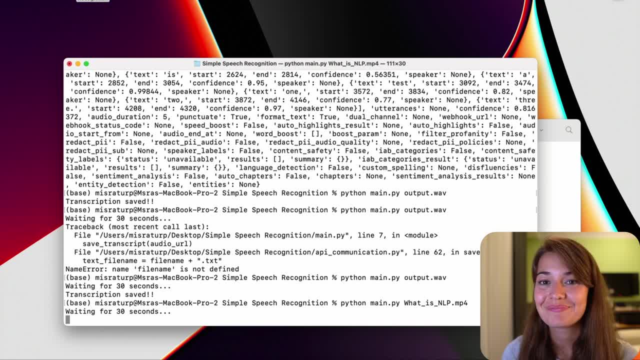 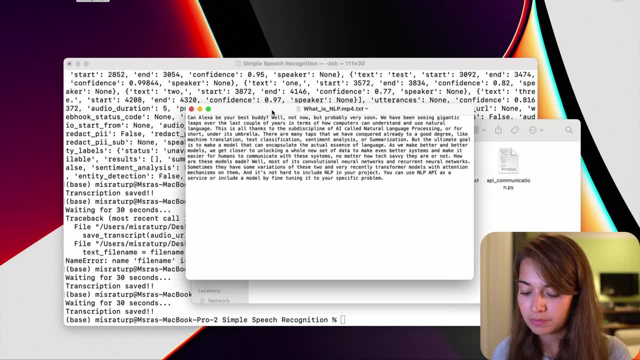 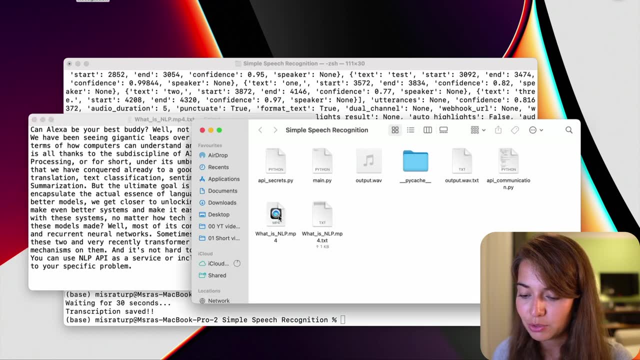 So we will see what the results are going to show us. Right, Here we go. The transcription is saved. We find it here, Right, Okay, All right, This is exactly what I was talking about. Let's listen to it while the transcription is open. 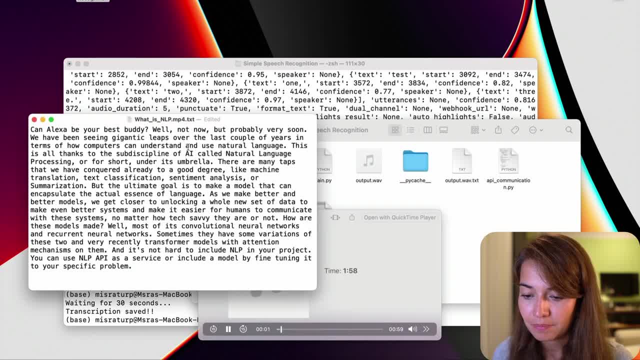 Can Alexa be your best buddy? Well, not now, but probably very soon. We have been seeing gigantic leaps over the last couple of years in terms of how computers can understand and use natural language. All right, You get the idea. So our code works. 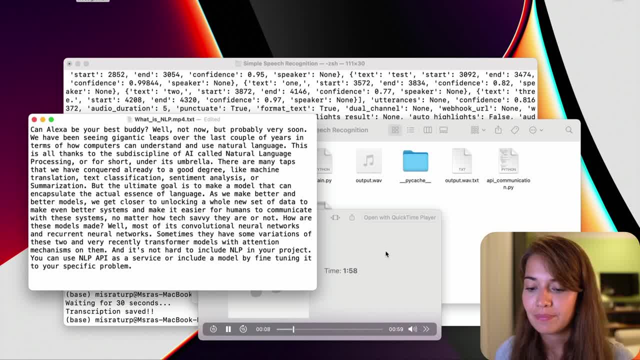 This is amazing. I hope you've been able to follow along. If you want to have the code, don't forget that you can go get it in the GitHub repository. We've prepared for you using the code. All right, Thank you. 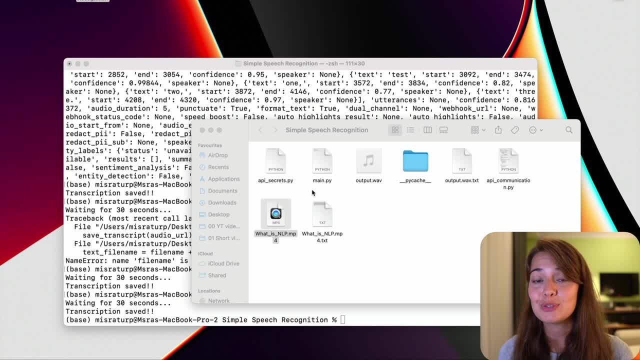 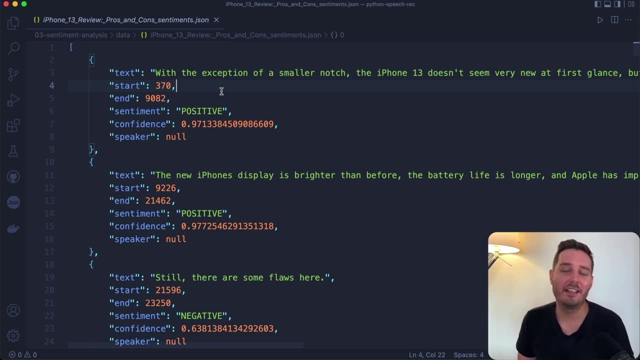 You can see the link in the description. Welcome back to the third projects. on this one, I teach you how to apply sentiment analysis to YouTube videos, So you will learn how to use the YouTube DL package to automatically download YouTube videos or only extract the information you need. 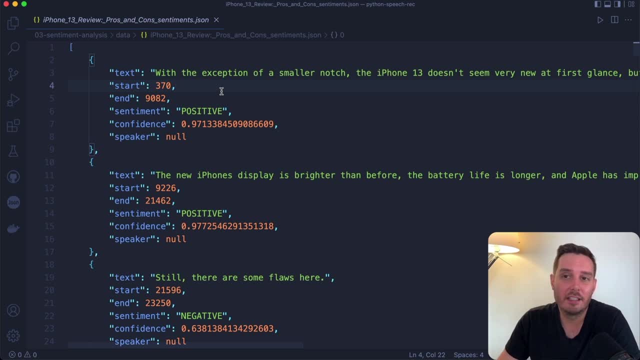 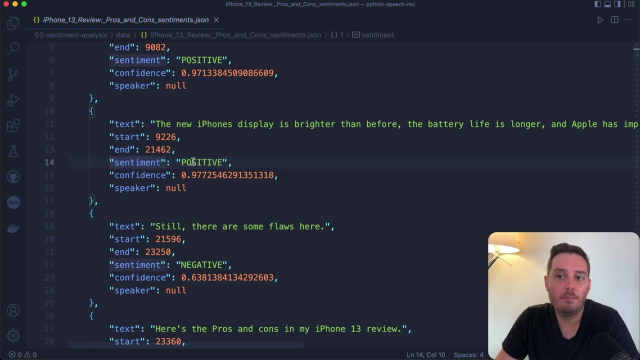 And then I also teach you how to apply sentiment analysis. So in this example, I use iPhone 30 review videos and the result that we get looks like this: So for each sentence in the video, we get the text And then we also get the sentiment. So this could be positive, negative or neutral, For example. 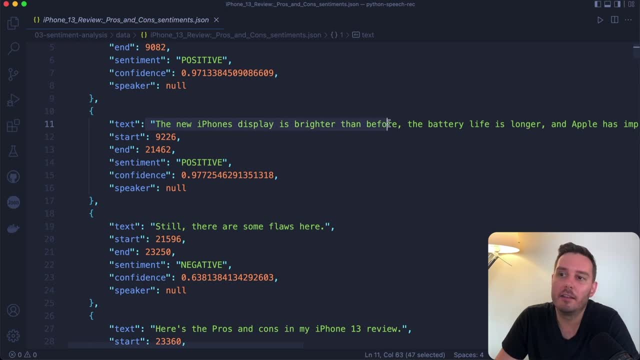 if we read this text here, the new iPhone display is brighter than before, the battery life is longer and so on, And the sentiment is positive. And here the text is still, there are some flaws And now the sentiment is negative. So this works pretty well And this can be applied to so many use cases. 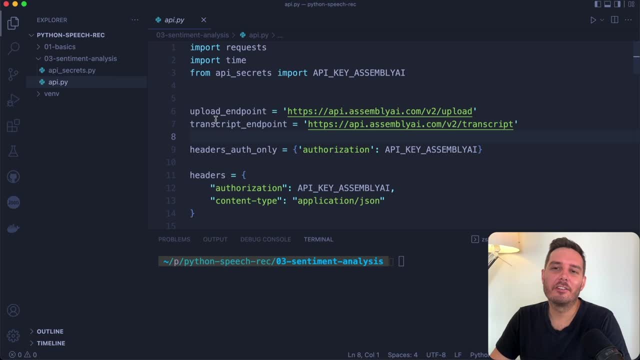 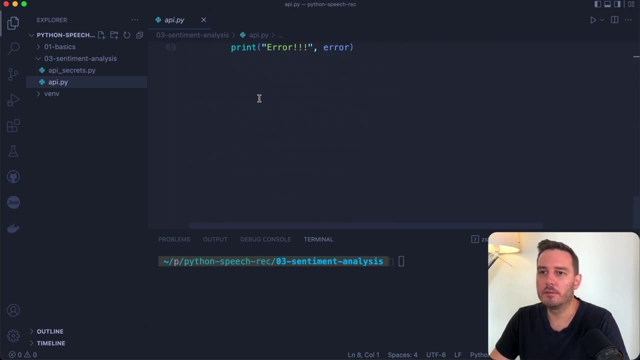 So let's get started and see how to do this. So here I've created a new project folder And we already have our API secrets and the API PI file with the helper functions to work with the assembly AI API. And now let's create two more files, So the mainpy file that will combine. 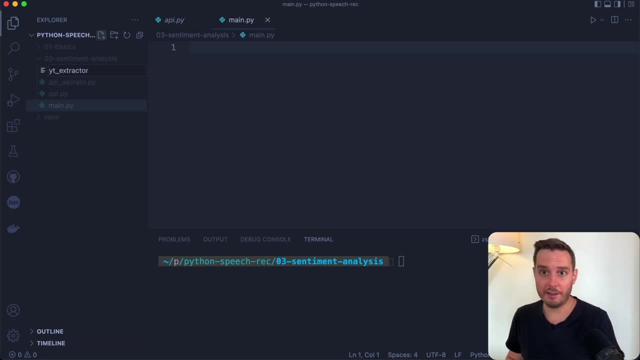 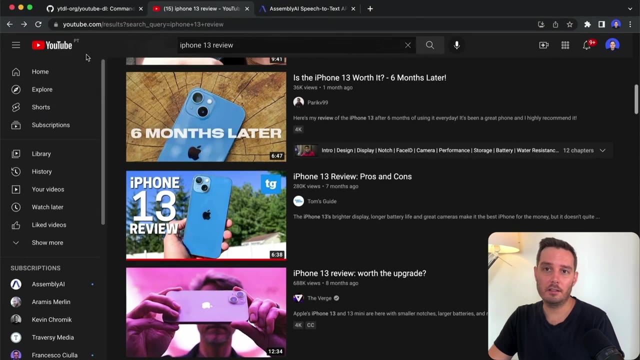 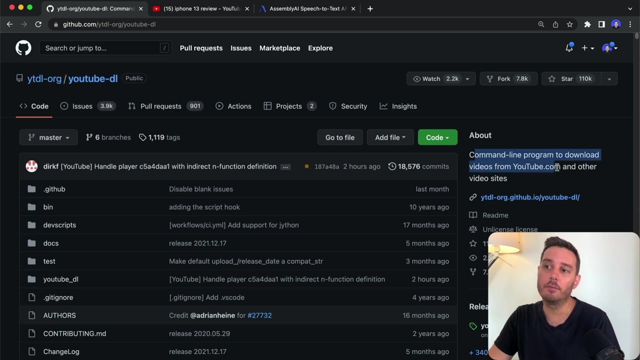 everything and the YouTube extractor files. This is another helper file to extract the infos from the YouTube video, And for this we are going to use the YouTube DL package. This is a very popular command line program to download videos from YouTube, YouTube and other sites And we can use this as command line program, But we can also use this in 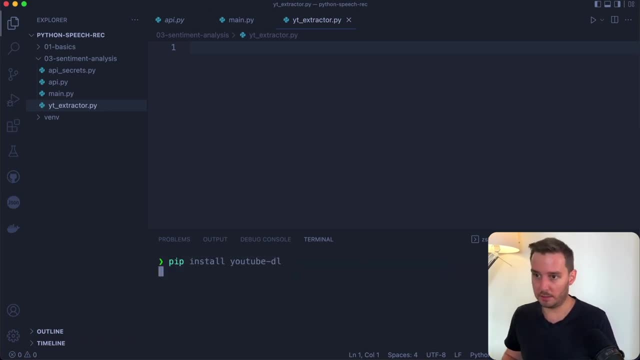 Python. So for this we say pip, install YouTube DL, And then we can import this. So we say import YouTube DL, And then we set up an instance. So we say y DL equals YouTube DL, dot YouTube DL. And now I'm going to show you how you can download a video file and also how you can 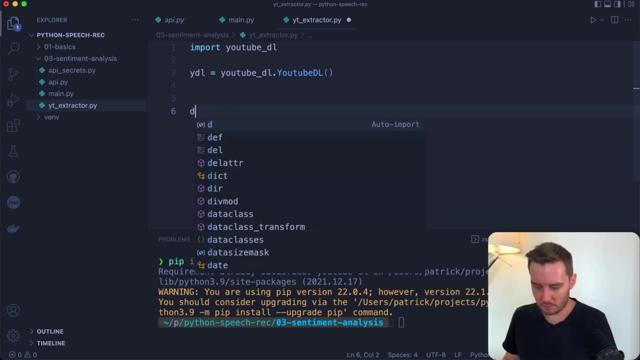 extract the infos from a video. So let's create a helper function that I call get video infos And this takes an URL, And now we use the y DL object as a context manager. So we say with y DL, then we say result equals y DL, dot extract info And this gets the 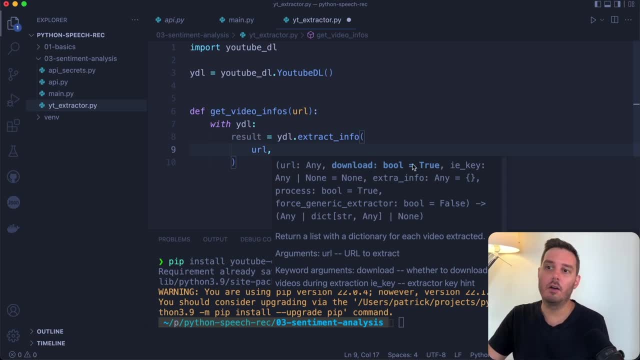 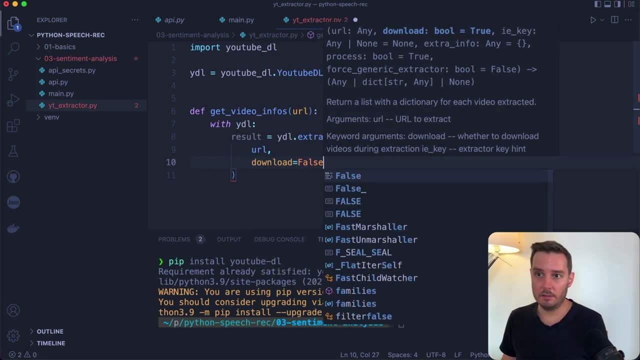 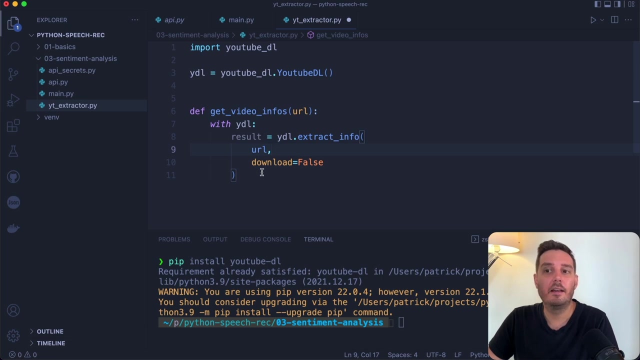 URL And by default it has download equals true. So this would also download the file. But in my case I say download equals false Because of course we could download the file and then upload it to assembly AI. But we can actually skip this step and just extract the URL of the hosted file. 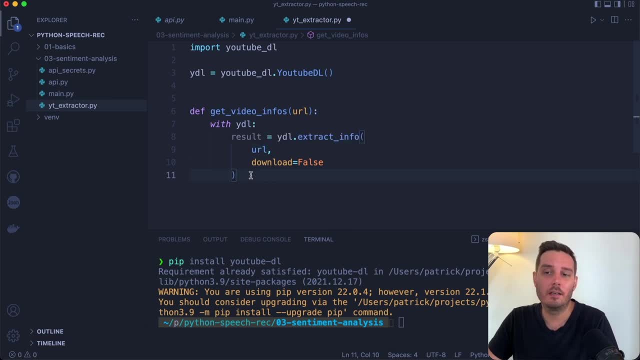 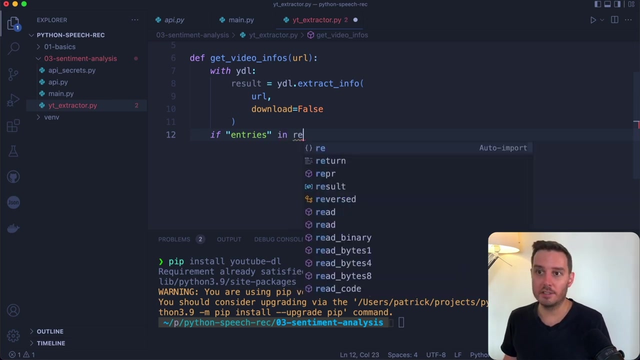 And then we can pass this to the transcribe endpoint in assembly AI So we can set download equals false here. then we do one more check So we say if entries, if the entries key is in the result, then this means we have a playlist URL here. And then we 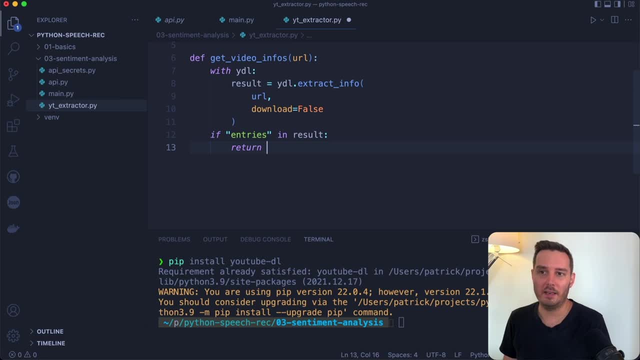 want to return only the first video of this playlist. So we say return result with the key entries and then the result zero or entry zero, And otherwise we return the results simply. So this is the whole video info object. And then let's create another helper file that I call get audio URL And this: 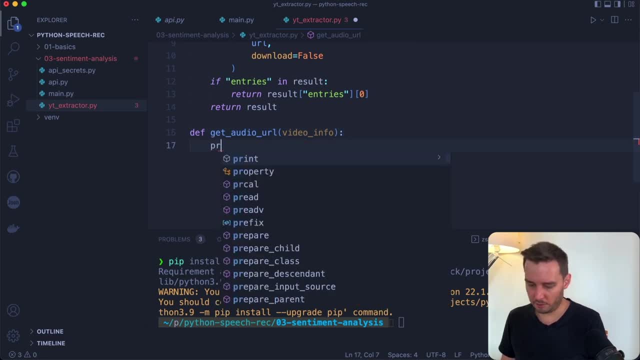 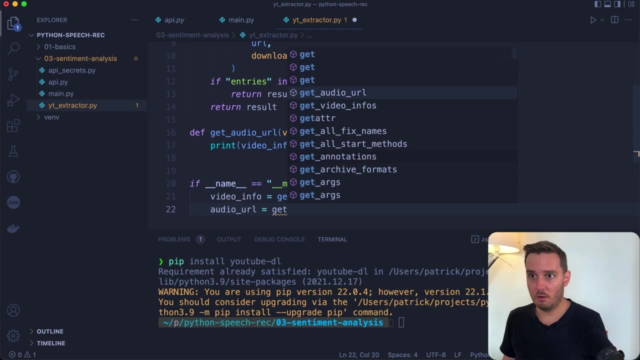 gets the video infos, And first of all let's simply print all the video infos to see how this looks like. So now let's say if underscore name equals equals main, And then let's first extract the video info. So video info equals get video infos. this needs an URL. And then we say audio URL equals get audio URL. 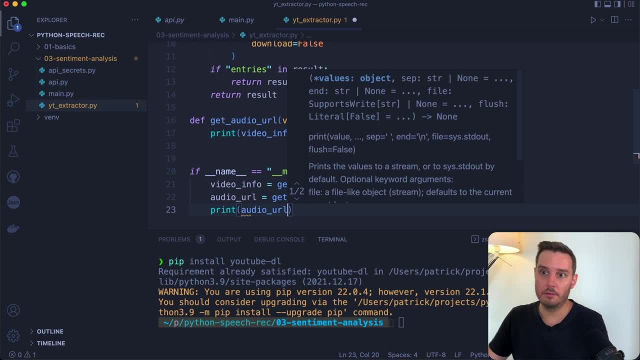 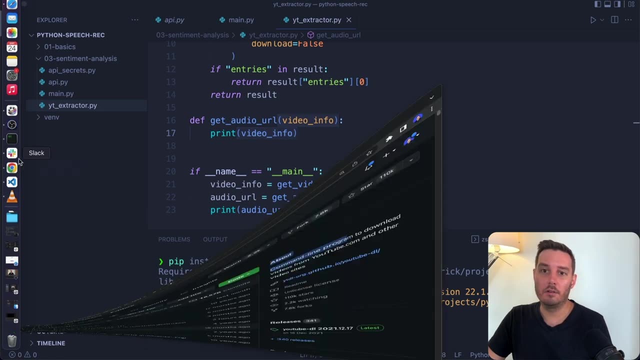 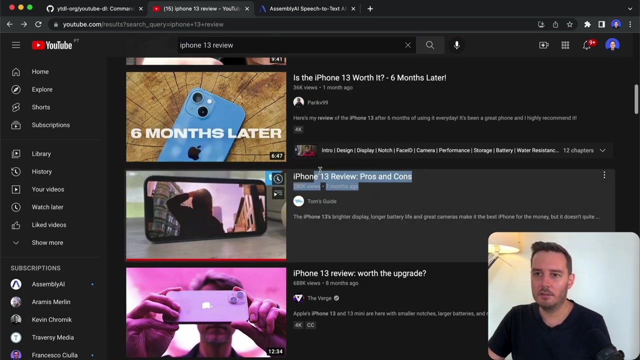 And then we want to print the audio URL. So right now this is none because we don't return anything. get an example URL. So for this I went to YouTube and search for iPhone 13 review And I choose this video. So I found 13 review pros and cons. So we can click on this and 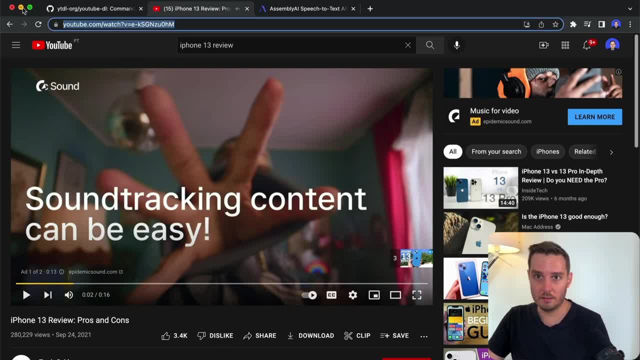 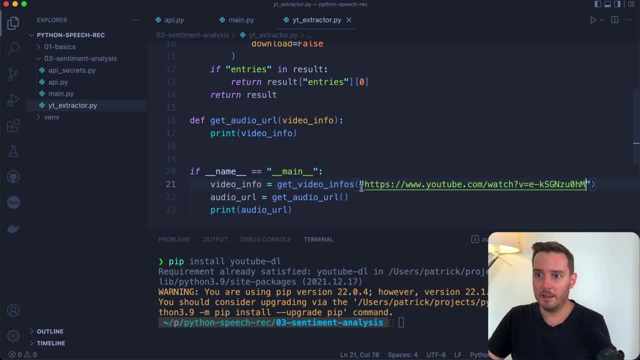 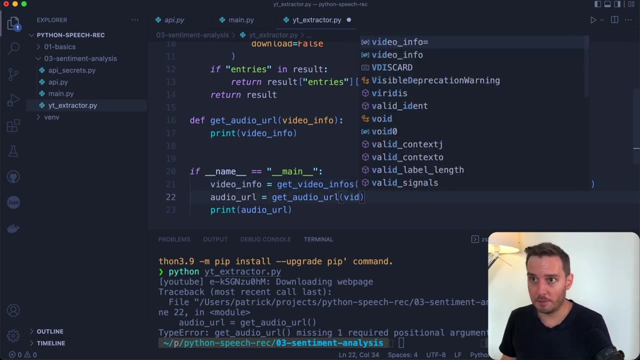 then we have to watch an ad. but we can actually copy this URL right away And then put it in here as a string. And now, if we run this, then so we run Python YouTube extractor dot pi, then it should print the whole URL. So yeah, actually here I have to pass this YouTube. 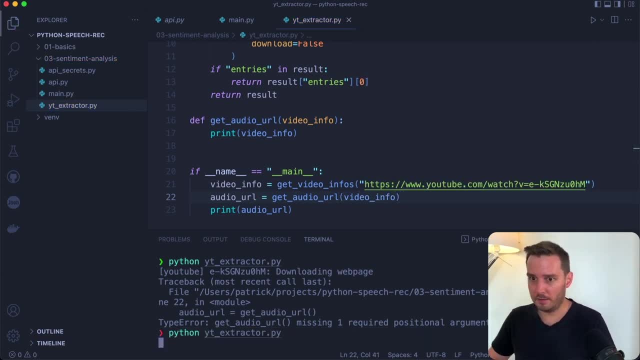 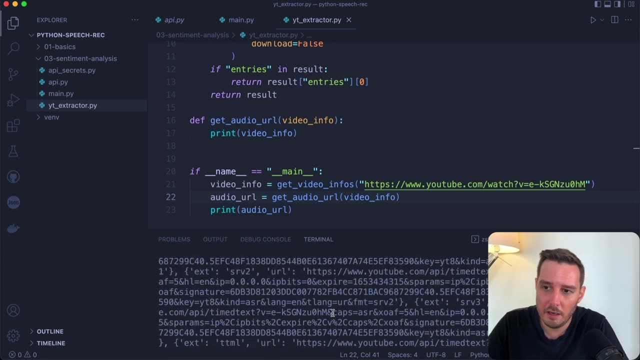 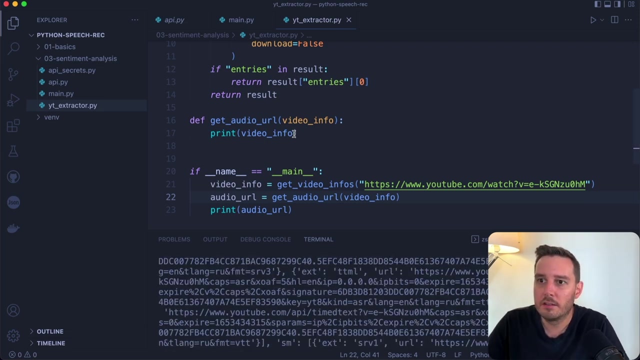 info And let's try this again. And yeah, so here it extracts the whole, or it printed the whole info. So this is actually a very long object, a very long dictionary. So I can tell you that this has a key in it. 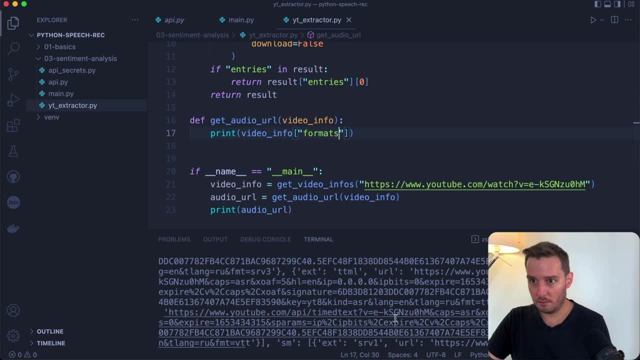 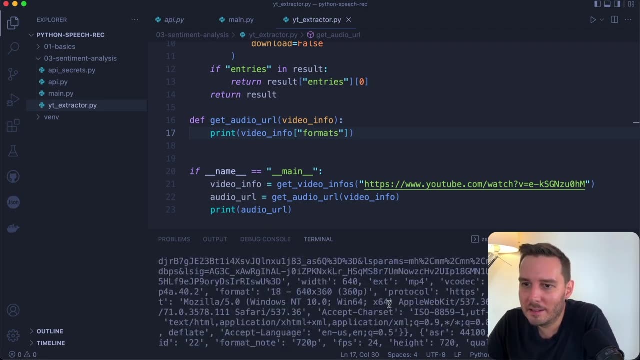 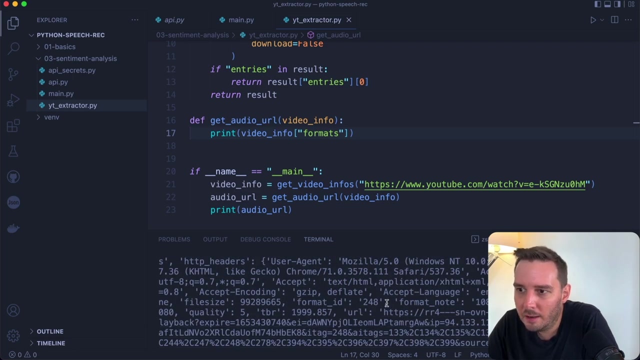 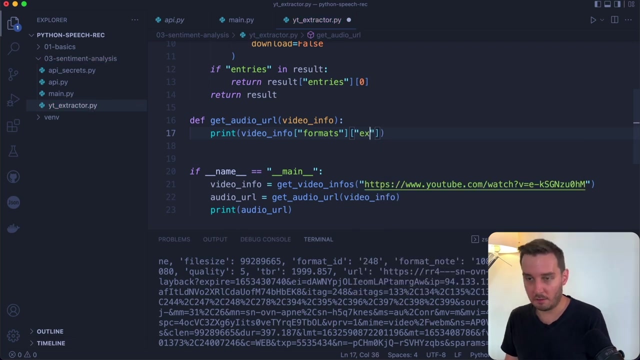 that is called formats. So let's actually print only the formats, And if we run this, then this is also still a very large, very large dictionary. But then again, this is an inner dictionary And this has a key that is called, or actually, this is a list, So now we can iterate over. 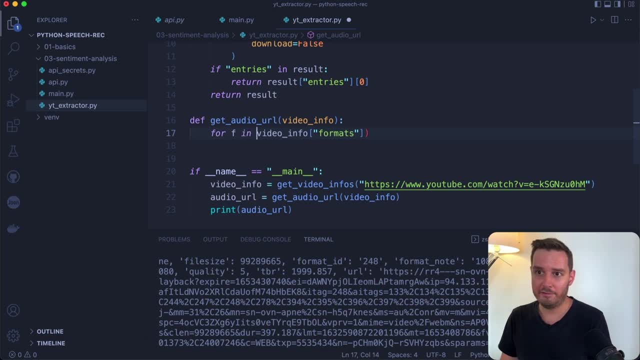 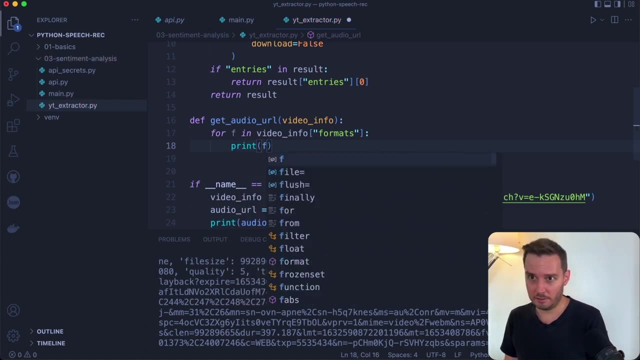 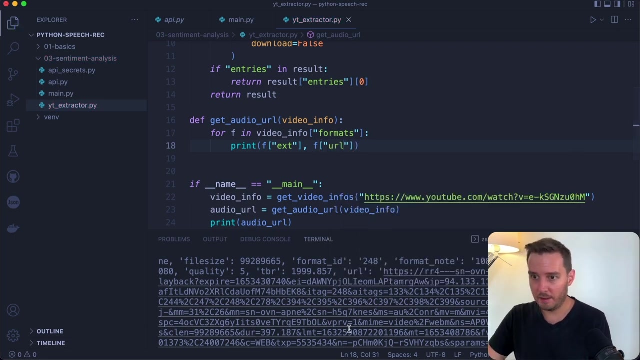 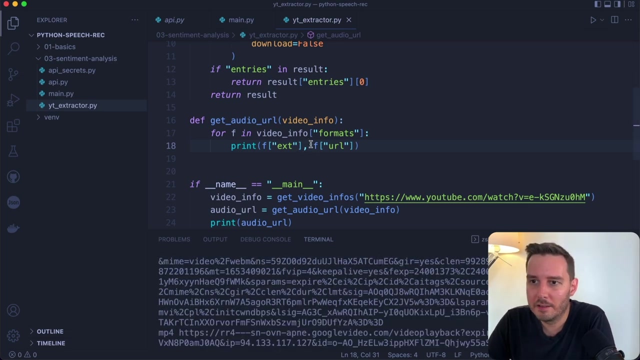 this. So here we say for F in video info formats and then we can print the f. let's print f dots And it has the key x for extension And it also has a URL. So we also want to print f dot URL. And now if we run this, then let's see what happens. Let's actually comment. 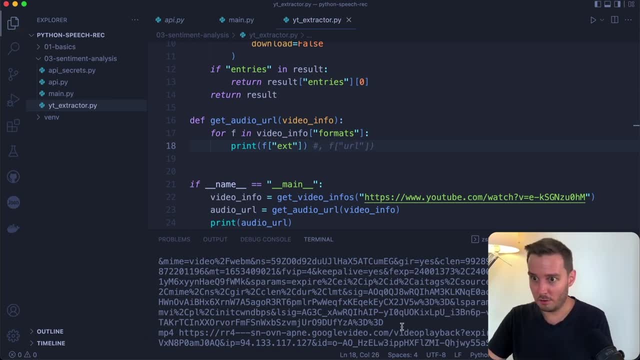 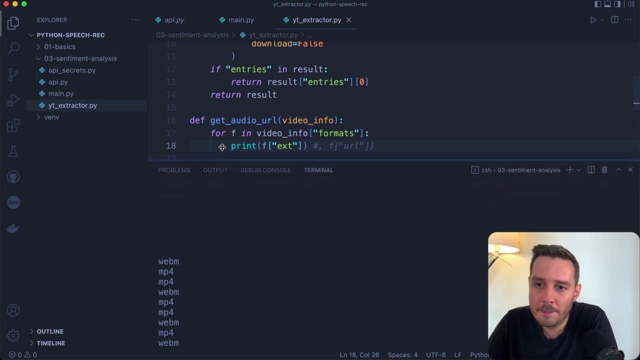 out the URL, because this is super long. So let's print only the extension. And now we see we have a lot of different extensions, because it actually start the video in a lot of different formats And with a lot of different resolutions and so on. So what we want is this one. So the m for a 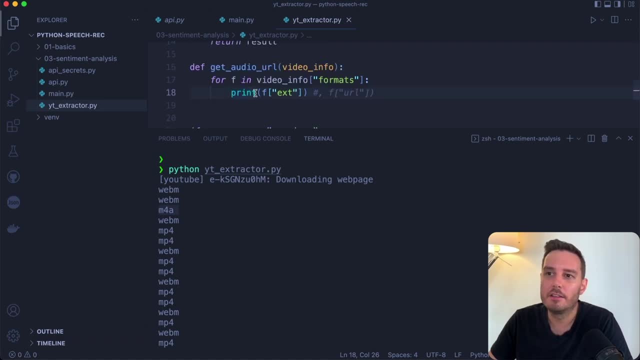 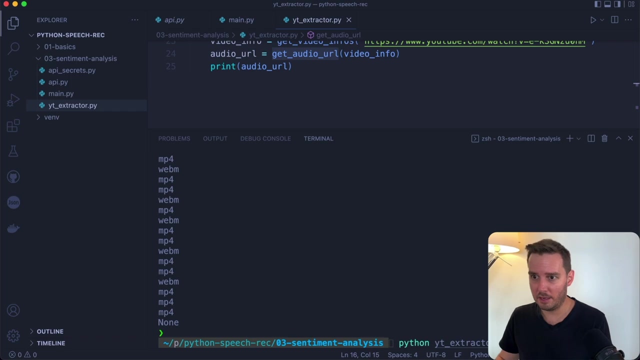 this is a audio format ending. So we now check if the format, if the extension equals, equals m for a, then we return the f URL key. So this is the audio URL And if we save this and then print this at the very end, 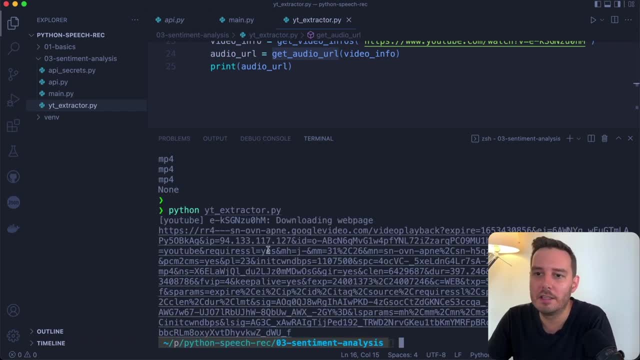 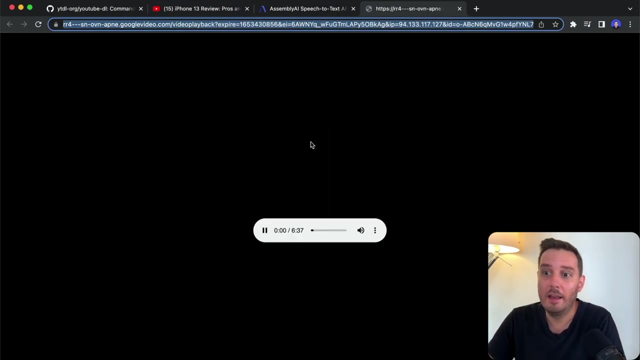 then we should get the URL to this hosted file So you can see this is at this URL. So this is not related to youtubecom. So now let's, for example, click on this And then we have this in our browser so we could listen to the audio file. 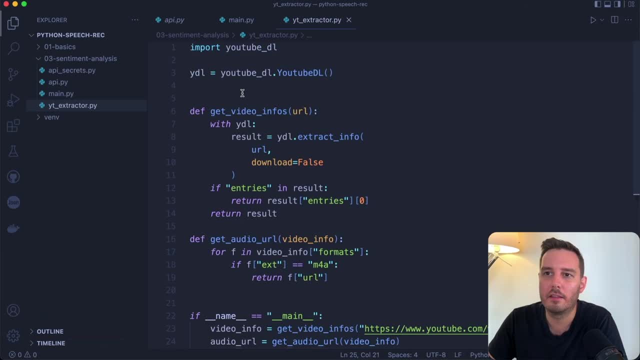 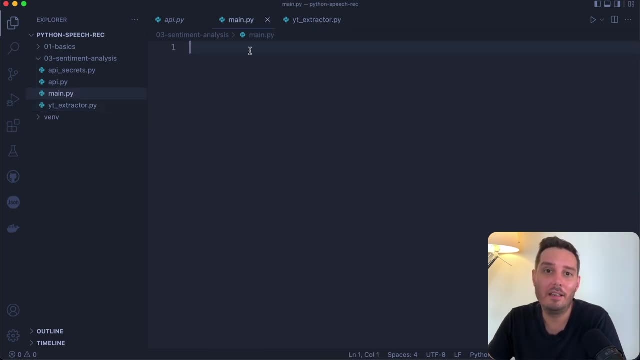 So yeah, this is the first part: how to work with the YouTube DL package to extract the infos. And now let's combine this in the mainpy. So in mainpy we combine the YouTube extractor infos with assembly AI and extract the transcript of the video and also the sentiment classification. 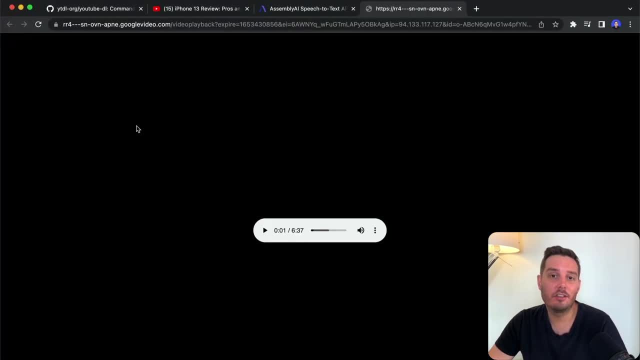 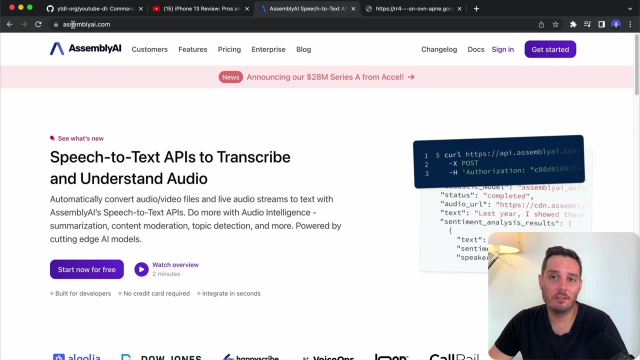 results. So sentiment classification is usually a pretty difficult task, but assembly AI makes it super simple to apply this. So if we go to the website assemblyaicom and have a look at the features, then we see they provide core transcription. So this is basically. 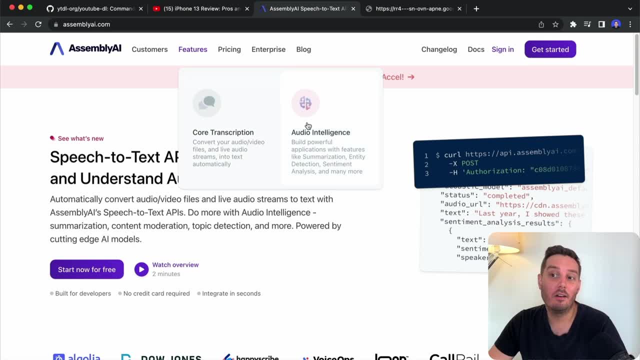 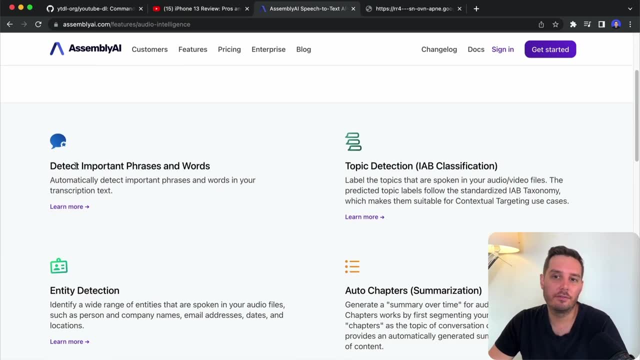 the speech recognition we've seen in the last part, But they also offer audio intelligence features and they are pretty cool. So there are a lot of features you can use. for example, detect important phrases and words, topic detection, auto chapters. so auto summary. 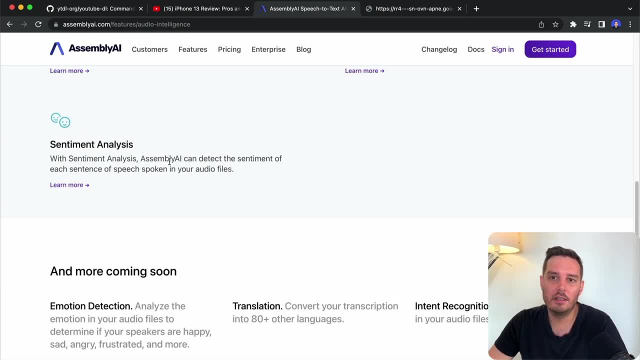 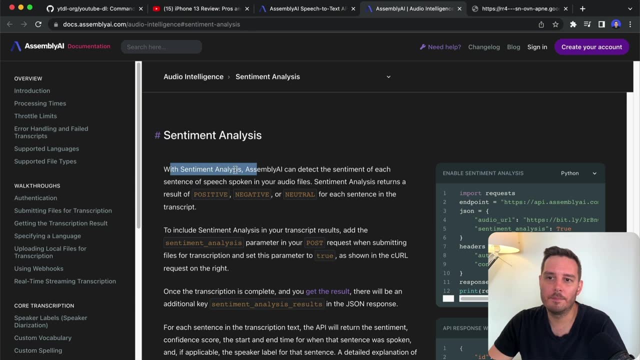 summaries and much more. And if we scroll down then here we find sentiment analysis. So if we click on this then we see a short description. So with sentiment analysis, assembly AI can detect the sentiment of each sentence of speech spoken in your audio files. 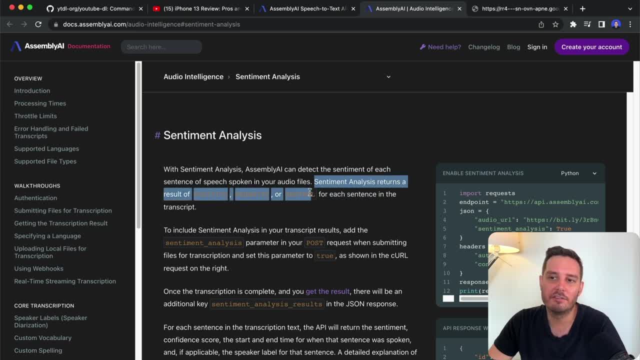 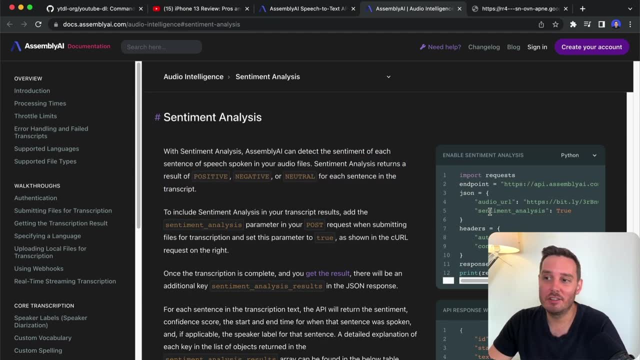 Sentiment analysis returns a result of positive, negative or neutral for each sentence in the transcript. So this is exactly what we need here, And it's actually super, super simple to use this. So the only thing we have to change is when we call the transcript. 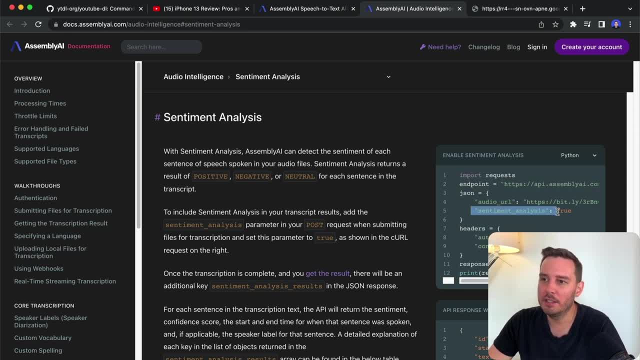 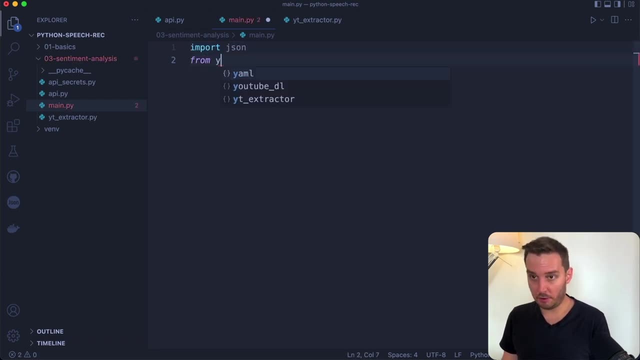 endpoint. we also have to send sentiment analysis. equals true as JSON data. So this is all we need to do. So let's go to our code and implement this. So let's import all the files we need. So we want JSON. then we say: from YouTube extractor, we import, get audio URL and get video info. 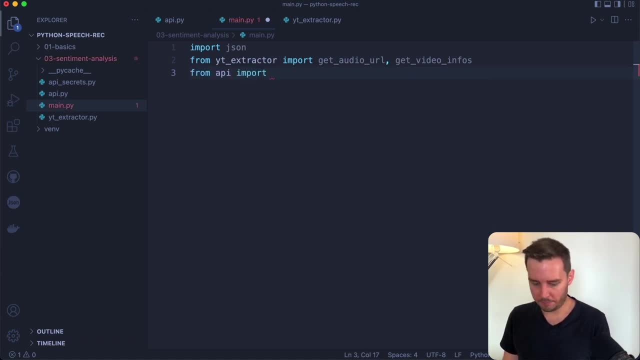 And from our API helper file we import save transcripts. then here I create one helper function that I call save video sentiments And this gets the URL, And here we get the video infos by calling: get video infos with the URL. then we get the audio URL by calling. 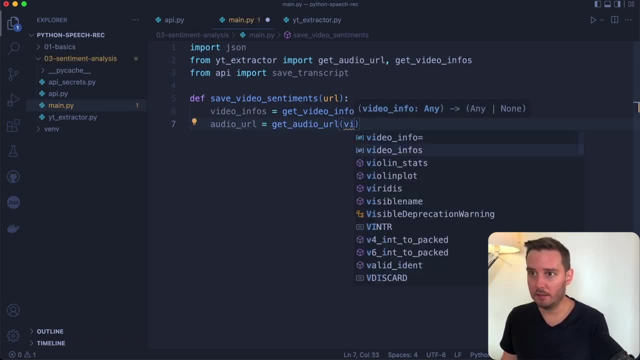 get audio your l, and this gets the video infos. And then I simply call the Save transcript function and this gets the audio URL And it also gets eight title And for the title I want to use the title of the video, so we can get this from the video. 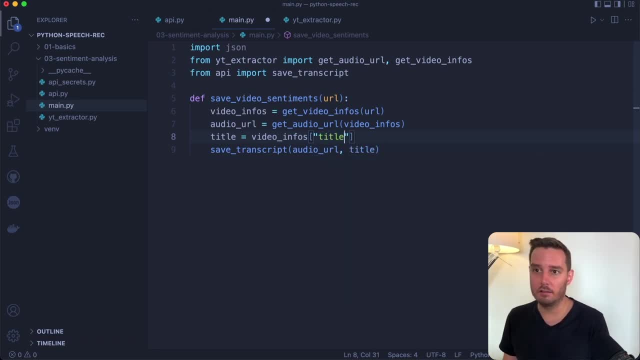 infos. So this has a key that is called title. And then I want to slightly modify this. So I say title equals title dot strip. So I want to remove all leading and trailing whitespace, And then I want to replace all spaces with a underscore. And then I also say: 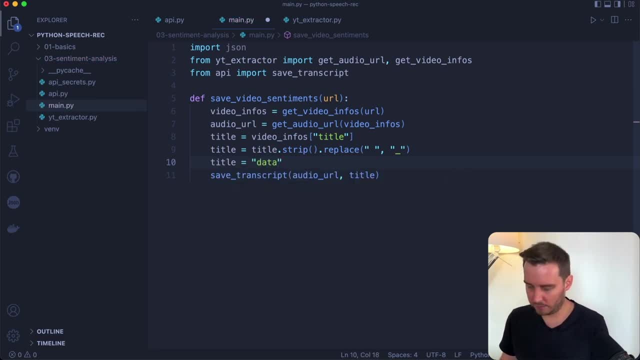 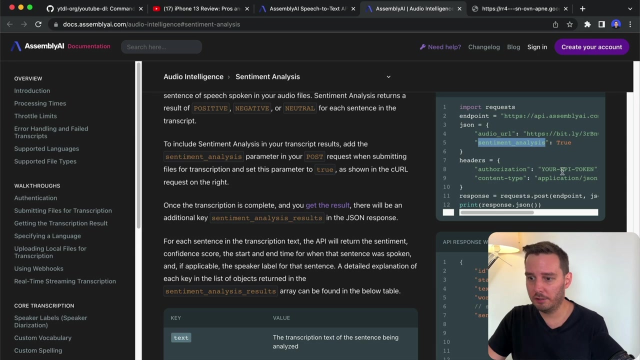 title equals data slash plus title, So I want to store this in a separate folder. So here we create this and call this data, And now we have to modify this slightly. So if we have a look back then we see this needs the additional argument: sentiment analysis. And now so in. 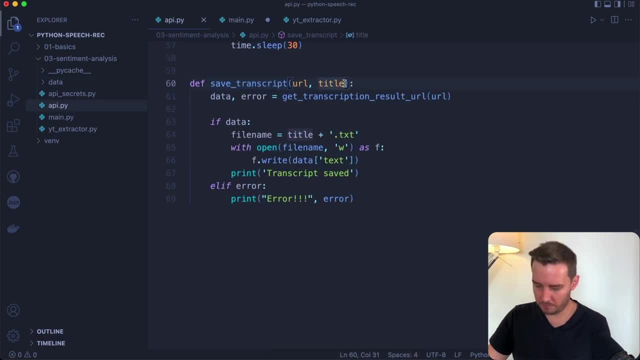 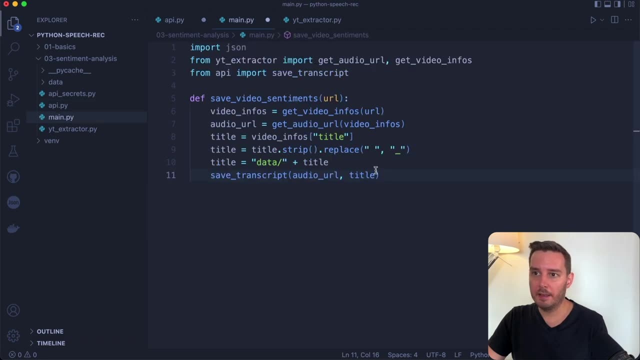 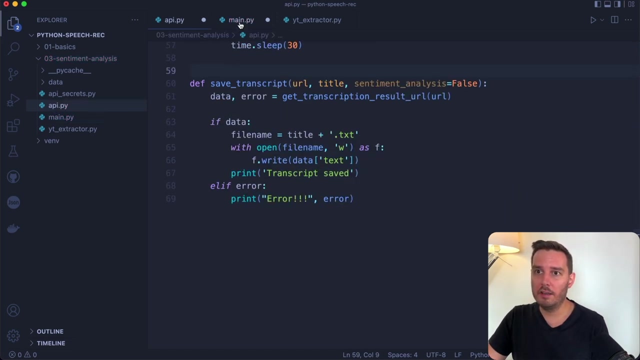 the safe transcript file. I will put this as additional argument And I will give this a default of false. And then here we say: sentiment analysis equals true, And now we have to pass this through. So we have to pass this to the get transcription result URL. So this also needs this parameter. 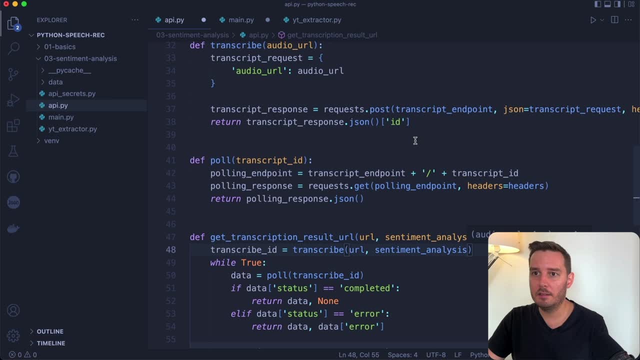 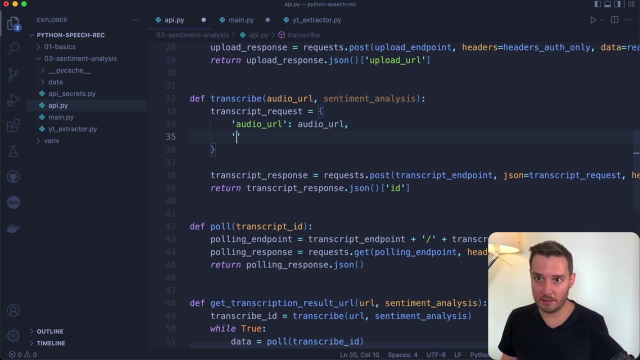 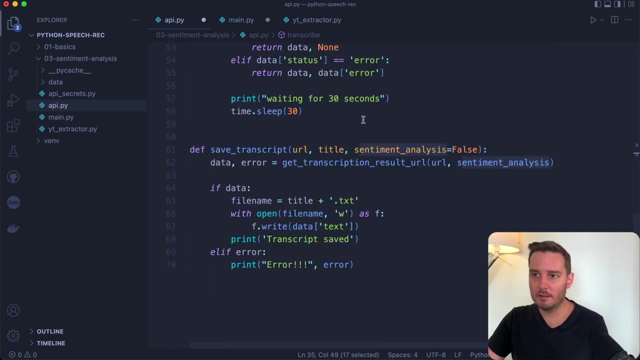 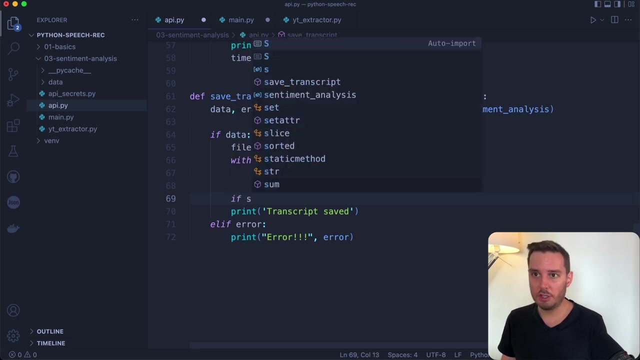 Then the transcribe needs the parameter, And here this needs the parameter, And now, as a JSON data that we sent, we put sentiment analysis equals true or false, And this is all that we need, And now, of course, I also want to save this. So here we check If the parameter is true. 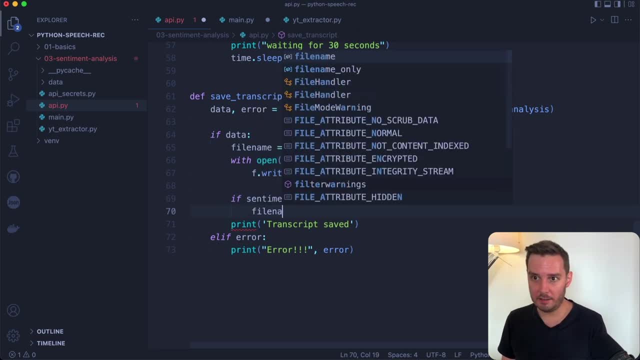 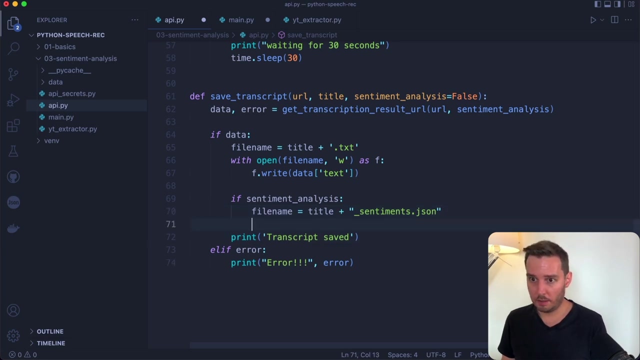 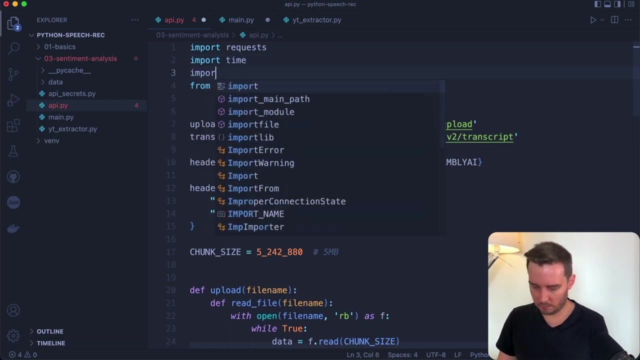 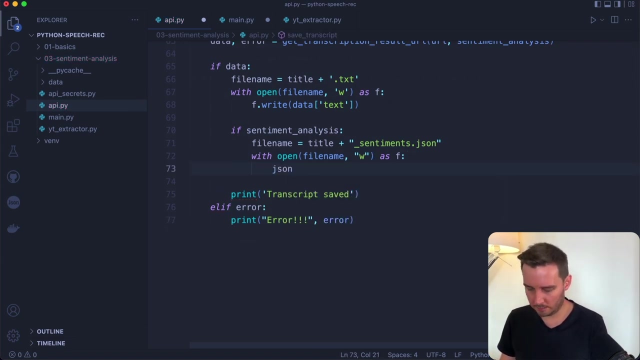 then I create a separate file. So again I say file name equals title plus. and then let's call this underscore sent to man's dot JSON. And now I say with with, open the file name in write mode as F, and then I import Jason in the top import JSON. And then here we simply say Jason, DOTS. 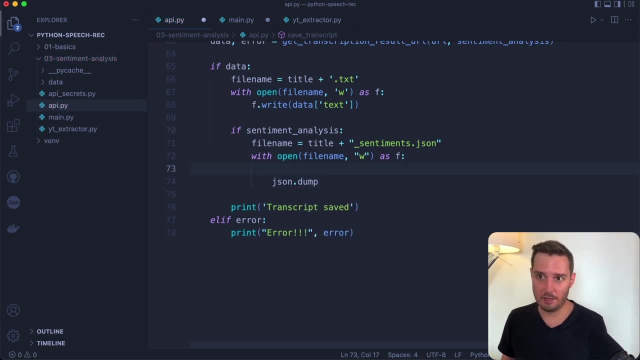 dump, And first we have to extract the infos, of course. so we call this: sentiments equals data, And then the key. If we have a look at the documentation, then here we see the JSON, which is essentially the type of data we want to import. So now we know the data. 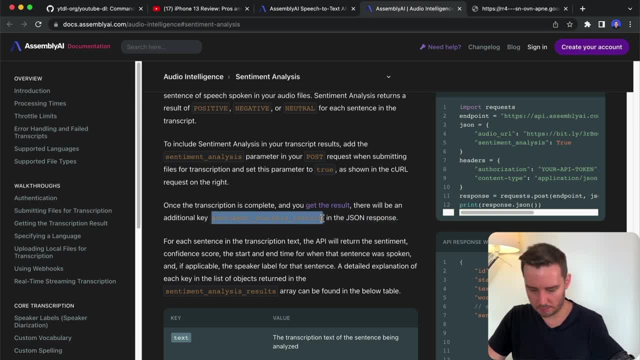 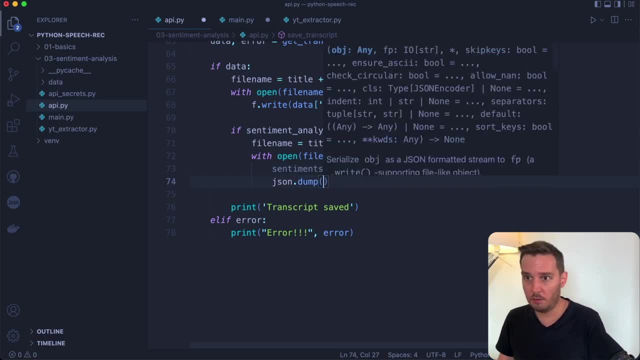 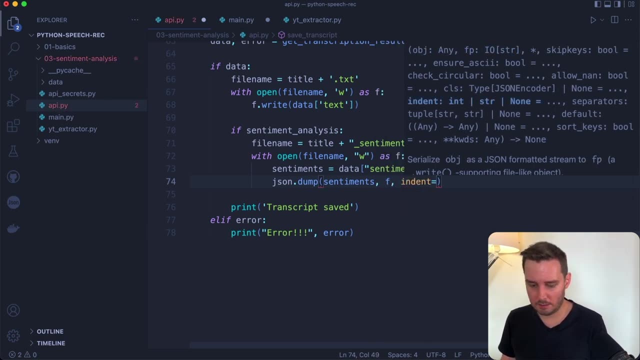 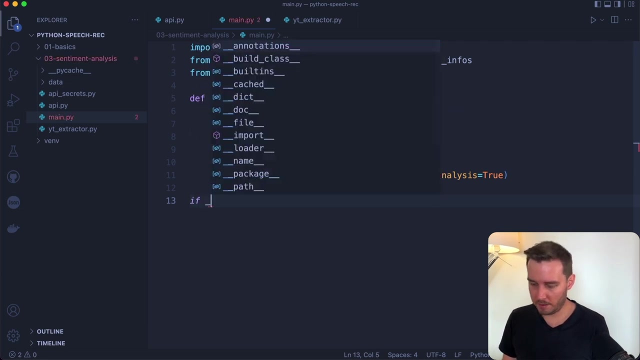 JSON response now has this additional key sentiment analysis results. So we use this and then we dump the sentiments into the file. And I also want to say indent equals four to make this a little bit more readable. And now in the main, dot pi, we call the function. 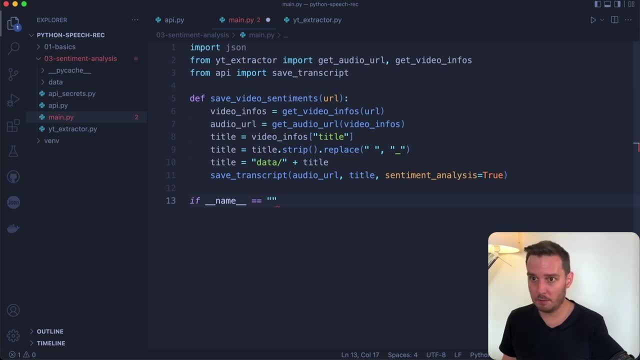 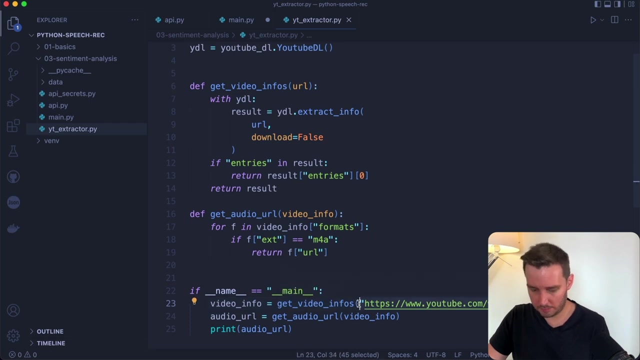 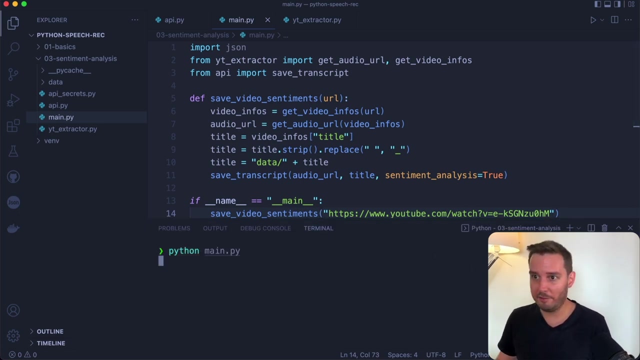 and say: if underscore name equals, equals underscore main, and then I want to call the safe video sentiments, And the URL is this one. So let's copy and paste this in here. And now let's run the mainpi file and hope that everything works. So the website is downloaded. 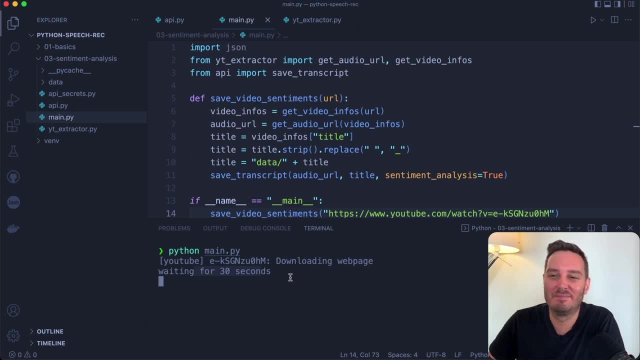 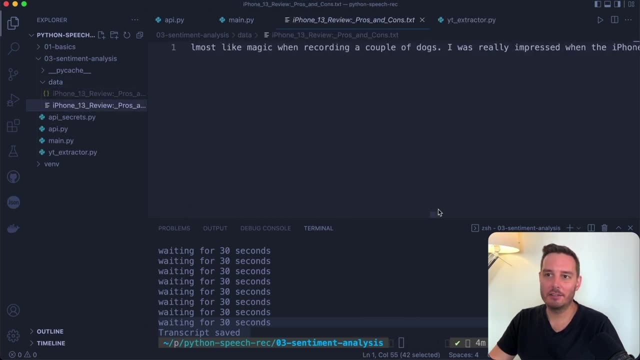 and transcription starts. So this looks good. So let's wait. Alright, so this was successful and the transcript was saved And now we have a look at the data folder. then here we get the transcript of the video And we also see our JSON file with all the sentiments. So for each, 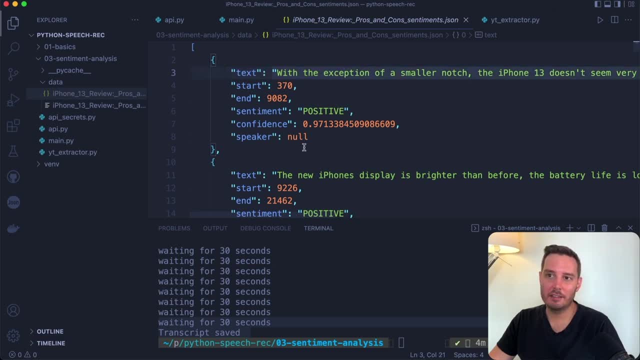 sentiment, we get the text of the sentence. So, for example, this one, with the exception of a smaller notch, the iPhone 13 doesn't seem very new at first glance, But when you start using this flagship you start to appreciate a bunch of welcome upgrades. then we get the start and end. 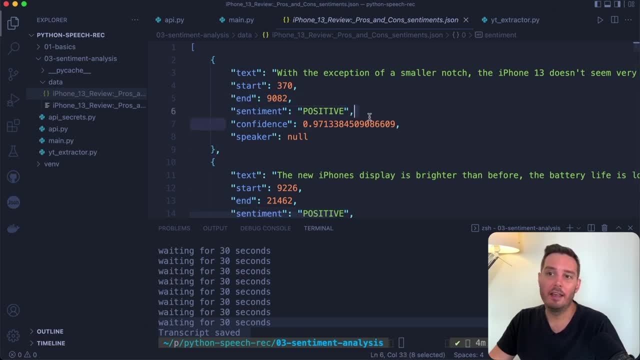 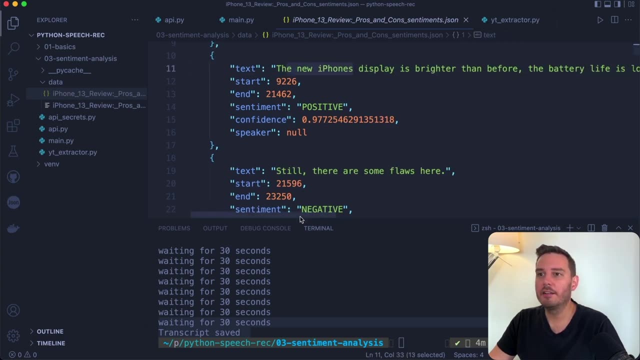 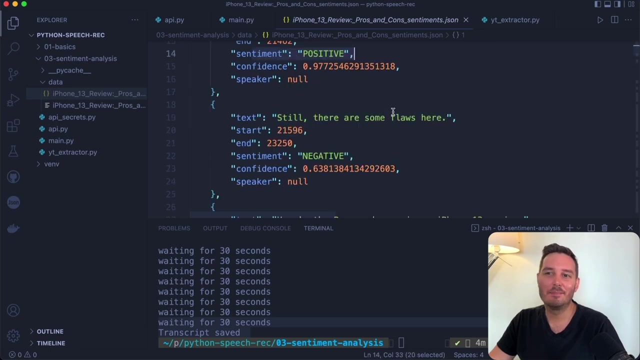 time. then we get the sentiment, which is positive, And we also get the confidence, which is pretty high. Then the next example: the new iPhone display is brighter than before, the battery life is longer and Apple has improved blah, blah, blah. So here also the sentiment is positive. 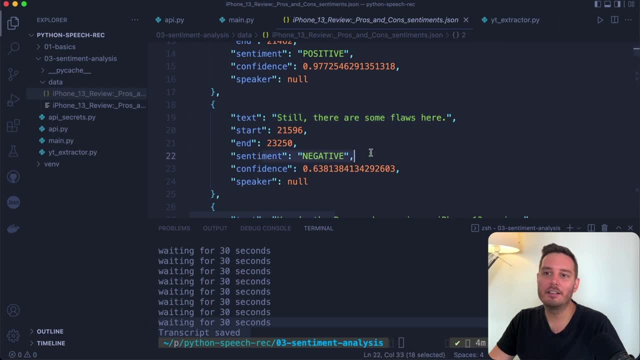 then we have: still there are some flaws here And now the sentiment is negative, So this works better than before. So here also the sentiment is positive. then we have: still there are some flaws here and now the sentiment is negative, So this works. 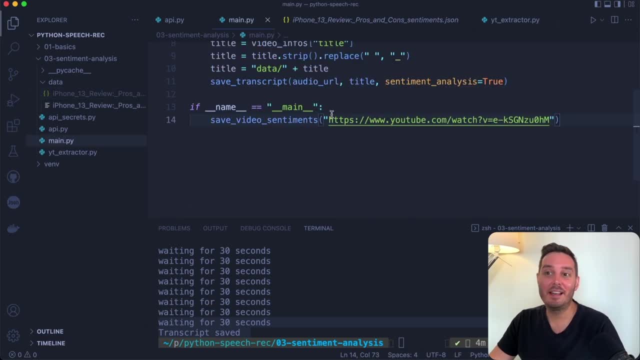 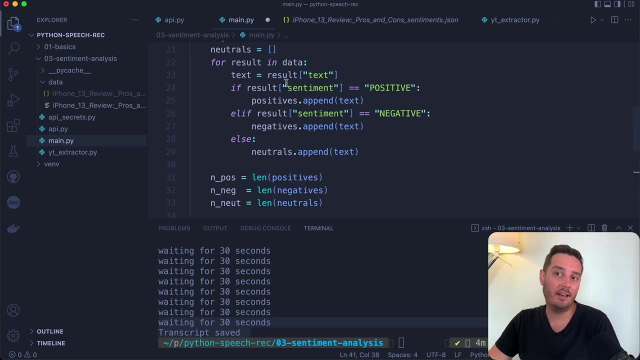 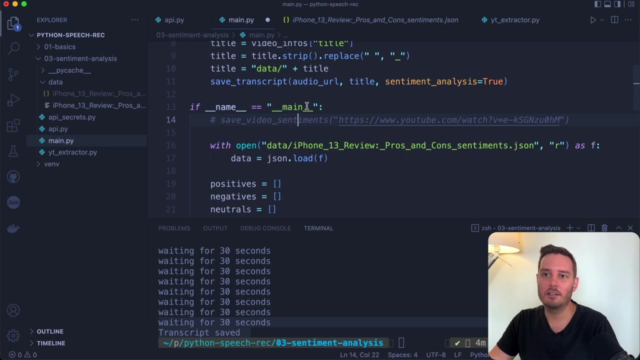 pretty well And, yeah, this is how you can apply sentiment analysis with assembly AI. Now I want to show you a little bit more code, how we could analyze this, for example. So now we can comment this out, So we don't need to download this again. then we can read our JSON file And: 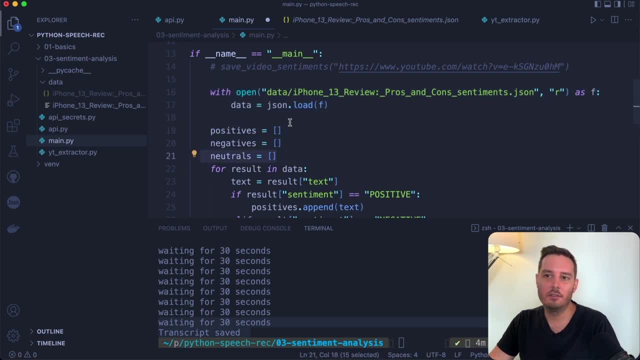 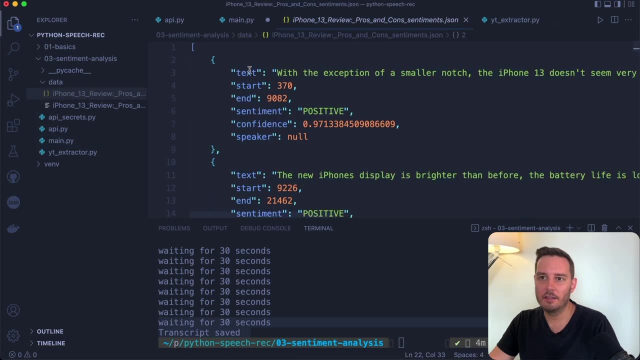 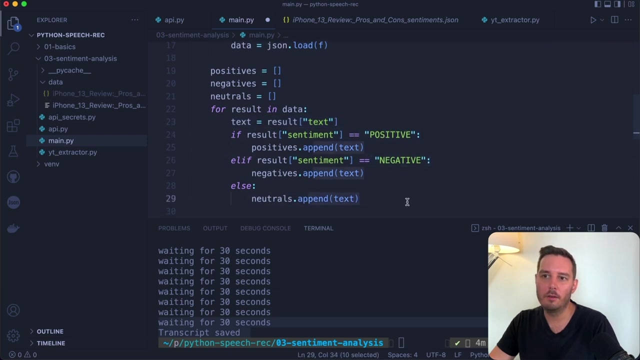 here we start: the positives, negatives and neutrals, So we iterate over the data And then we extract the text. so the text and we also extract the sentiment. So then we check if this is positive, negative or neutral and append it to the corresponding list. 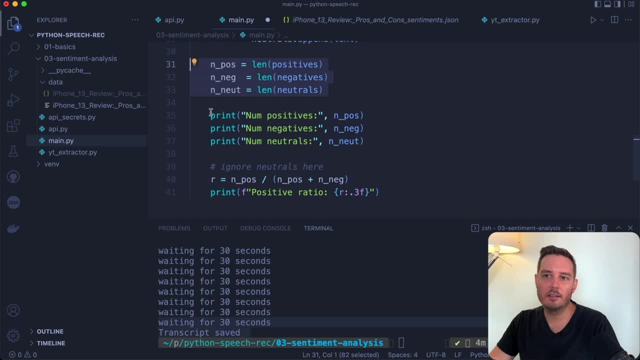 then we can calculate the length of each list And then we can print the number of positives, negatives and neutrals, And we can also, for example, calculate the positive ratio. So here we ignore the neutrals and simply do the number of positives divided by the number of. 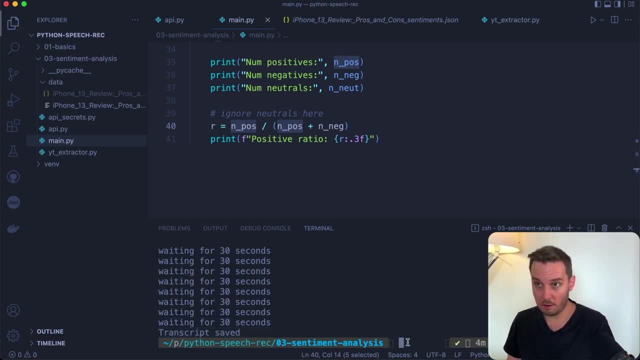 positives plus the number of negatives. And now if we save this and run this again, then here we get the number of positives, So 38, only four negatives. overall positive ratio is 90%. So with this you can get a pretty quick overview of a review, for example. 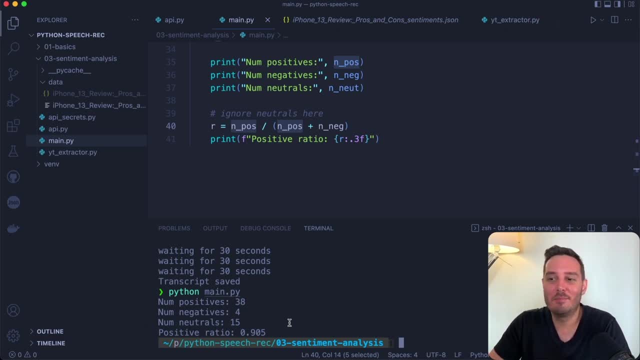 And, yeah, I think the sentiment classification feature can be applied to so many different use cases. It's so cool. So, yeah, I hope you really enjoyed this project. and now what would be really cool is if we could display this information in a nice looking. 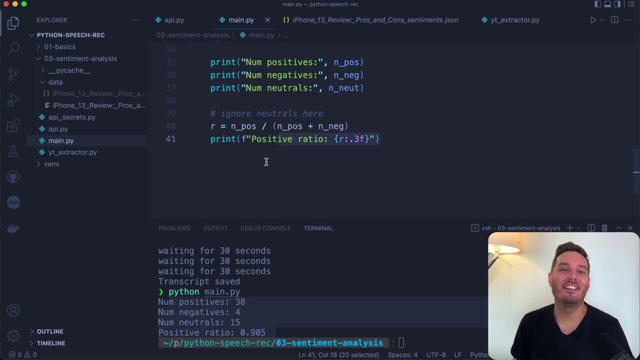 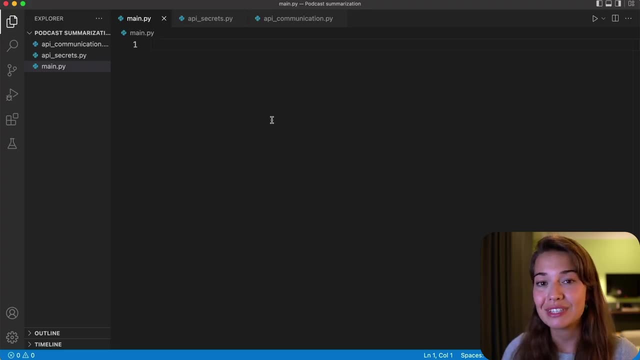 web app, And this is actually one thing that you will learn in the next tutorial, together with Misra. So let's move on to the next project. All right, now it's time to build a podcast summarization app, And we're also going to build a web interface for this application In this. 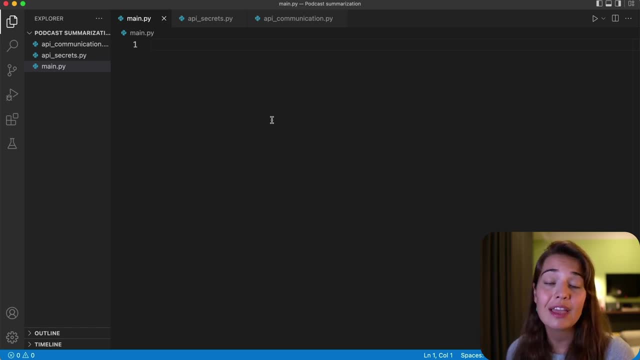 project. we are again going to use assembly AI's API that offers the chapterization, summarization features, And we are going to get the podcast from the listen notes API, So let's get into it. Here's what our app is going to look like once we. 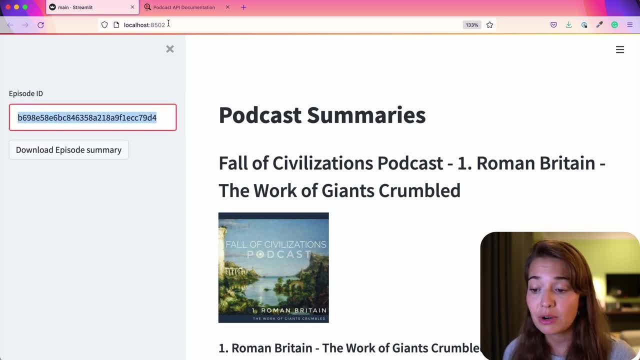 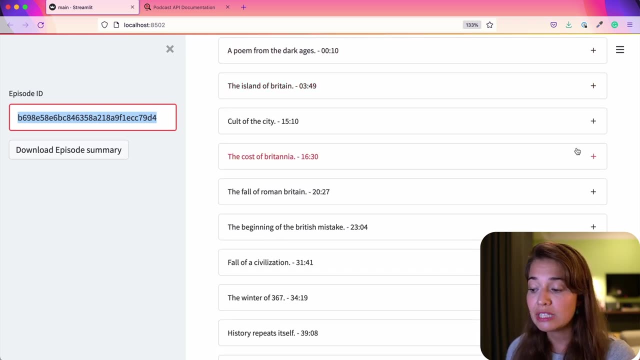 are done with it. So we will get a episode ID from listen notes API. I will show you how to do that, And when we click this button, it will give us first the title of the podcast and an image, the name of the episode, and then we will be able to see different chapters and when they start in. 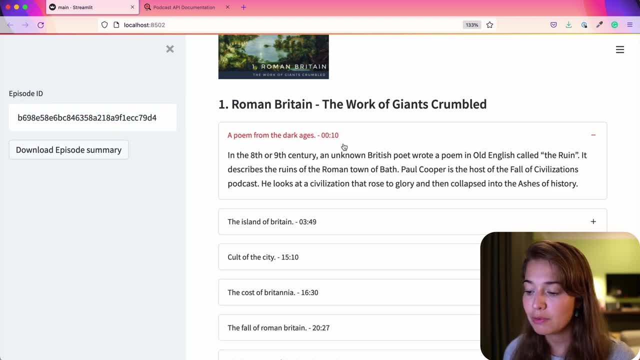 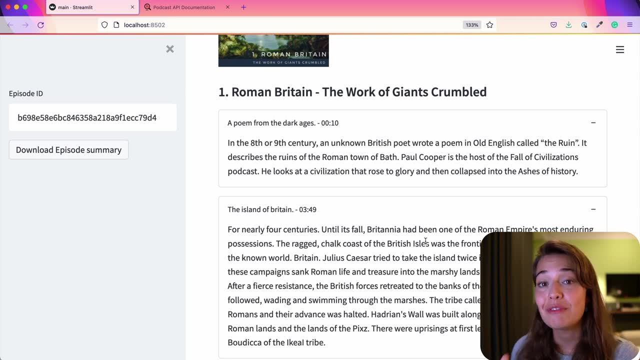 this episode, And if we click these expanders, we will be able to read a summary of the chapter of this episode. This is all quite exciting: to start building a web front end for our application too, So let's start building it So in this project. 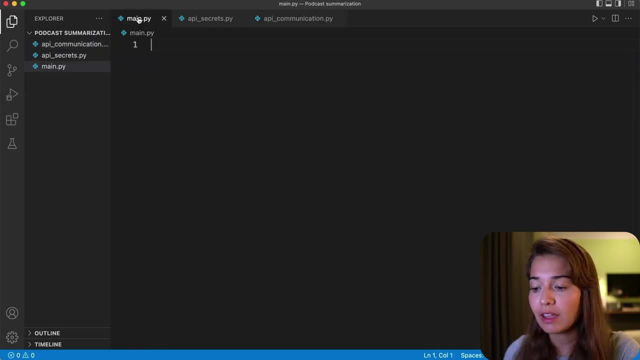 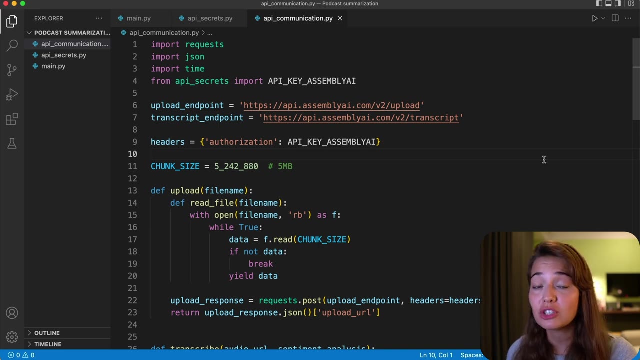 like in the previous ones, we are going to have a main script And we're going to have a supporting script- API communication- where we have all of our supporting functions that we want to use over and over again. We built this before, So this is the exact same one from the third project, the project. 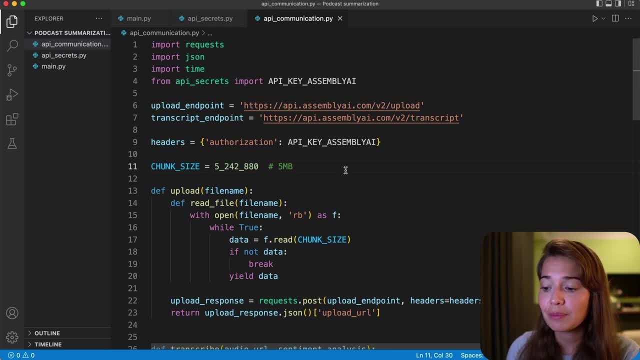 that we created And we will only need to update this and change some things to start doing podcast summarization. But the first thing that I want to update here is that we will not actually need the upload endpoint anymore, So I'm just going to go ahead and delete that one, because the transcripts 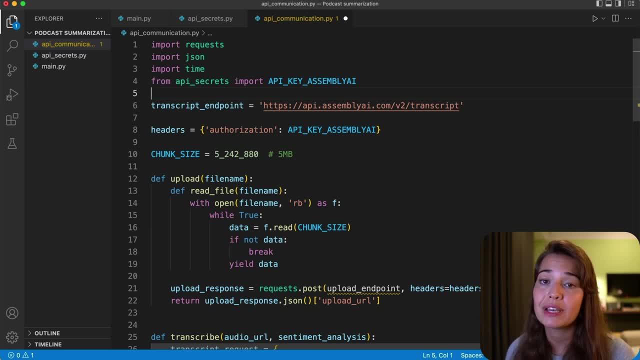 are going to be, or sorry, the podcasts are going to be received from the listen notes API, So it's going to be somewhere on the internet. we will not download them to our own computer, So we can immediately tell assembly AI. hey, here's the audio file, here is the. 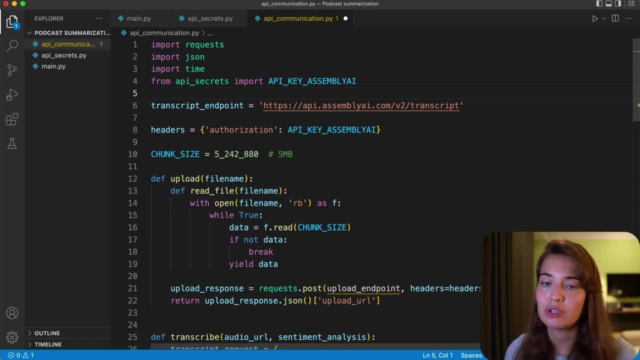 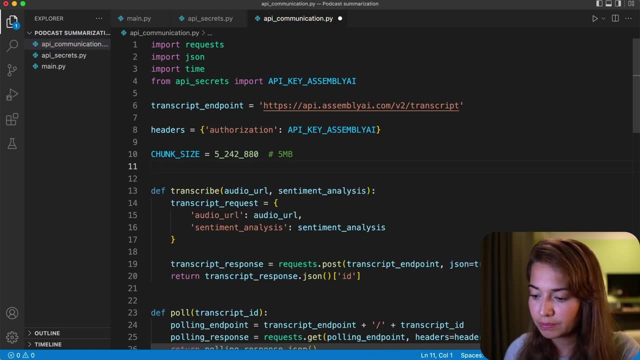 address of the audio file that I want you to transcribe, and it will be able to do that, so there will be no download or upload needed. That's why I also don't need the upload function. Also, the chunk size not relevant anymore. Alright, so that's good for now, And the next thing that 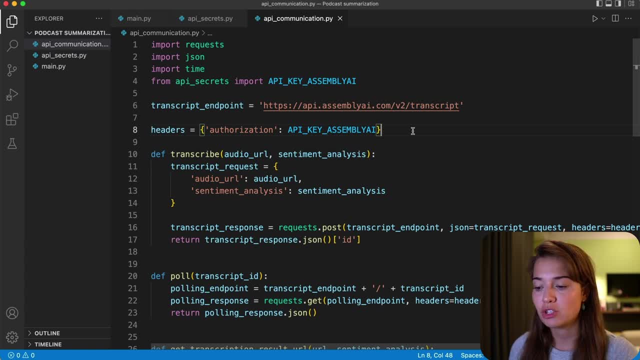 we want to do is to set up the Listen notes API communication. So we are going to use assembly AI to create the summaries of the podcasts and we will get these podcasts from listen notes. If you never heard of listening notes, then you know that I have a list of languages you don't get to know. 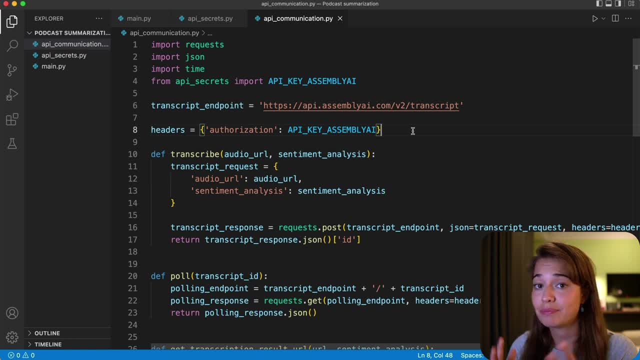 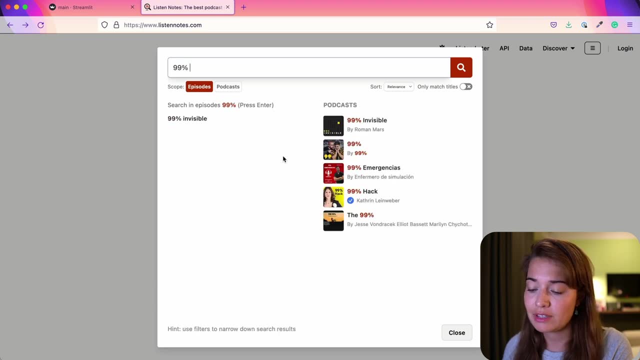 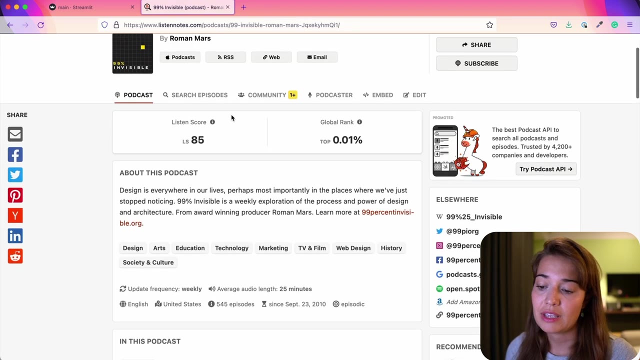 heard of it before. Listen Notes is basically a database of podcasts- I think nearly all of the podcasts- So you can search for any podcast. For example, one of my favorites is 99% Invisible And you will be able to get all of its information plus the episodes, So you can search for episodes. 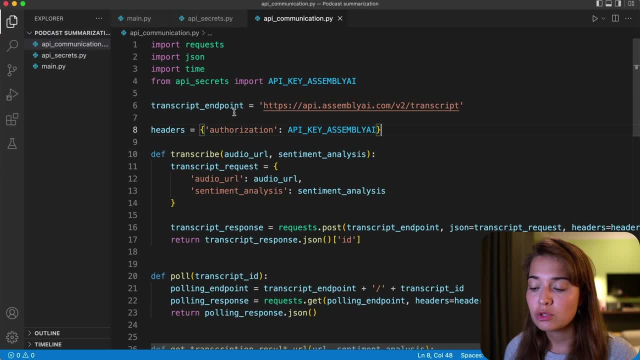 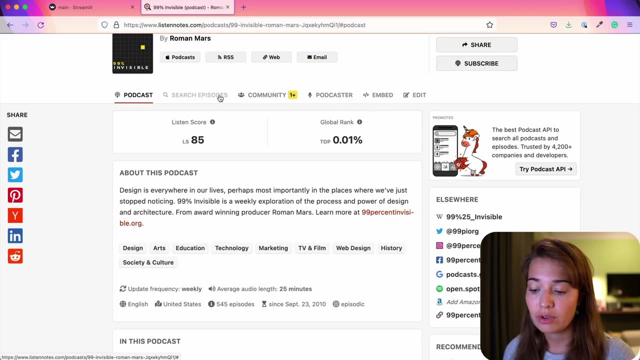 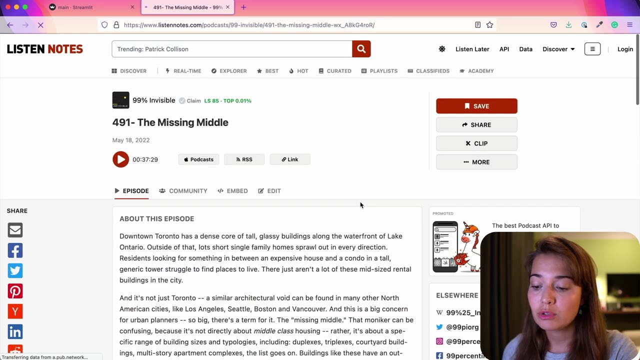 here, if you would like to. What we're going to do with Listen Notes is that we are going to send it a episode ID, like specific episode ID that we will find on the platform itself. So let's say, I want to get the latest episode of 99% Invisible If I go to the episode page and go. 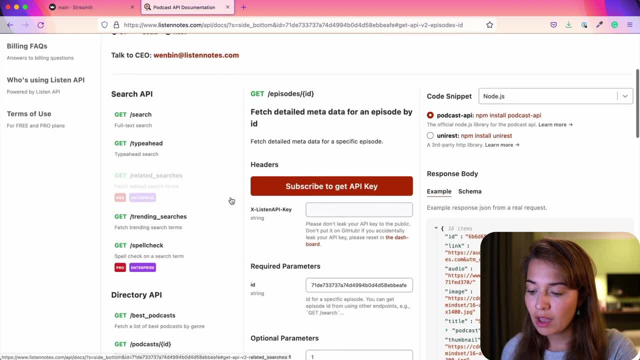 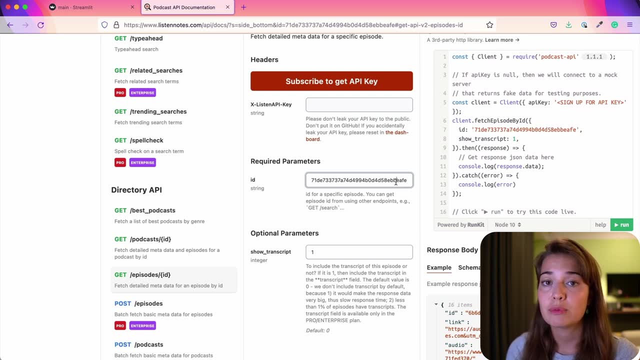 down to use API to fetch this episode, I will see a ID. So this is the ID of the specific ID of this episode And using this ID, I will be able to get this episode and send it to Assembly AI And this is exactly the ID that we are going to send it to. So I'm going to go down to the episode page and 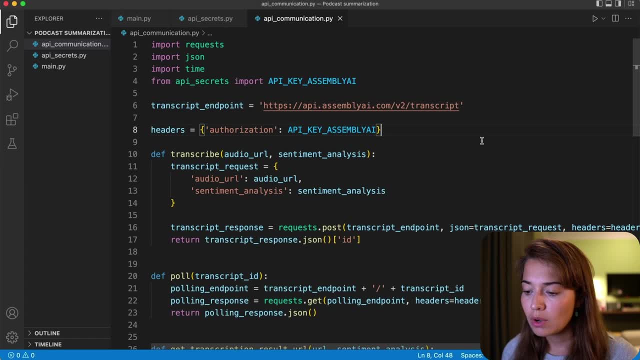 send it to Assembly AI And this is exactly the ID that we are going to send it to. So I'm going to need on our application. So to get that, first of course we need the ListenNotes endpoint. ListenNote has a bunch. 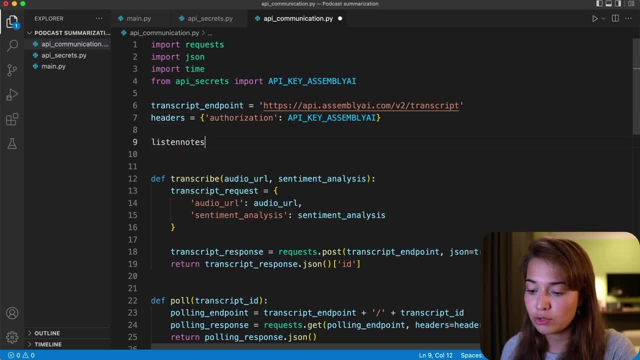 of different endpoints, But the one that we need is the episode endpoint to get the episode information. So I will just name this ListenNotes episode endpoint and it is this one, And of course we also need the header again to authenticate ourselves. 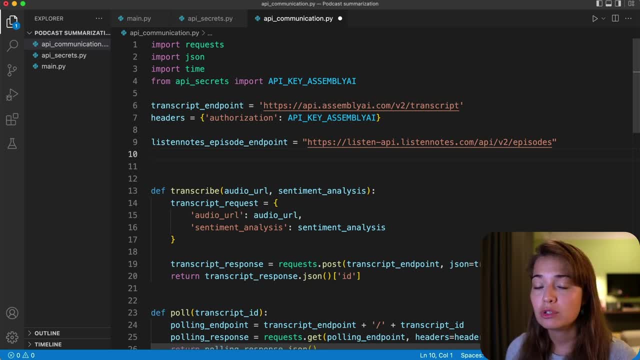 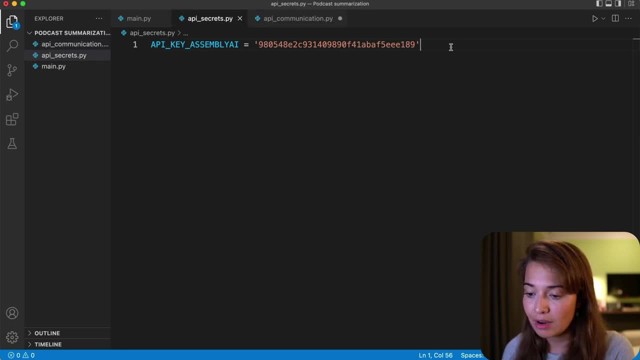 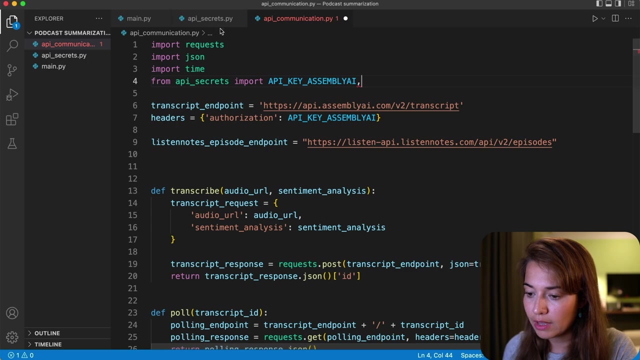 And in the header we're going to need to put a API key. So all you have to do is go to ListenNotes, create an account and get an API key for yourself, And we are going to go and paste it here And here, as you know, we are importing the API key for assembly AI. 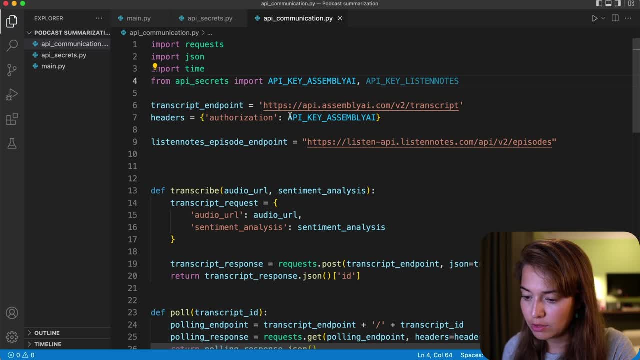 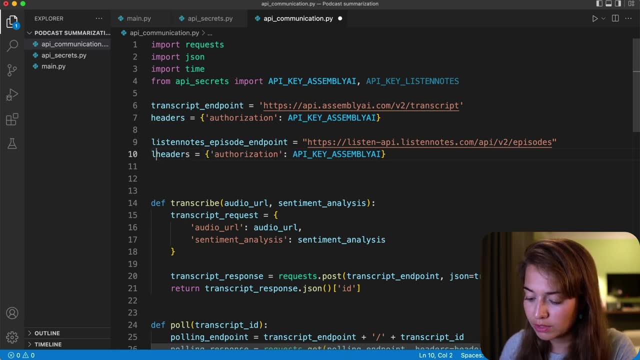 Now I'm also going to import the API key for ListenNotes And we are going to send it With our API key, Our requests to ListenNotes. So I will call this the ListenNotes headers And this is the assembly AI headers. 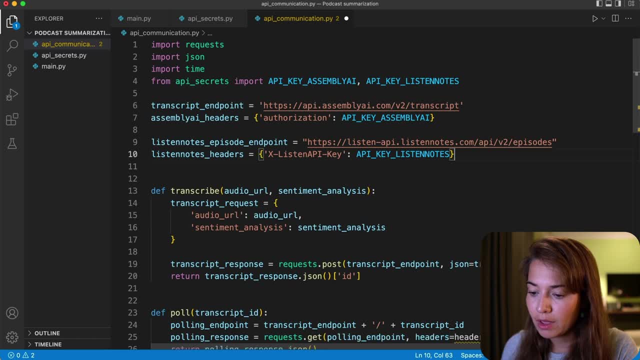 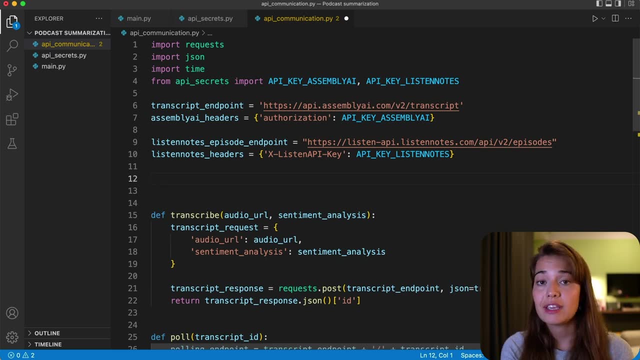 And for ListenNotes, this is named xListenAPI key. Alright, the first thing that I want to do is to build a new function that is able to get the episode ID and give us the URL to the podcast's audio file. So I will call this one. 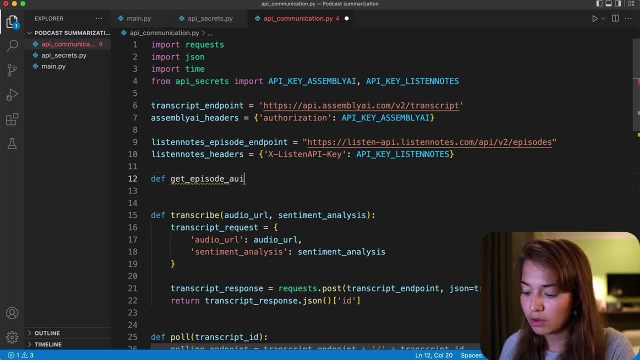 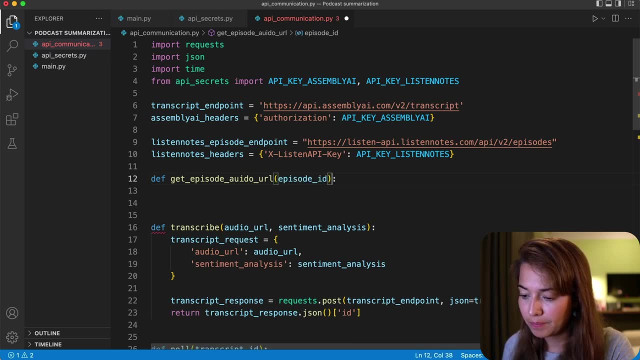 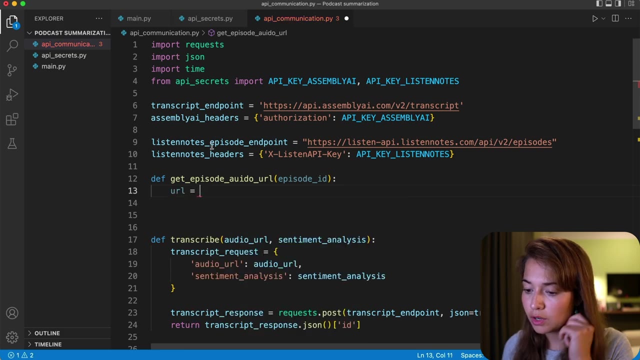 Get episode audio URL And it is going to get an episode ID And we're going to send a get request to ListenNotes. Let's build the URL first. The URL is going to consist of the ListenNotes episode endpoint and a dash plus the episode. 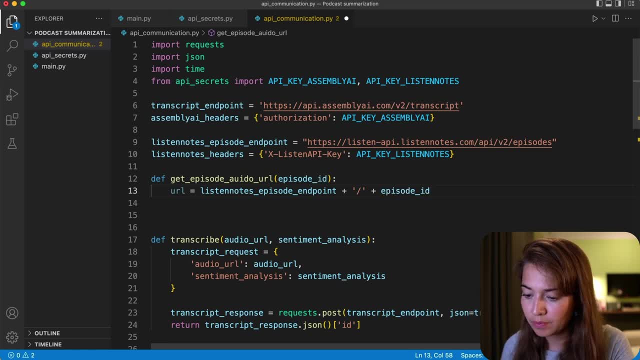 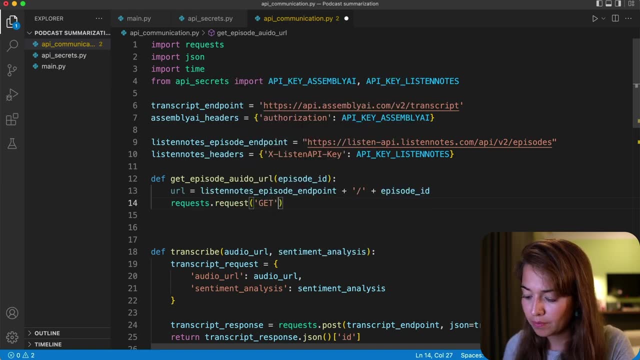 ID And we are going to send a get request to this URL. I will call the response. We get a response for now, And the last thing that we need, of course, is the headers for authentication, And that one is called ListenNotes headers. 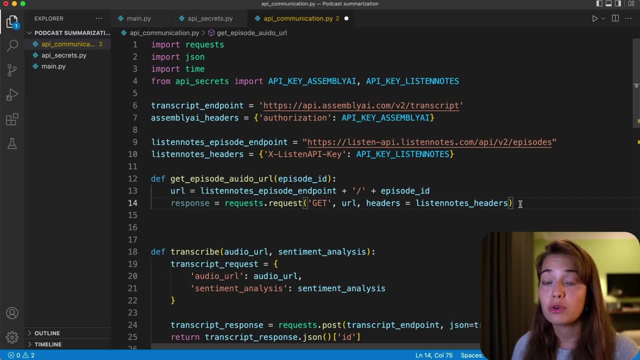 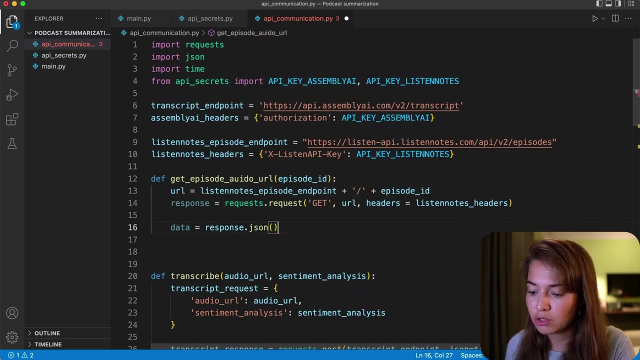 So after we do this, we should be able to get a URL for the episode ID, And the information is going to be sent in a JSON format, so this way we'll be able to see it. So maybe let's try this at first and see that it works. 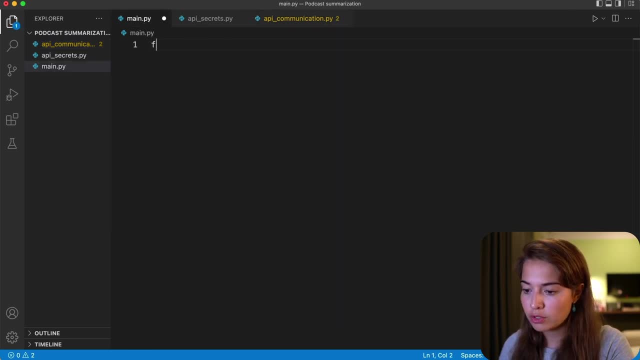 So to do that, I am just going to again import from API communications, import everything. I'll just make this a simple Python script for now And I'm going to call get episode audio URL And I will use the episode ID that I found here. 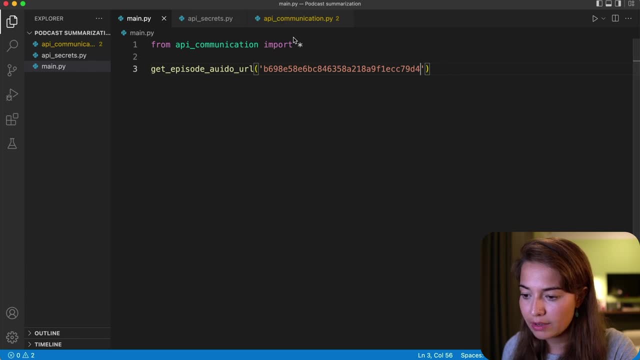 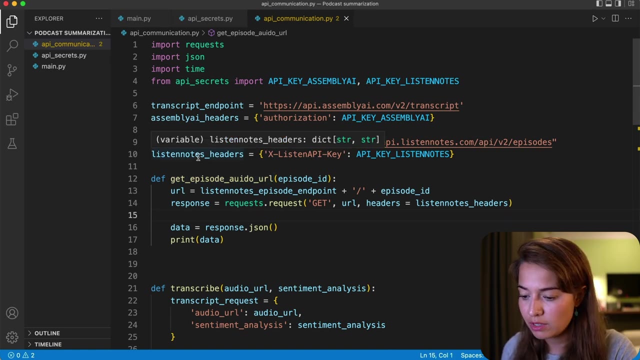 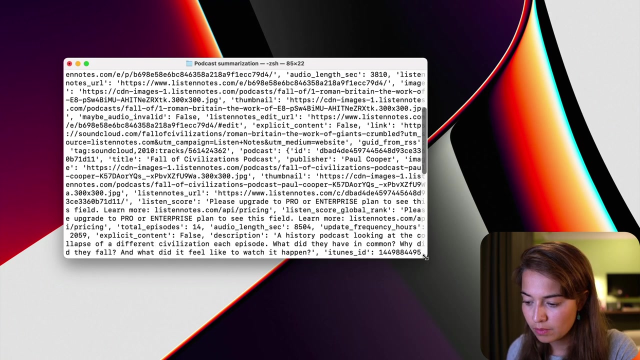 This one is to keep things simple And, as a result, we will print the response that we get from listen notes, So let's run this and see what happens. All right, this is really long, So maybe I will use a pretty print. 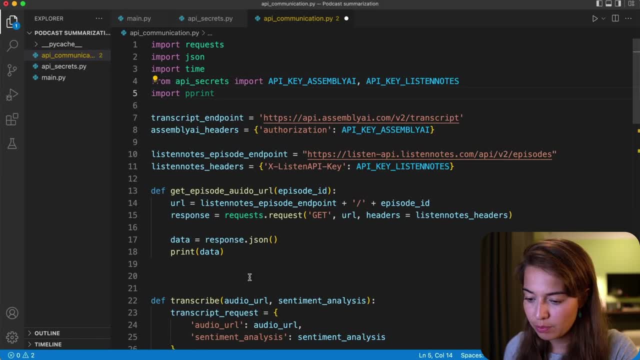 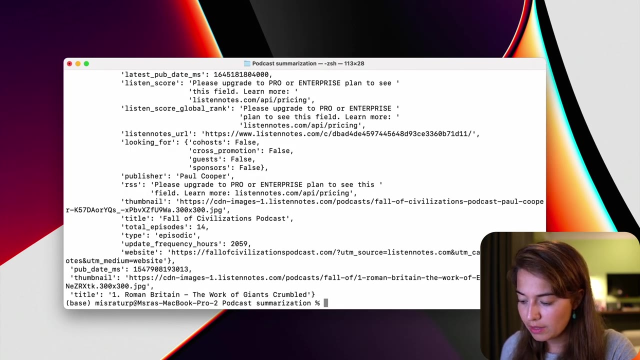 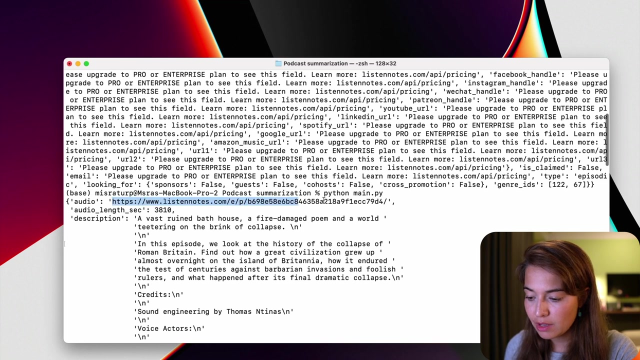 To make it more readable. So this pretty print here, And instead of this, just use pretty print. Okay, let's do it again. All right, that is slightly better. Let's see what kind of information we are working with. Nice, we get the audio URL here. 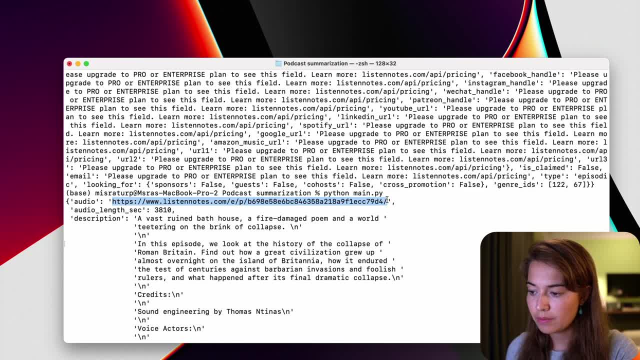 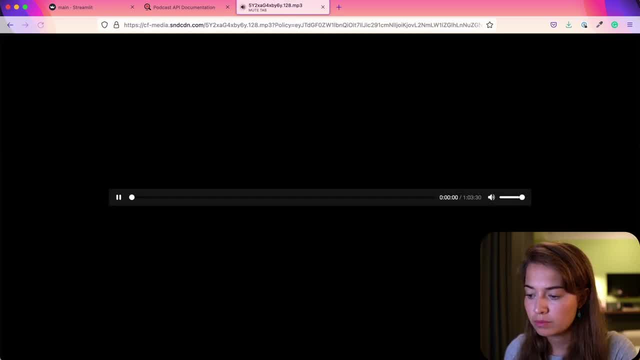 This is the URL of the audio. Let's see where that takes us. Yeah, this is just the audio of this podcast. You can hear it. VeroCity, that the Roman advance was halted. Nice, All right. So this is exactly what we need. 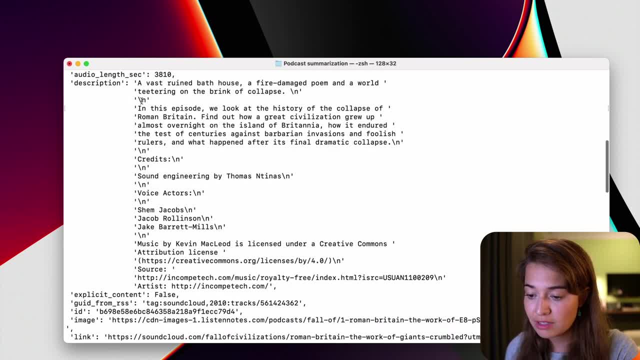 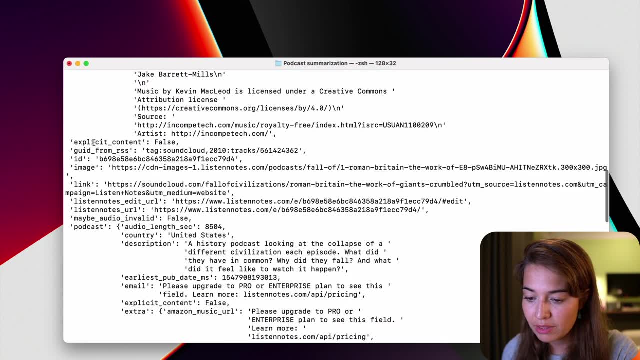 But if you want, you can also get some extra information about the podcast. If you want to display it in some way, we will definitely display it. This is a description of the episode, Whether there is explicit content or not. the image of this episode and some extra information. 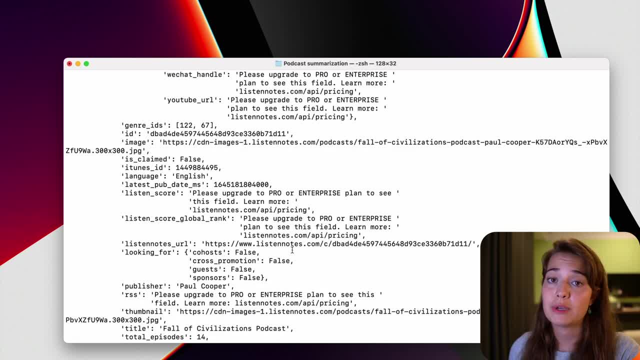 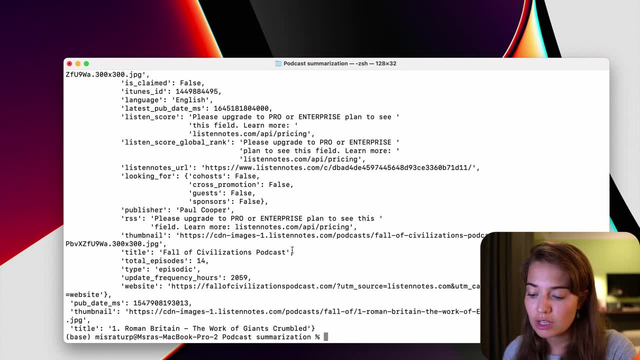 about the podcast. like Facebook handle, Google handle, et cetera, So you get a lot of information. So if you want to make your web application and your interface even more interesting, more interactive, you can, of course, include more of this in your application. 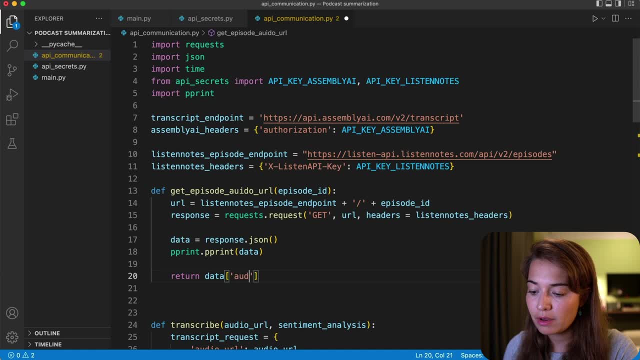 So if we just return data audio from here, we will actually just return the audio URL. But you know, now that we have all this information might as well extract some more of it. So some of the things that we can get as a thumbnail of this episode. name of the podcast. 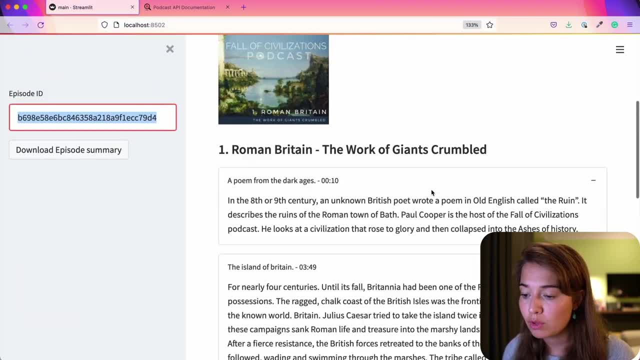 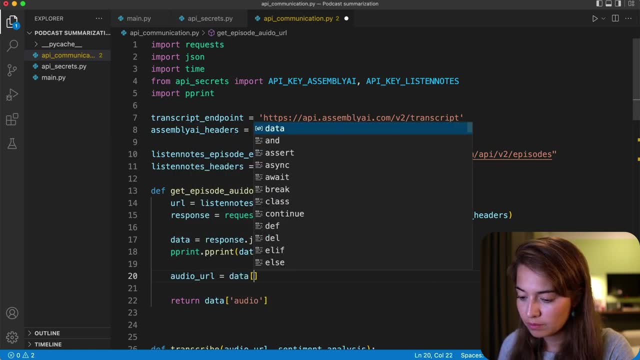 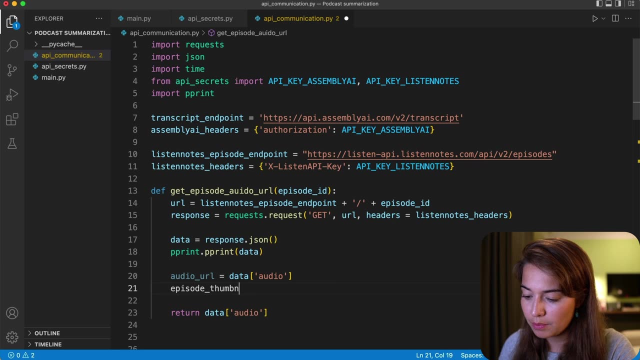 and title of this episode, for example. like we said, we will display here, So let's do that. This will be the audio URL. We will also get the episode thumbnail. Thumbnail, We can get the podcast title That will be in podcasts and then podcast specific information. 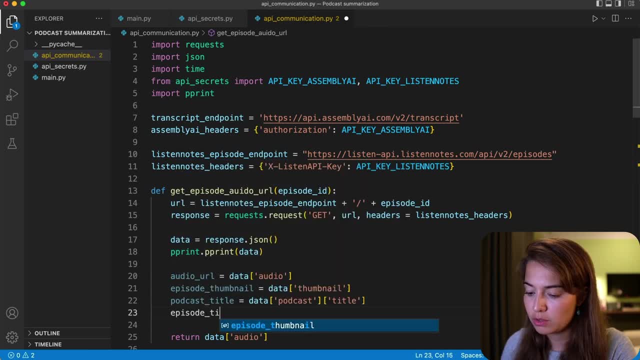 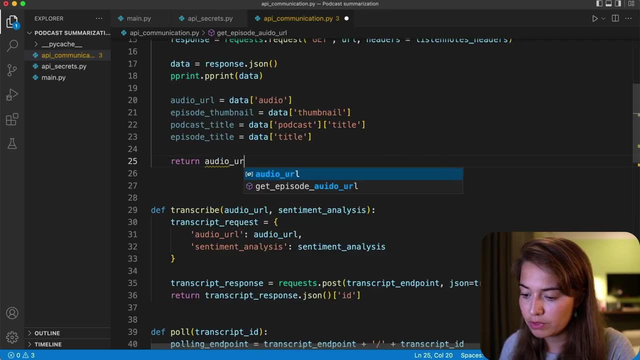 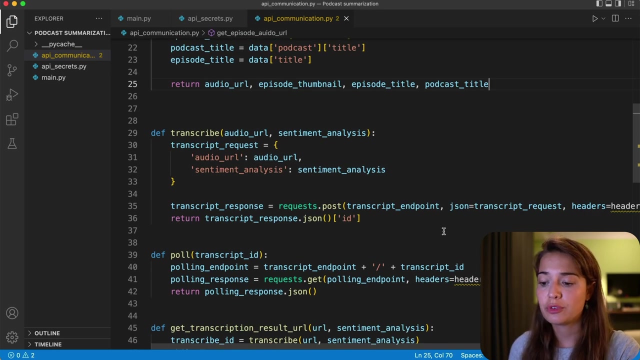 And then we get the title And, lastly, episode title. I think it is just title And we can just pass all of this information back: Episode thumbnail, Episode Title and podcast title. So we don't really need to change much from the rest of the functions. 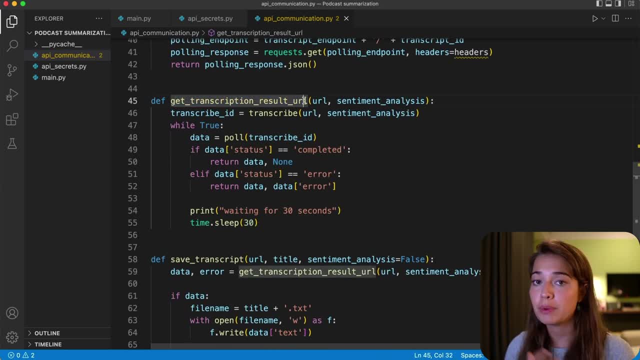 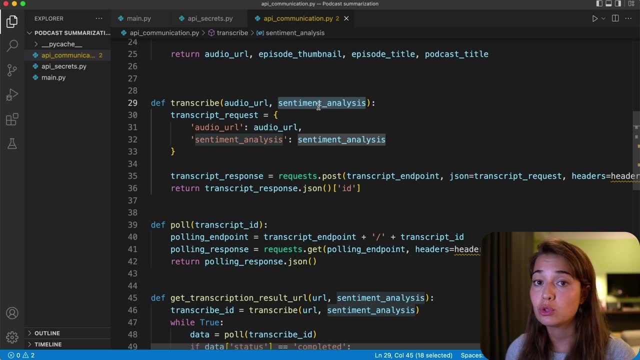 For example, transcribe poll, get transcription result that we already built beforehand. The only thing that we need to change is now: we're not going to do sentiment analysis. We want to use auto chapters, features of Assembly AI. So I am just going to rename these to auto chapters. 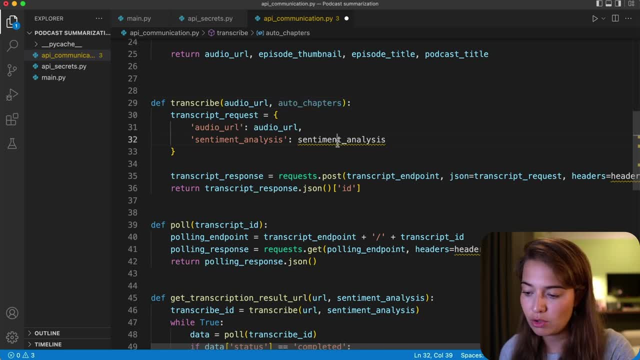 This is just the name of a variable, So it is not that important. You can keep it the same, But for readability it's probably better to keep it the same. For readability it's probably better to change it to auto chapters. 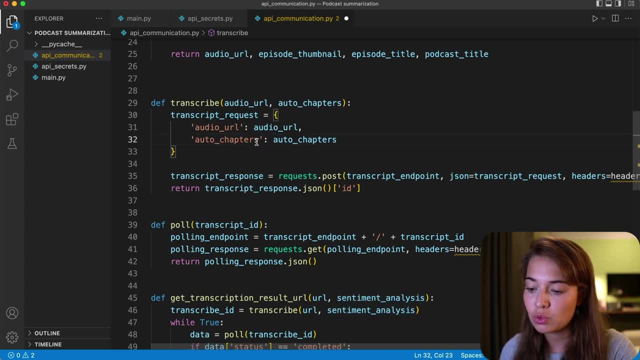 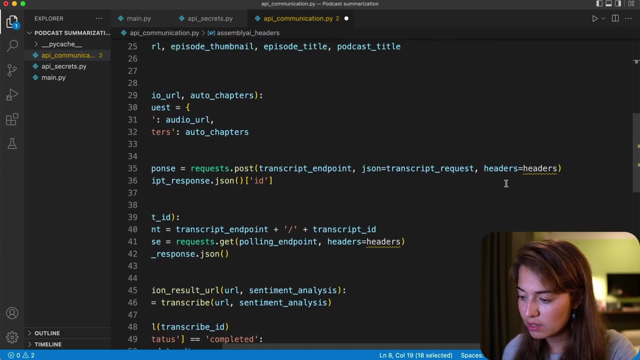 But here in this variable we need to change this name to auto chapters, because we are sending this request to Assembly AI And it needs to know that we want auto chapters. What else? We also just updated the name of the header, So it's not only headers now. 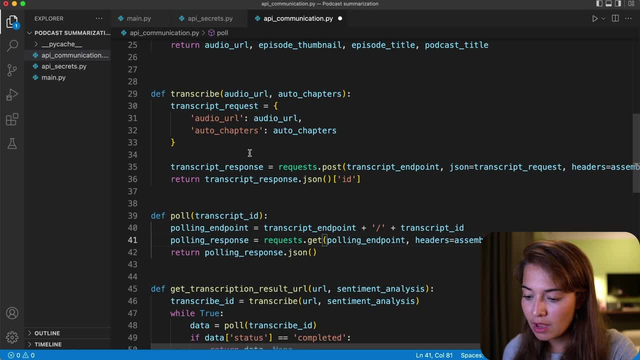 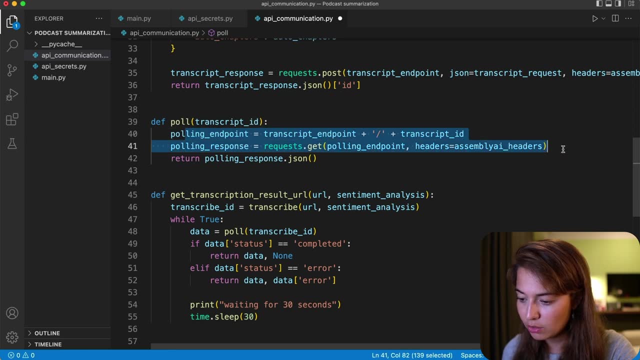 It's Assembly AI headers. Same here In the polling. we do not need to change anything. We are only asking if the transcription is done Or not. Again, in get transcription result URL, we want to change it to auto chapters. 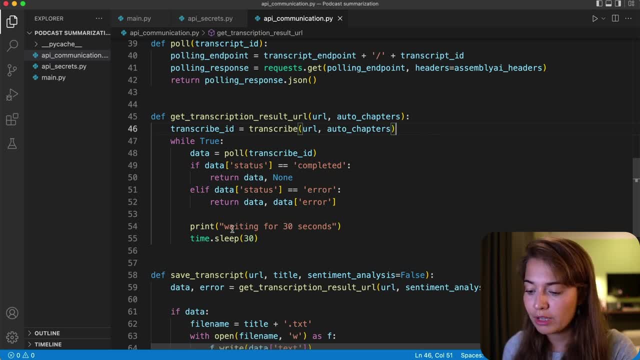 One other thing that I want to change is it's very small, but normally we were waiting for 30 seconds, But now I want to wait for 60 seconds because podcast episodes tend to be a little bit longer, So we want to wait a little bit longer in between. asking Assembly AI if the transcription is ready. 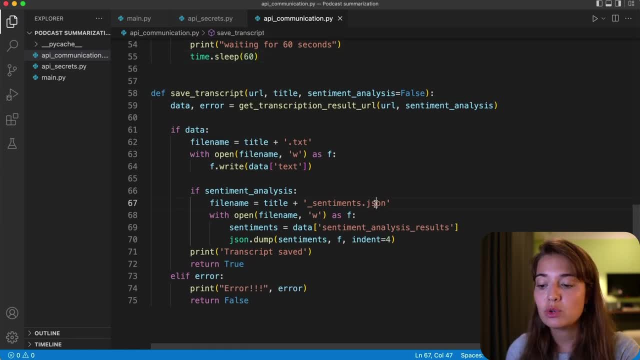 or not. Well, this is a no, So we're going to have to do another change, But the main work is going to happen in the save transcript function. So the main change we're going to need to do in save transcript function is that before we were 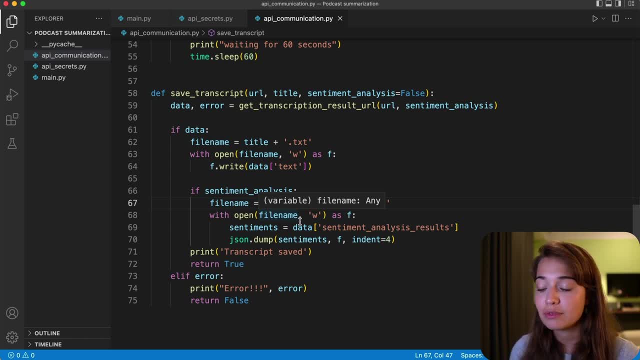 uploading our audio to Assembly AI And then we were getting the results back. But instead this time we are going to only have a episode ID And then we are going to get the URL from Listen Notes And then we are going to pass that to Assembly AI to start the transcription. 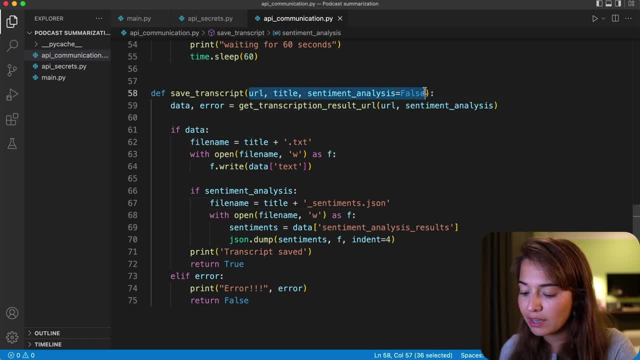 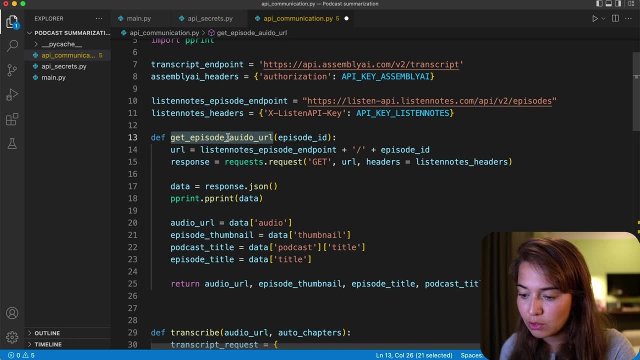 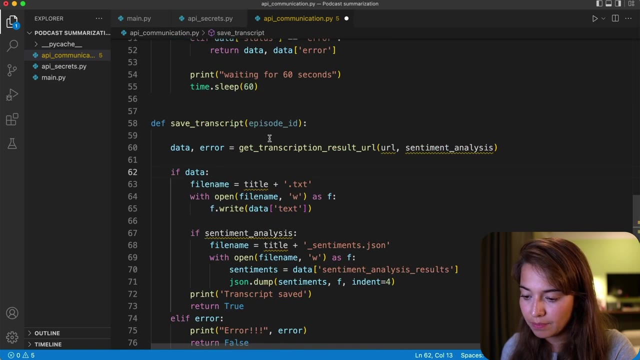 So what I want to do here is to of URL and title. I will just give save transcript the episode ID And then I will run the get episode audio URL from oops from inside the save transcript And, as a result, what we're getting is: 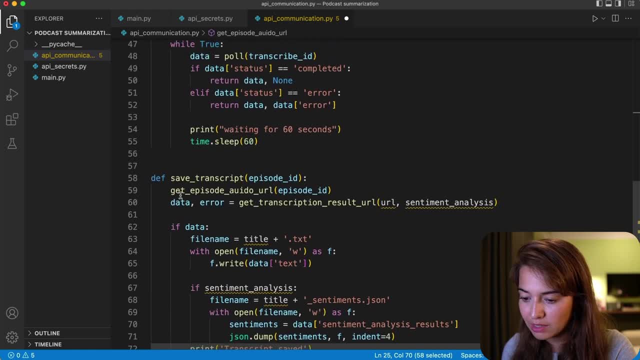 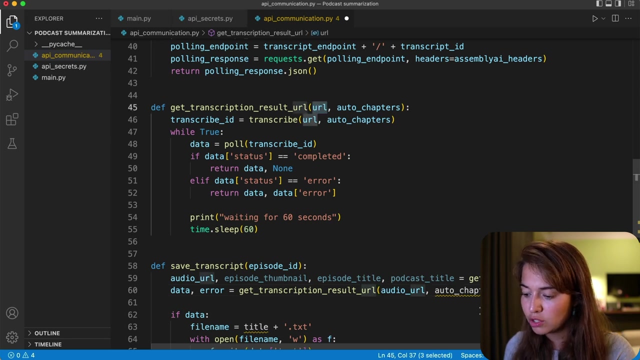 order URL, episode thumbnail, episode title and podcast title. Again, we are not doing sentiment analysis, we are doing order chapters And we need to pass the order URL to get transcription result URL. get transcription result URL. gets the order URL as URL and order chapters, but it is not. 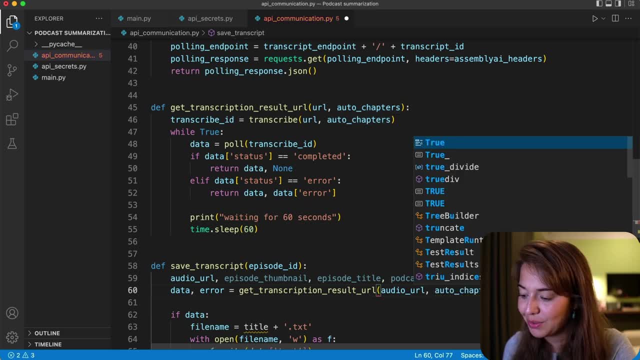 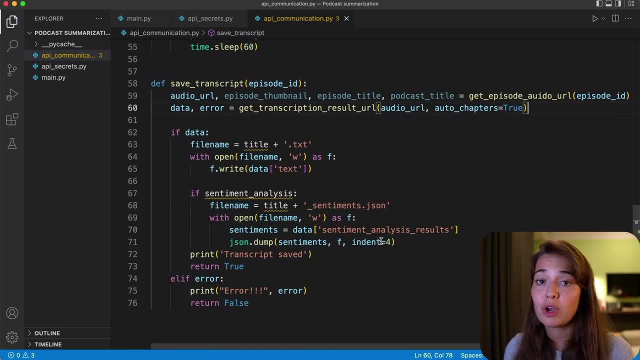 defined. So you know this is what we want to do, So let's call it true here. The next thing that we want to do is to deal with the response that we get from assembly AI. So let's first see what the response from assembly AI looks like when we are doing order chapters, and then let's 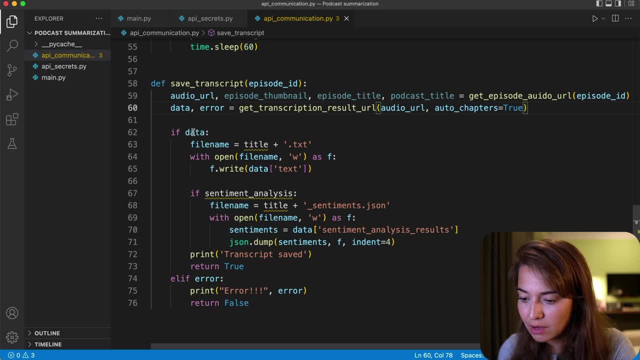 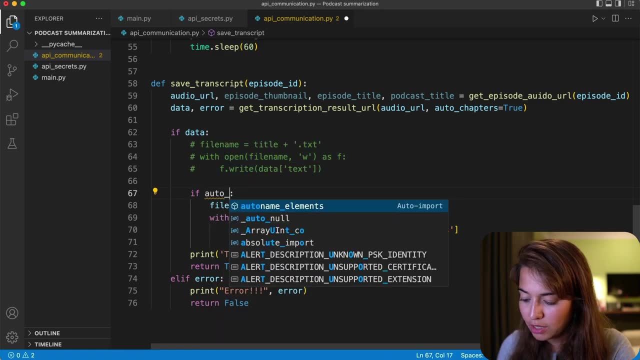 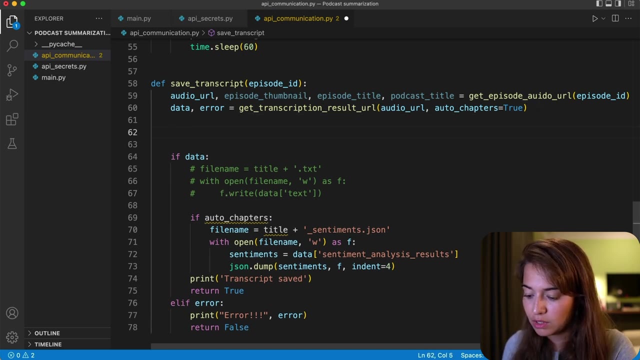 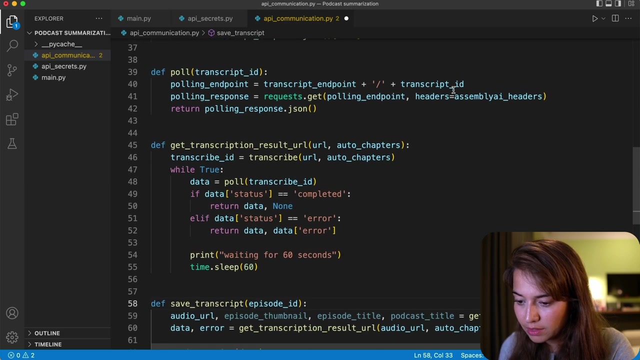 deal with it, But let's fix some of the problems here, So I will not save it into a file for now. I can comment these out. This will be order chapters. The main thing that I want to do is see what the result looks like. right, So I will pretty print the data And the data. 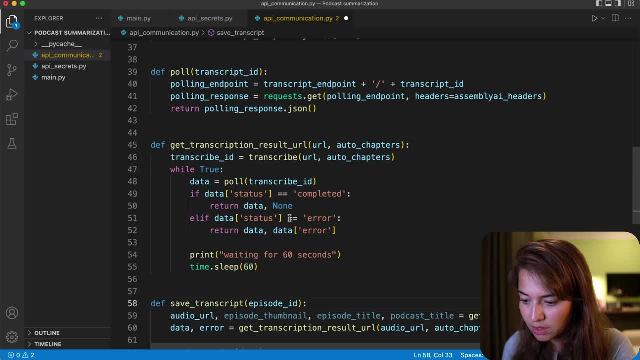 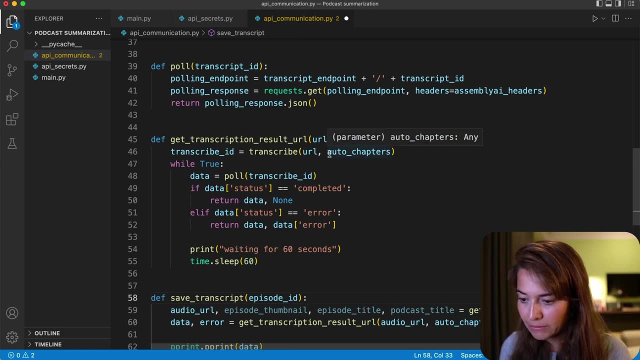 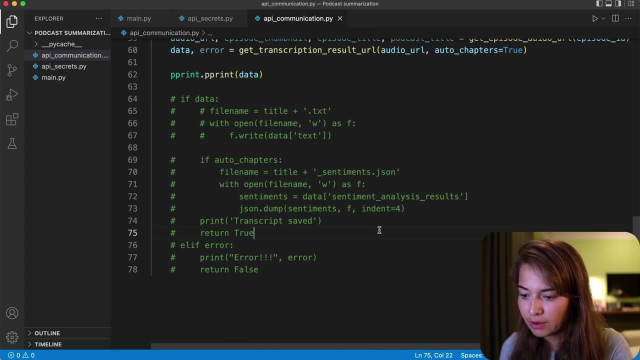 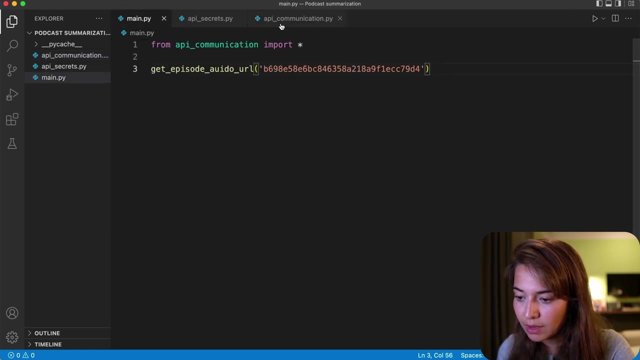 is already in JSON format: Travcribe. Yes, it is, Yeah, so I will just show that. So I'm just going to comment these out for now, just so that you know we have an idea of what the response looks like To run this. I will just pass the episode ID. to save, transform And you'll see that, since this white book of numbers looks like as I mentioned at the end, I think I don't have much in mind At the end of this class. I'll just leave this on here. On the page one is I'm going to go to world and I'm just going to click the EMS and kü. intellectually. 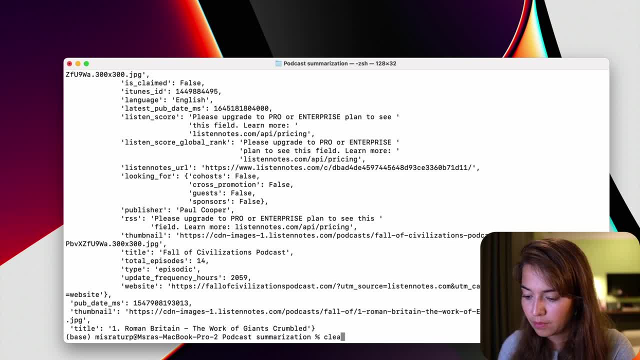 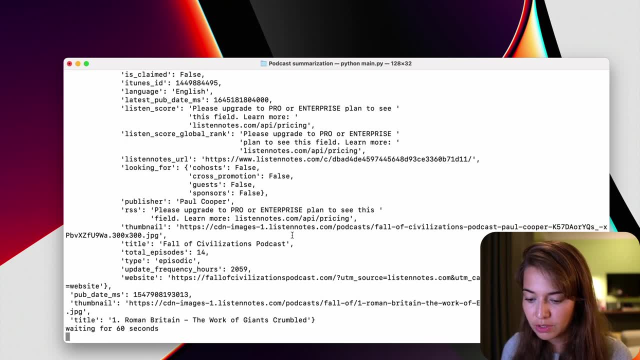 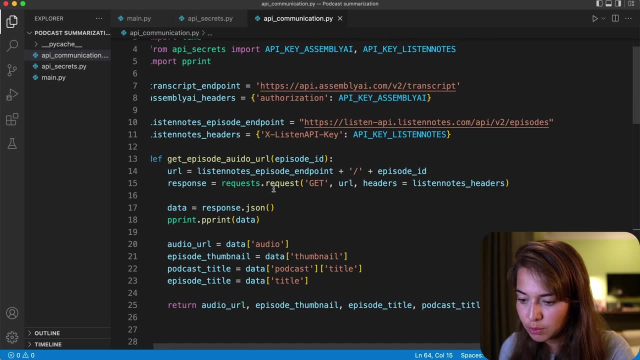 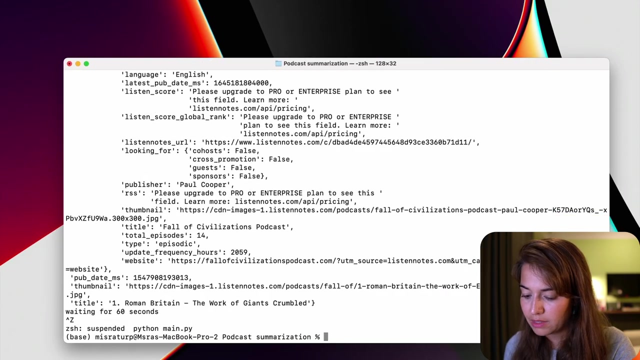 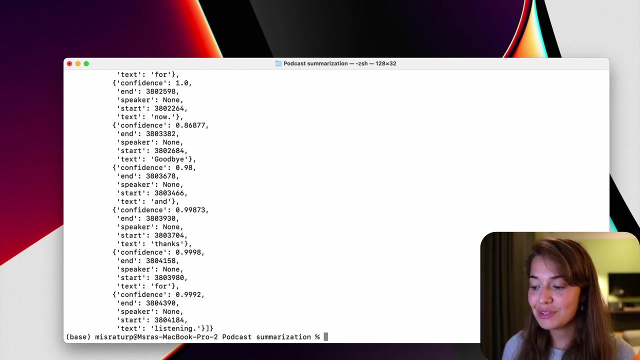 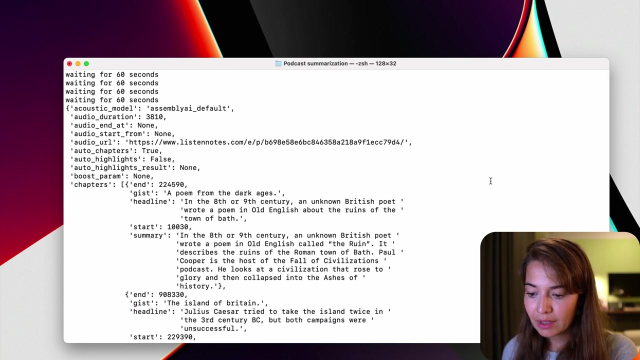 transcript. Oh, we're still printing this one, so I will actually stop printing the response from listen notes and let's start it again. Alright, so we got the results. Let's see what it looks like. It's a lot of information. Let's scroll to the top. What we wanted was the chapters, basically, So let's see what. 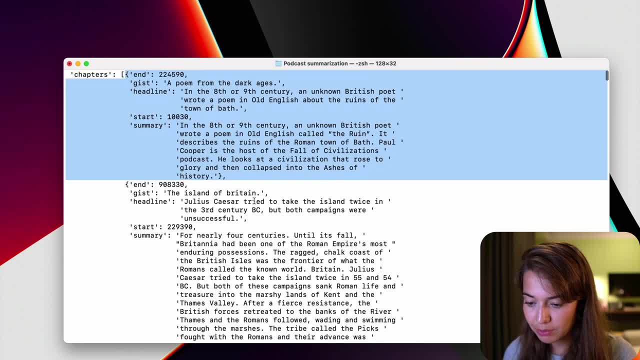 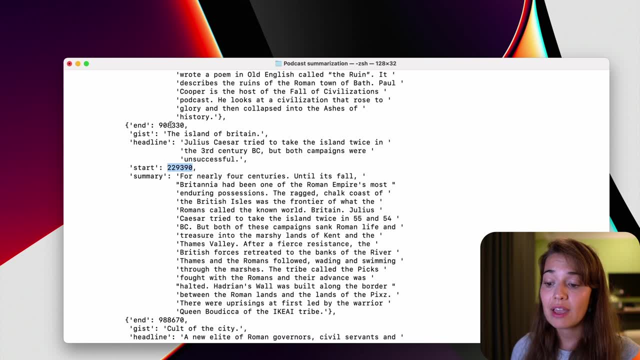 the chapter information includes. So, as you can see, this is one chapter and this is another chapter. So for each chapter we have the starting point and then we have the ending point, the gist of the chapter. so, really quickly, what is this chapter about? We have a headline. 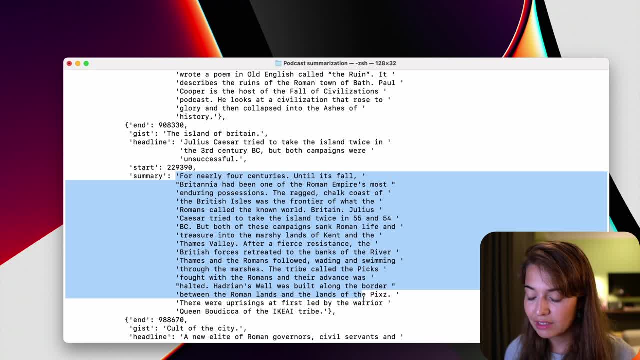 for this chapter And a summary. So, in a couple of sentences, what is happening in this chapter? what is the presenter talking about? What we want to do is to show this information on our application, on our web interface. So that's why what we want right now is to extract this information. 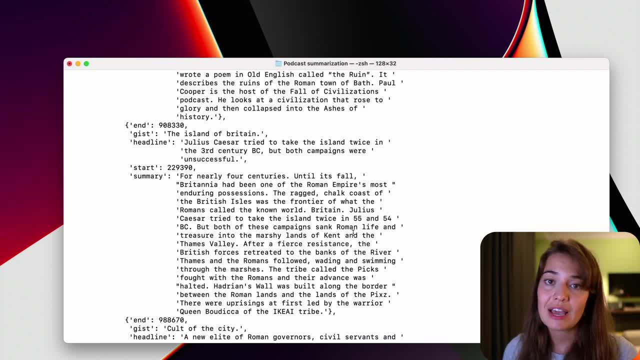 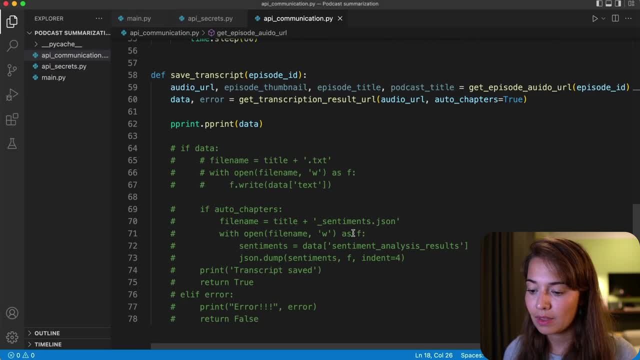 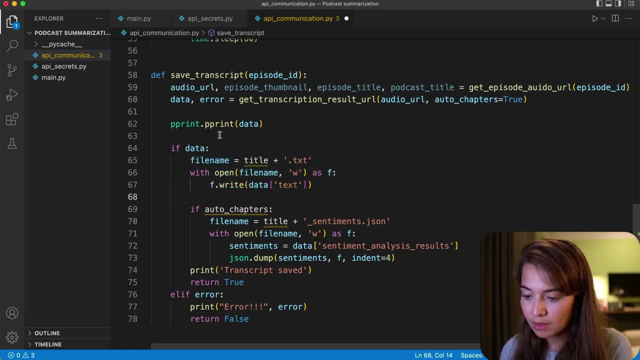 from the response we get from assembly AI and then save it somewhere and then we can visualize it on our Streamlit application. So I will do the commenting here, Also here. So I will call this file with the episode ID. It will be episode ID dot txt And as 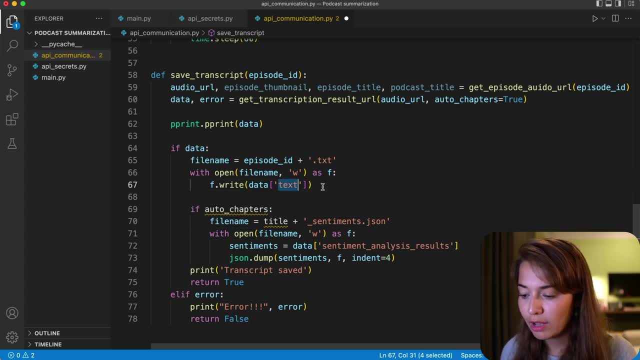 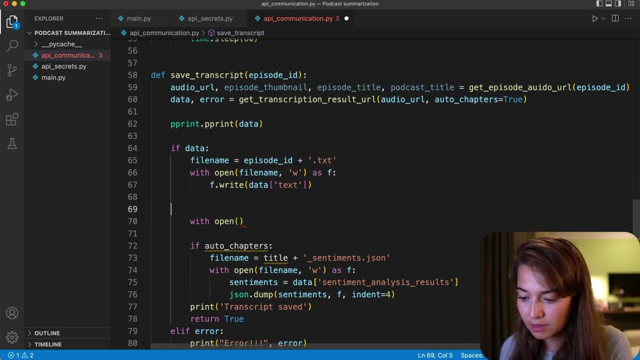 we always do. I'm just going to save the transcripts. You know we don't have to touch this so much, But I will start another file and let's call this chapters file name. And I'm going to call this Chapter Bear sounds like this, and this one will be episode ID. 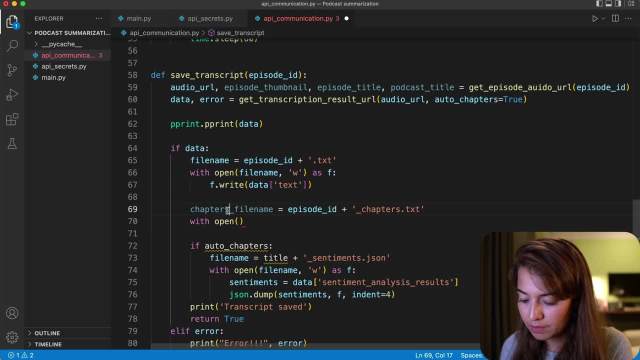 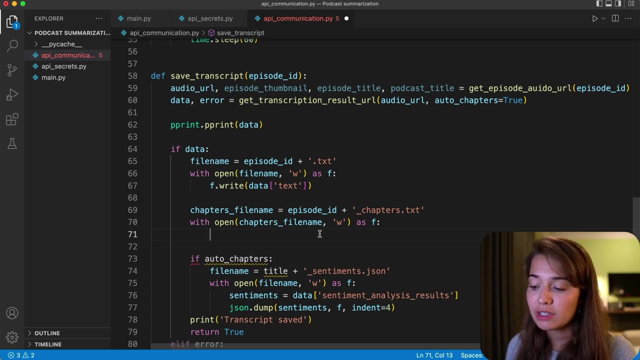 Thetrack. Maybe let's go like chapters dot txt. Alright, so the chapters will be another file. so I'm going to keep all the chapter information somewhere else And in here I'm going to write some of the information I got from assembly Ai specifically. 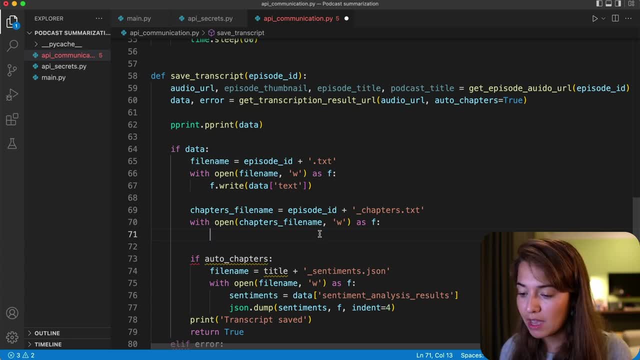 the chapter information And I'm also going to include some of the information. share nai notes, API. One mistake here: I do not want it to be a text file. I want it to be a JSON file so that it will be easier to parse, easier to read later. for me, The first thing that 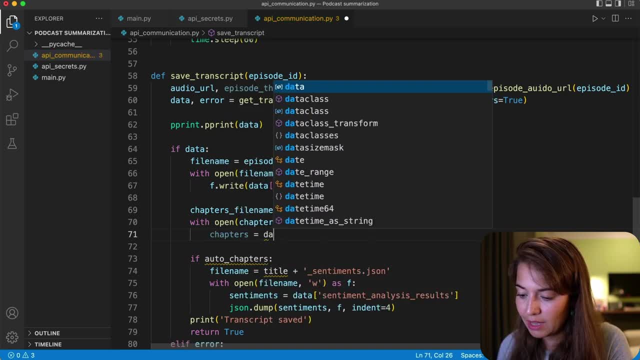 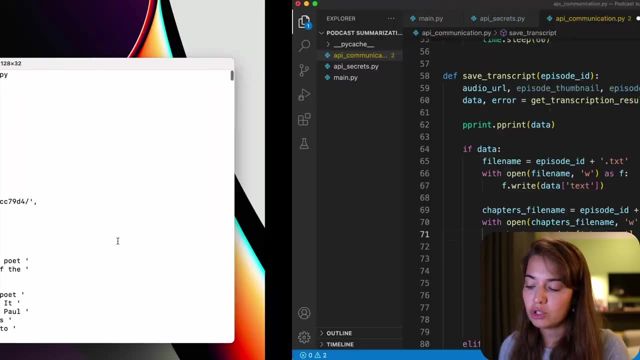 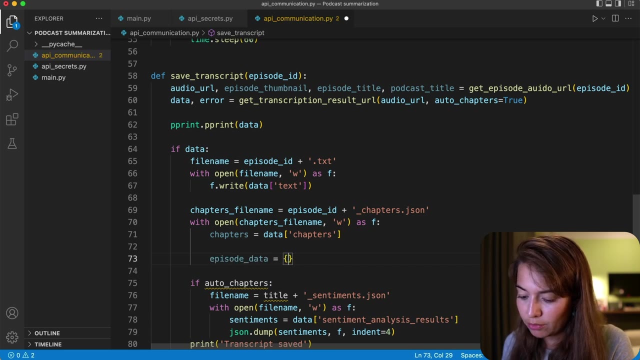 I want is the chapters And I'm going to get that from the data variable. It's called chapters, So let's check. This section is called chapters. Yeah, So let's start it. I will say episode data At first. let's include the chapters again. I will call a chapters And then inside. 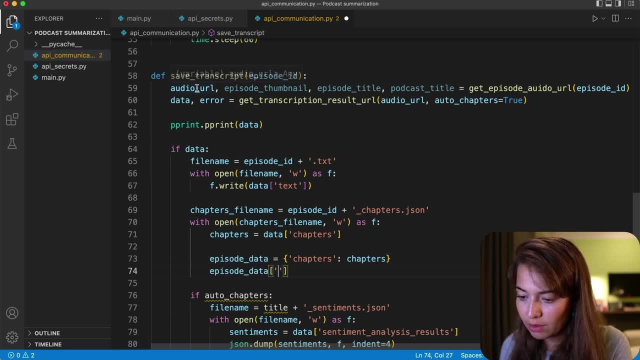 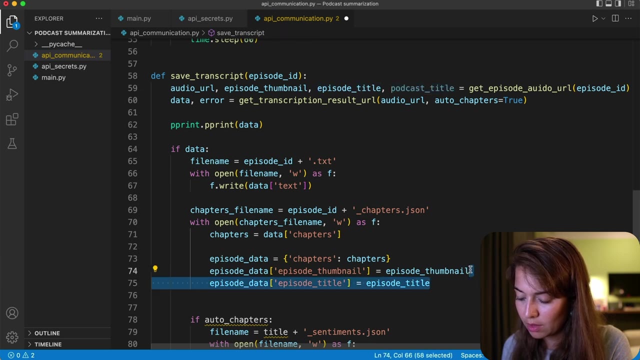 this episode data. what do I want? I want the episode thumbnail, I want the episode title And I want the podcast title. So that's it for now. Thank you for watching my Auf Wiedersehen. See you next time, Bye, bye. 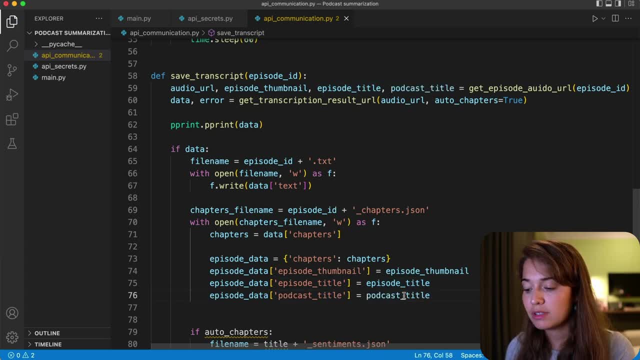 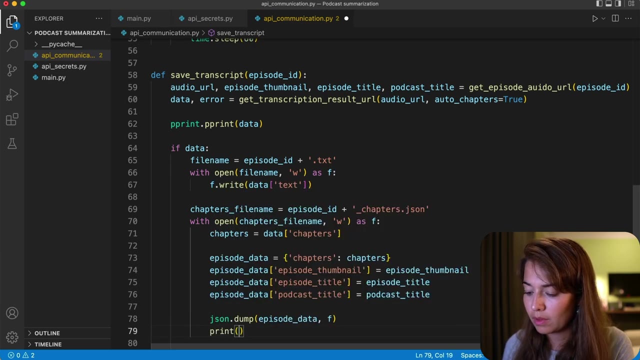 I have all of this information in one place saved on my file system. I can just read it whenever I want and display it to the user And finally dump that to the file so data, and I'll let the user know that the transcript is saved. 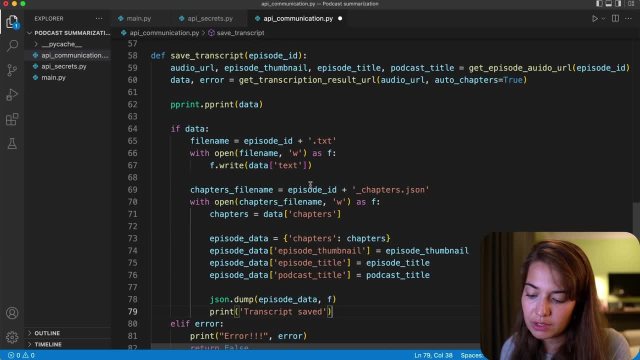 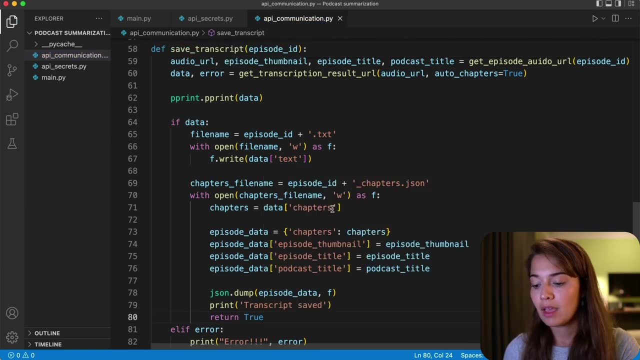 This part. we don't need anymore. And again, if there's an error, we will just say that there is an error will return true, Now that we've got this far ready. up till now, what we do is get the URL from based. 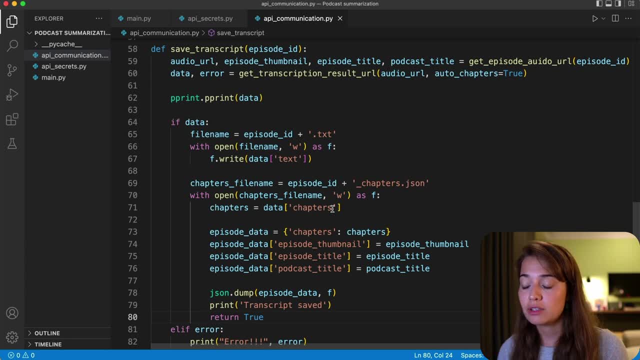 on the episode ID from listen notes and then send it to this URL to assemble. the AI gets audio chapters information and then save it to a file. So let's see that this works well And, while it's running, we will start the stream. 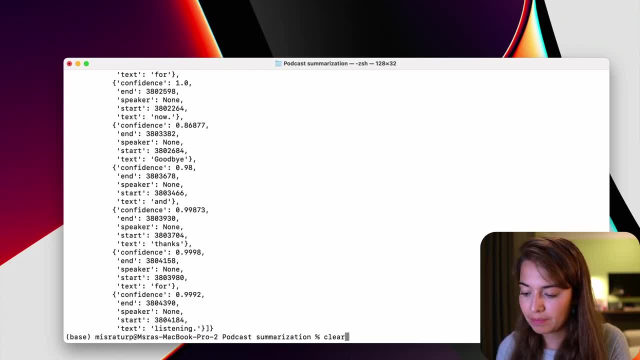 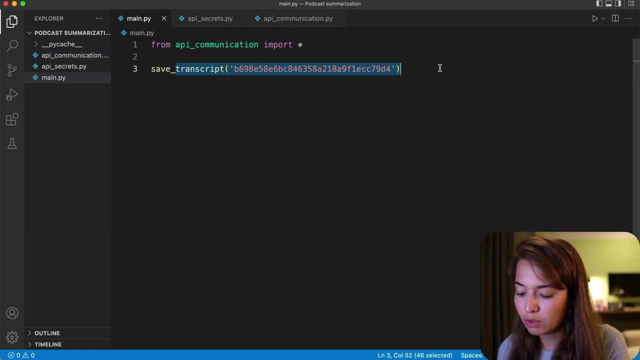 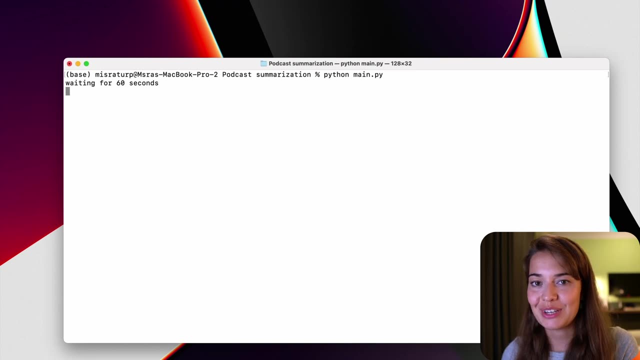 That application. So I will just run this again. But in the main we of course need to call save transcript. Okay, we're already doing it, So I will just run the application And let's also start building our stream it application now. 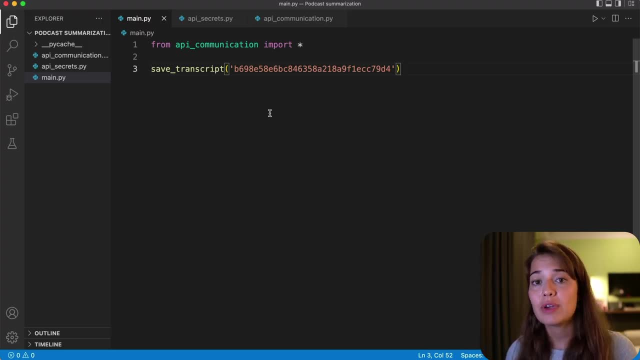 So if you've never heard of streamlet before, it is a really easy way to start building web interfaces for your application, specifically for Python. It's very simple to use. It is It's a very simple API. it's a very simple library. 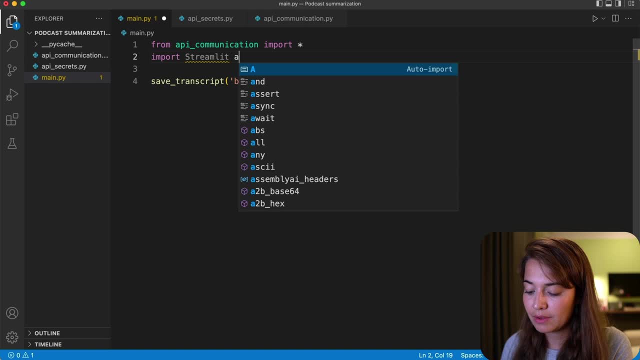 So what you have to do is you call your import streamlet as SD. if you want it to use it simply, And let's say, if you want to, you know, put a title in your application. all you need to do is SD title and then you can show that it is a title. 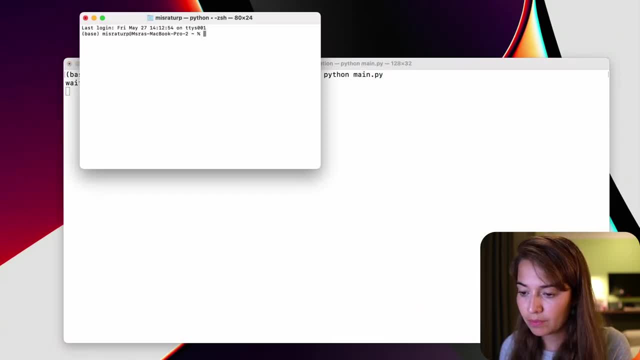 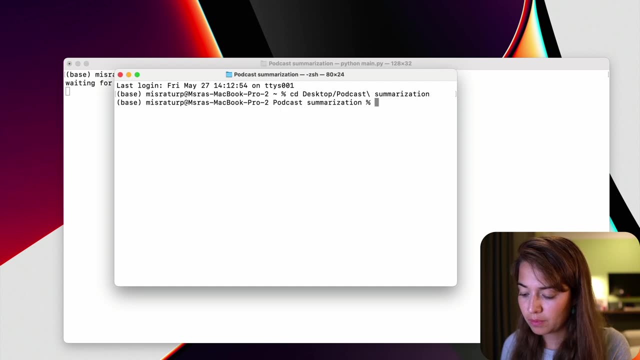 So I will run this separately To show you how it works. Okay, Okay, So let's go And to run streamlet applications. you just need to say streamlet, run mainpy. Streamlet is installed on your computer like any other Python library. 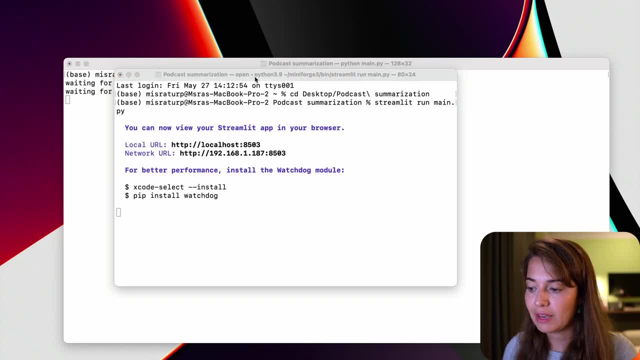 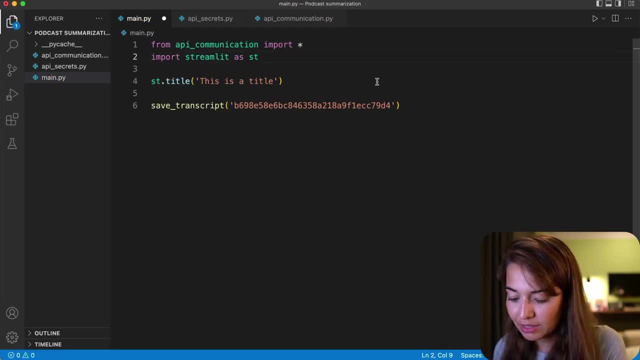 So you just need to use pip, Say pip, install streamlet, and you will be good to go, Unless you make a mistake and call streamlet with a capital S, which is not the case. it needs to be a lowercase S, So let's do that again. 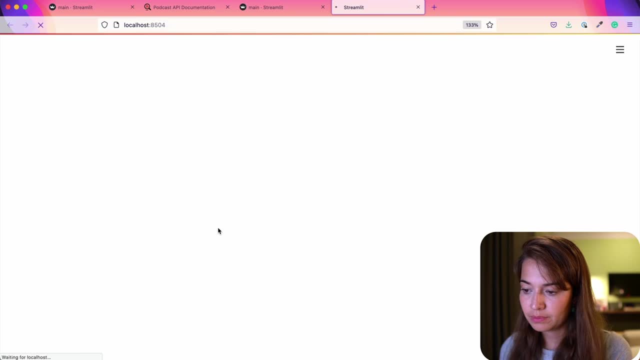 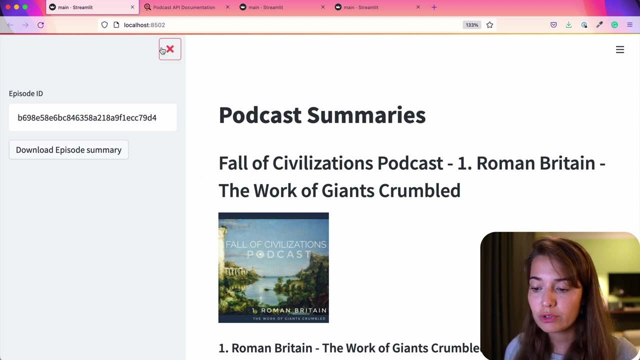 Okay, Okay, All right, So this is actually an application. The only thing we're showing right now is a title, And we know what we want it to look like is this, So I will start building the elements in this application. So the first thing that you know strikes us is that we have a sidebar. 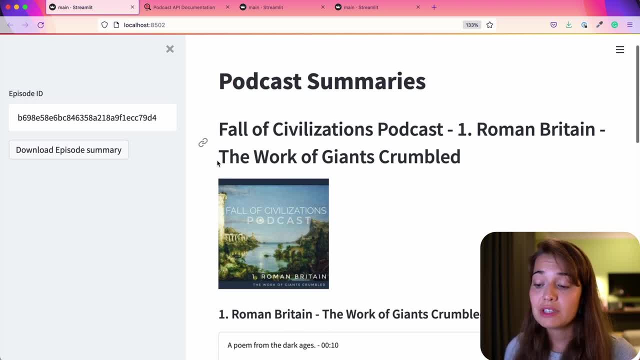 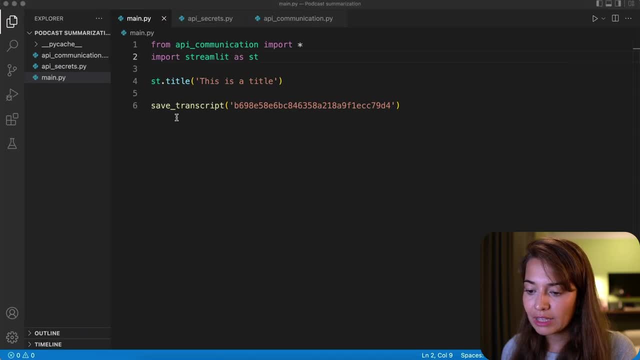 We have a title that says podcast summaries And then we start showing the information from the information we got from the APIs that we've been using. So let's put a sidebar. Maybe let's fix the title first. We want to say podcast summaries. 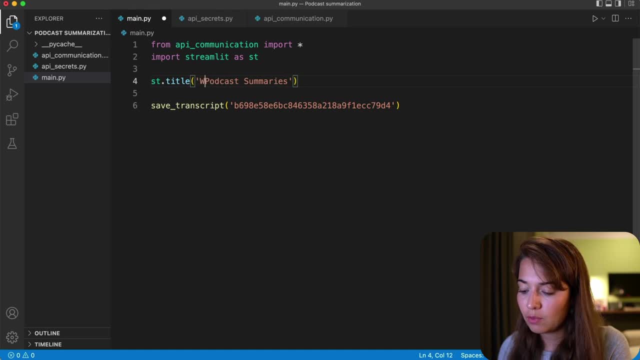 Title says podcast summaries. Or you can even say welcome to our to my application that creates podcast summaries. Let's see. Maybe that will be too long, but we'll see. And let's create the sidebar. It's quite simple. You call streamletpy. 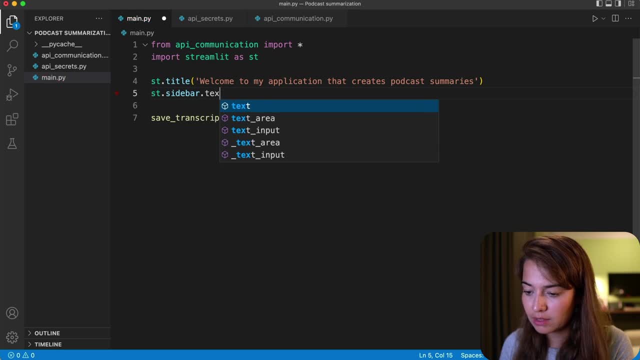 Okay, Streamlet sidebartextinput. Yeah, And then you know, you can say please input an episode ID, And I can also have a button at the end of the sidebar that says get podcast summary, Maybe with an exclamation point too. 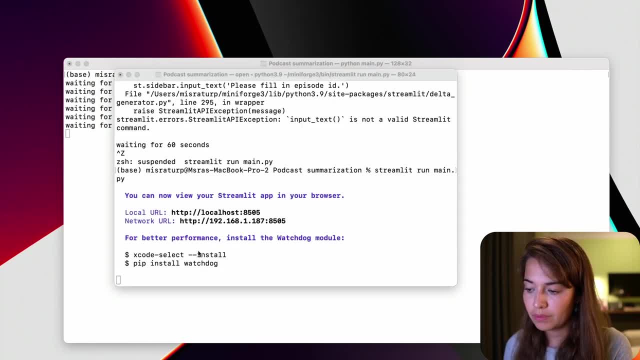 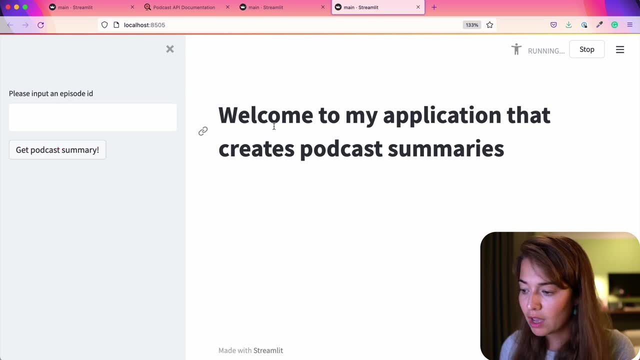 So let's run it again, Okay, All right. All right, Let's see. Okay, This is looking more like it. It says welcome to my application that creates podcast summaries. I can put an episode ID here and then I can say get podcast summary. 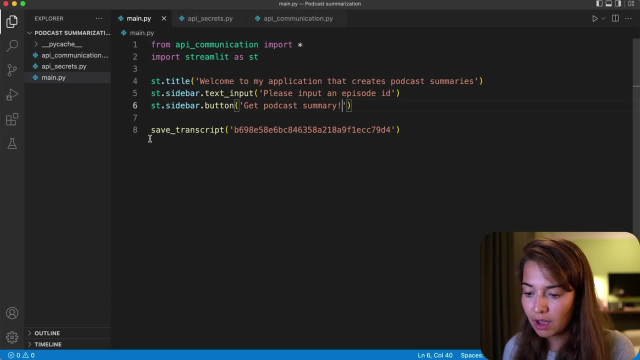 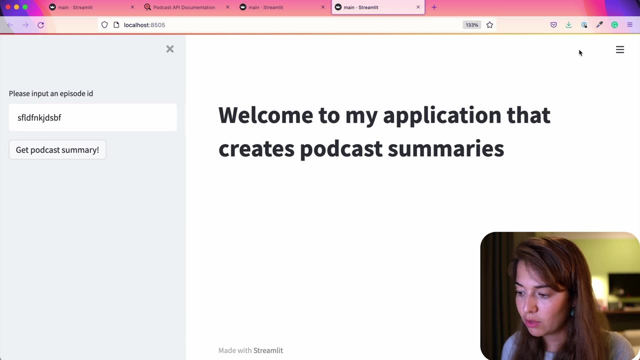 So you see that it is running. It is running because I forgot to comment out this one. So it's actually running the whole application. I'll just stop it for now because we don't have any way of displaying whatever we get back from the APIs. 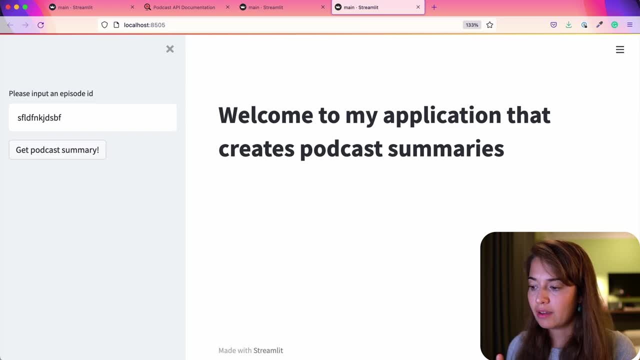 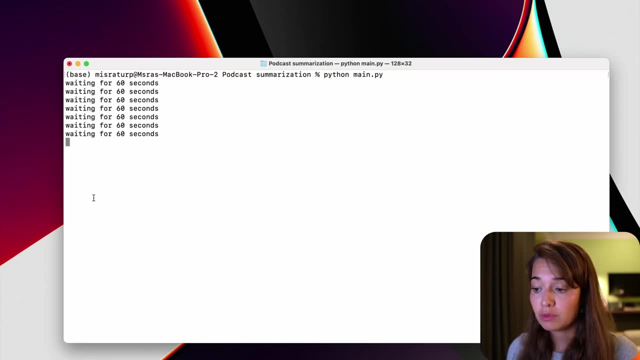 So I'll stop this now. Okay, And now that we have the application looking more or less like what we want it to look like, let's wait for the chapter results to be printed on our file, and then we will see what it looks like. 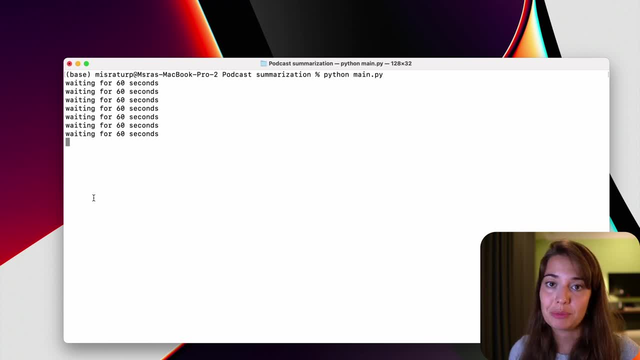 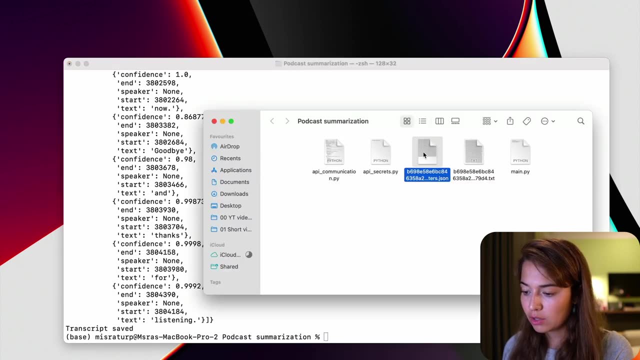 And then we can start parsing it and then showing it to the user on our Streamlet application. Okay, So the transcription is saved. Our auto chapter creation is done. Let's take a look at what it looks like. We have the chapter section. 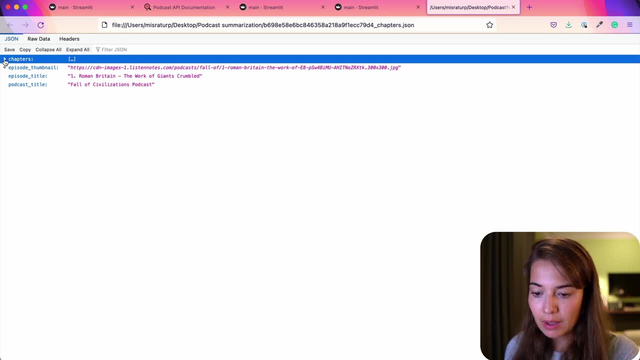 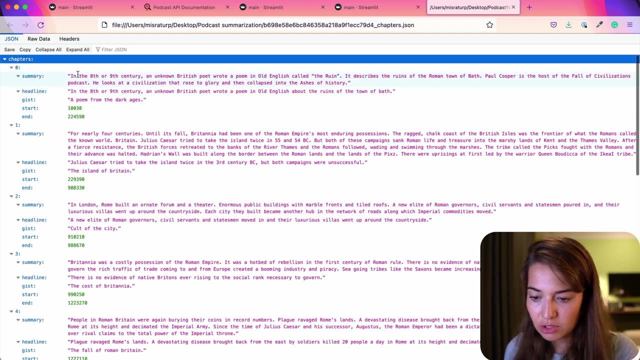 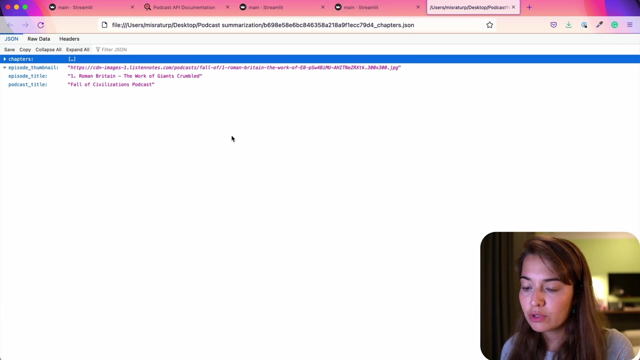 We have the episode thumbnail, Episode title and podcast title, all good. In the chapters we have chapter numbers and inside each chapter we have the summary headline, Just start and end. So it looks good. Let's start showing this, The first thing that I want to show, of course, like we did in the beginning, like we showed, 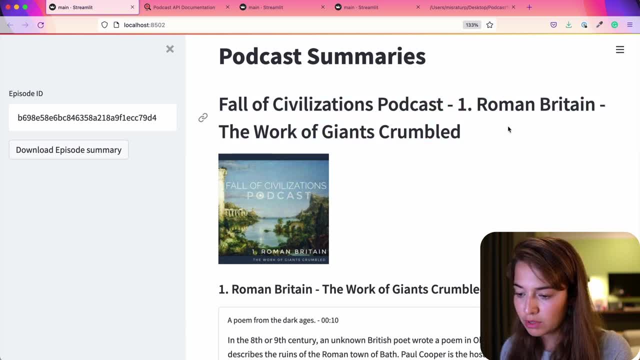 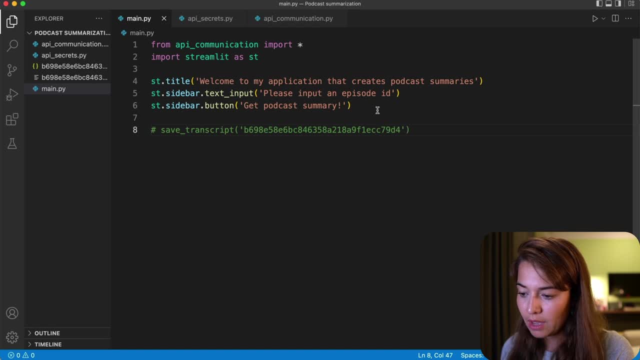 in the beginning is the name of the episode or maybe name of the podcast, plus the name of the episode And then the episode thumbnail. So how I'm going to show that is again using Streamlet And that is going to be the header for me. 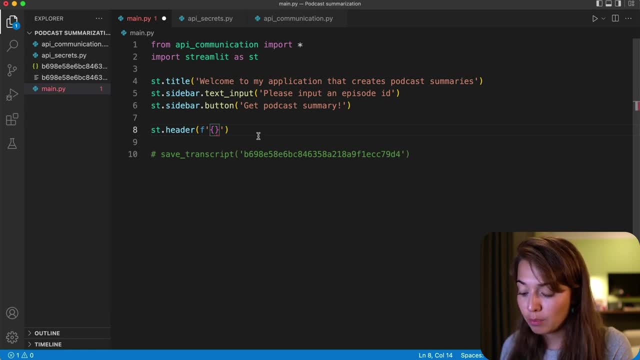 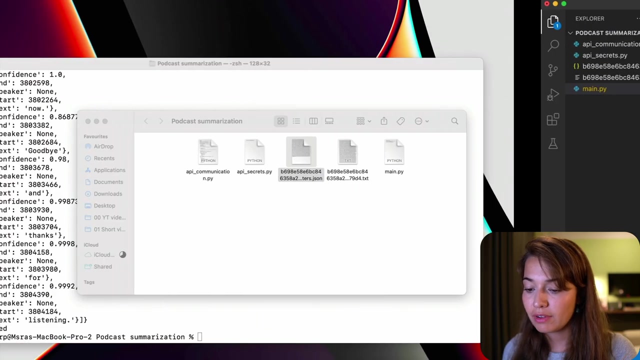 And I will include the podcast title, Maybe with a dash in between, and the episode title, But, as you can see, we do not have it yet, So first we need to open the file that includes these things and the file that includes those things. 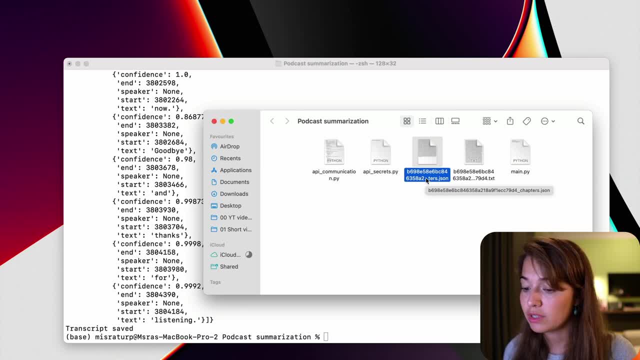 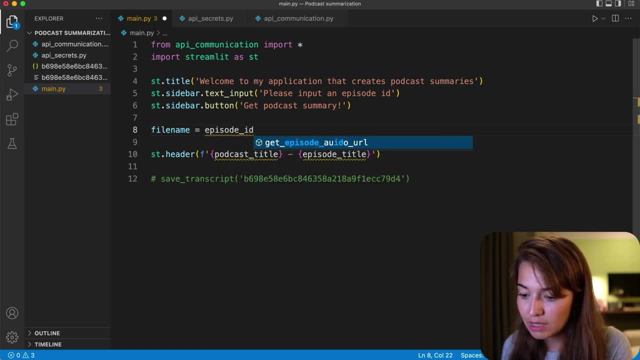 It's the episodeidunderscorechaptersjson, So let's start that again. File name would be episodeidunderscorechaptersjson. And where do I get the episode ID? I get the episode ID from the text input. So the user is going to input an episode ID and then I'm going to save it here in this. 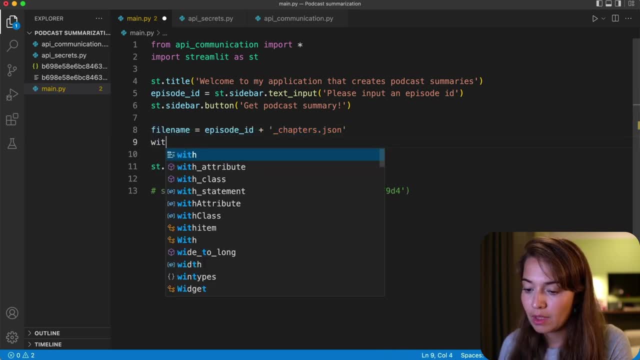 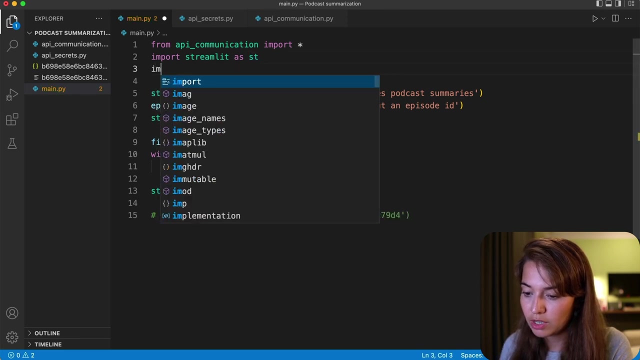 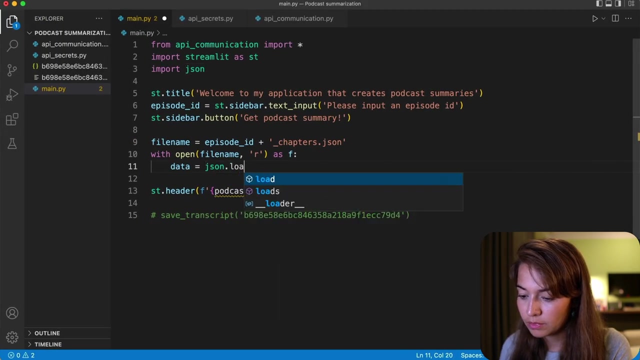 variable, and that way I will have the file name. So then I just need to open this file And let's call it data. for example, I need to import JSON, of course, And load it into the variable data. So, in this variable data, what do we have? 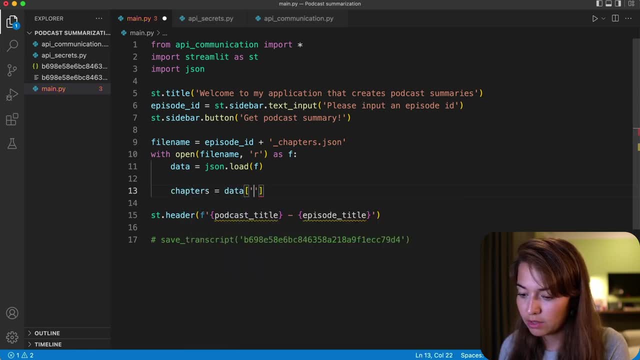 We have the chapters, So first let's get the chapters- Data chapters- And then what we want to get is the podcast title And then the episode title. Let's change the names, episode title, And we also want the thumbnail. 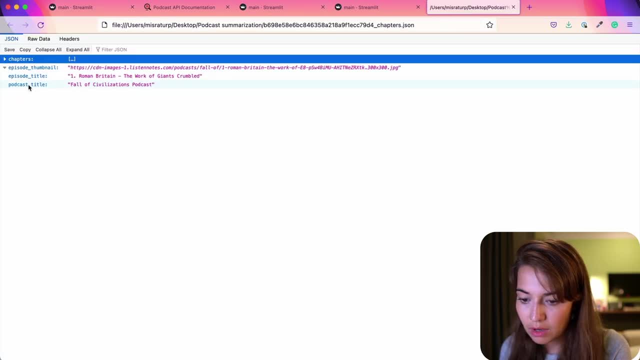 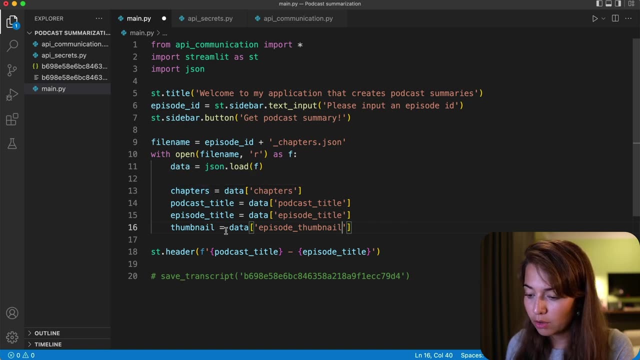 And what did we call the thumbnail? We can see here episode thumbnail. All right, So we're already showing the podcast title and episode title, streamlit header, And then we can show the image thumbnail with the streamlit image function And from this point on, the next thing that we want to show is the chapters. of course, 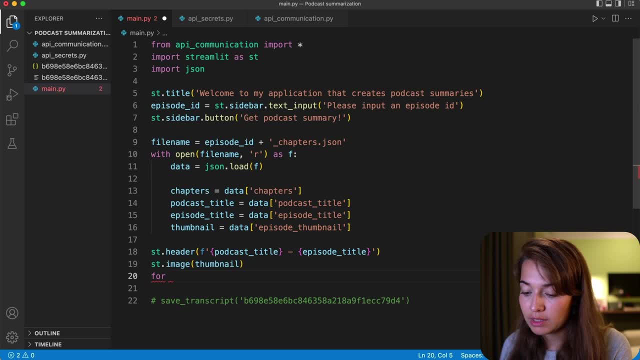 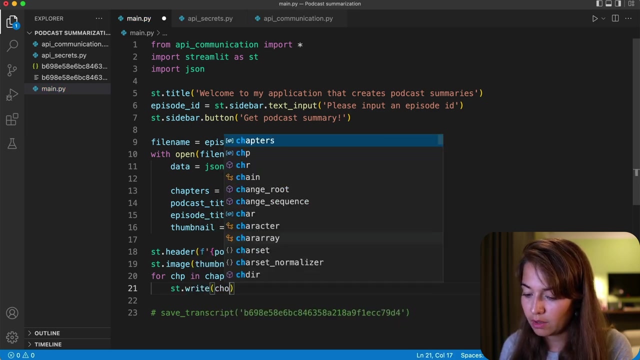 One thing we can do. for example, we can use a for loop. We can say for chap in chapters, For example, we can use a for loop. You know, you can just say streamlit, write or just show the chap, but that's one way. 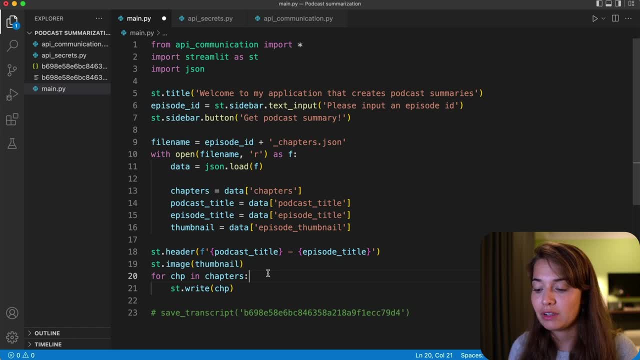 of doing it, But then you're going to have a lot of text one after another, and it's not really nice. What we want is like in the original one I showed you at the beginning: we want expanders. So it's quite easy to create expanders with streamlit again. you just say streamlit expander. 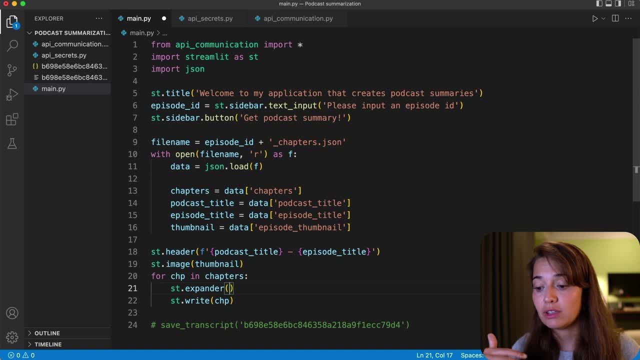 and then you want you write what kind of information you want to be in your expander. So as the title of the expander I will write here what I want in title And whatever I want inside the expander I'm going to write inside. 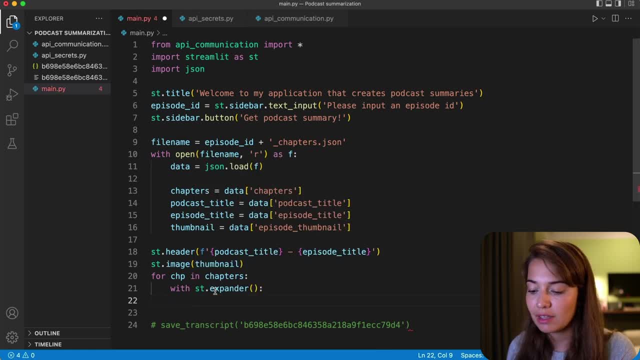 So I do not need to use a streamlit thing again, because this is going to be inside the expander And inside the expander. what I want is the summary. So I think it was called summary. Let's just check again here in our JSON file. 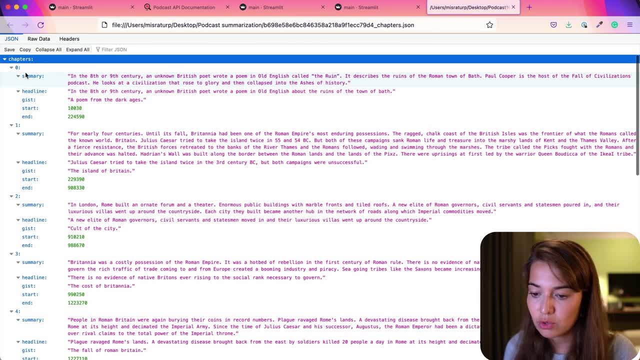 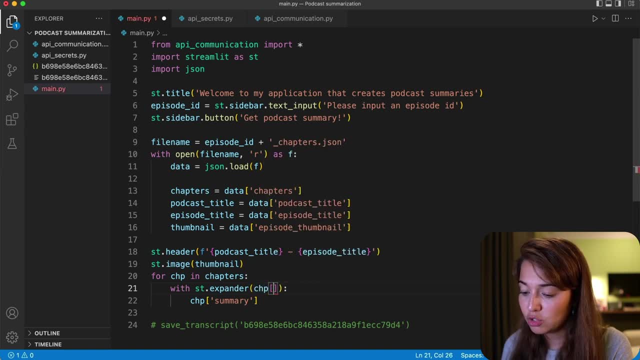 Okay, So in chapters we have summaries called summary. Yes, So I want the summary to be in there And, as a title of the expander, I want there to be the gist of each chapter. So for each chapter is going to show me the expanders. 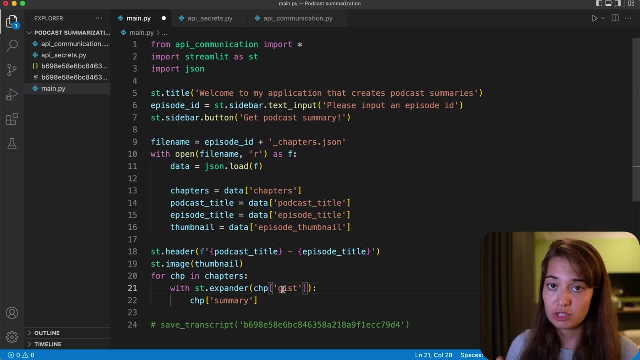 For each chapter there will be expanders and the title of the expander will be the gist of this chapter, And inside the expander we are going to have the summary of this chapter. So let's run this and see how it looks. 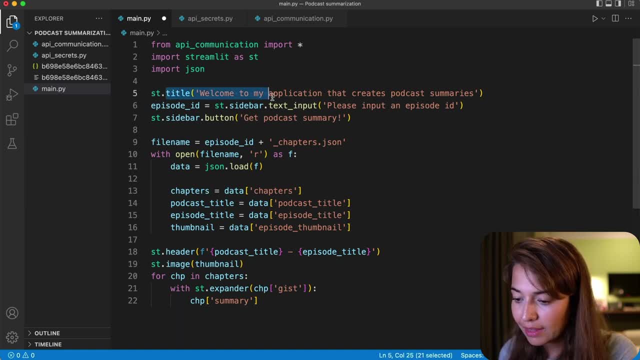 But let's, let's first make sure that everything works. So I have the title and then I asked for a episode ID from the user. There is a button that starts this process, And for that to happen, I'll just call this button. 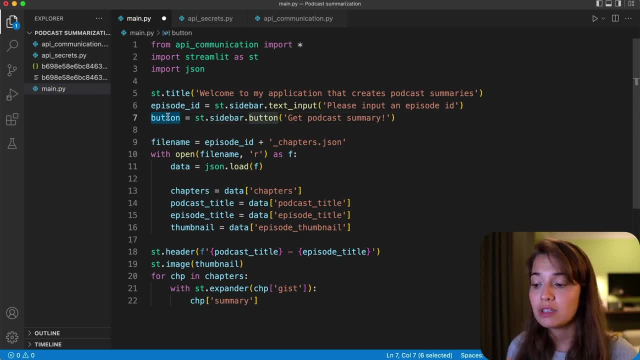 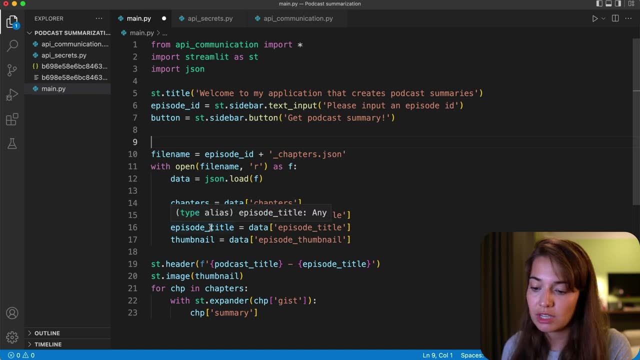 So we this information, this button variable has information of whether this button has been pressed or not, And I only want this part, this part, to happen, this visualization, the display part, to happen if the button has been pressed. So I'm going to wrap this all in a condition. 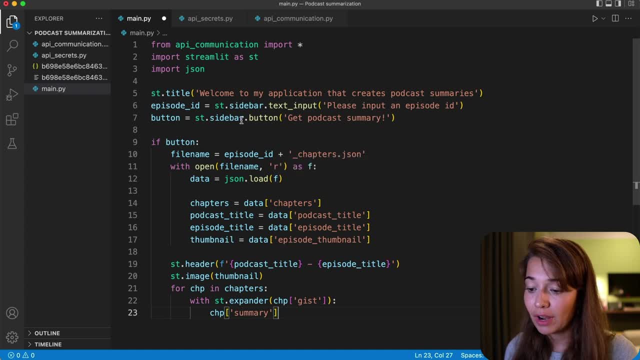 So otherwise it's not going to happen. Yes, but right now, if someone presses the button, nothing really happens. So we also need to add an action to this button, And how we're going to do that is we're going to say on click. 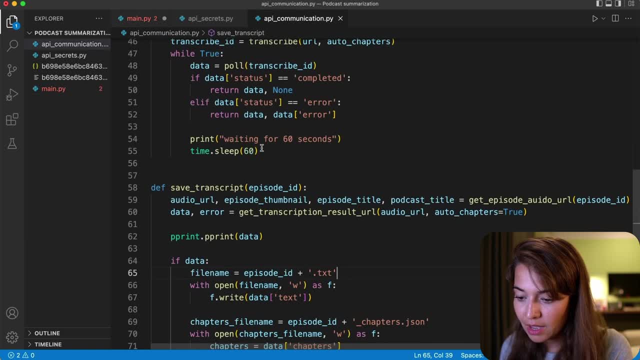 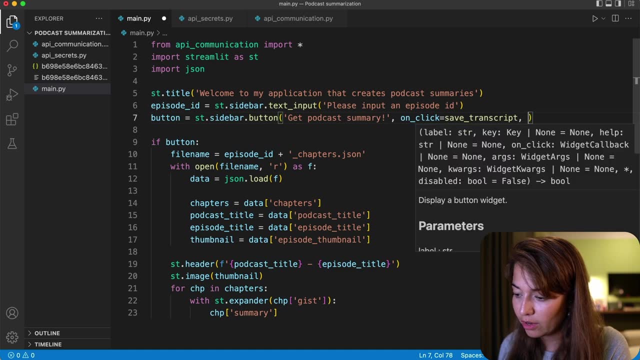 If this button is clicked, what we want to happen is the save transcript file to be run. So I'm going to call it here in the on click argument. And we also have arguments right. And here is how you pass arguments To your function that you call from your button. 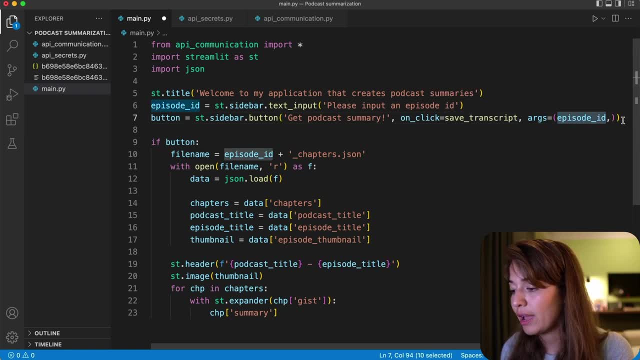 This is a tuple. That's why you write the variable or the argument that you're passing to the function, and the first one And the second one is empty. Now, when the button is clicked, this one should run and we should be able to see all the information. 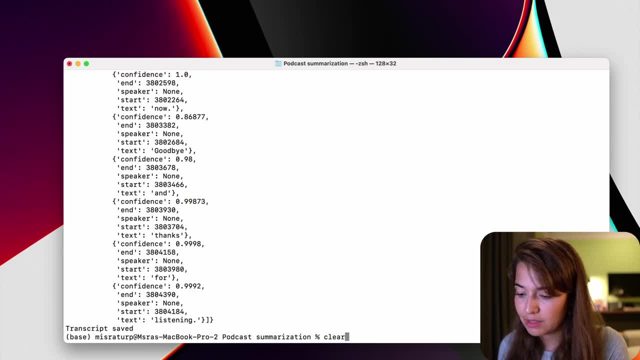 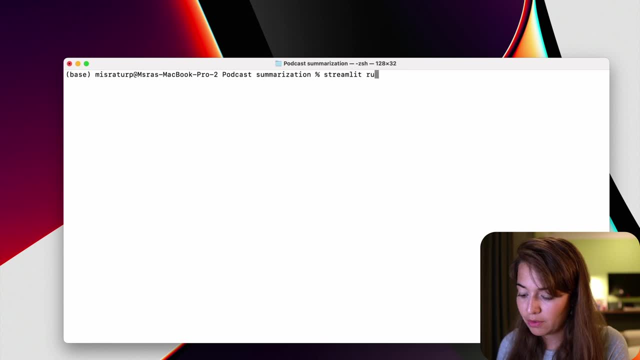 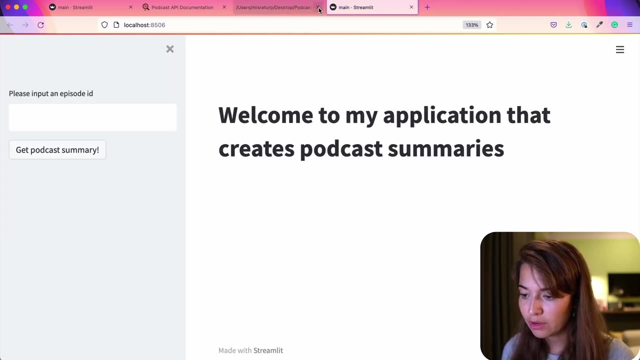 on our application. So let's run it again and see what happens. Yeah, we need to run the streamlit application this time. streamlit run main, that pi. I'll close the old ones. so we know the difference and which one is which. 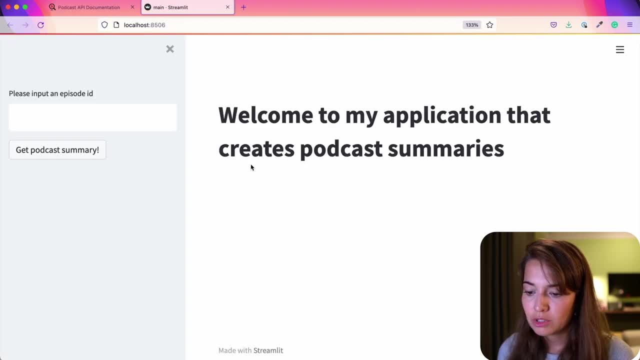 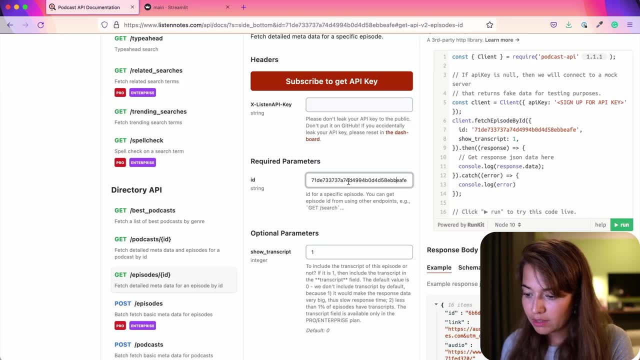 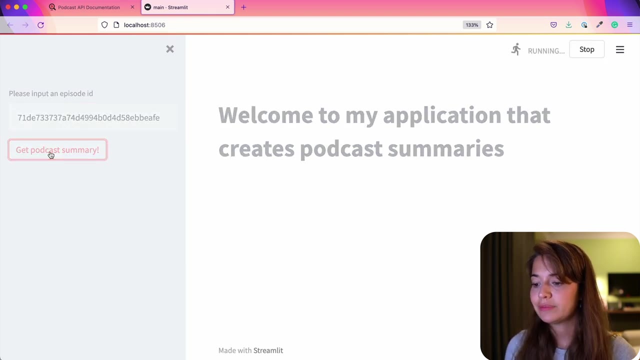 This is just the example from the beginning. All right, So we want to get a podcast, we want to display it. I will get this one again. Let's get the podcast summary. And here it is. We have the title. Welcome to my application. 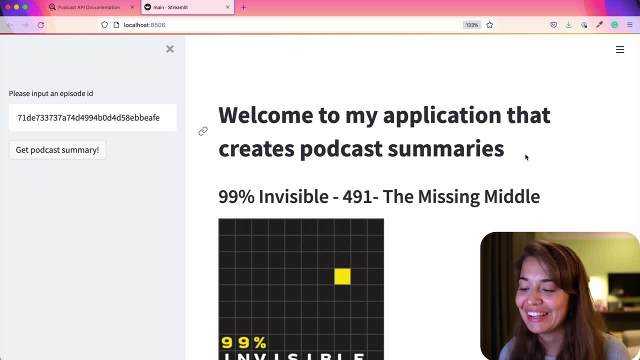 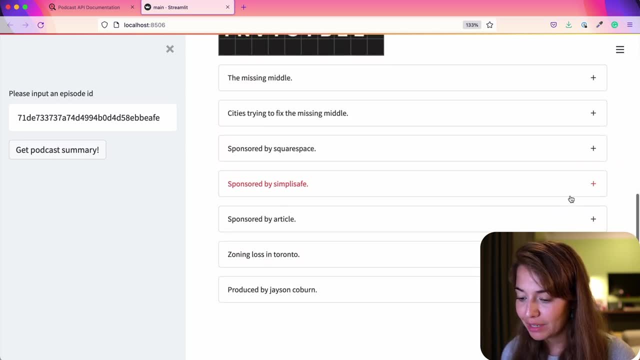 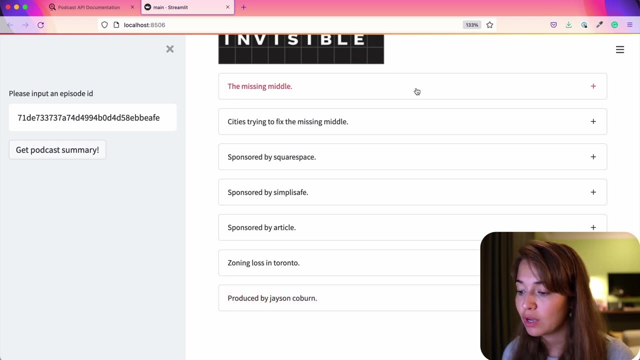 That crazy podcast summary is okay. maybe that's a bit too long, I will shorten it: The name of the podcast, name of the episode, number of the episode- also the missing middle, And here are my chapters. So apparently there are 1234567 chapters assembly AI's API was able to find and each. 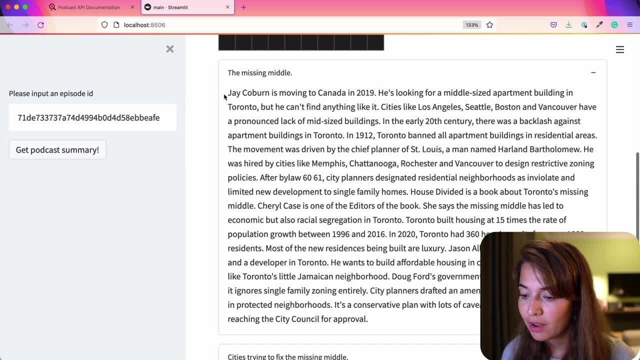 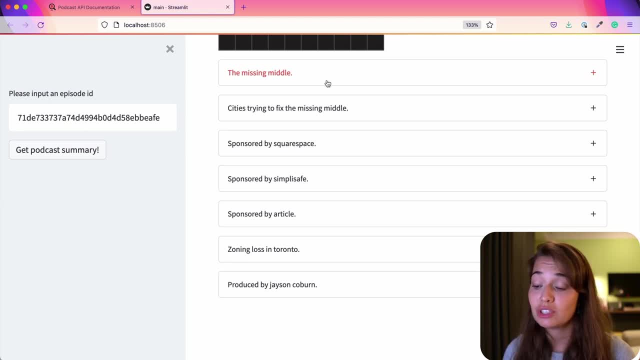 chapter. we have the gist of the chapter as a title of the expander and the chapter summer here. Well, one last thing that I want to add is a start and end point of the. So just the start point of the chapter here, because I want to show, like, how long each chapter. 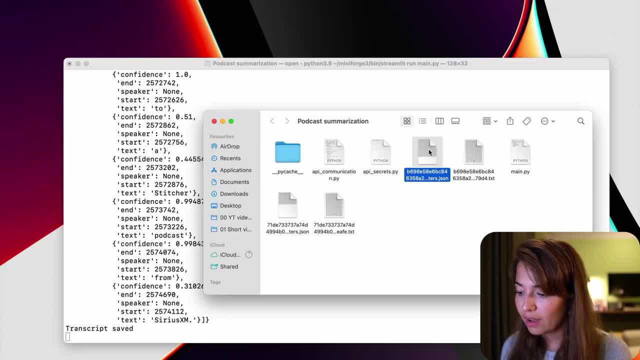 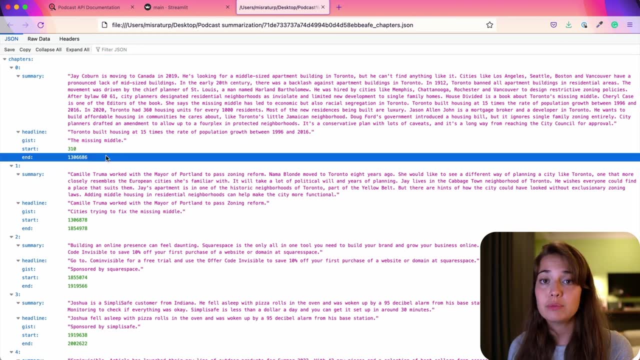 is maybe, so let's do that. So for that I want to see in this JSON file how it looks. so the start looks like this: So these numbers might look a bit random to you, but basically they are milliseconds, So I want to turn it into minutes and seconds and, if applicable, hours. minutes and seconds. 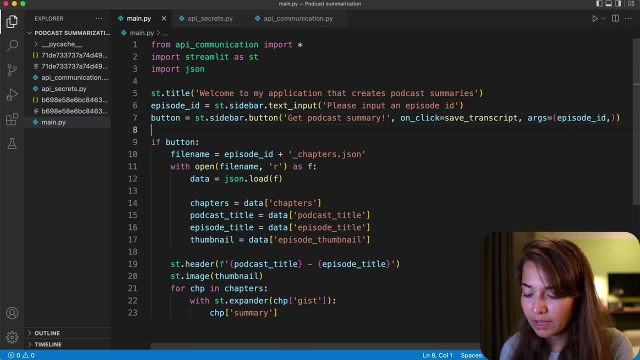 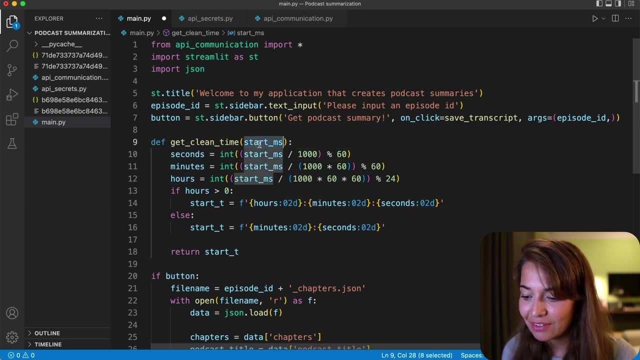 and there is already a function that can do that. Here it is. I need to, you know, work on it for a long time. basically, you get the milliseconds and when you get the milliseconds, you can get the seconds out of it. how many seconds? 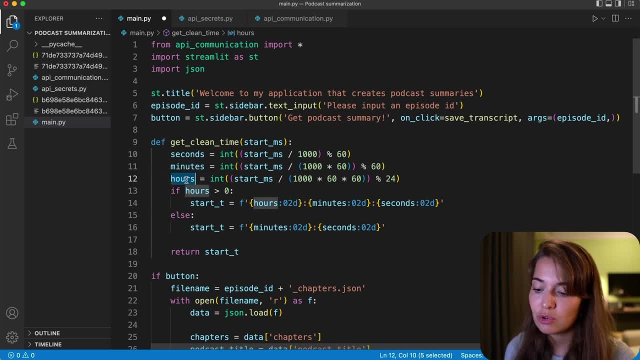 there are, how many minutes there are and how many hours there are. So basically, you're counting the hours, and everything that is on top of the hour is mentioned as a minute if it doesn't add up to an hour and everything that does not add up to a minute. 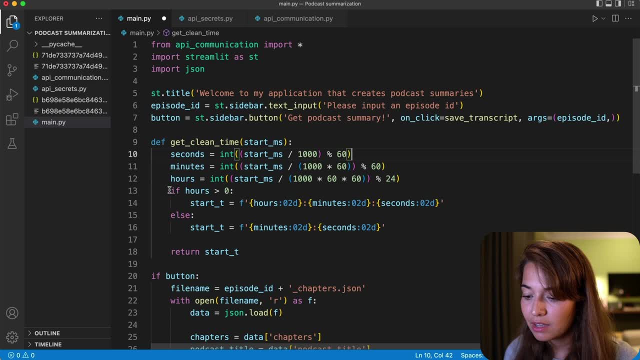 is pointed out as seconds, And here is what we will return. So we'll say the start time is either hours, minutes and seconds. So we'll say the start time is either hours, minutes and seconds. So we'll say the start time is either hours, minutes and seconds. 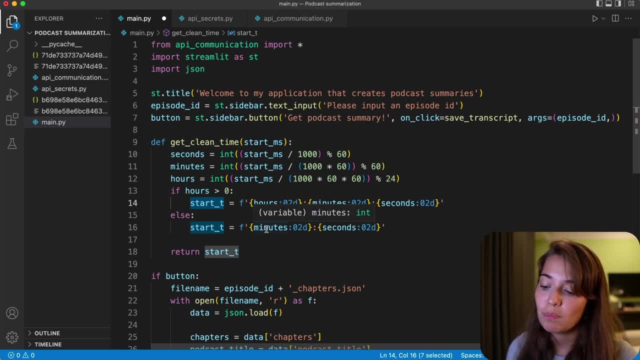 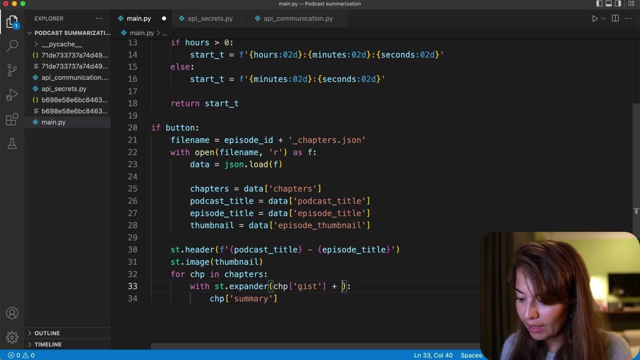 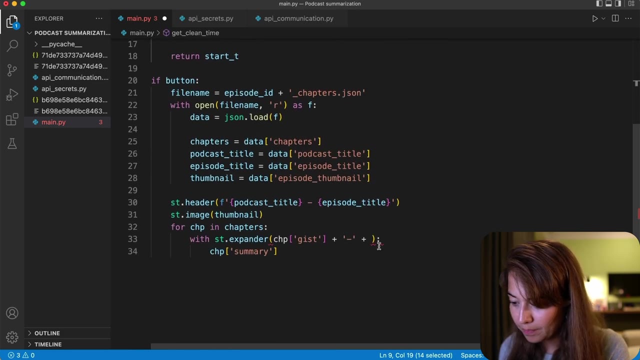 And if there is no hours, we don't have to say zero, something, something. So just show minutes and then seconds. And how I'm going to show it is within the expender title And I can, you know, show it with a dash in between. I'll say: get clean time. 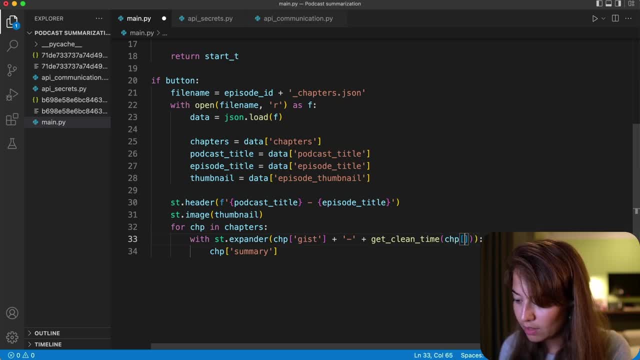 And in there, what I want is a chapter start. let's see what it was. it is just just start. okay, All right, let's run it one more time and then see what our application looks like. Awesome, Okay, this is our application. 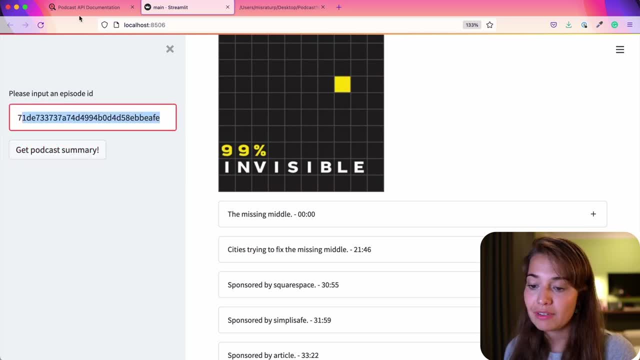 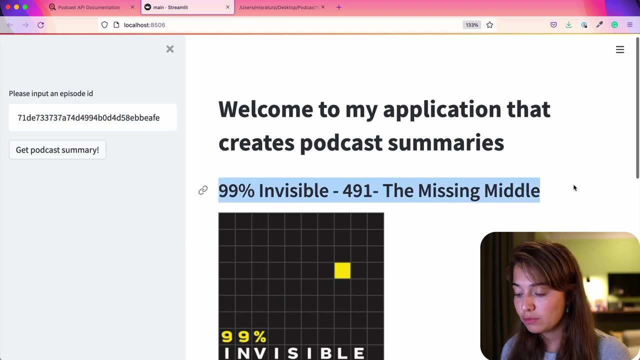 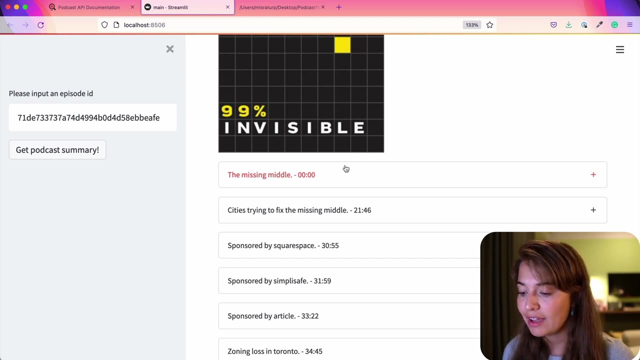 On the sidebar we can input a episode ID that we get from listen notes. we can say: get podcast summary. it will show a nice title. title of the podcast. title of the episode, show us a thumbnail of this episode And for each chapter we show the gist of the chapter, kind of like a headline. when 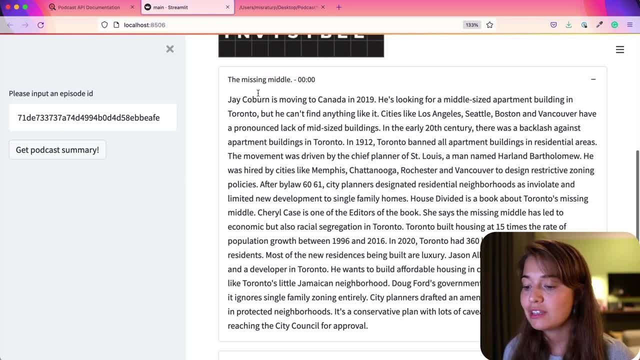 this chapter started, And when you click the expender, when you expand it, you get the summary of the chapter. So that's what we're going to do here. So let's go ahead and run it one more time. I hope you enjoyed this chapter. 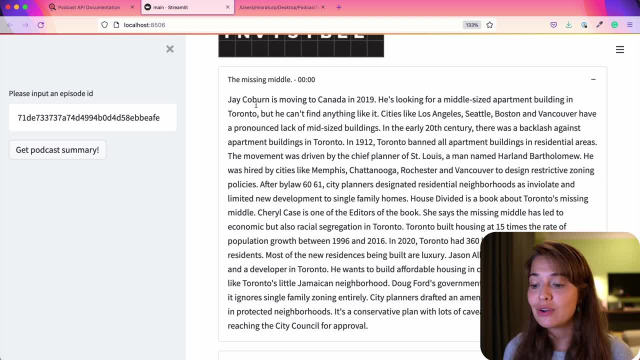 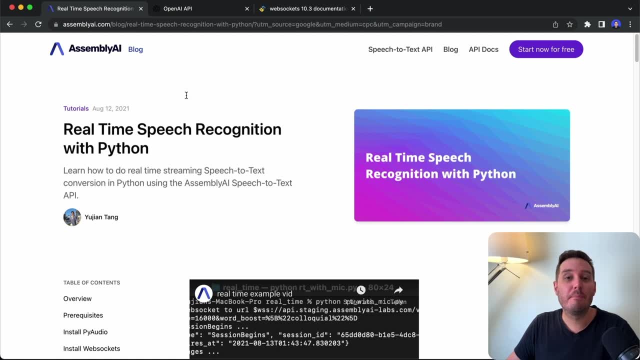 So this is what we set out to do, and we achieved it. I hope you were able to follow along again. don't forget to go grab the code from the GitHub repository. Welcome to the final project And this one. you will learn a bunch of new, exciting technologies. 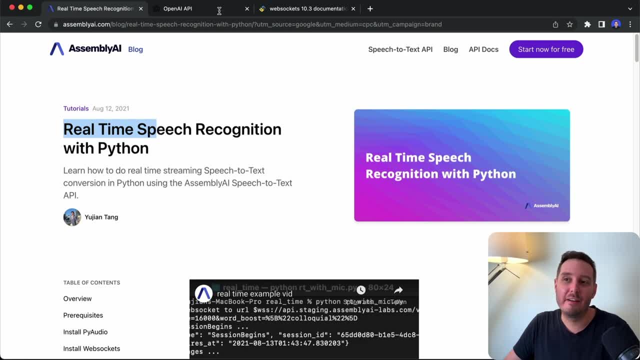 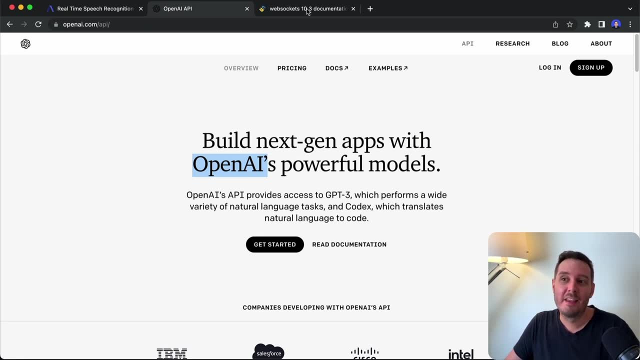 First of all, you will learn how to do real time speech recognition in Python. then you will learn how to use the open AI API and build a virtual assistant or chat bot. And finally, you will learn a little bit about WebSockets and how to use async IO in Python. 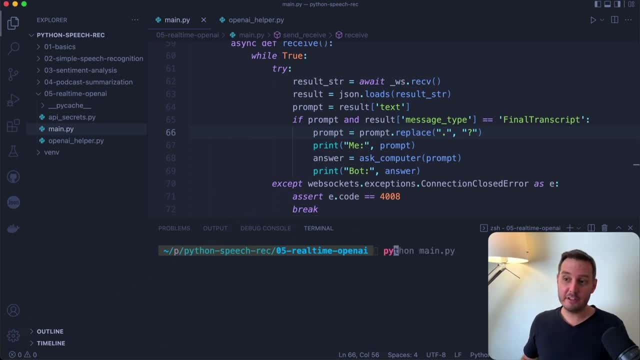 and how to use the open AI API to create a chatbot. So I think this is going to be really fun And first of all, let me show you the final project. So now, when I run the code, I can start talking to my bot and ask questions. 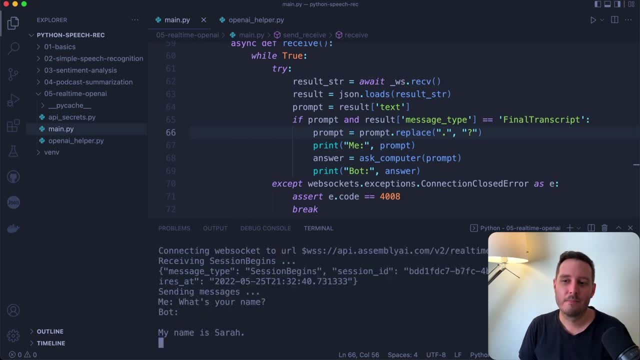 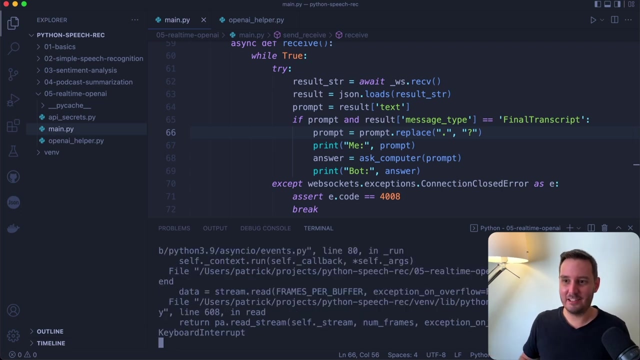 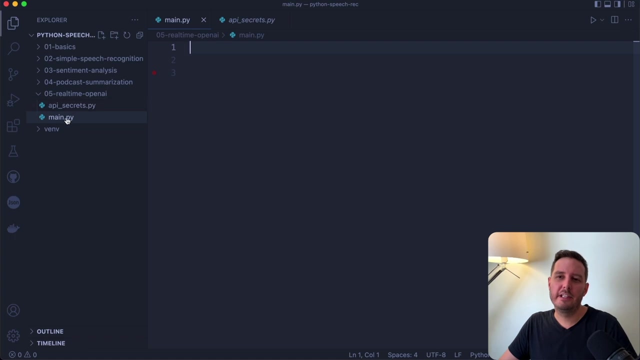 What's your name, How old are you, What's the best ice cream? And you see, this works. So I think this is super exciting. So now let's get started. All right, so here I have a new project folder, And again we have our API secrets file. 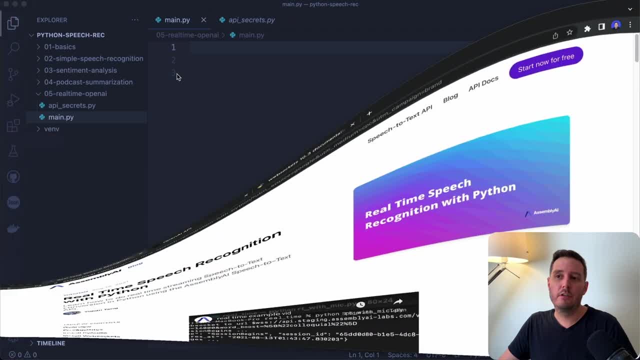 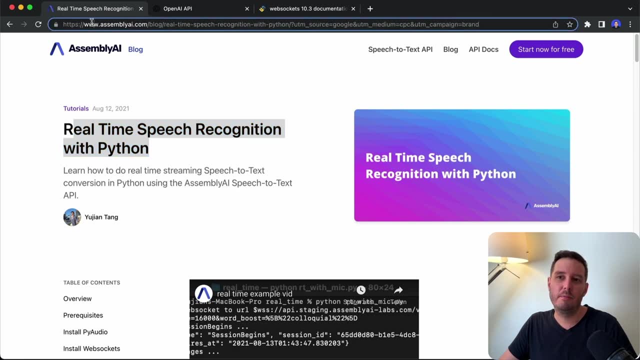 and now a new mainpy file, And the first thing we're going to do is set up real-time speech recognition, And for this we have a detailed blog post on the assembly AI blog. This will walk you through this step by step. 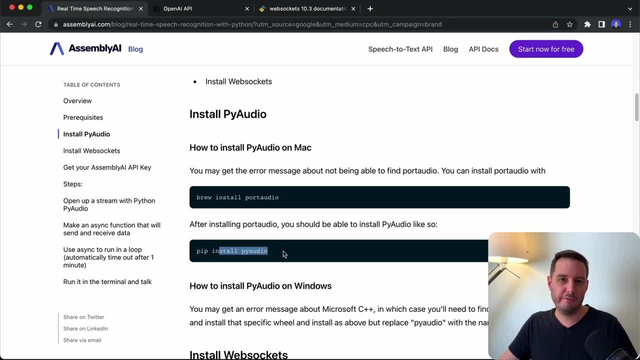 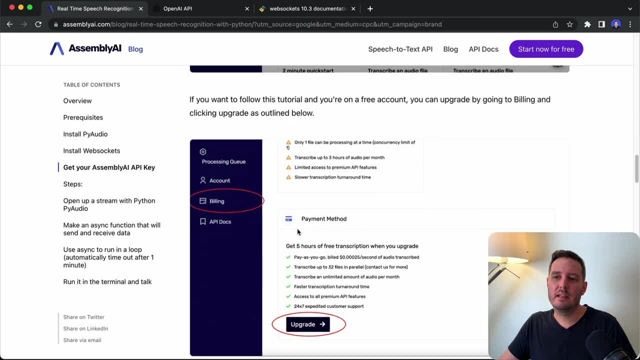 So first of all we need PyAudio to do the microphone recording. So this is the very same thing that we learned in part one. Then we use WebSockets And then we use the assembly AI real-time speech recognition feature that works over WebSockets. 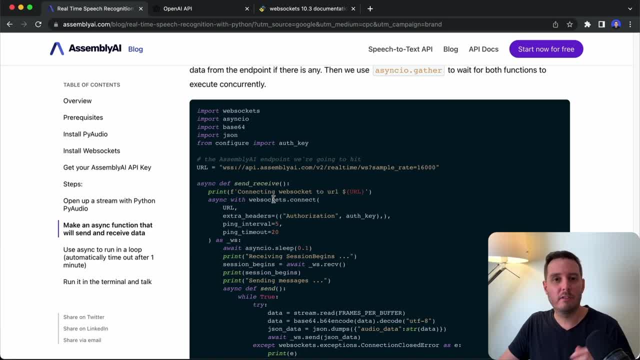 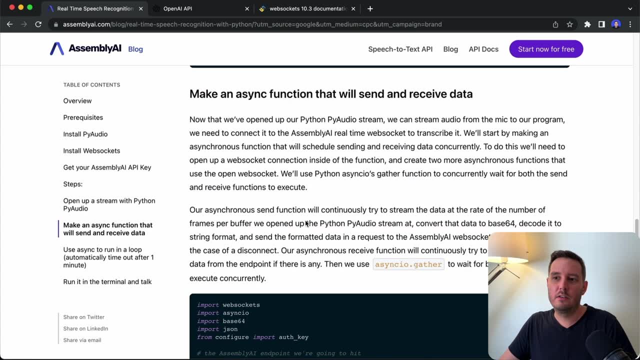 And then we create a function to send the data from our microphone recording and also a function to receive the data, And then we can do whatever we want with this. So, but in order to just copy and paste this, let's actually code this together. 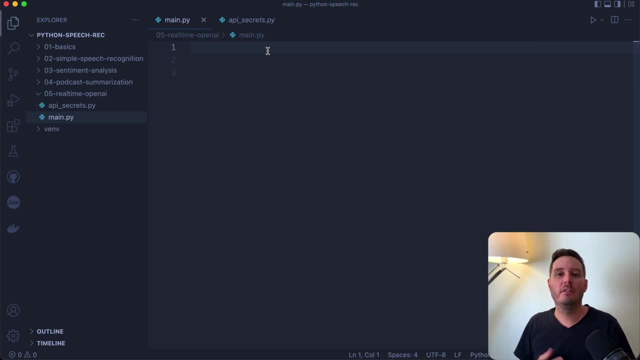 So let's get started. One note here: in order to use the real-time feature, you need to upgrade your account though. So yeah, but anyway, let's get started. So let's import all the things we need. So we want PyAudio again. 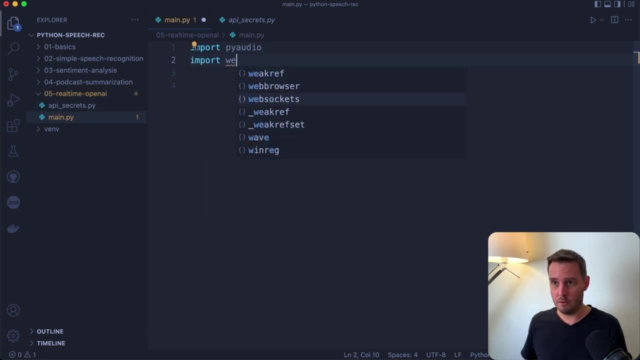 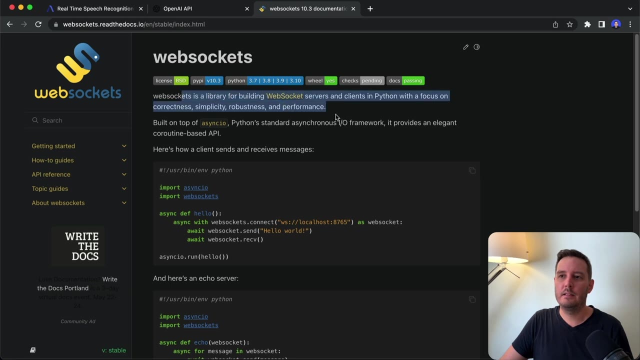 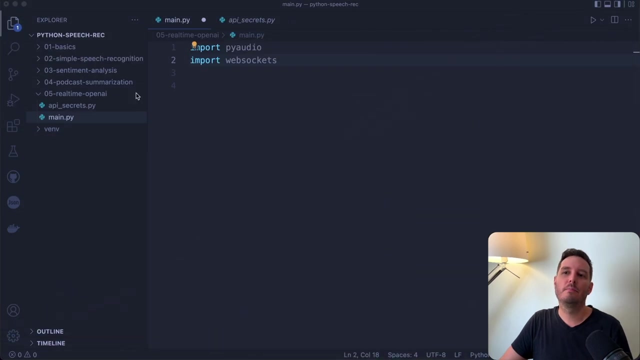 Then we need WebSockets. So we say: import WebSockets And this is a third party library that I showed you in the beginning that makes it easy to work with WebSockets, And this is built on top of async IO. So now we're going to build. 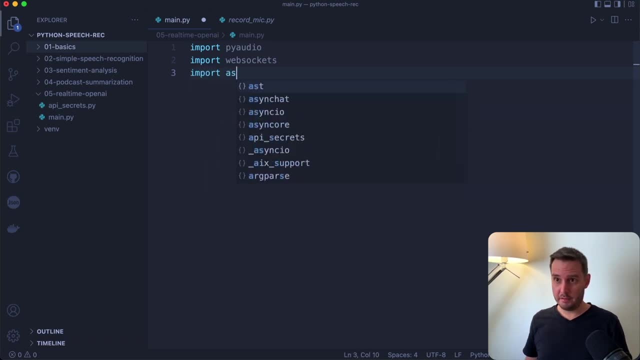 an async code, Then we also import async IO. We also import base64.. So we need to encode the data to a base64 string before we send this And then we import JSON to receive the JSON result And then we say: from API secrets. 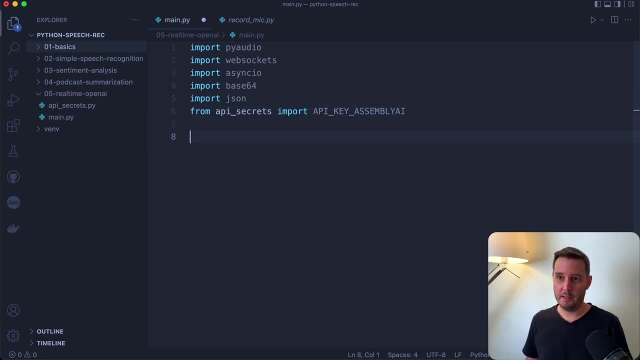 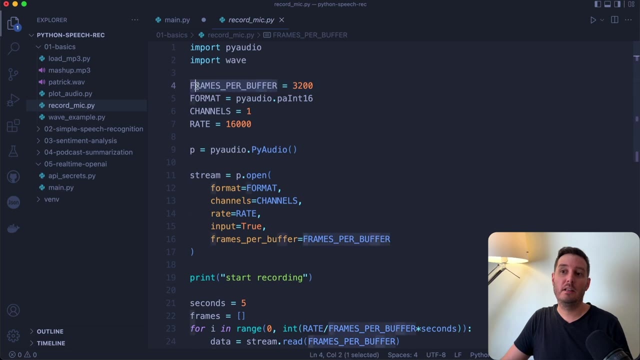 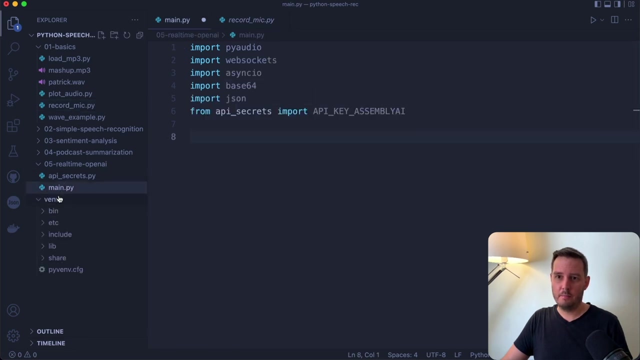 we import our API key from assembly AI, And now the first thing we set up is set up our microphone. So for this we use the exact same code that we learned in part one. So I simply copy and paste this part from here: 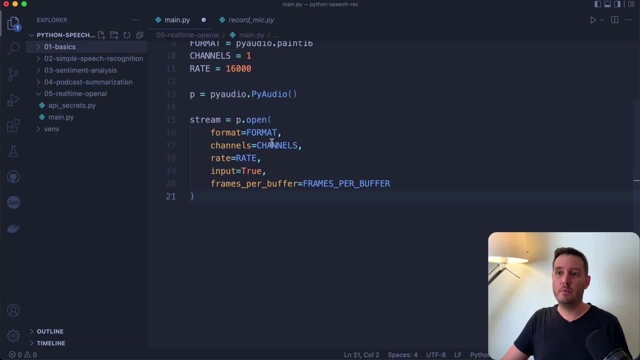 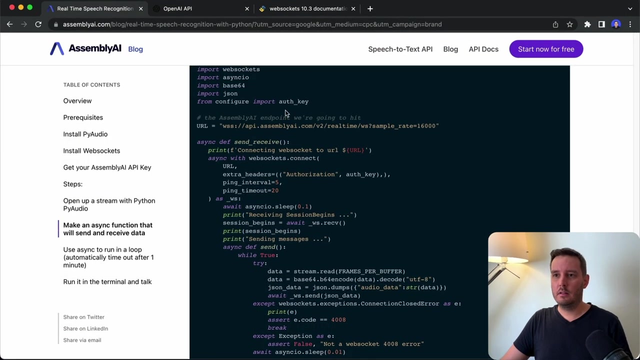 So let's copy and paste. So we set up our parameters, then our PyAudio instance, and then we create our stream, And now we need to define the URL for the WebSocket, And we can find this on the blog post: home post. 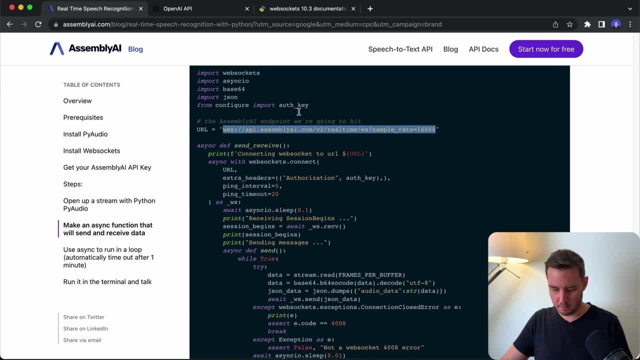 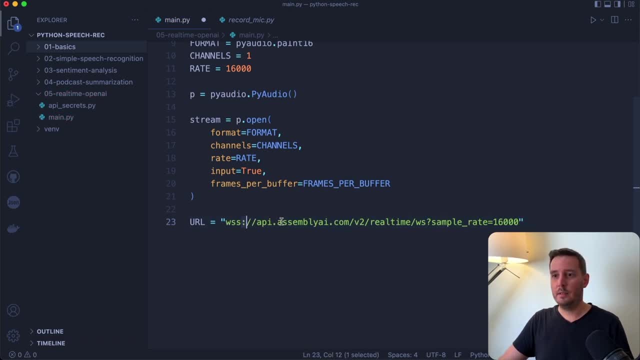 So here I can copy and paste the URL. So the URL is at WebSockets and then assemblyaicom and then real time, And then the last part is also important. So here we say: question mark: sample rate equals 16,000. 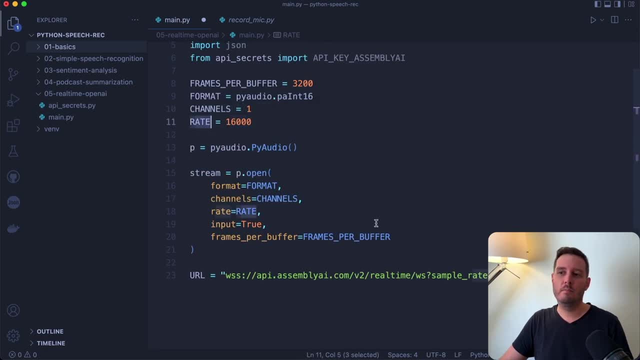 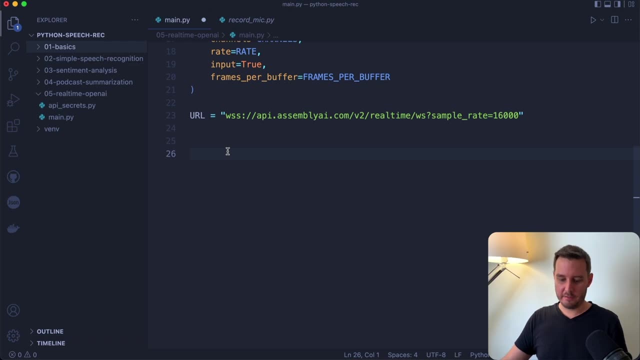 So this is the same rates that we use here, So make sure to align this with what you have. And now we create one function to set up. So we use a available function here, which is send and receive the data, And this is a async function. 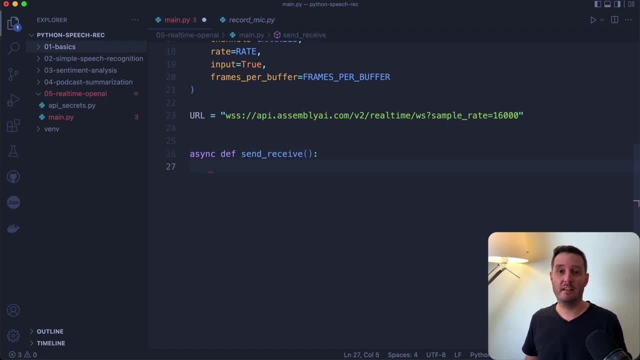 So we say async- def and we call the send received. So this is responsible for both sending and receiving the data. And now we connect to the WebSocket and we do this with a async context manager. So again we say async, and then with 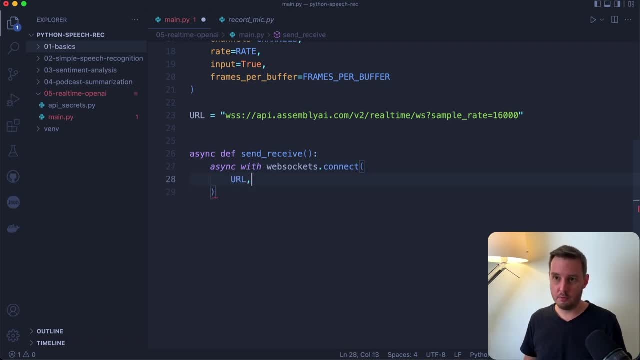 and then WebSockets dot, connect, And now we specify the parameters, your L, Then say send, then we say a, we set a ping timeout, And we can set this to 20.. For example, then we want a ping interval and this should be five. And then we also need to send our authorization token. 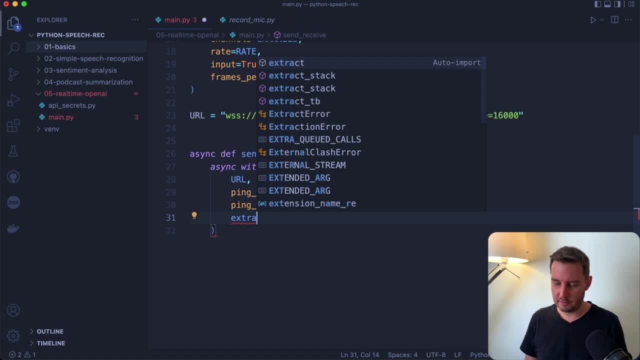 So the key or the parameter for this is extra headers, And this is a dictionary with the key authorization and the value is our token, And then we say async with s and then we can call this what we want. So I say underscore w s for WebSocket, Then first we wait to let this connect. 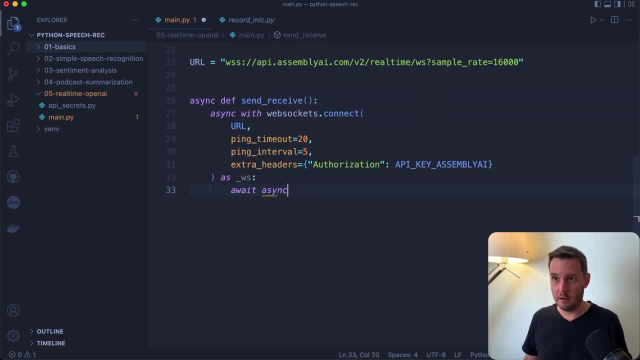 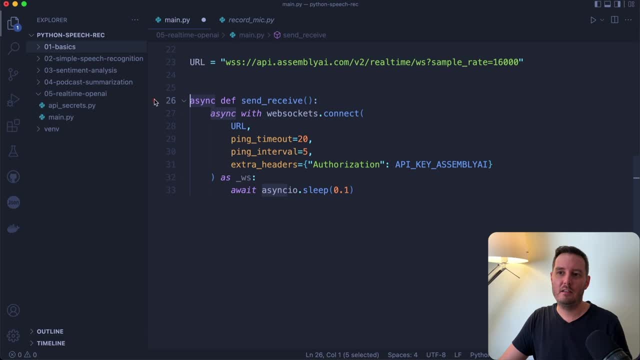 use time with sleep. So we are inside a async function, So we have to use the async sleep function, And then we wait, or we we try to connect and wait for the result. So we say session underscore begins equals, and then again a wait underscore w s, And then this is called r e s. 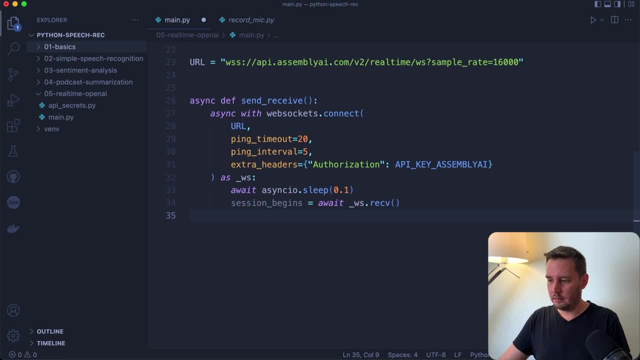 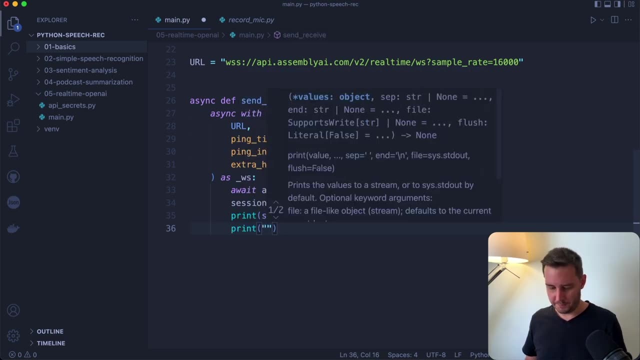 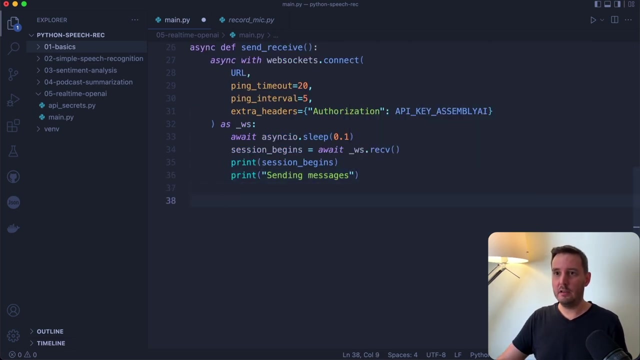 v for receive, I guess, And then we can print the data and see how this looks. Let's also print sending messages, And now we need two inner functions. So again a async function. so we say async death send, And for now we simply say pass, And then we say async. 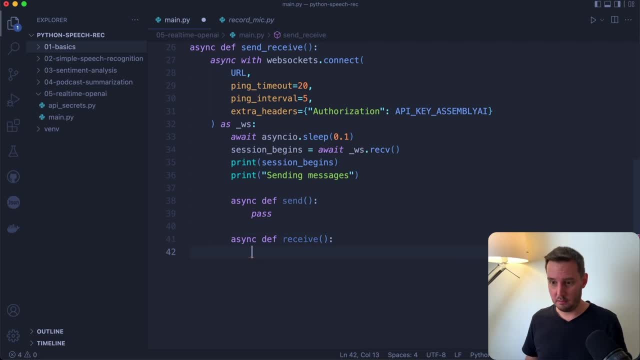 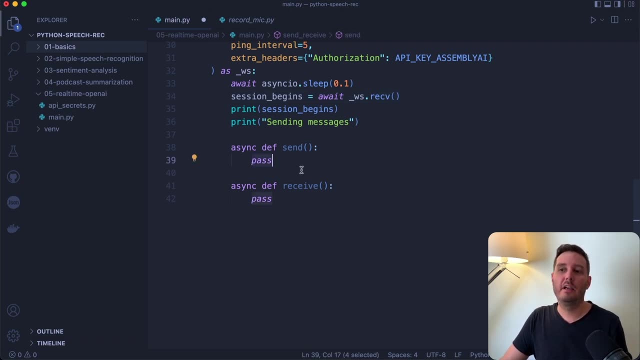 death receive. And here also we pass. And actually these are both. these: both will have a infinite while true loop, So they will run infinitely and listen for incoming data. So here we say while true, And for now let's just print sending. And here we also say while: 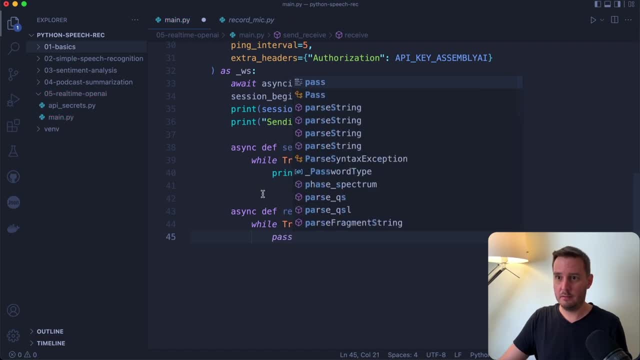 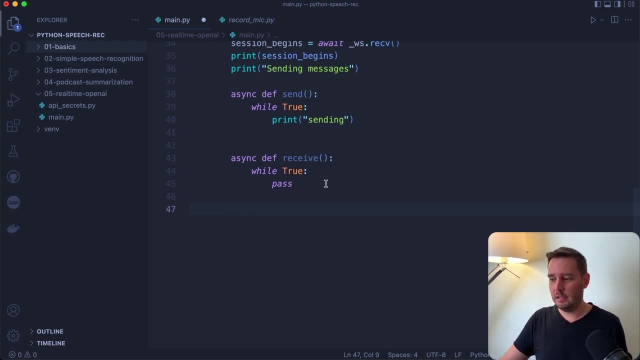 true, And here we simply pass. So I don't want to spoil our output. And now, after this, we need to combine them in a async IO ways. So in order to do this, we say we call the gather function, So it's called async IO dot gather. And now here we: gather sent. 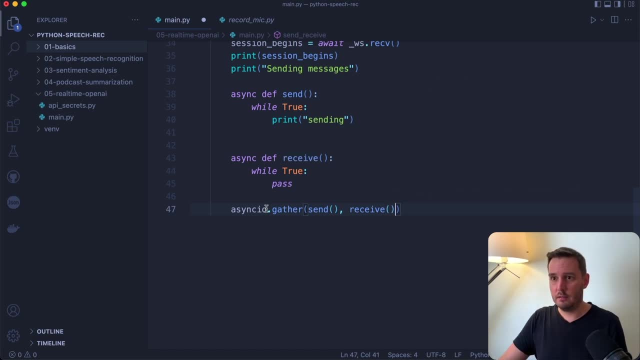 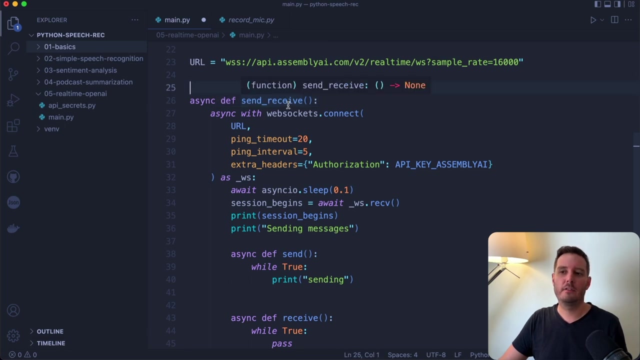 and receive, And this will return two things, So the send results and the receive results. So actually we don't need this, But just in case we have this here And now. after defining this function, of course we also have to run the code, And we have to run this in an infinite loop And in. 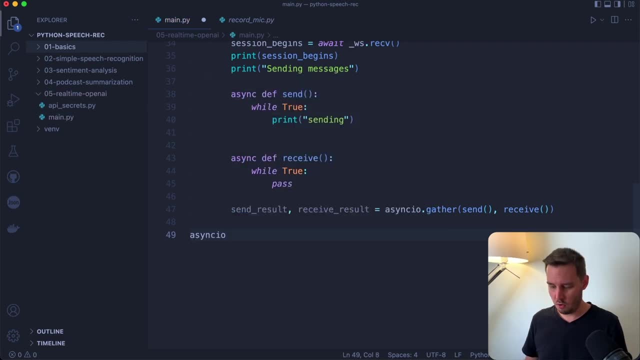 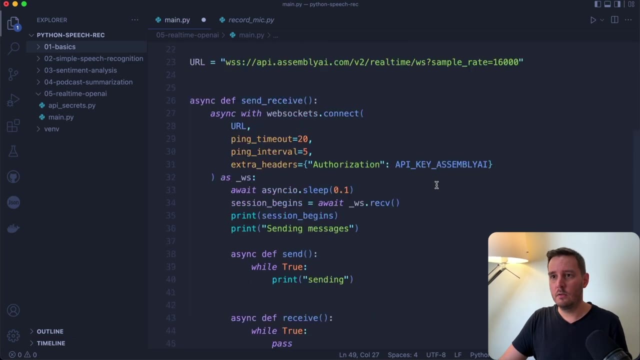 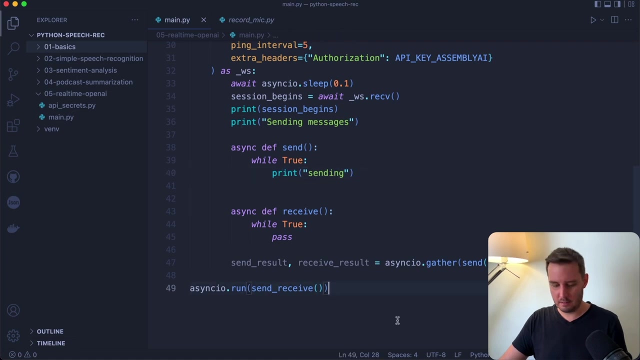 to do this. we call a sync IO and then dot run and then our send receive function. So now this should connect and then should print sending all the time. So let's run this and hope that this works. So yeah, it's already connected and sending work. So you see, that's why. 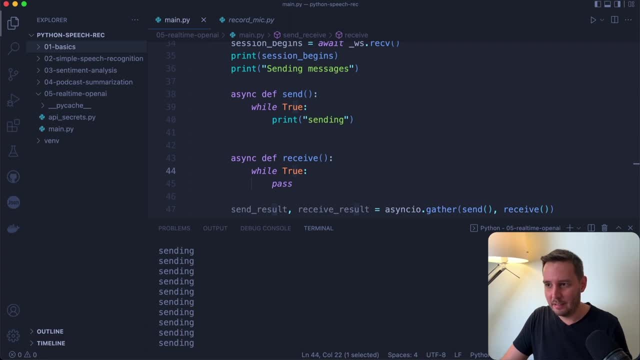 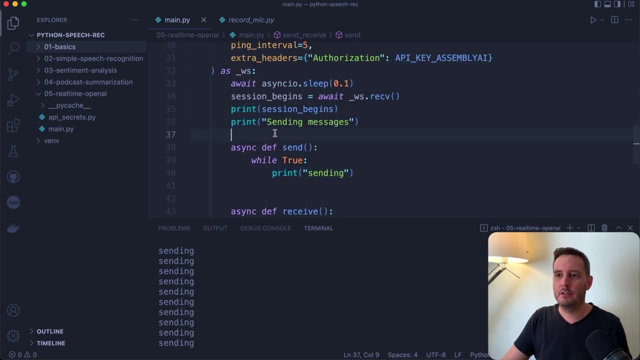 I didn't put the receive in here as well. So we get a lot of outputs And, yeah, I can't even scroll to the top anymore. But basically, yeah, it should have printed this once And then. now this is working so far, So we can continue implementing these two functions now. So now let's implement. 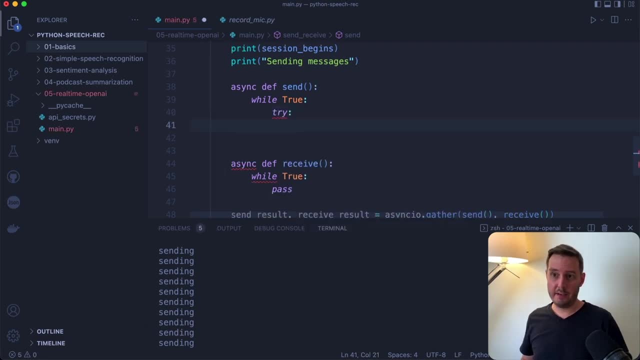 the send function first And we wrap this in a try except block, And now we read the microphone input. So we say stream dot reads, and then we specify the frames per buffer. And I also want to say exception on overflow equals false. So sometimes when the WebSocket connection is too, 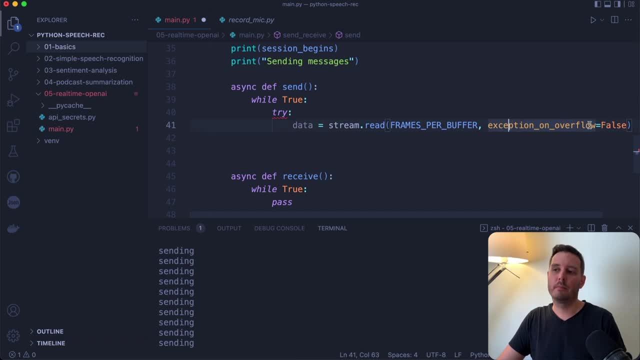 slow, there might be an overflow, And then we have an exception. but I don't want this. it should still work. And then we need to convert this or encode it in base 64. So we say base 64, B 64.. 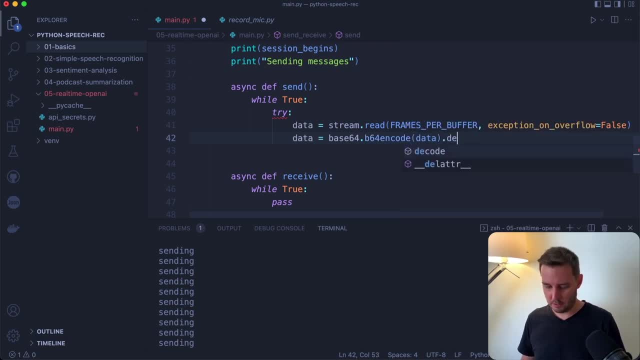 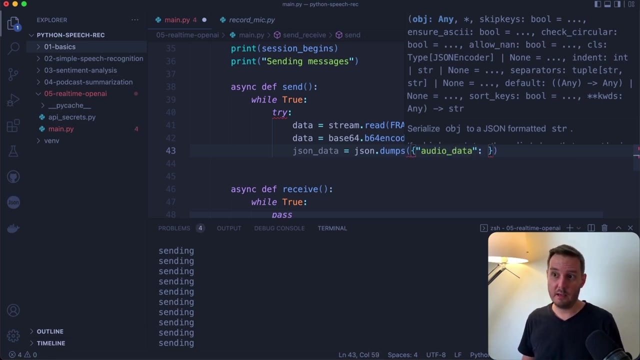 encode our data and then we decode it again in utf Eight. This is what assembly AI expects. then we need to convert it to a JSON object. So we say JSON dump s, And then this is a dictionary with the key audio data. So again, this is what assembly AI needs. And then here we put in the 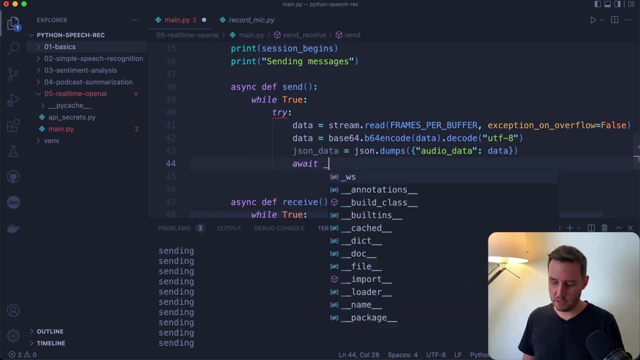 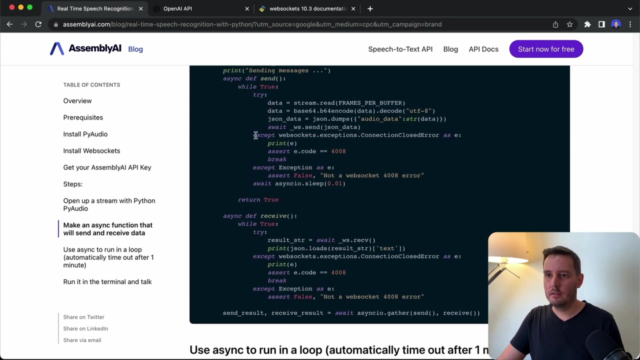 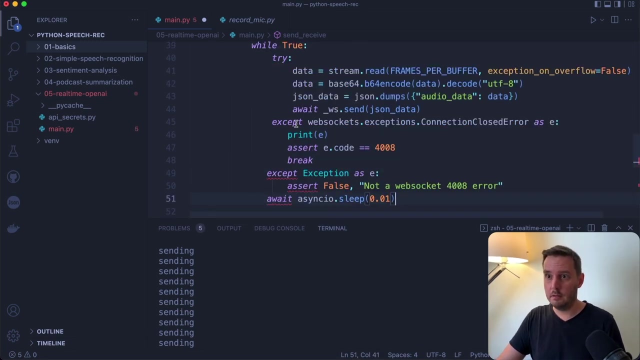 data And then we send this and we also have to await this. So awaits W s send the JSON data and then we have to catch a few errors. So let's copy this from our blog post. So these ones, let's copy and paste this in here. So we accept a WebSockets exceptions connection closed. 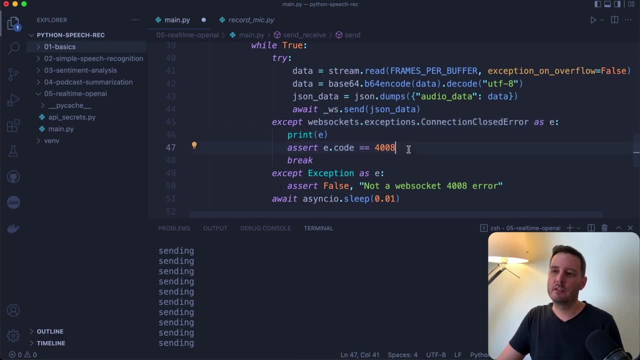 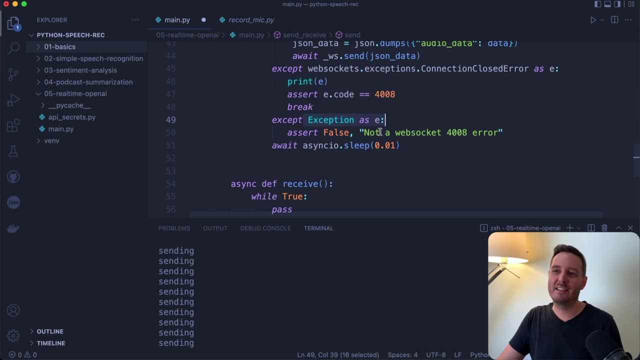 in command, And then we are going to make sure that our users have a Independent world that we can then build on here, so that we can also create an error here- I am not going to code here- And then we are going to pass it. let's see if we can. 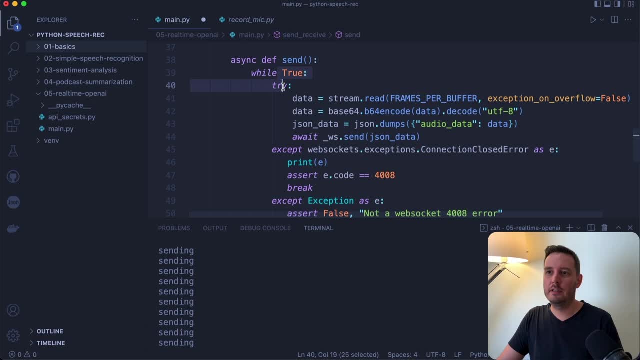 or we can just write it and then we are going to remove this error. we will name it error, Then we print the error, then we make sure it's of this code and then we also break And then we catch every other error. So it's not best practice to do it like this, But it's fine for this simple tutorial. 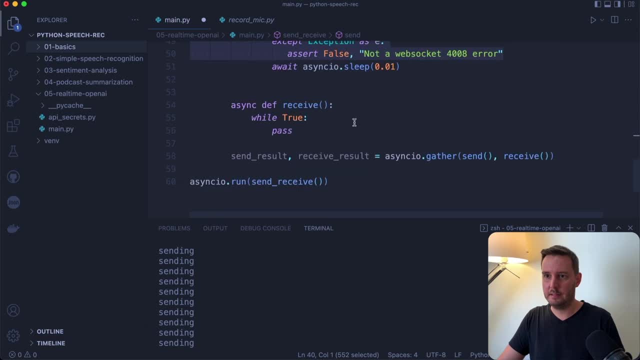 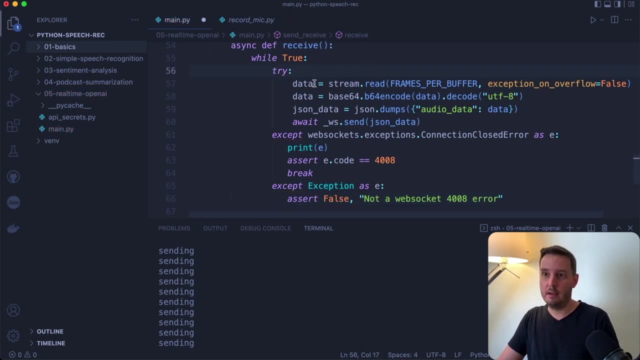 And then we assert here, and then after each while- true iteration, we also sleep again. And yeah, so now we can copy this whole code and paste it into a JavaScript. And then we have our error and we have code and paste it into this. So the code is very similar here, So we have the same try. 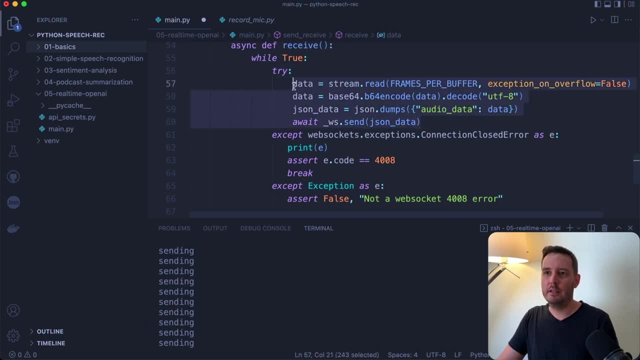 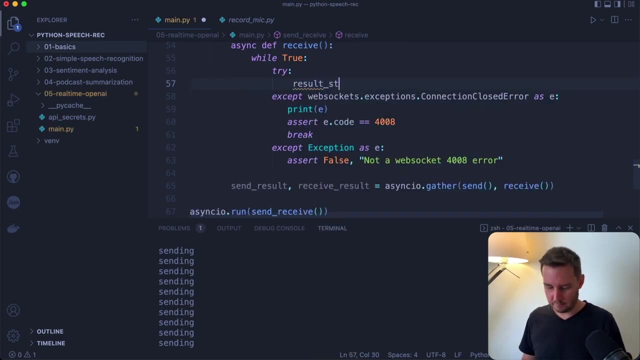 except. but now here of course we have to wait for the transcription result from assembly AI. So we say: result, string equals, and then again we wait, and then the w s r e s v. then we can convert this to a dictionary by saying: results equals json dot load from. 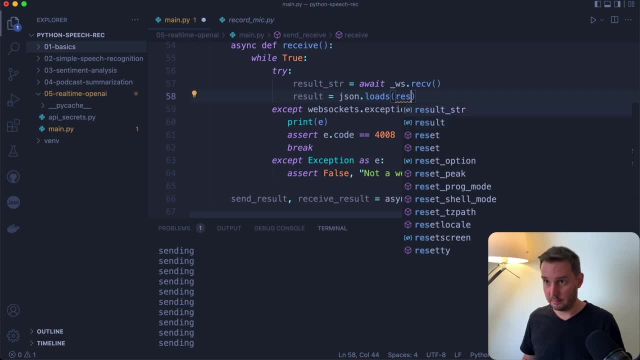 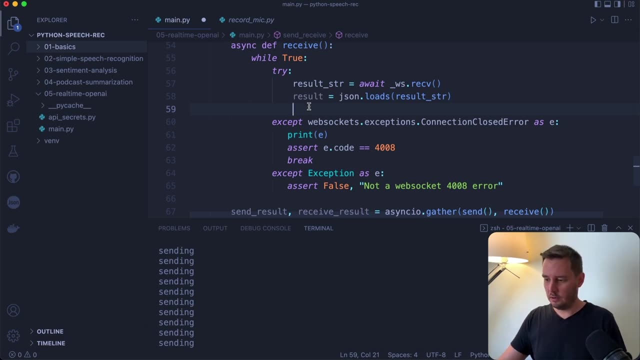 a string and here the result string, And now this has a view. So this is a JSON object. or now you are doing, you're doing something, Now just precisely the check. So this is an Python, it's a dictionary, So now we can check a few keys So we can get the prompt. or actually now 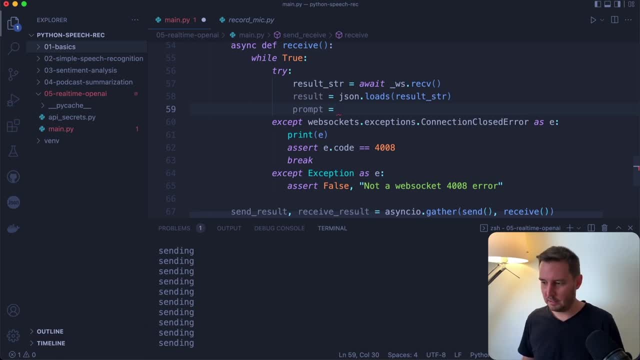 this is the transcription of what we said. So we say prompt equals results, and then it has the key text And it also has a key that is called message type. So now we check if we have a prompt and if the results and then the key message underscore type. And now this should be final transcripts. 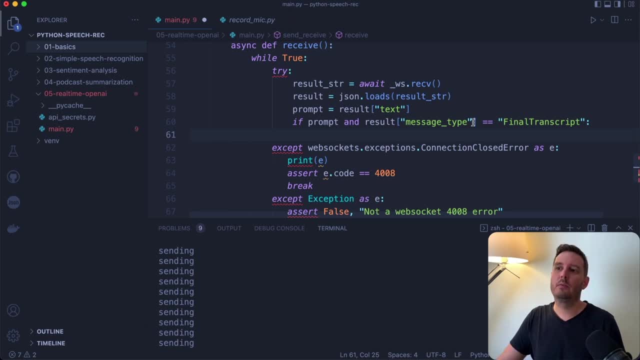 And now what assembly is doing? it will, while we are talking, it will already start sending the transcript, And once we finished our sentence it will do another pass and make a few small corrections if necessary, And then we get the final transcript. So we want only the final. 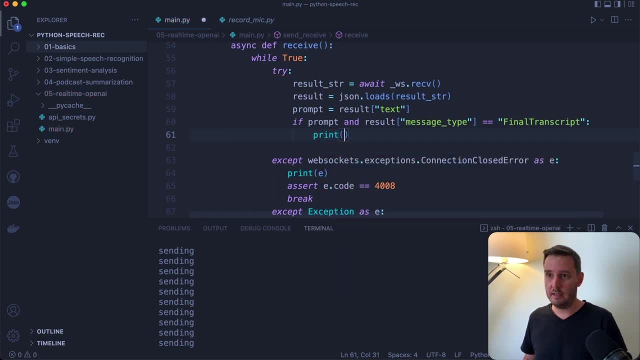 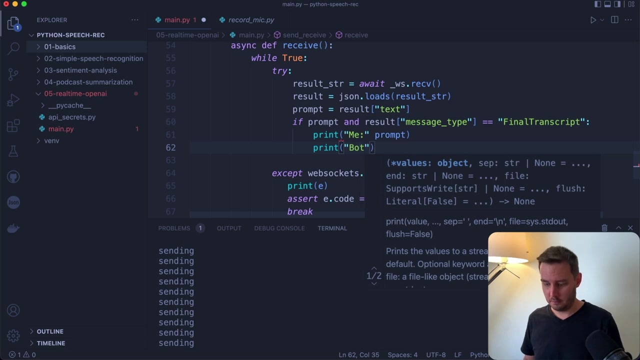 transcripts. And now, for now, let's print me, and then let's print the prompt. And now we want to use our chatbot. So now let's print bots And then let's. for now, let's simply print, Let's print a random text for now, And then we set up this in the next step. But first I want to 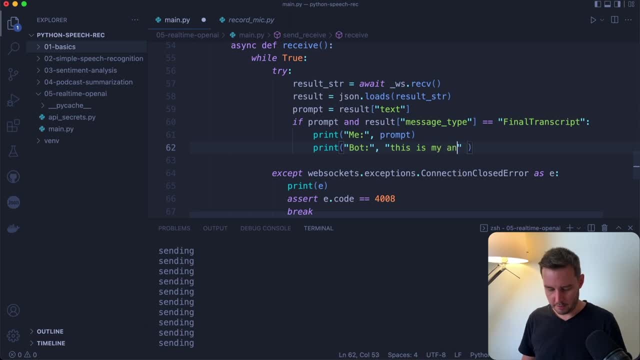 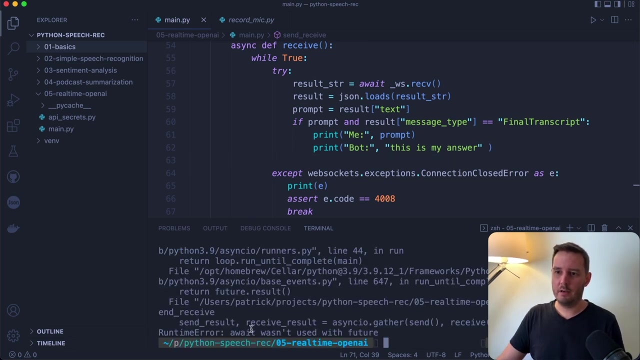 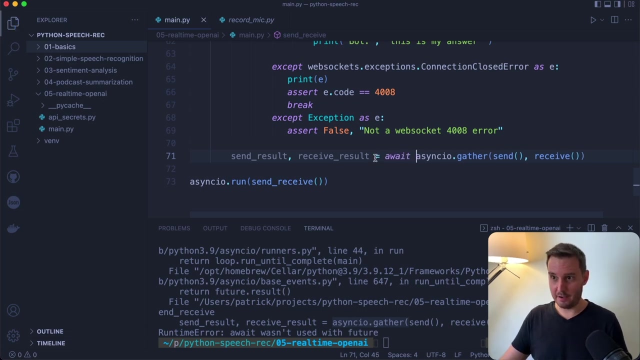 test this. So let's say: this is my answer And this is all that we need for the receive functions. So let's clear this and run this and test this. Oh, we get an error. await wasn't used with future async IO gather. Oh, this is a classic mistake, Of course. here I have to say await. 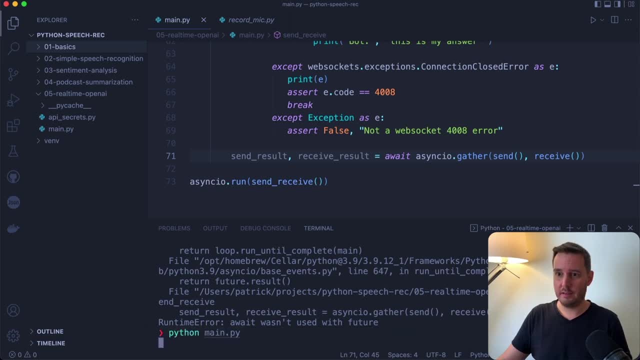 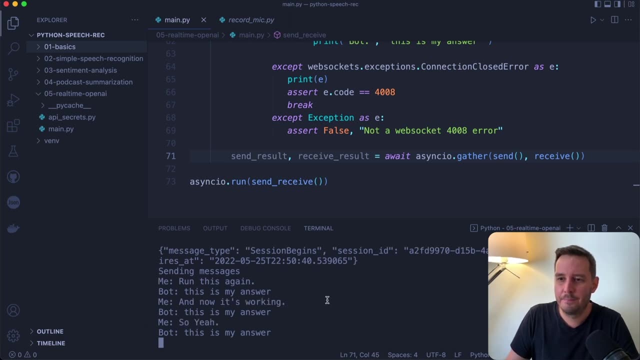 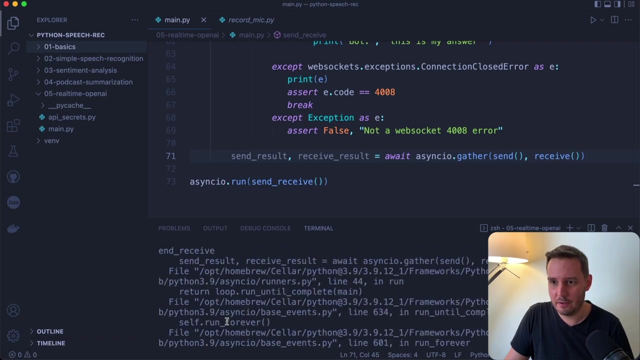 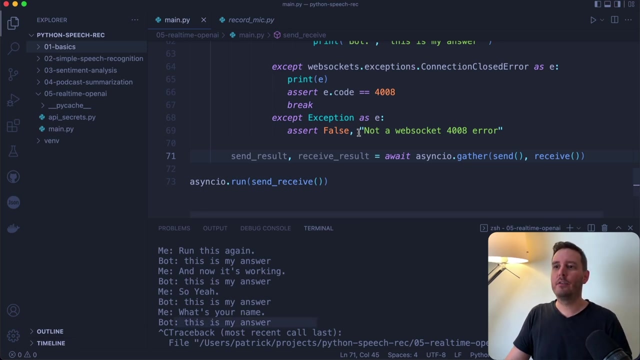 Async IO gather. So let's run this again. And now it's working. So, yeah, what's your name? And you see the transcript is working. So now I stopped this. But if I scroll up what's your name, and each time we get this as my answer. So this is working. And now, of course, here we want to do a. 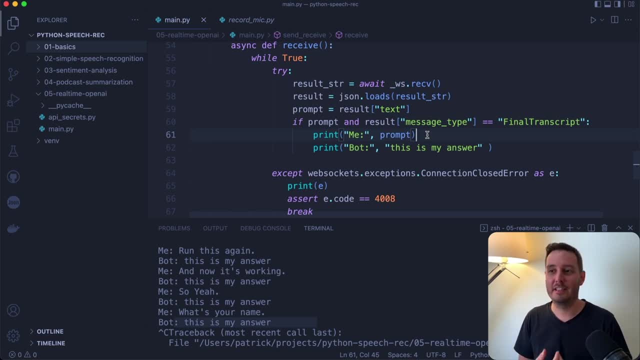 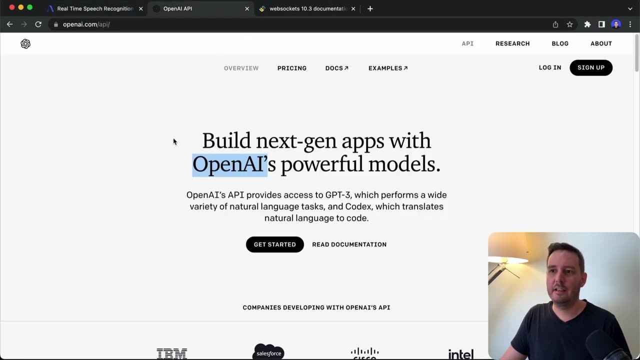 clever thing with our prompt and use our virtual assistant. So for this we now set up open AI, So they have an API that provides access to GPT three, and this can perform a wide variety of natural language tasks. So in order to use this you have to sign up, but you can do. 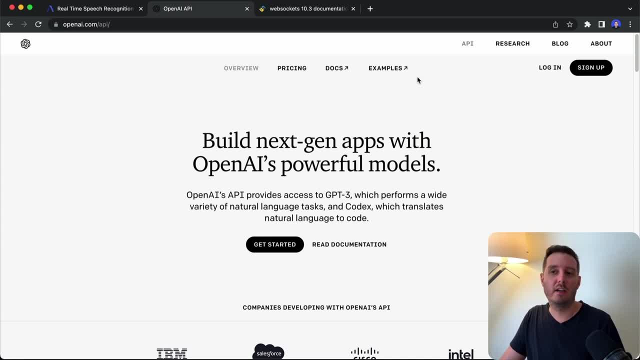 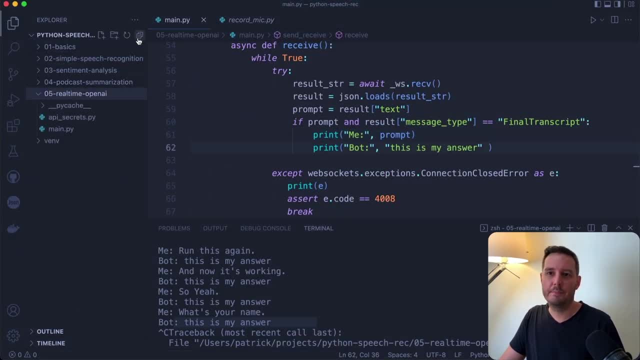 this for free and you get a free. you get free credits. So this will be more than enough. you'll, James Dr ột, to play around with this, And it's actually super simple to set this up, So let's create a new file. 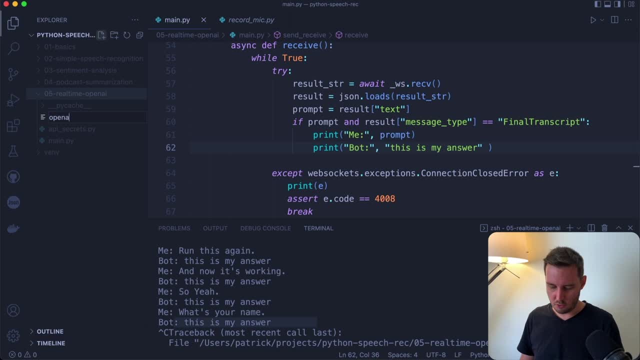 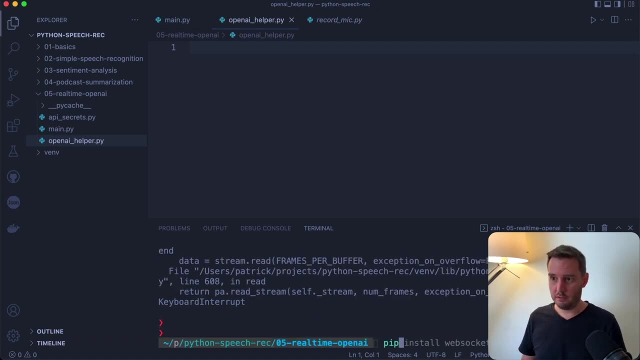 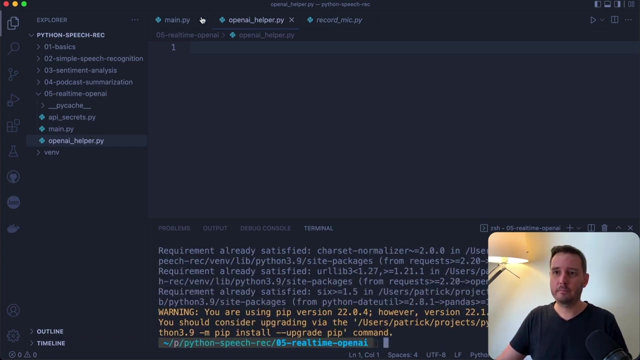 And I call this, let's call this open AI helper dot pi. And then we also have to install this. So we have to say: pip, install open AI. And then we also, after signing up, you get a API token, So we have to copy this in API secrets and then we can use this. And now we 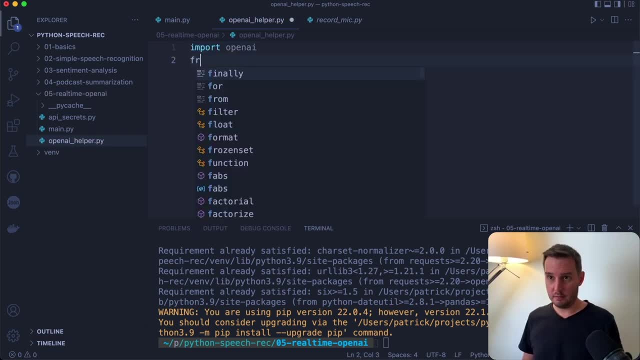 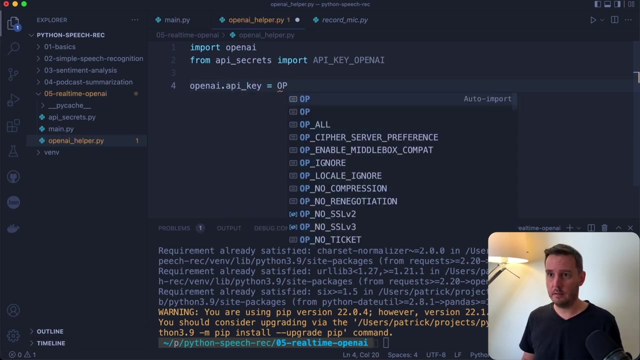 can import open AI And we also need to import our secrets. So from API secrets we import our API key, open AI. then we have to set this. so we say open AI dot. API key equals API key And now we can go to open API. And then we have to set the API key. So we type in a keyword And now we 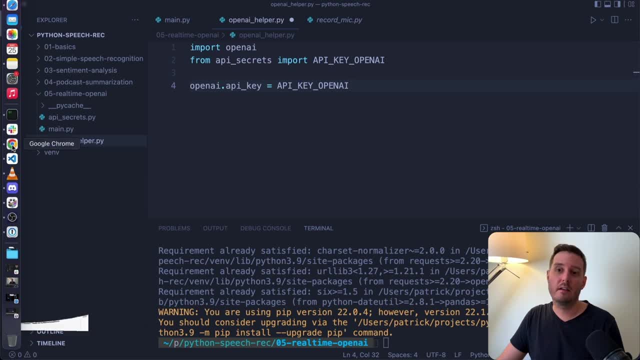 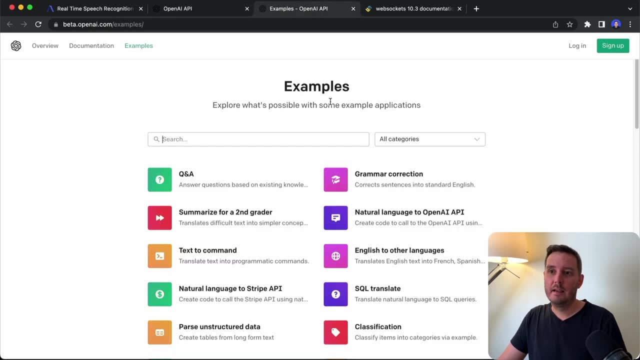 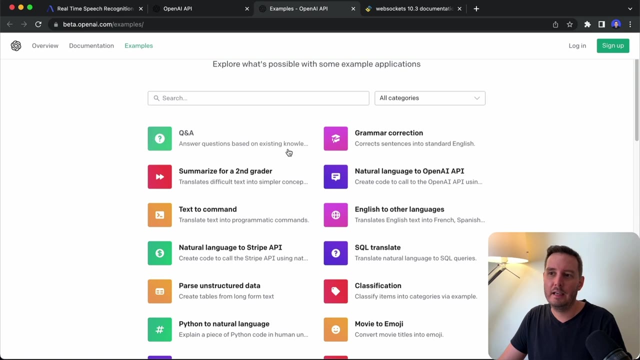 want to do question answering. So the OpenAI API is actually super simple to use. So we can click on examples And then we see a bunch of different examples. So OpenAI can do a lot of things, for example, q&a, grammar correction, text to command classification- a lot of different stuff. 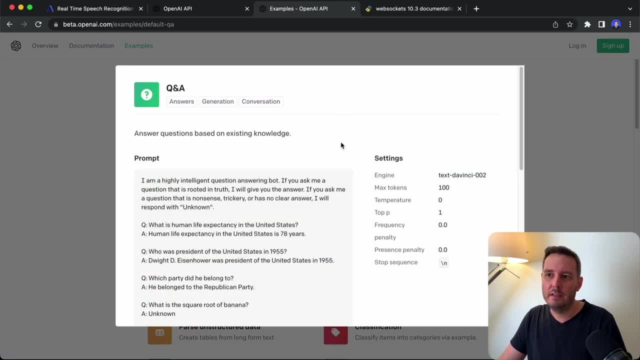 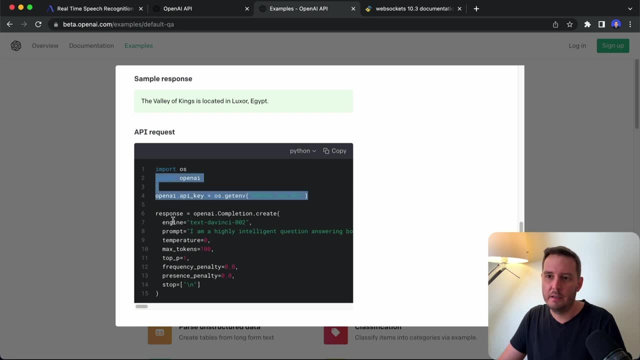 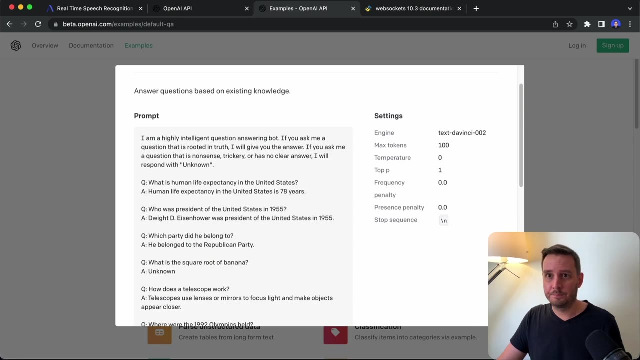 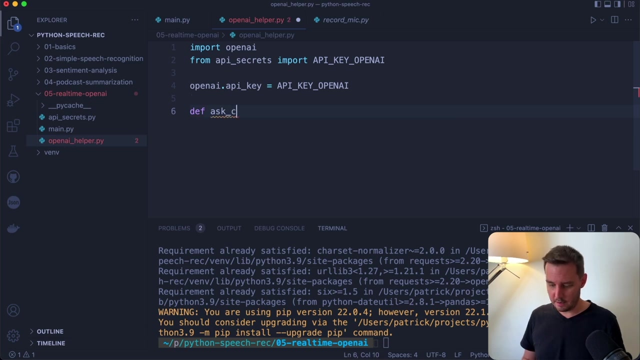 So let's click on q&a And if we scroll down then here we find the code example. So we already set our API key And now we need to grab this And let's copy this And let's create a helper function. So define, and let's call this: ask Computer, and this gets the prompt as input. 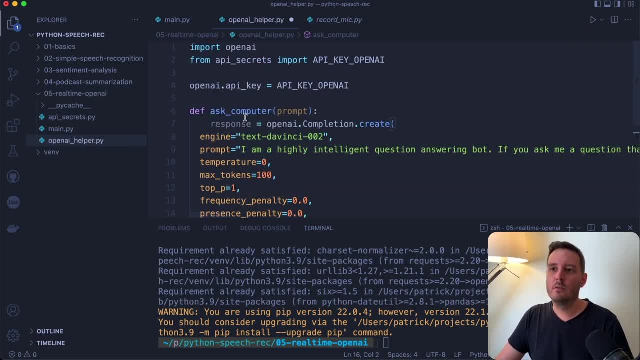 And now we have the answer that says ask, And then we can select the task that we'd like to do, So let's do that, And then we have our initial container that we need to use. So if we click on now, I paste this in here. So we say: a response equals open AI dot completion, dot create. 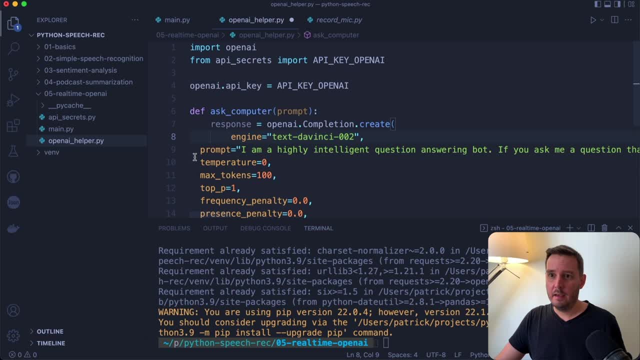 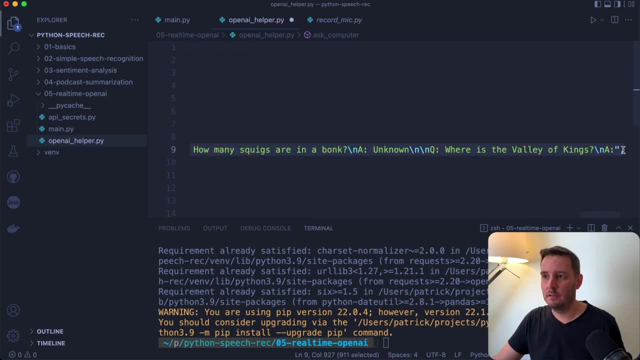 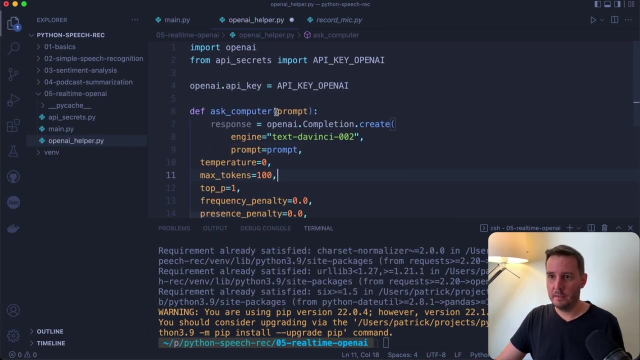 then here we specify an engine, And now we specify the prompt, And in our case the prompt is going to be the prompt that we put in. So prompt equals prompt from the parameter. And now there are a lot of other different parameters that you could check out in the. 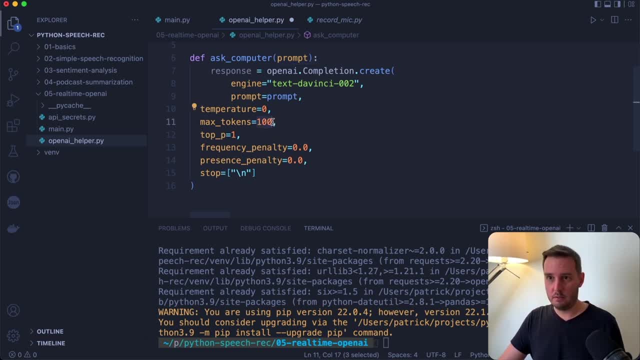 documentation. So in my case, I only want to keep the max token, So this will specify how long the result can be. And yeah, let's say, 100 is fine for this. And now, this is all that we need, And now, of course, we need to return the response, And this is actually a 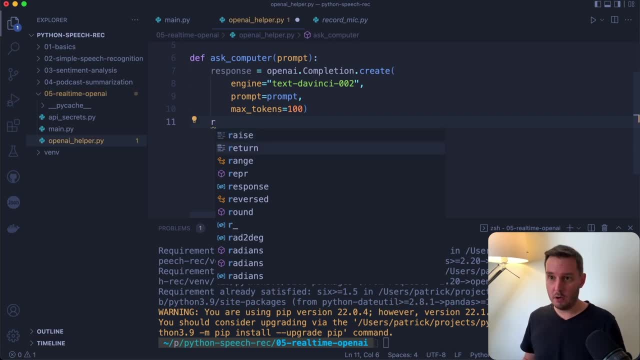 JSON. object: Again or now a dictionary, and we only want to extract the first possible response. So it can also send more, if you specify this here. So in our case we only get one, And then we say response, And this is in the key choices, and then the index zero, So the first. 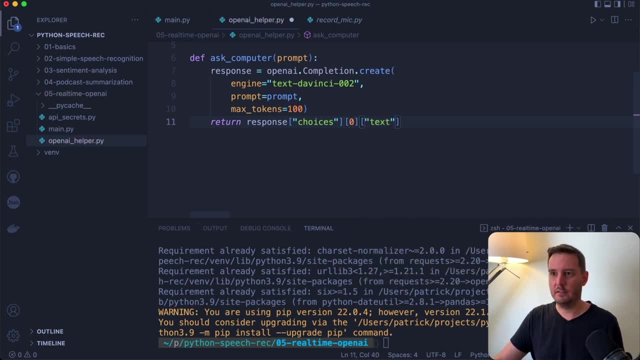 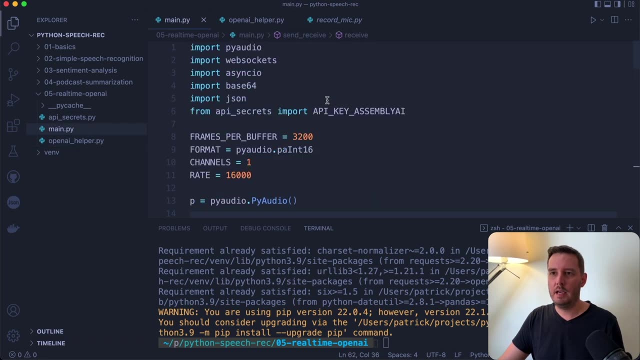 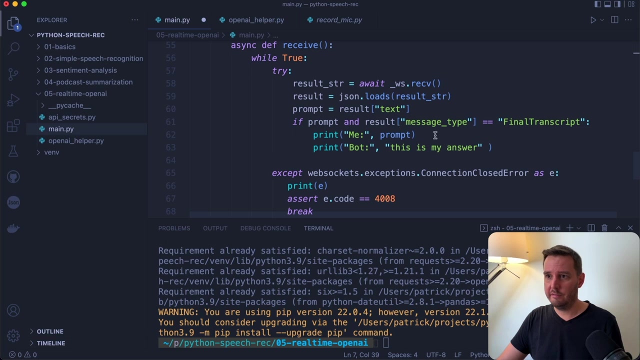 choice and then the key text. So this will be the actual response From GPT three. And now, in the main, the only thing we have to do is say: from open AI helper, we import, ask com pewter, and then down here in the receive functions. And now here we say: 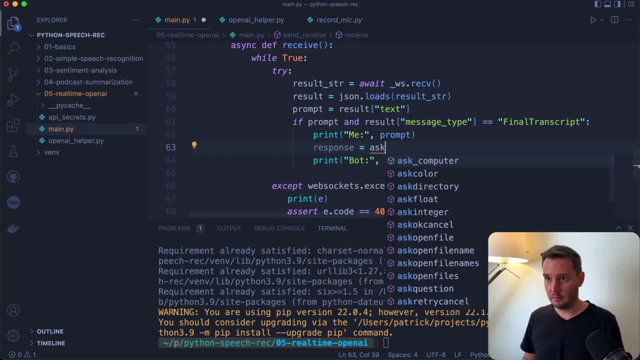 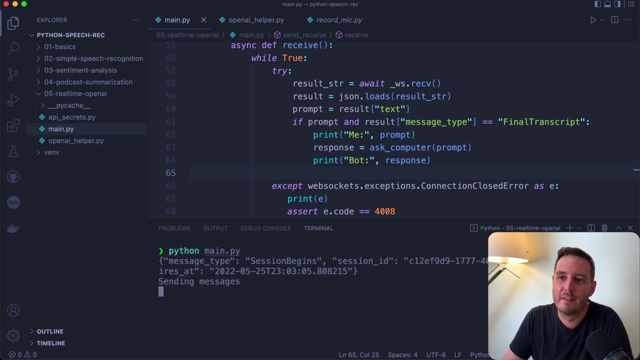 response equals ask computer, and then we put in the prompt And then here this will be our response, And now this should be everything that we need. So now let's again clear this and run the mainpy, And let's hope this works. What's your name? 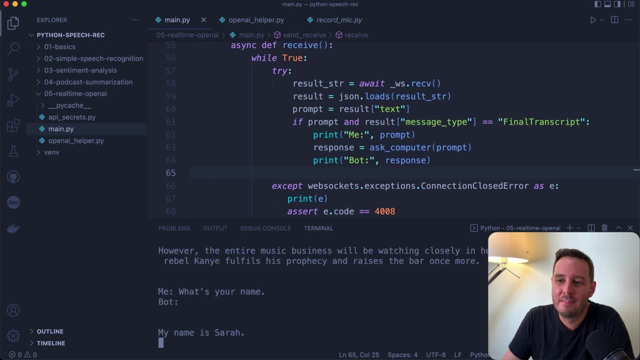 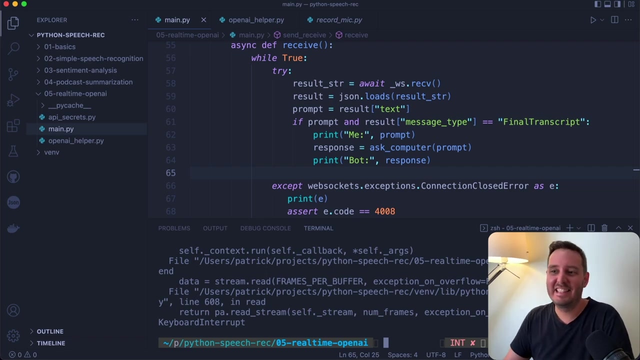 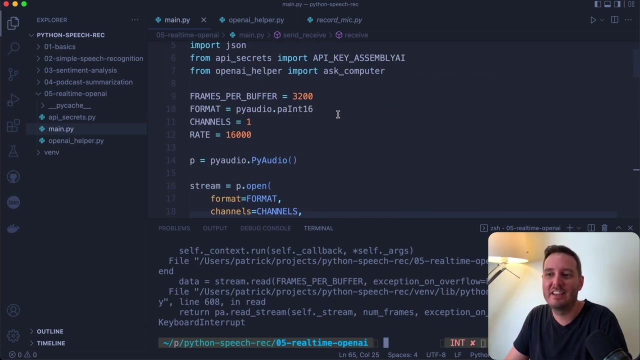 What's your name? How old are you? Where are you from? All right, so let's stop this again. And yeah, you see this works. And this is how you can build a virtual assistant that works, with real time speech recognition, together with open AI. 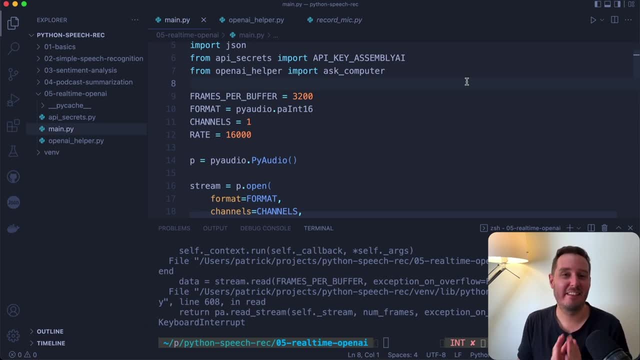 And, yeah, I really hope you enjoyed this project If you've watched this far. thank you so much for following along And also I hope to see you in the future on the assembly AI channel, because on there we also create a lot of content around Pythons. 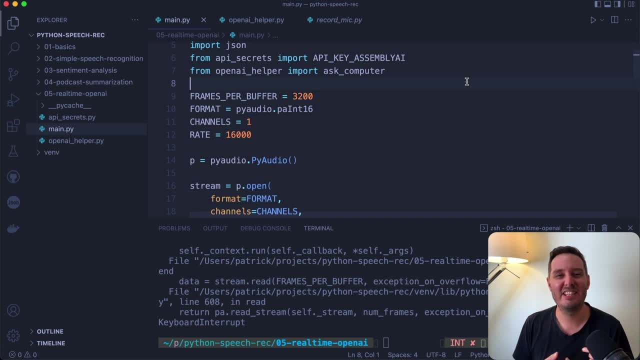 speech recognition and also machine learning. So please check it out, and then I hope to see you soon. Bye. 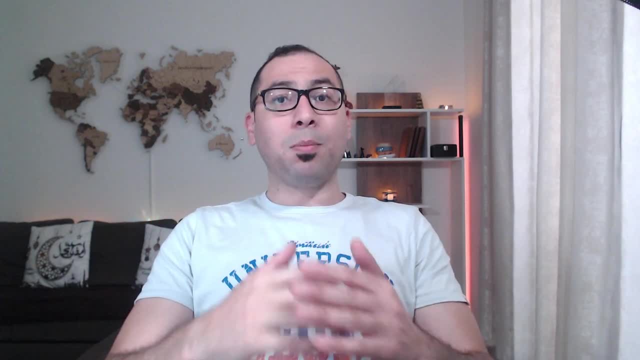 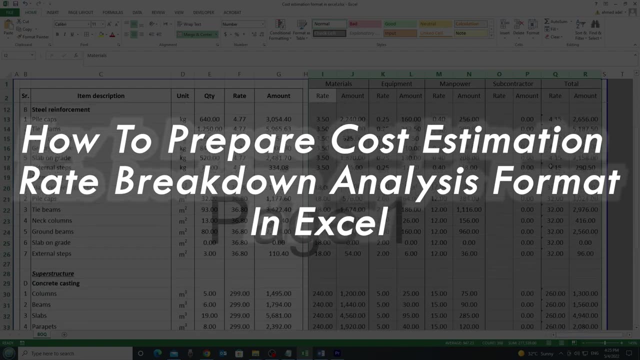 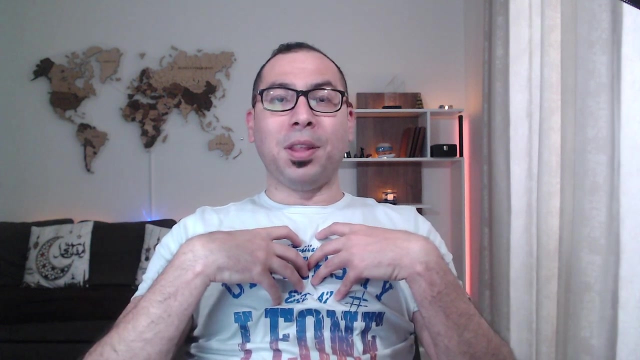 In this video I'll show you how to prepare cost estimation rate breakdown analysis in Excel, starting right now. Hello and welcome to Cost Engineering Professional. I am Ahmed Adel and here I help you develop the required skills and enhance your knowledge to elevate your cost. 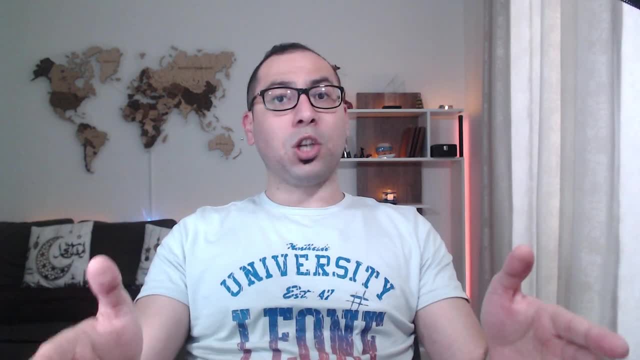 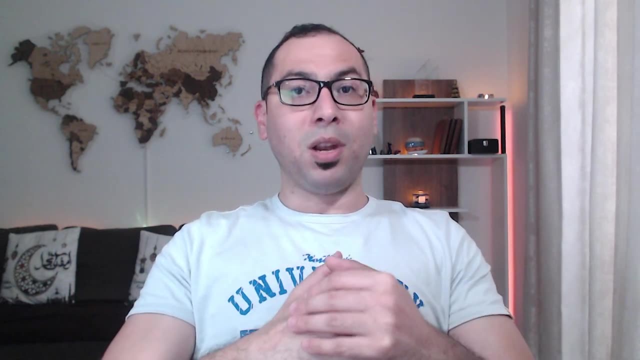 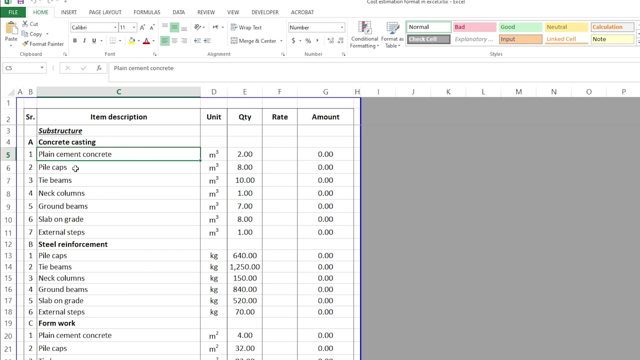 engineering career. So if this is something that you want, this channel is for you. Okay, with this out of the way, let's jump to the screen and see how can we do the cost estimation rate breakdown analysis format. So, as you can see here, I have a BOQ that is for some substructure works and some 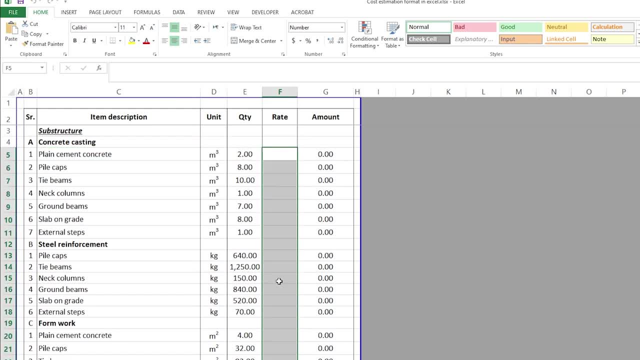 superstructure works and I want to estimate the cost. So that standard or the normal BOQ, you will find that the rate column is just one column where you can put the rate or whatever and you get the amount. But this is not what I want. I want to.